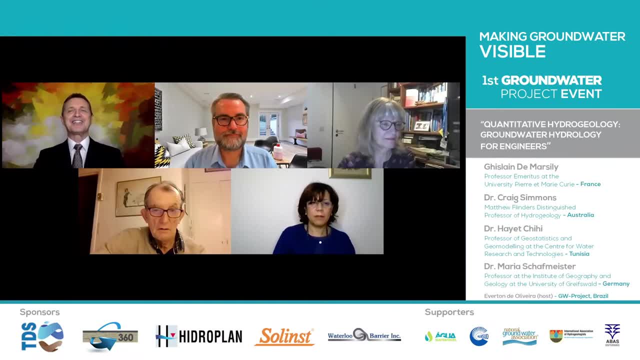 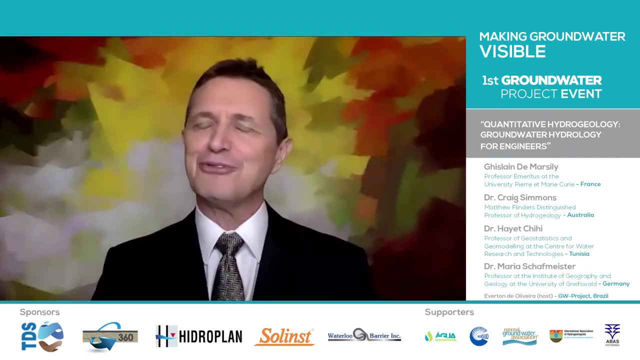 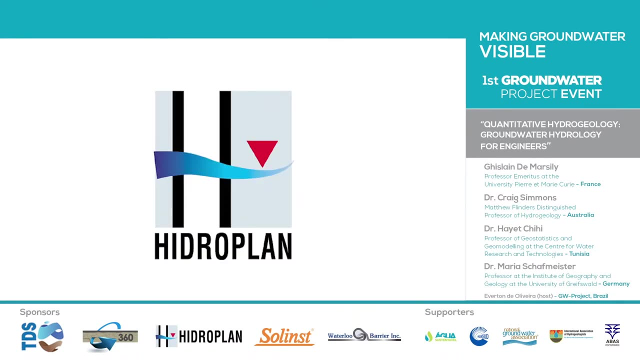 visible And, before we start, I would like to thank all our sponsors for making this event possible and free for all of you. TDS, Technical Development Solutions from Saudi Arabia. Hydroplan, a consulting company from Brazil. G360, from the University. 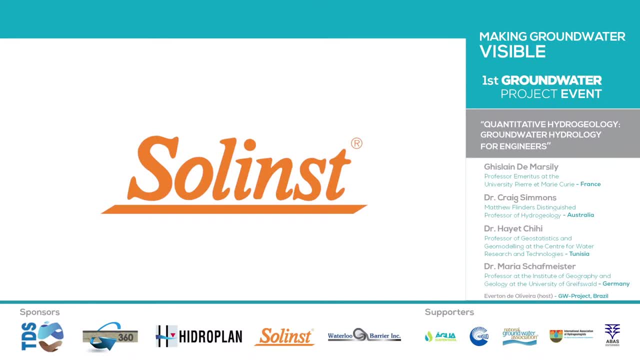 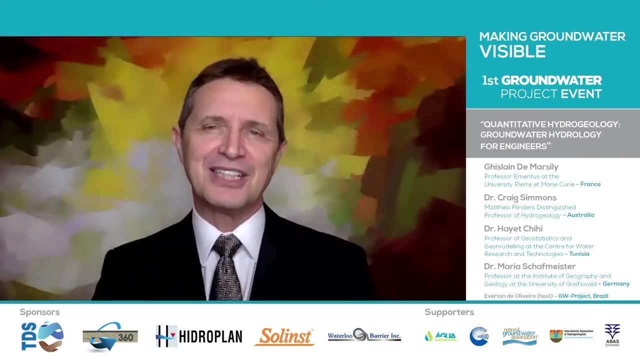 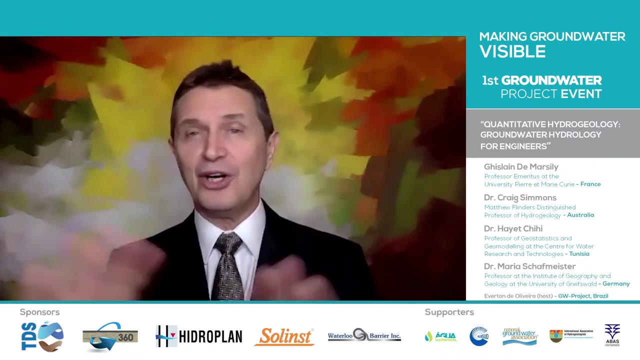 of Guelph in Canada, Solinst Equipments from Canada And Waterloo Barrier also from Canada, Hydroplan from Brazil, a consulting company, G360, from the University of Guelph and Waterloo Barrier, And also to all the individual donors. Without them, this noble endeavor, 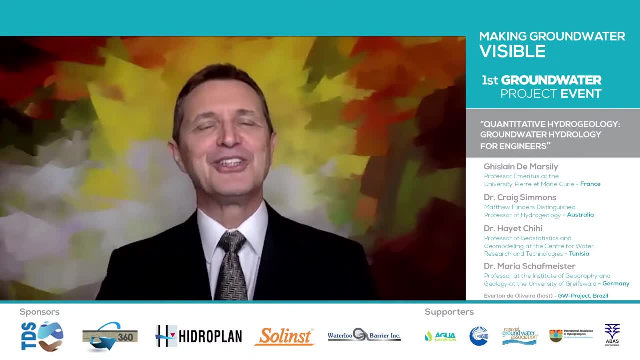 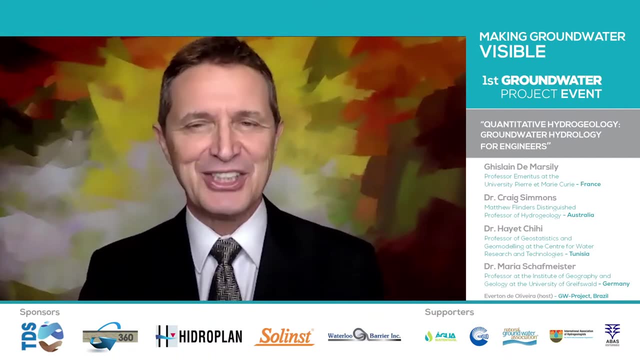 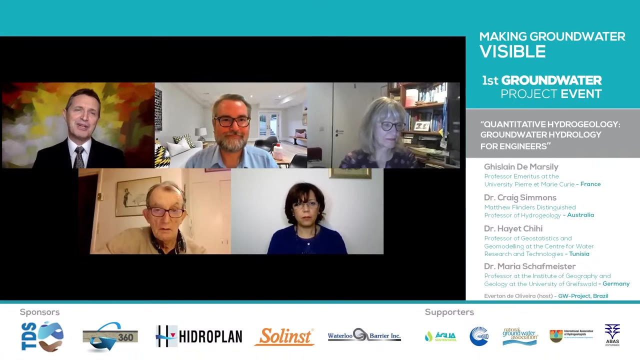 would not be possible. Please join them, Donate if you are an individual, or add the name of your company as a sponsor to a game-changer initiative. Okay, Lead by example is a very used-up expression, but here today it fully applies to our main speaker, Professor Guylain de Marseille. 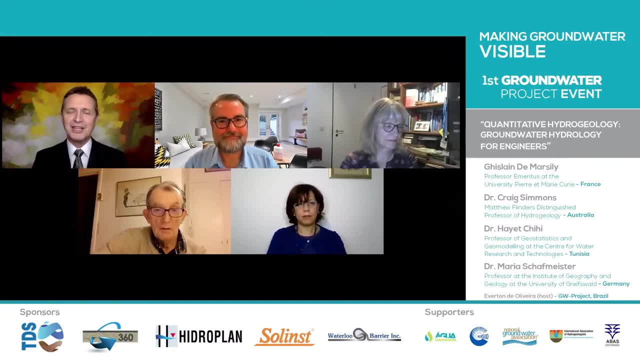 Professor Emeritus at the University Pierre-Henri Curie in France, He has an impressive career spanning from groundwater to food production- yes, passing through so many topics with such competence that he could easily give us that guilty feeling of being too lazy. On top of it, he is very friendly and generous. 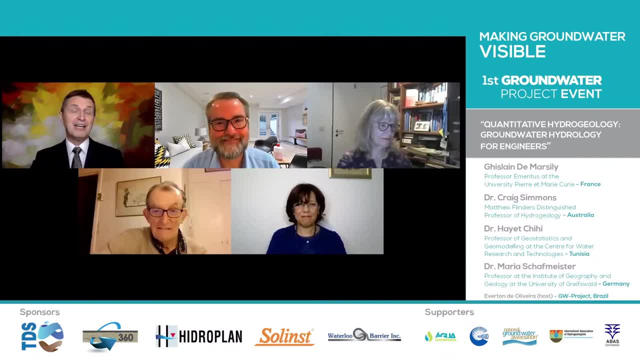 with his students and colleagues in particular, and with everyone in general. He produced books in French and English and are an early supporter of our groundwater project. We thank him for that. We'd like him to lend us his prestige to help spread the hydrogeology knowledge even further. 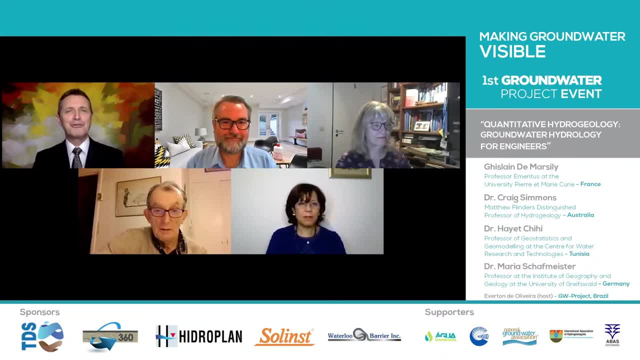 To make company to Professor de Marseille. we have three of his former students and colleagues that have been that have an impressive career of their own To talk about their careers and the push that they have to achieve. we invite Professor Guylain de Marseille to join us. Please join us. 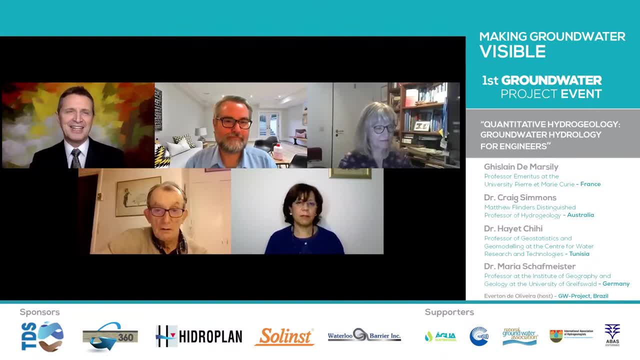 They are: Dr Craig Simmons, a Metro-Flinders Distinguished Professor of Hydrogeology in Australia. Dr Hayat Chihi, Professor of Geostatistics and Geomodelling at the Center for Water Research and Technologies in Tunisia. Dr Maria Schaffmeister, Professor of the Institute of Geography and Geology. 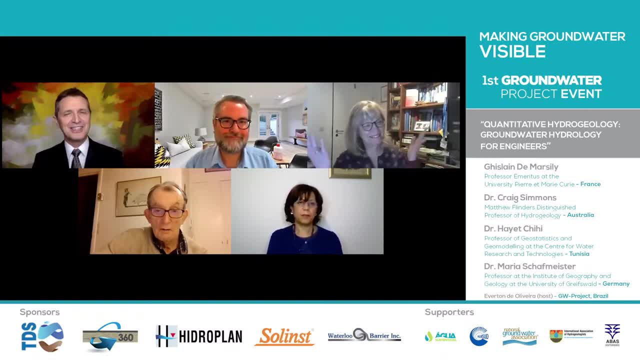 at the University of Graceland, Indonesia. Professor in Gearcheology at the University of Graceland and Professor in Geo-Geology at the University ofviously of Geology and Geology at the University of Greifswald of Jesus. my, my German is so poor, sorry for that. Greifswald in Germany. I hope I've got it. 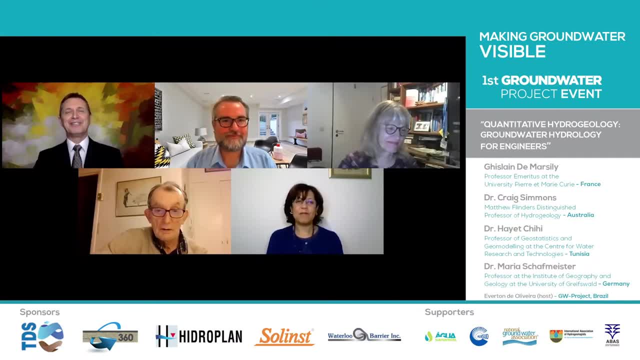 right this time. so I would like to thank all of them for their willingness to participate, especially Professor de Marcedie, from his dedication, and Professor Hyatt, who most kindly helped me put this session together. thank you very much, and please. now I'd like you to make a brief introduction about yourselves. Professor Guillain, you start a few lines about: 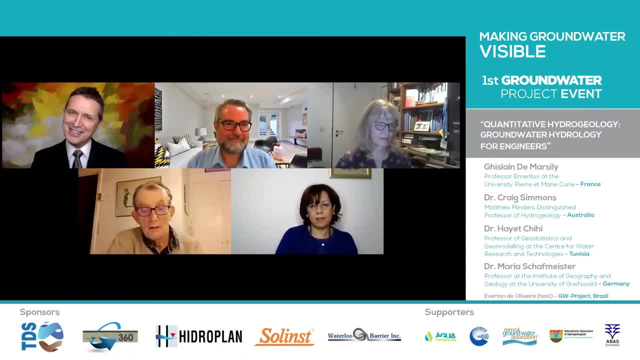 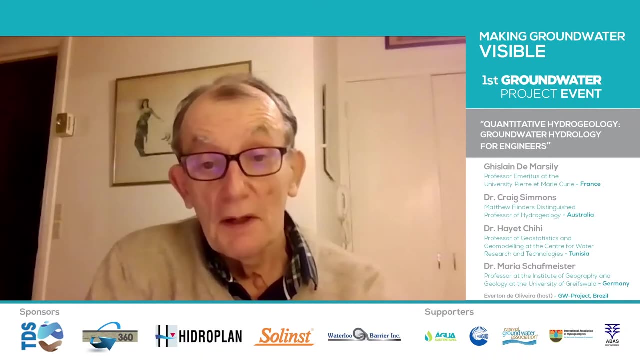 yourself if that was necessary. I know it's unnecessary, but let's be formal. make an introduction about yourself, please. well, thank you. thank you for the invitation and thank you for organizing this session. what can I say about myself? I think my initial degree was mining engineer, so I'm basically an engineer, and 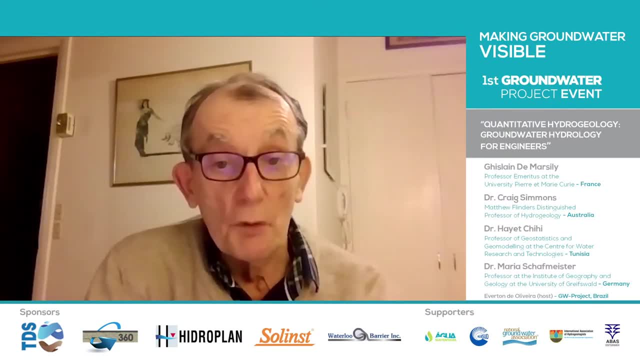 that will be translated in the writing of the book, which we will discuss in a moment. I wanted to study geology at the Paris School of Mines, but I was prevented to do that because, as many of you know, I have problems with my legs. I cannot walk very well and the Professor of 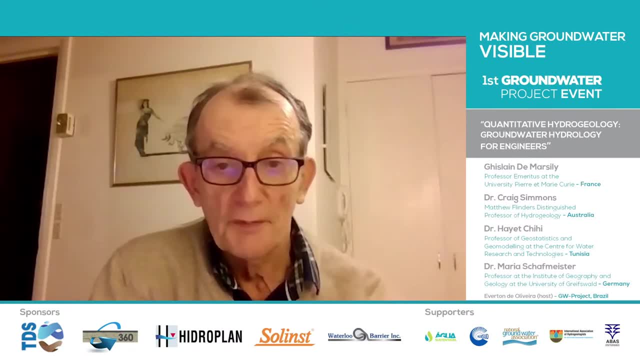 Geology, whose name was Jean Gauguel- he was an excellent professor- said: I don't want you in my office, but geologists must know how to walk, so get out of my office and do something else, not geology. so that was a sort of a disappointment for me, and I studied fluid mechanics instead of 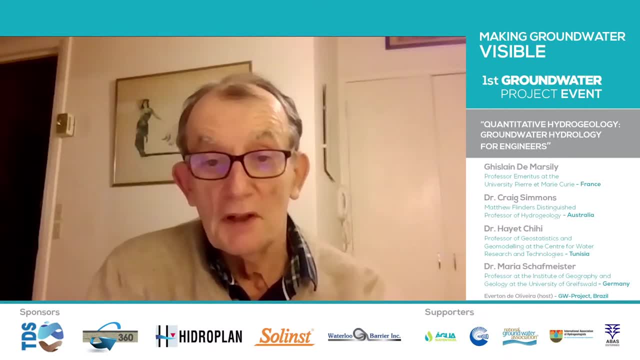 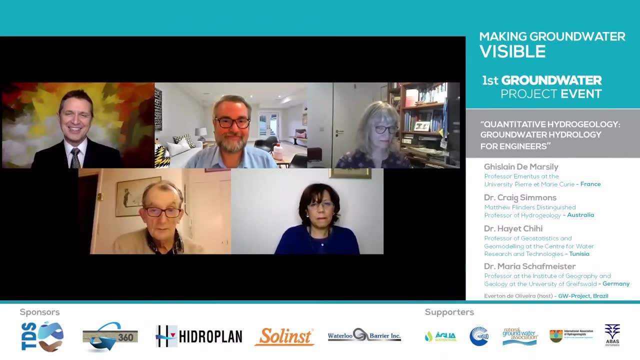 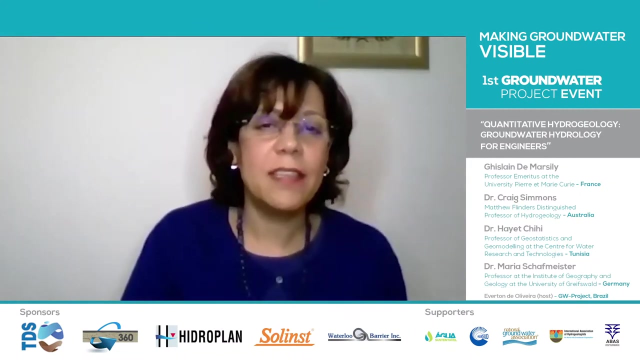 geology, but I took courses of geology later on in my career. oh, thank you, we're so glad you stayed on that's. that's so good for us. thank you very much, please, Hyatt. you're next from Tunisia. I am a professor at the Center for Water Research and Technologies. I am a teacher. 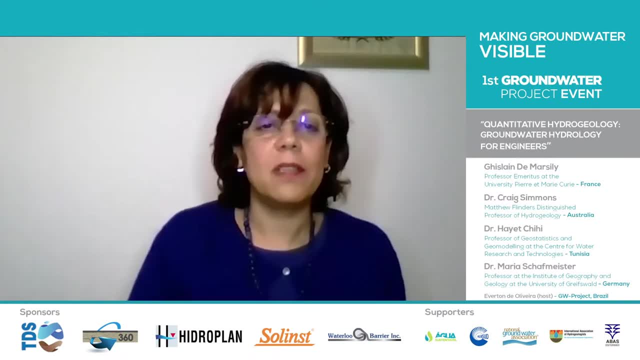 also at a few universities in Tunisia. I'm teaching your statistics mostly, and geomodeling. I have some projects that I am leading with my students, my colleagues from Tunisia and from International University also. uh, I've been a PhD student, a fortunate PhD student- of Guilain-de-Mercelis and his team. help us, me and my students, and I am grateful for that. thank you. 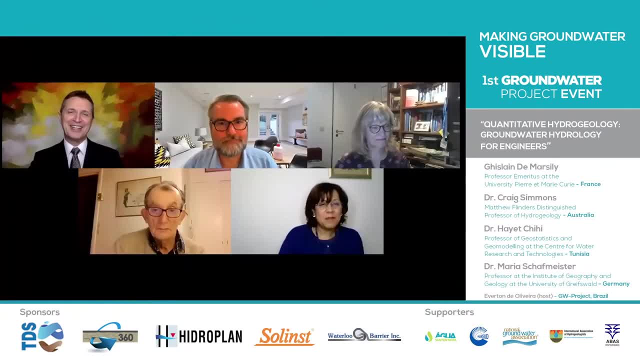 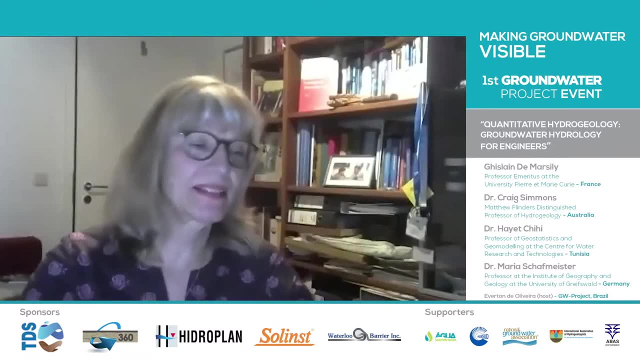 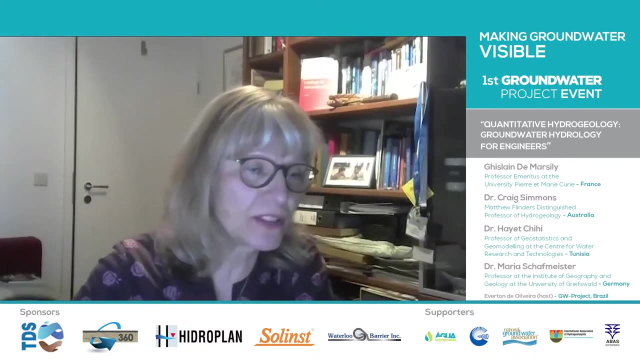 thank you very much. we are- we all are great grateful for that. um, Maria, please. yeah, my name is Maria Theresia Scharfmeister. I'm professor for Applied Geology and Hydrogeology at Greifswald University. uh, actually somewhat similar to your career, not so good, but 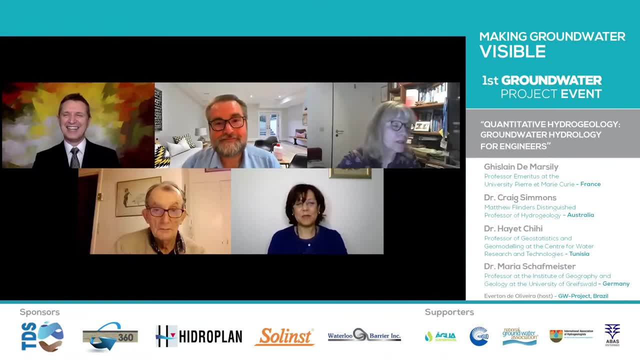 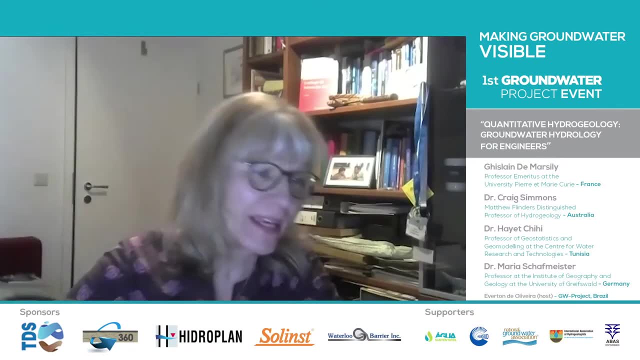 also I wanted to. I wanted to become a paleontologist. that was my goal, and I didn't achieve this because hydrogeology came into my way, and it was because of quantification hydrogeology that I wanted to do that. only the professor didn't want me. 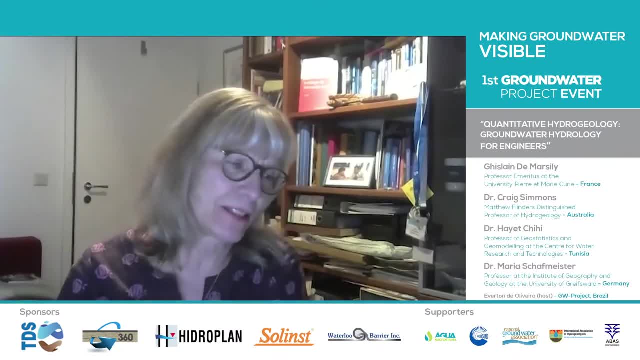 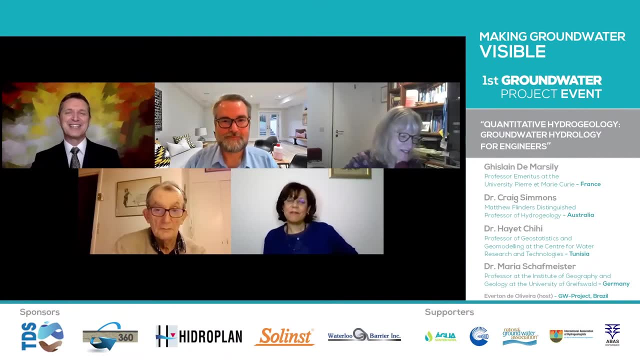 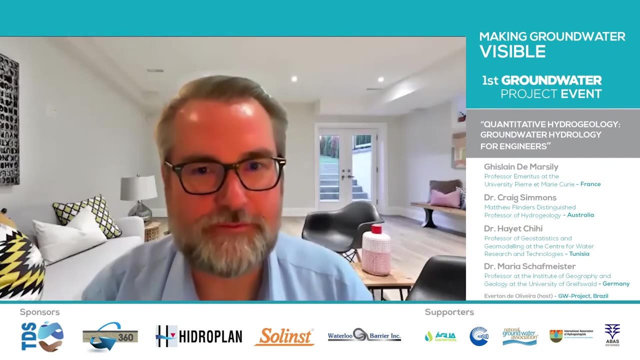 so I had to make a little detour, going by mathematical geology. that's my brief life, thank you very much. thank you very much. your turn, Craig, please. yeah, thanks, Everton, and it's a real pleasure to be here. I'm really honored to participate. so, um, but my background actually. 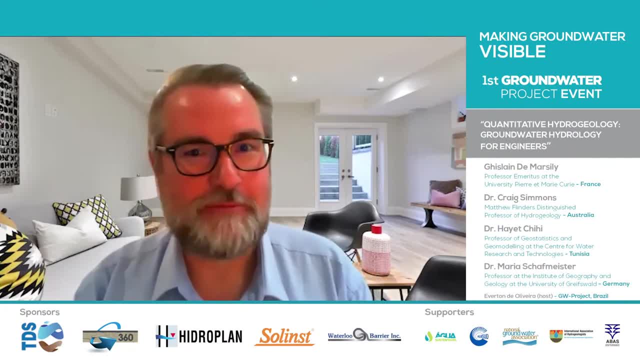 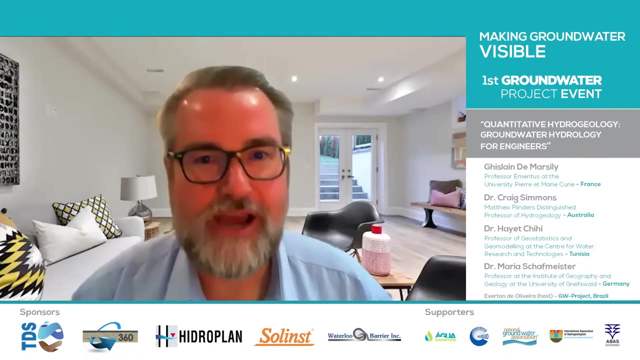 started out in Electrical and Electronic Engineering- So people often say water and electricity do not mix- And I had a slightly sort of contorted and detoured background as well. So I did engineering, followed by physics, and then had the fortune of doing a PhD in hydrogeology at CSIRO in the 1990s, where I got into groundwater modelling. 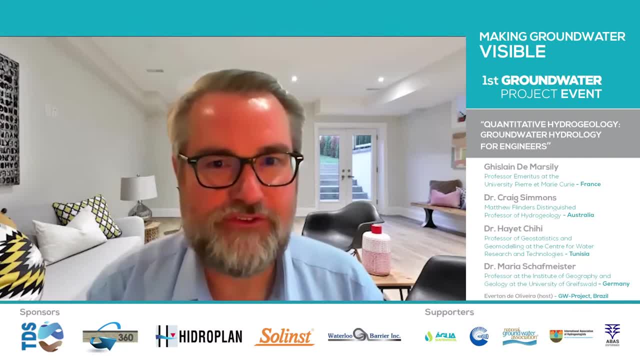 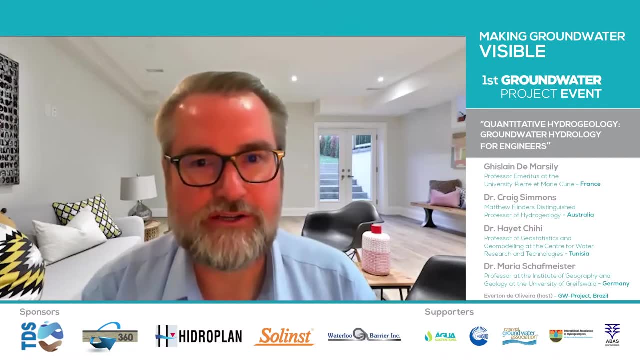 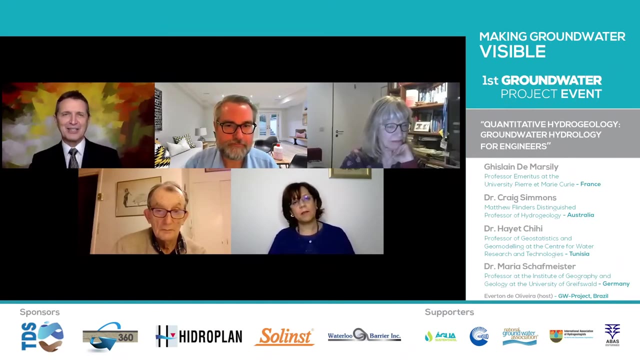 I'm now a professor of hydrogeology at Flinders University here in Australia and also the foundation director of the National Centre for Groundwater Research and Training in Australia. Thank you very much. Thanks for all of you for participating in that. It's a great pleasure and an honour having all of you here today. 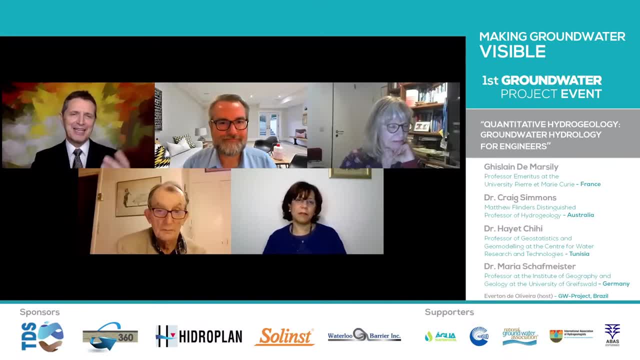 Now please, Guillaume, could you make your presentation please? It's not really a presentation, It's a A little bit of a story of how I came to write this book, Quantitative Hydrogeology, which is chopped up there in my shelf. 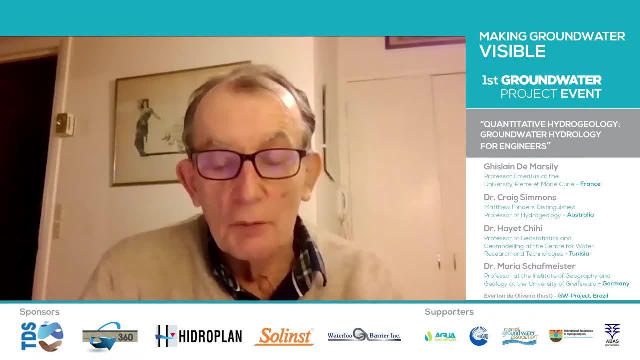 The story is that I was doing research in groundwater hydrology at the Paris School of Mines in Fontainebleau And with three months notice- advance notice- I was told that I should start teaching groundwater hydrology to the École des Mines students. 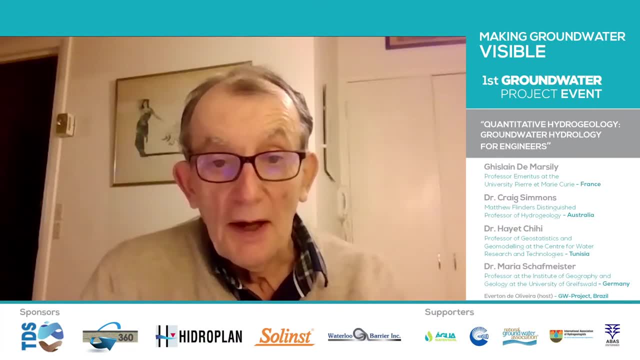 And so I said, OK, I shall be ready to teach the next quarter, next fall. So I had three months to prepare course. I had no experience in teaching. Therefore I said: what can I do to be ready in three months to teach a course which was going to be 30 classes? 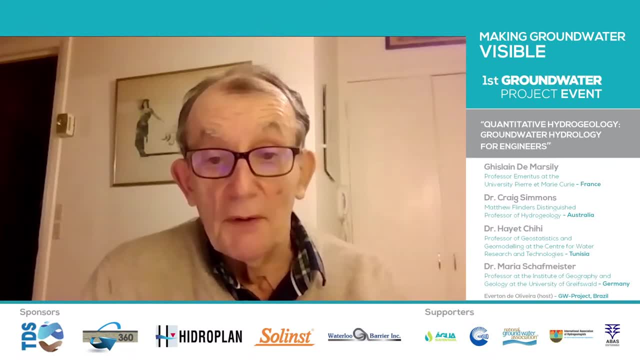 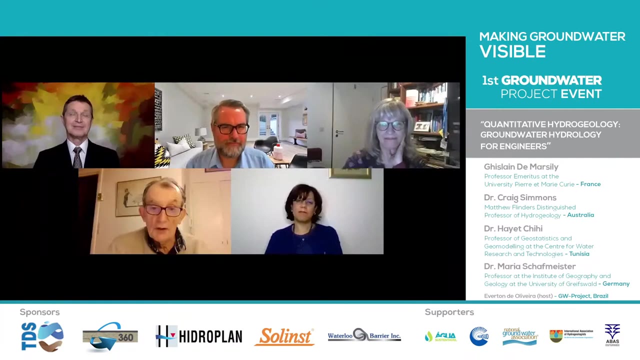 So it's long. So I started to read old books in French, in English, in German, in anything, And it's very presumptuous of me to say that, But let me give some final Million tubing. I read what I wanted to teach. I wanted to teach counter-hydrology, starting from basics. 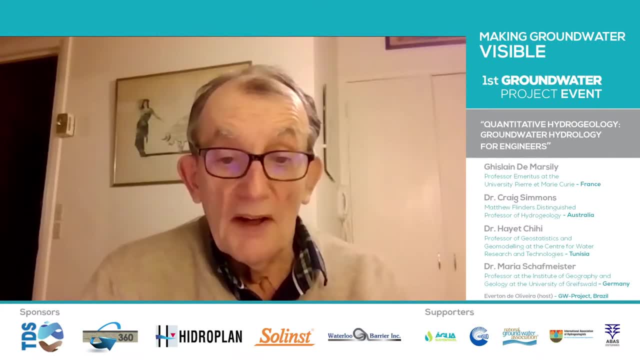 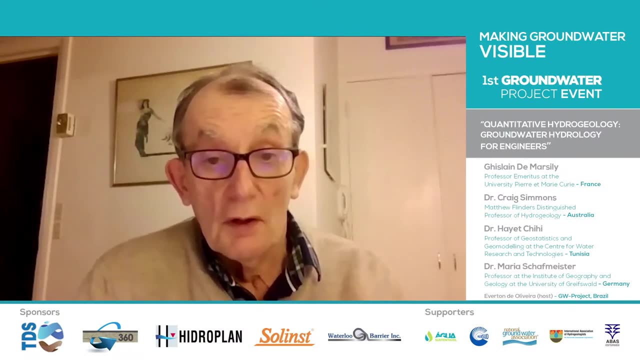 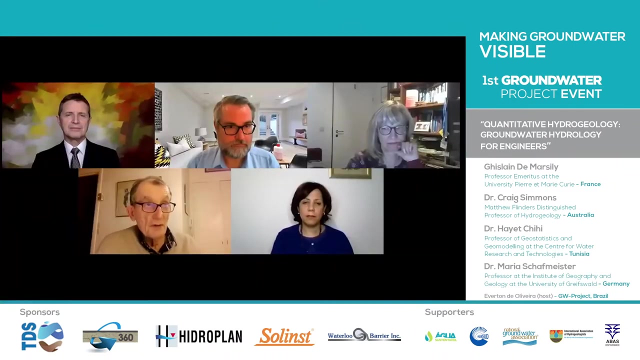 You know, for instance, in fluid mechanics, any problem of fluid mechanics is to quantify seven magnitudes, which are the pressure, the mass per unit volume, the viscosity, the three components of the velocity vector- and I forgot one: viscosity. and 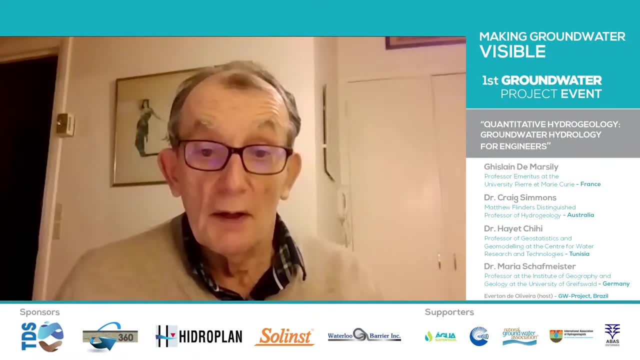 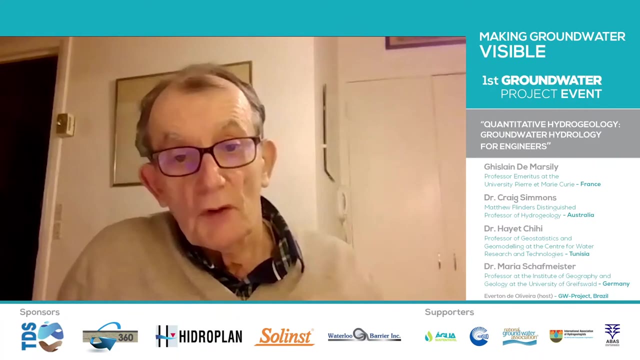 temperature, of course. So in order to solve any groundwater or flow problem, you need to write seven equations which enable you to calculate these seven magnitudes. So you know, I thought it was interesting to start the book by coupling it with fluid mechanics. 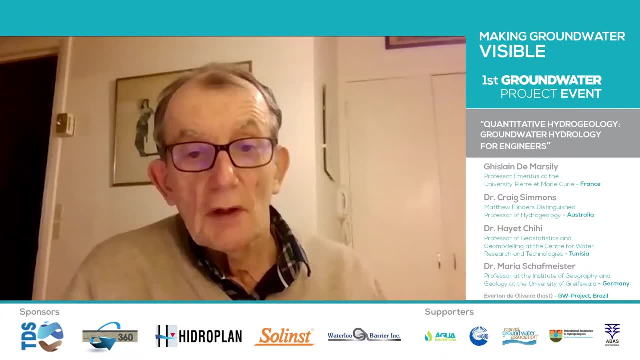 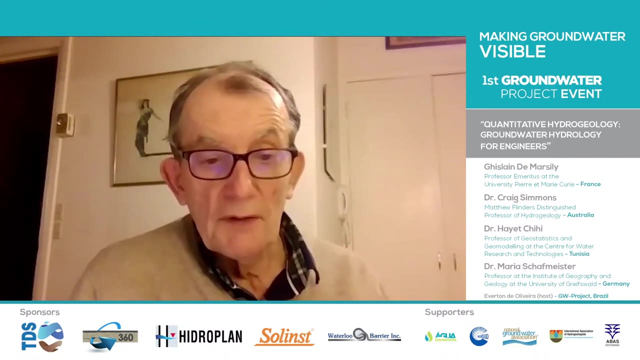 in general, And I understand that hydrogeology is the use of fluid mechanics in a particular medium which is very complex and which needs to be described in detail. So that was the start of the book And I think the books I had read prior to doing my course were doing that in a 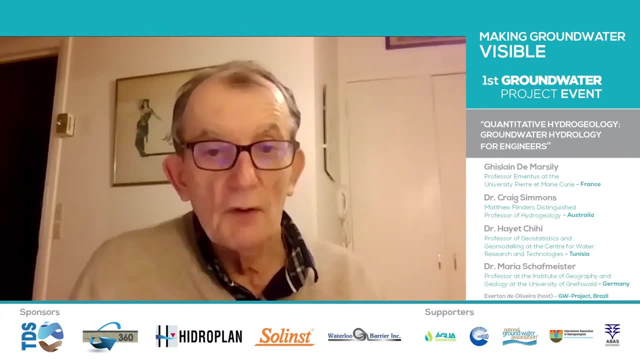 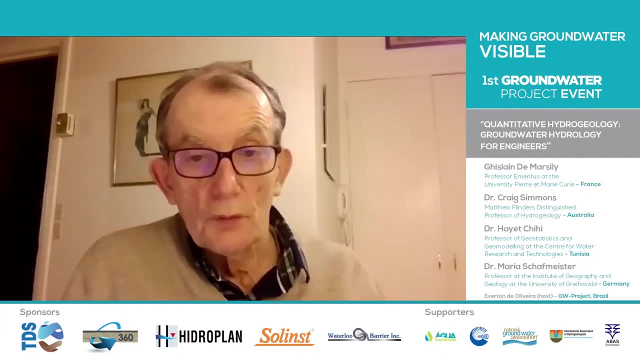 way or another, but not systematically. You start from physics, which you know, mechanics when you know, and then you build up the equations that you use to solve the groundwater problem. So the second thing I wanted to do is to put the context of hydrogeology not in a fluid. 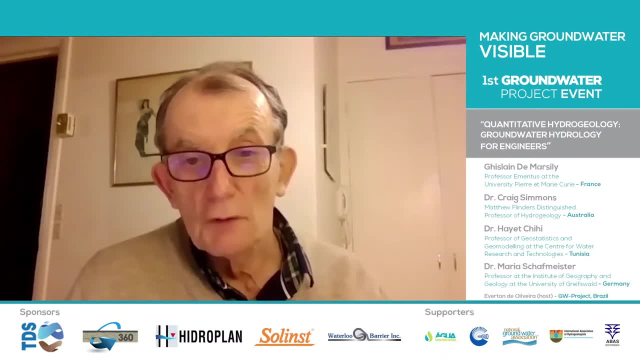 mechanics framework, but in a geological framework, because we are talking about geological layers, we are talking about viability of the properties of these layers and all that needs to be taken into account from the start. So I wanted to give you a little bit of background on that. So I would 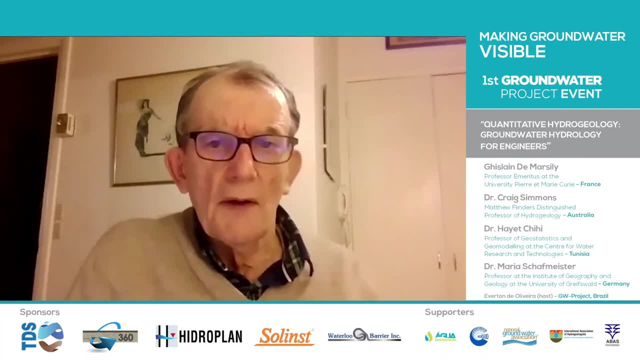 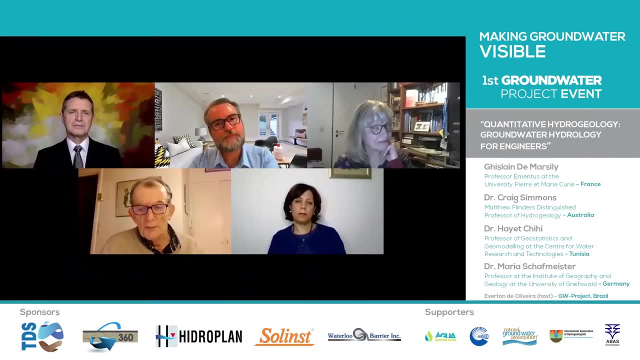 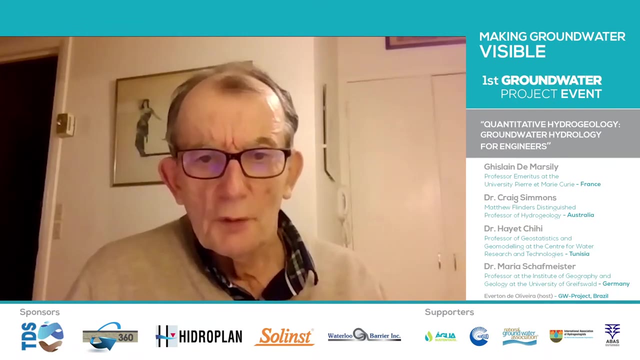 like to combine these two things: fluid mechanics on the one hand, and geology, heterogeneity, natural system and so on. So that's what I tried to do. So I was not able to complete my course before the start of the course. So I was a little bit worried because I had to teach. 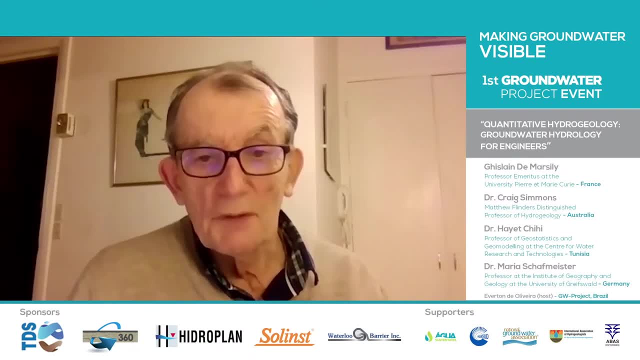 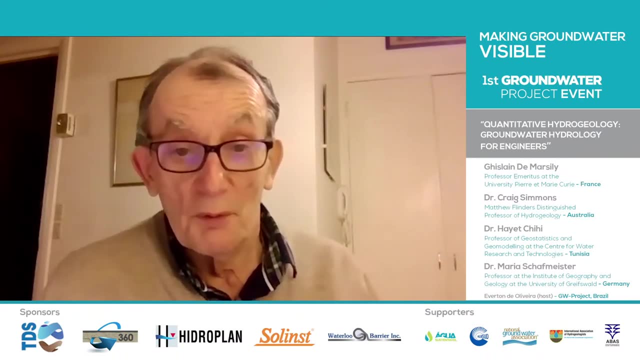 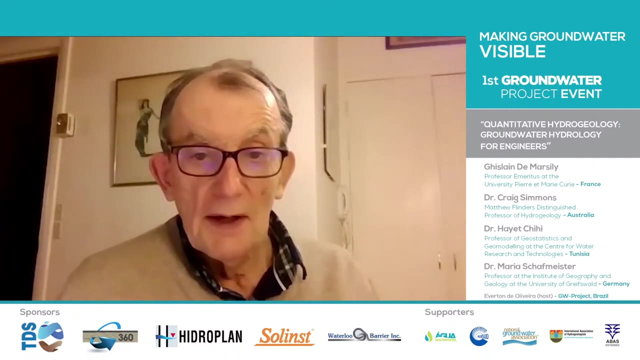 And so what I did is that every night before the class started, I had to work until past midday night to be sure that I would prepare the material I needed. So, in order to have the students follow me, I decided I would like to have a sort of the handwritten textbook that I would distribute to 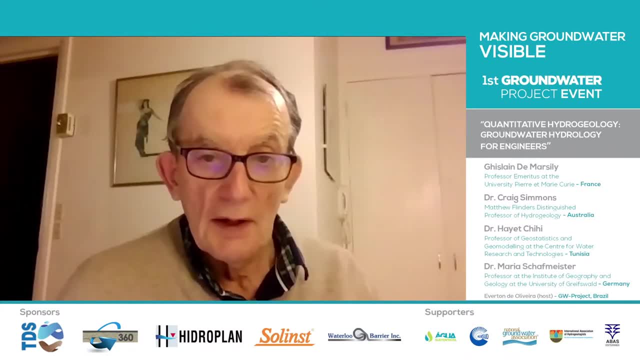 them so that they can look back at the note, at my notes, and use that for for the learning, for the ending of the class. So the book started that way. It was, I would say, semi finished in. I think this started in 73. after the first class, the first year of 30 classes, i had something which 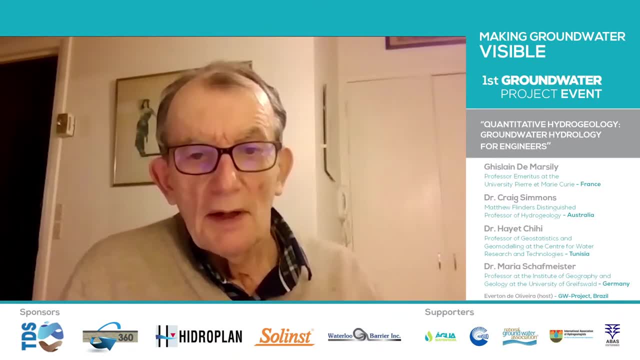 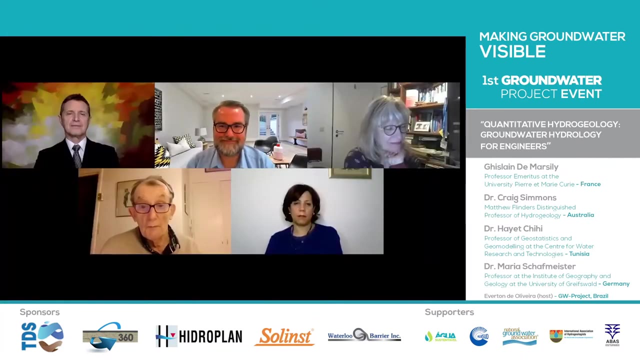 you know was not perfect, but at least had the material in, and so i modified and improved and polished those chapters in. uh, in the following classes and in, i was approached by a french editor, which you know because you've seen the french version of my book, which is masson, and 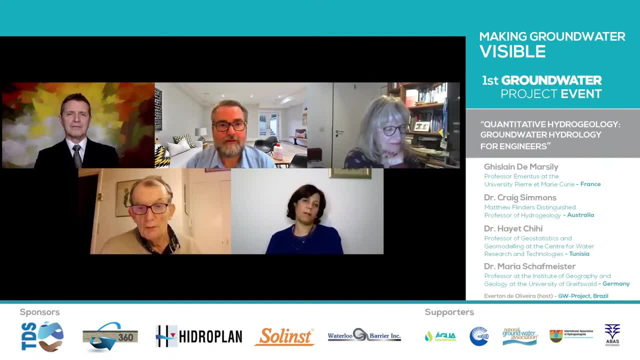 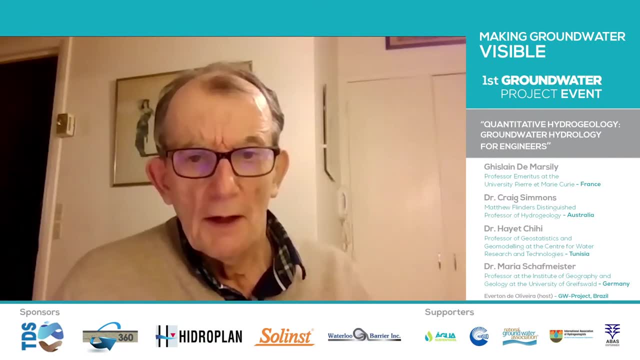 they said: well, your notes are interesting, why don't you make a book out of it? so i did that and i wrote in french. it was short, it was much shorter than the english version, and that was published, and in 81, in 1500 copies. and the book was never reprinted because it sold rather fast. 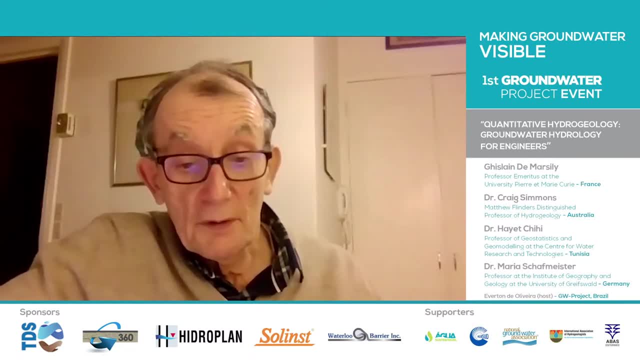 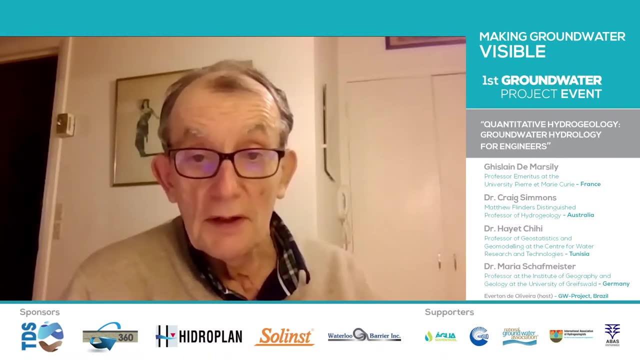 but masson was not interested in that and it's uh, it was abandoned, i would say. but then i had the luck to with to meet a colleague at the canadian colleague whose name is dick jackson, dr dick jackson, who is in fact american, but he moved to the 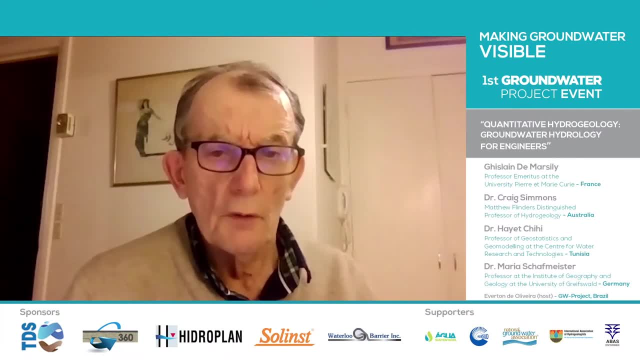 us. he lived in canada and then he came back to work for the us company called intera in austin texas and he was doing consulting and he was an excellent hydrogeologist, so he could read french and of course he spoke english and he found my book on. 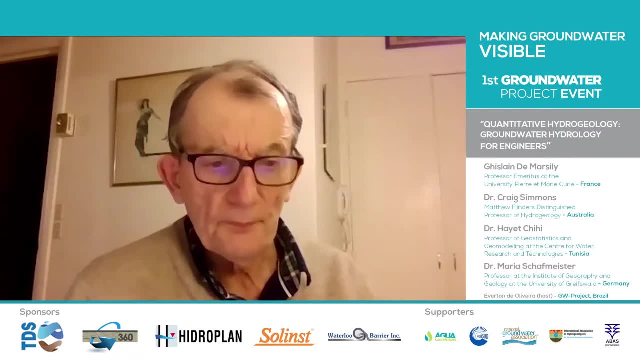 in a library or in a bookshelf and he came to me and he said: you know, this is very interesting what you've written, and the same book does not exist in english, so i encourage you to translate that book and put it into english. and also where he said: i didn't have that in mind. is that well? 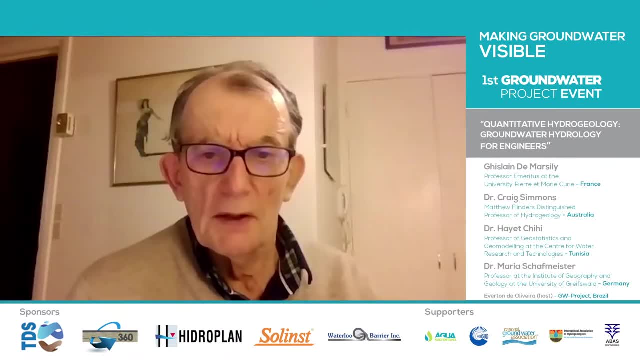 french in france. one technique which is being developed is geostatistics, which of course applies very well to hydrogeology, and there's nothing written today in hydrogeology and geostat, so why don't you add the chapter on geostatistics applied to hydrology, which is 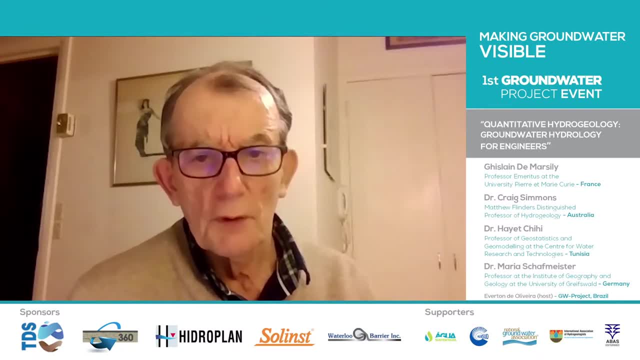 what i did, what i did. so the book evolved by this suggestion of dick jackson, who is a good friend, and he's still a good friend, and i had some difficulties convincing us publishers to publish that book because they found or they thought that the book was too complex and would 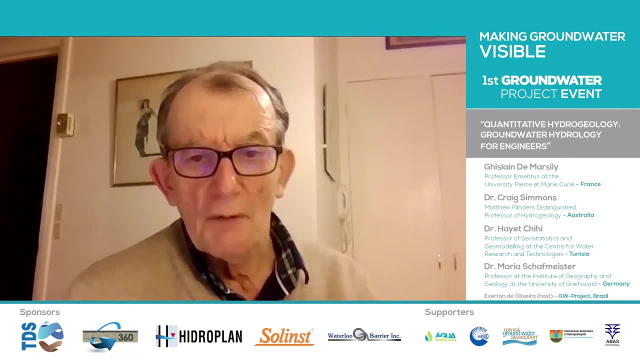 not feed the needs of average american students, which he. it turned out that it was wrong because i think the american students who took, who used that book for textbook in master degrees, surely really i think they, i hope at least they- liked it. so this is certainly the way the book was. 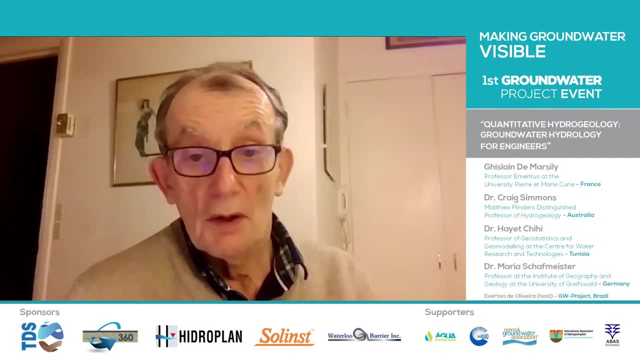 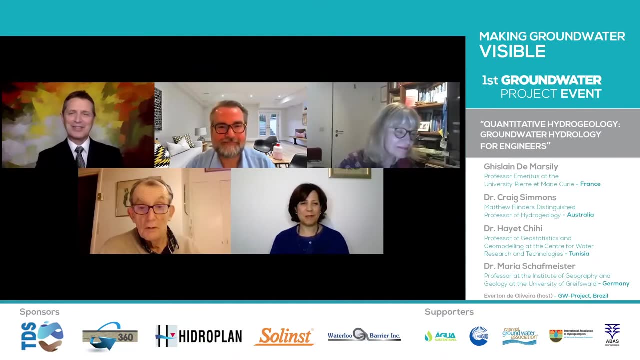 completed. it's because of the pressure added by dick jackson, which i thank for what he did. it's a very good story, quite interesting, quite interesting. so, and uh, was it the book translated to another language- english and french? no, i forgot to say that the translator for my book to french 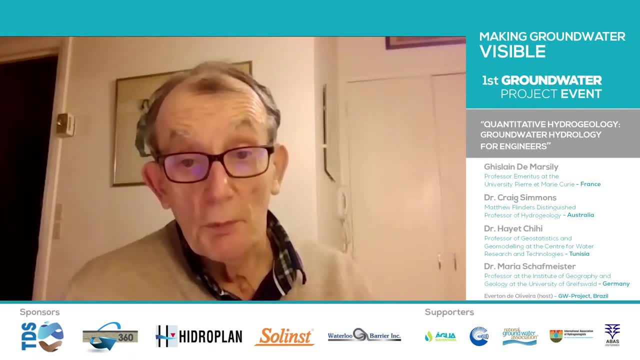 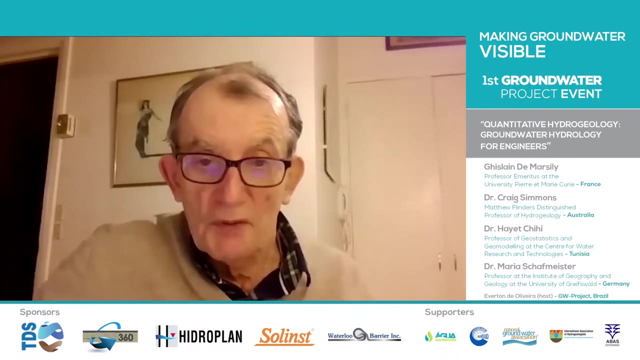 from french to english was done by my wife. my wife is a professional translator and we work together. she did the english writing, and i'm not a judge, because i speak french in principle, or mainly french, and my english is well shaggy. so, uh, but i think what? 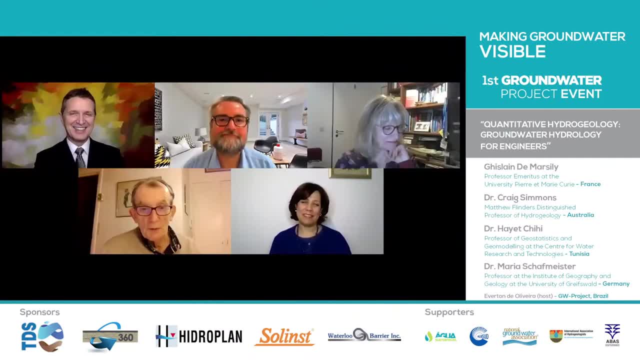 she did is good, so i'm i'm glad that she helped me to do that. no, i'm not a great judge because i speak portuguese, but yeah, for me your english is very good. thank you all right, thank you very much. well, we'll we'll. we'll dig into your information a little later. just let's, let's listen to the. 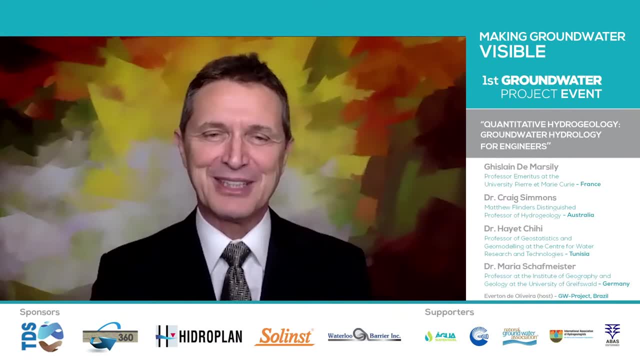 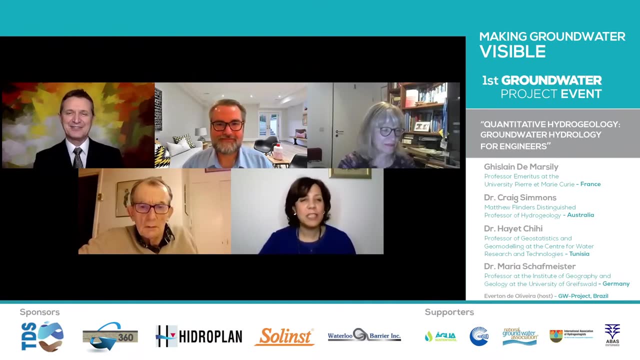 others and then we'll go back to you just a moment, you know. thank you very much for now. let's go. hi, you're next. yes, we can't share the screen, please, you, you, you can, you, you have to share, please, you have to share from your computer, uh, so, uh, i'm going to uh listen that uh, the, the, the. 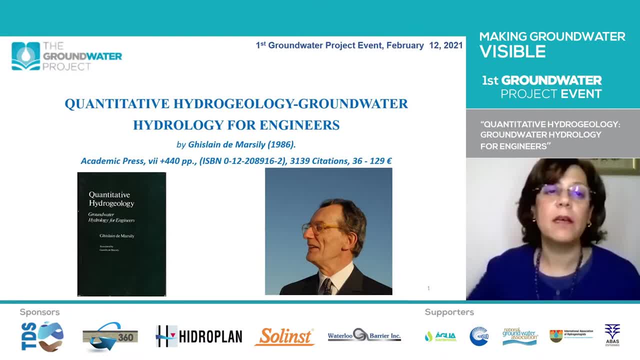 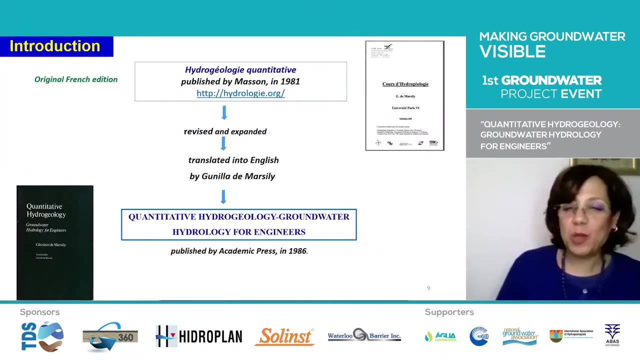 the classic book of the classic book of uh guillain-marceli entitled the quantitative hydrogeology- groundwater hydrology for engineers. so quantitative hydrogeology- groundwater hydrology for engineers- is a revised and expanded version of the original french edition entitled hydrogeology. 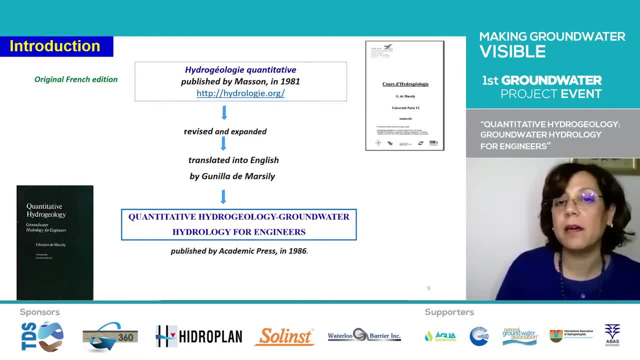 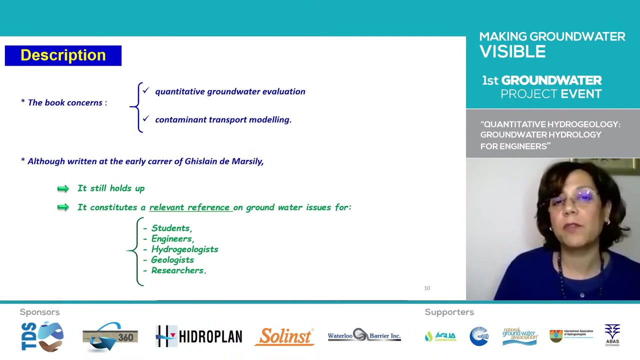 quantitative, published by masson in 1981. then it was translated to english by gulina de marceli and published in by academic press in 1986.. so the book concerns mostly of concerns mostly quantitative groundwater evaluation and contaminant transport modeling, although it was written at the early career of guillain-marceli. 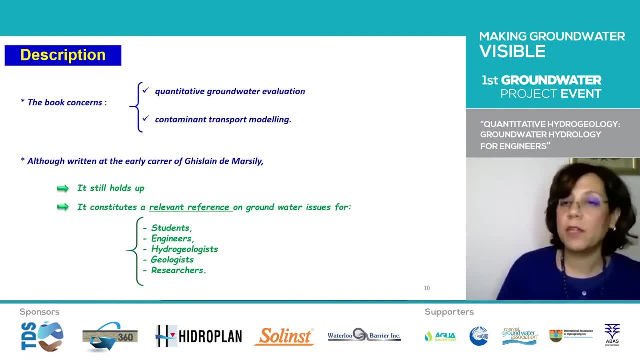 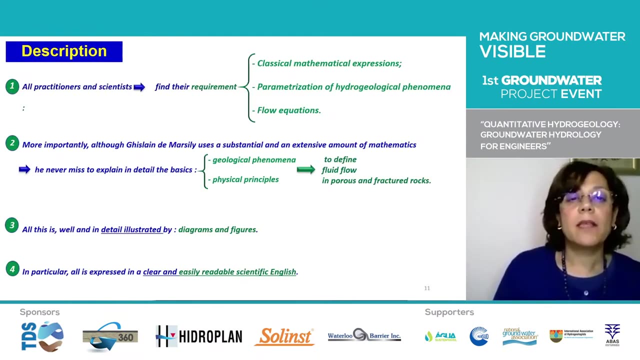 this book still holds up and it constitutes a relevant reference on groundwater issues for students, engineers, hydrogeologists, geologists and research in general. why? because all practitioners and the scientists will find their requirement from classical mathematical expressions and hydro parameterization, of hydrogeological parameters, to flow equations. more importantly, although 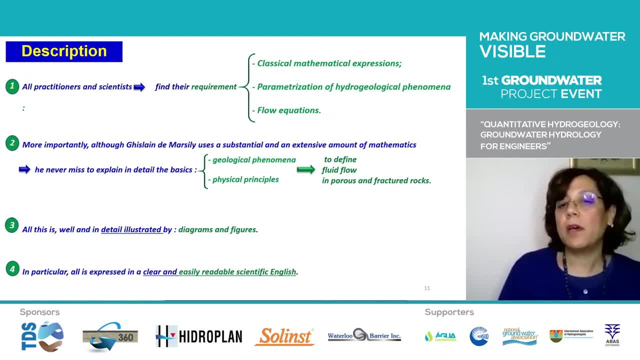 the de marijuana uses a substantial and extensive amount of mathematical equations. he never missed to explain in detail the basics of the issue, with the geological phenomena and the physical principles to define the fluid equations in force and fractured media. All this is well illustrated and in detail. 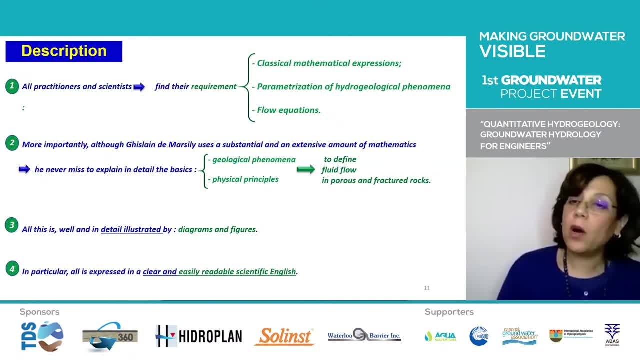 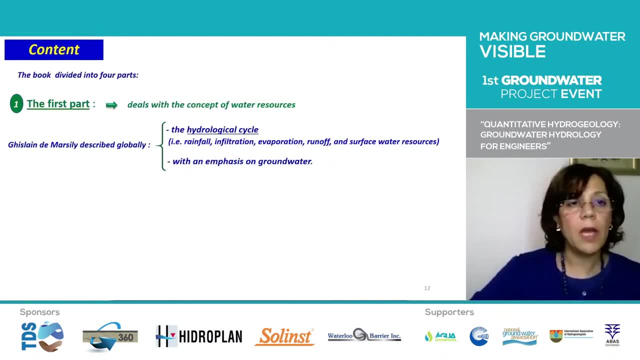 by diagrams and figures. In particular, all is expressed in easily readable scientific English. For the content, the book is subdivided into four parts. The first part deals with the concept of water resources, where Guylain de Marsilly described globally the hydrogeology cycle, with an emphasis on groundwater. 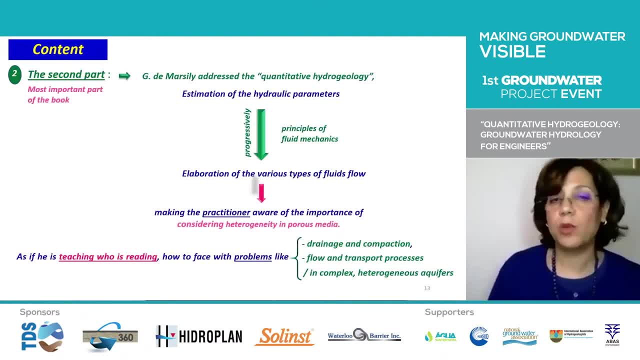 The second part, which is the most important in the book, Guylain de Marsilly addressed progressively the quantitative hydrogeology, from estimation of the hydraulic parameters to the elaboration of various type of fluid flow. And this is the first part. This is then followed by adopting: 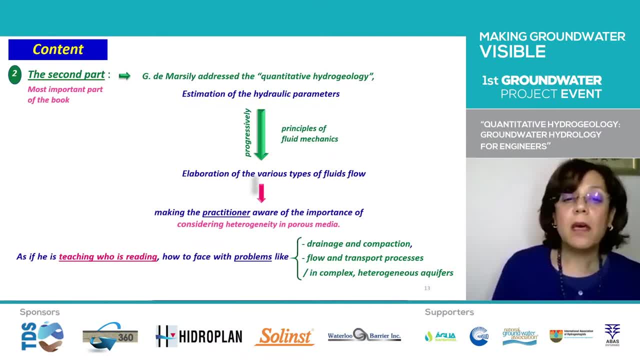 by applying principles of fluid mechanics, making the practitioner aware of the importance of considering and integrating heterogeneity in forced media and in aquifers, But this is done in a manner as if he is teaching the reader how to face with problems like drainage and compaction flow. 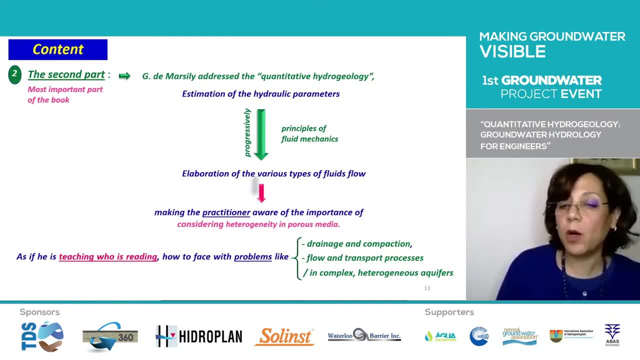 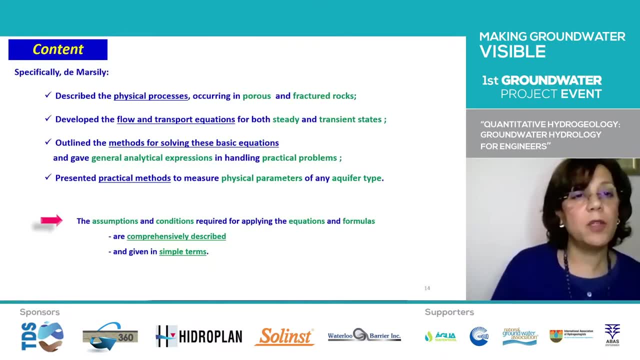 and drainage transport process, all this in complex, heterogeneous aquifers. Specifically, de Massilly in this chapter describes the physical process occurring in porous and fractured rocks. Also, he developed the flow and the transport equations in both steady and transient states And he outlined the methods for solving these basic equations. 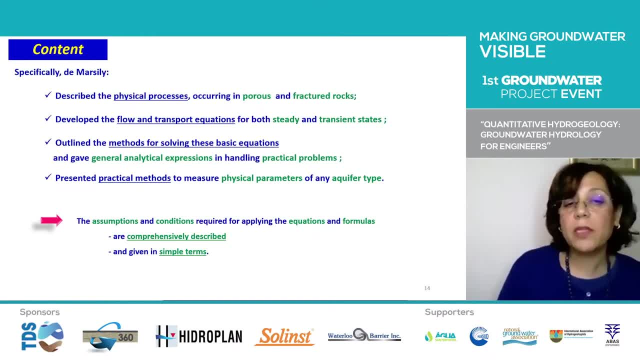 And, finally, he presented practical methods to measure the physical parameters and the properties of any aquifer type. All the assumptions and equations required for applying these formulas and these equations are comprehensively described, and in simple terms, In the third part, Guylain de Massilly. 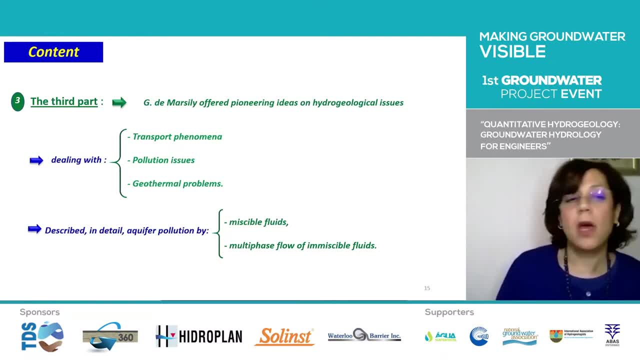 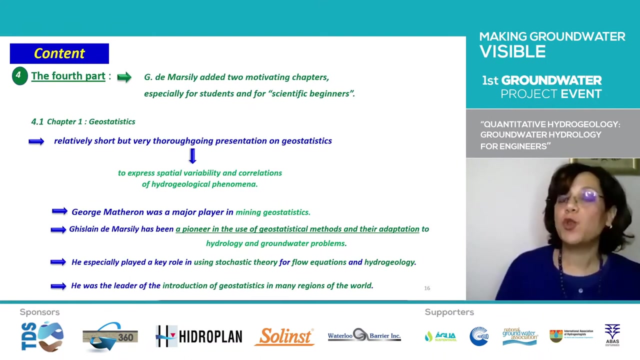 offered ideas on hydrogeological issues dealing with transport phenomena, pollution issues and geothermal problems. He describes in detail aquifer pollution by emissive fluids and the multi-phase flow of emissive fluids In the fourth part, Guylain de Massilly. 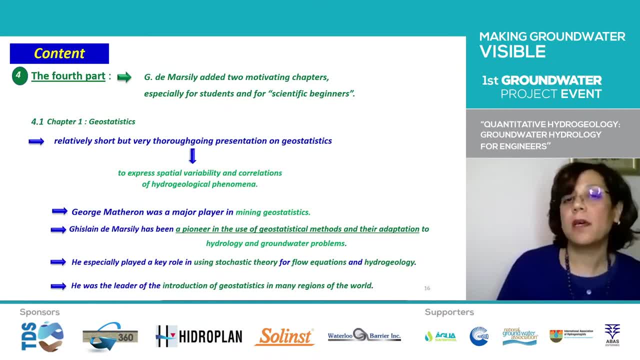 added two motivating chapters, especially for students and scientific beginners. The first chapter deals with geostatistics And this is presented in a relatively and but thoroughly presentation to express the spatial variability and correlation of the hydrogeological parameters. I would like to say something about geostatistics. 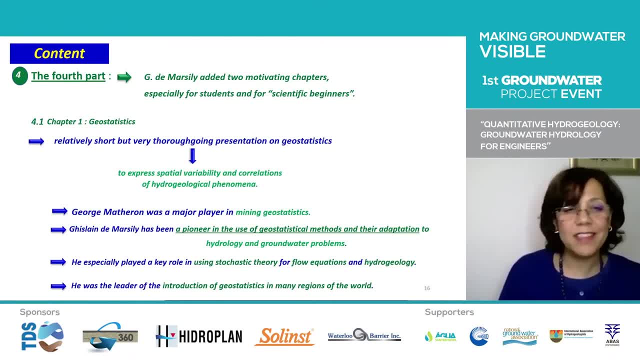 because I was in the center of geostatistics and I know very well Georges Matteron, But his was the major in mining geostatistics. Guylain de Massilly is the in introducing geostatistics in hydrogeological issues and problems. 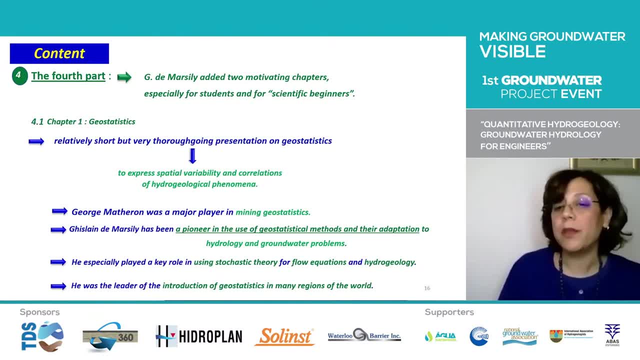 Principally he introduced the stochastic theory in the equation and in the estimation of the hydrogeological parameters. Also, he was the first to introduce geostatistics in many countries in the world, And at the beginning it was in the USA. 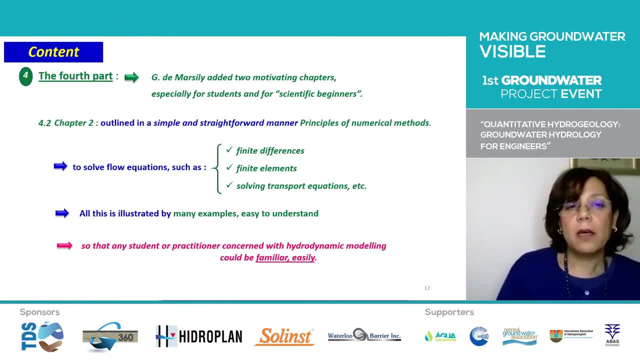 The second chapter in this fourth part, Guylain de Massilly outlined in a simple way the principle of numerical equations to solve the flow equation, such as the finite differences, the element differences and solving transport equations. All this is illustrated by many simple examples. 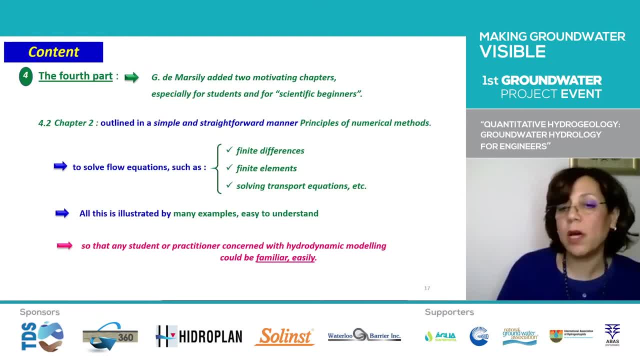 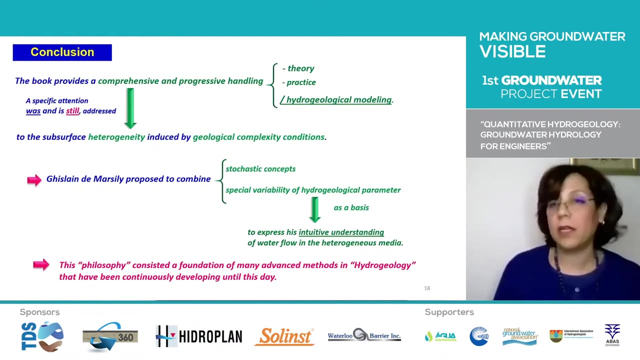 so that any student or practitioner concerned with hydrodynamic modeling could be familiar with easily Presenting this book in this manner. I could say that the book provides a comprehensive and progressive holding of the theory, the practice in hydrogeological modeling. Specific attention was and is still addressed. 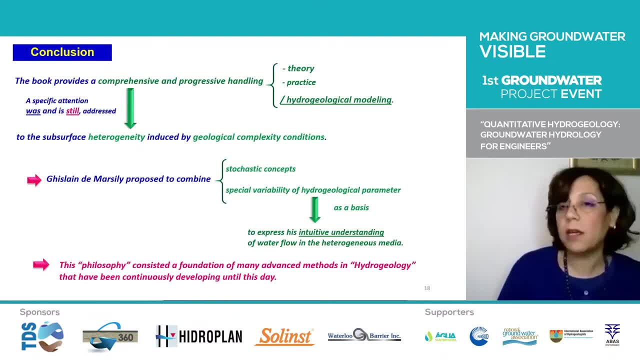 by Guylaine de Marcelly in introducing heterogeneity and complex geology in hydrogeological modeling. For this, Guylaine de Marcelly proposed to combine the stochastic concepts and the spatial variability of hydrogeological parameters and variables as a basis to explain his intuitive understanding. 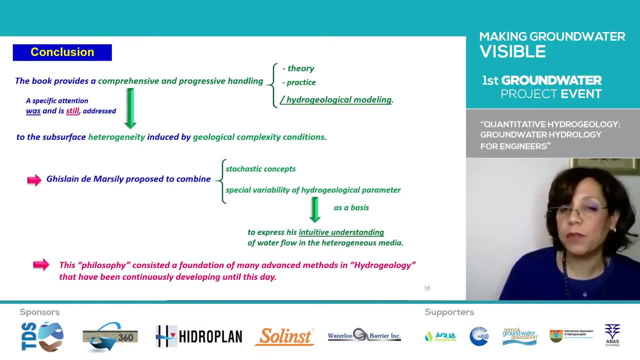 of water flow in heterogeneous aquifer. I think that this is a philosophy which constituted a foundation of many advanced methods and research in hydrogeology that have been continuously developed until this day, And this, I think, will be more developed by my colleague, Maria. 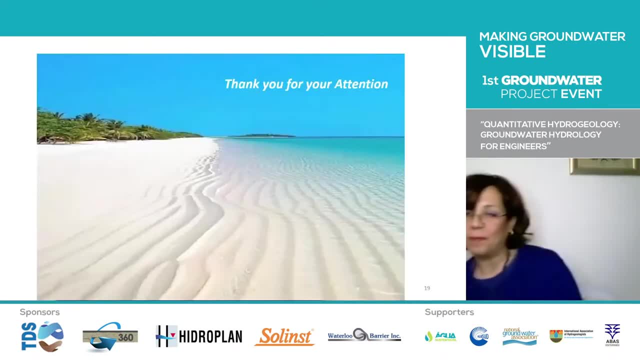 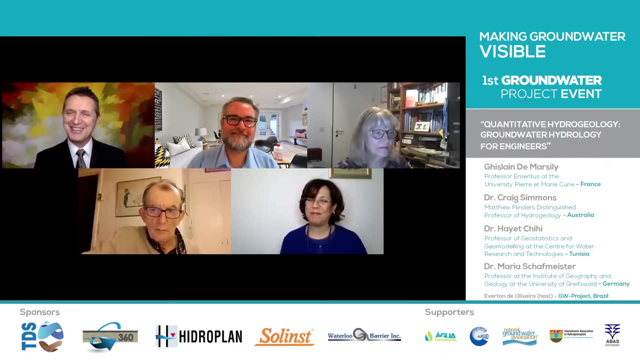 Thank you for your attention. Thank you very much, Haya. You started a bit shaky, but then you move along quite well. Thank you, congratulations. I thought that was the English right, But that was perfect. Thank you very much. 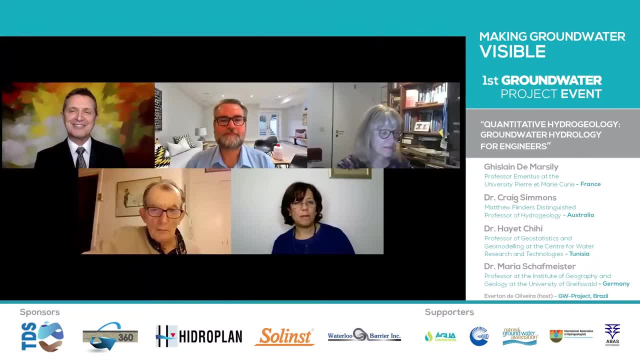 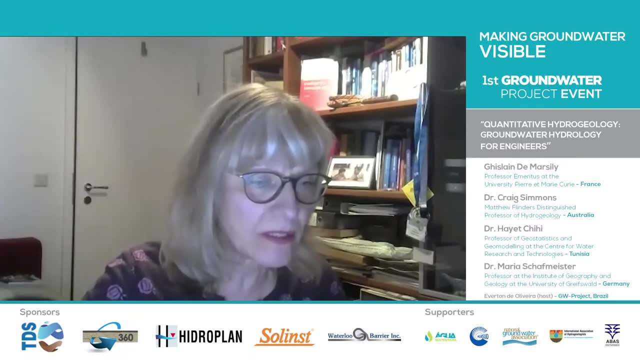 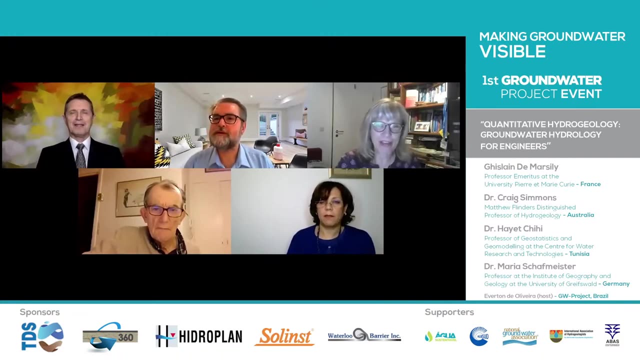 So, Maria, your turn, please. Yeah, Also, I'd like to give a little presentation. I hope it works. Can you see something? Yes, Perfect, OK, So we've now learned so much again about Guylaine's book. 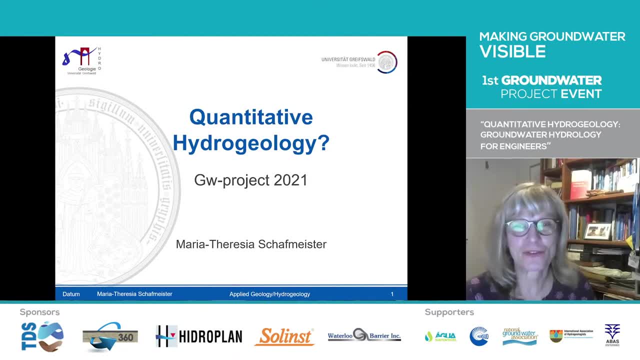 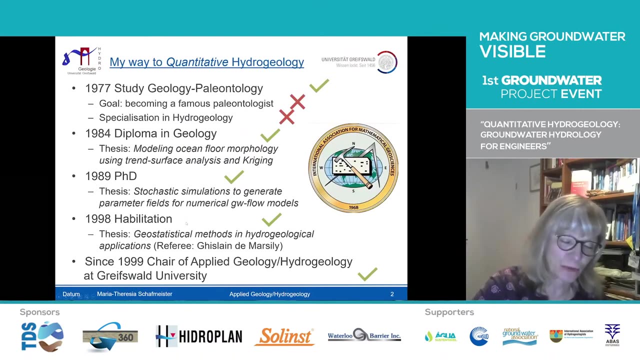 which we all knew. So I try to give a more general aspect Of quantitative hydrogeology, And you see that I put a question mark here First, still as I told you before what my way to quantitative hydrogeology was. 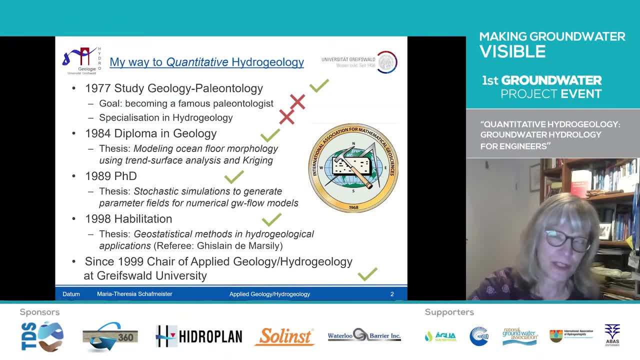 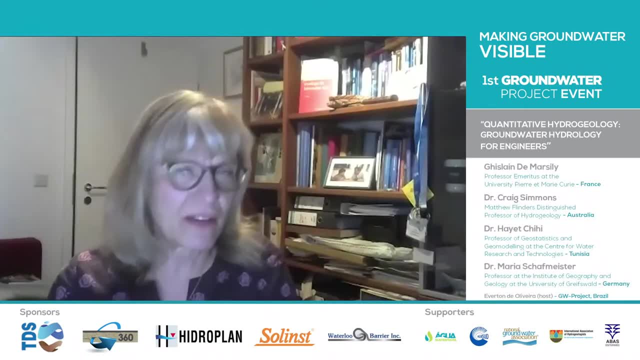 as I said, I wanted to become a paleontologist And it turned out this is exactly not what I'm trying to do, So describing things qualitatively. I learned very soon that I love to work with numbers and to quantify things. 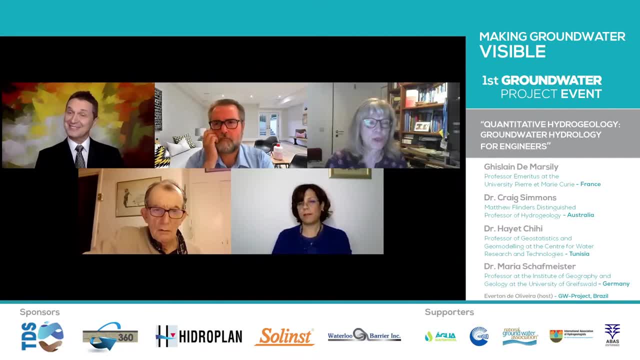 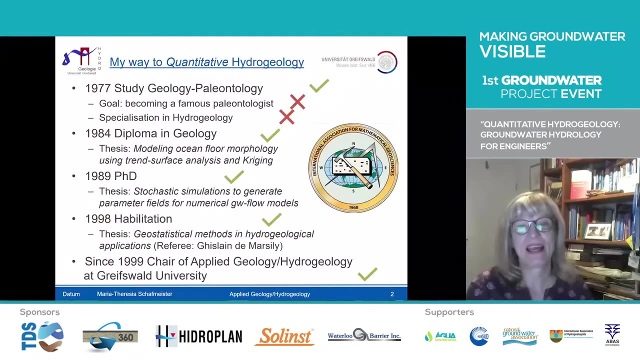 Not, as many geologists might do go to the field and say: well, we have a rock which is red and probably very, very old. So this is too qualitative for me. So, as I said then, I wanted to become a hydrogeologist. 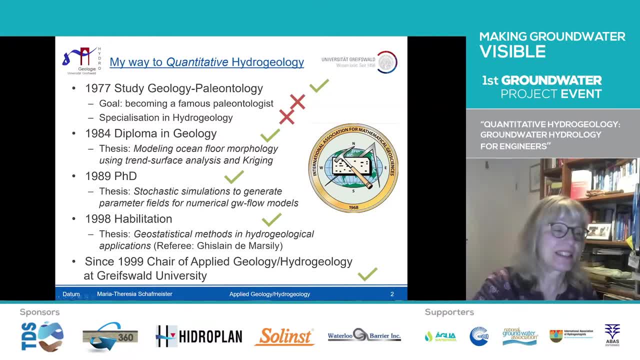 The professor didn't like me so I could not do hydrogeology. But then I turned, I did a detour and I came to mathematical geology, And you see here the emblem of IMG, the International Association of Mathematical Geology. 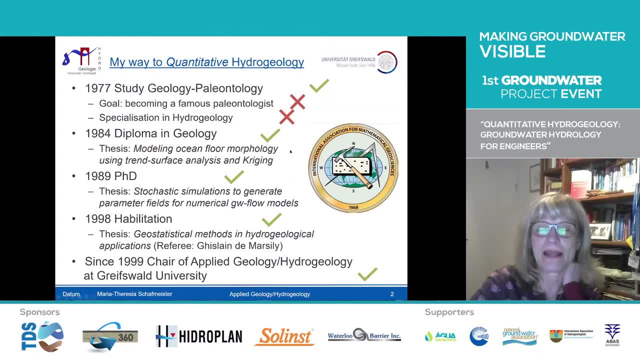 I put this here because it shows a little bit of my history too, Because I started at the beginning of the 80s to work with computers as a geologist. Geologists usually didn't like equations and computers, They like their hammer, which you can see here. 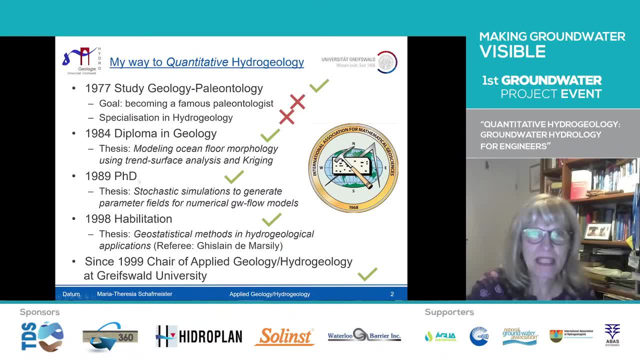 And so This was my big advantage, that I started to work with computers, with punch cards and everything, and programming in Fortran- to those who still know this name: Fortran, this language. So- and I did this detour and I learned something. 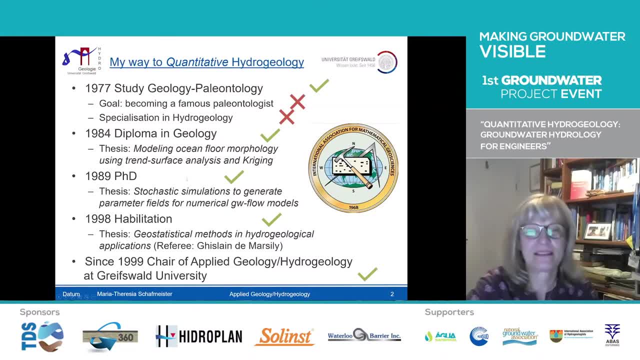 about geostatistics and my thesis was on Kriging and trend surface analysis. But then I made my way to hydrogeology. I started to learn groundwater modeling And my PhD thesis was on generating stochastic fields of hydraulic conductivity and other parameters to be used in numerical models. 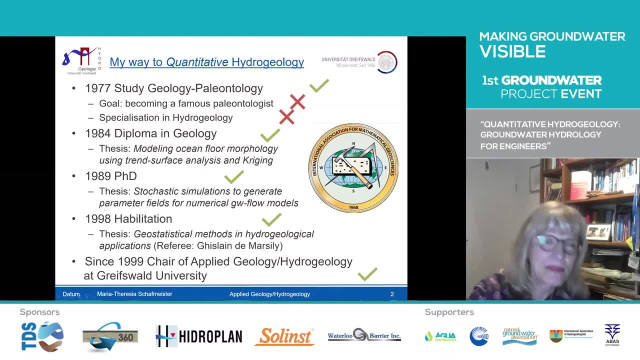 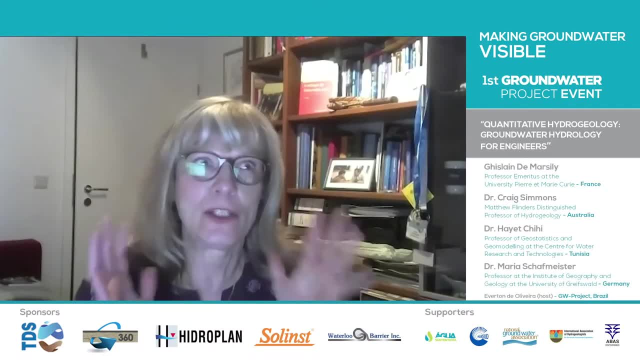 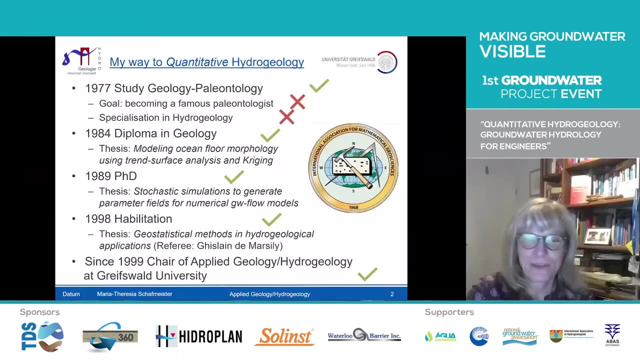 And this was my way here. And it was exactly this time, in 1988, that I first met Ghislain in person, And I was so amazed because I knew him, of course, from his books and his publications, And I said: to see this man was a great, great thing for me. 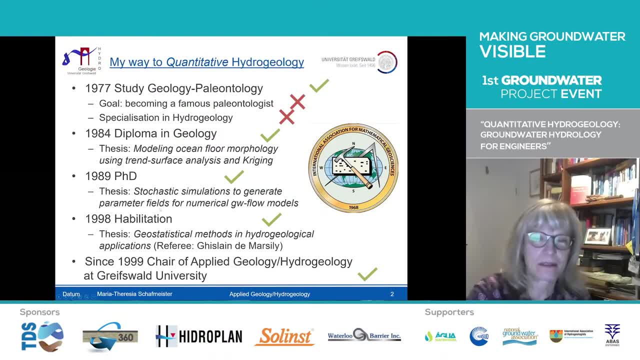 Then I did my habilitation. You know, in Germany we have the second PhD thesis, And I mentioned this because Ghislain was so nice to serve as referee of my habilitation, which was written in German. So thank you for this again. 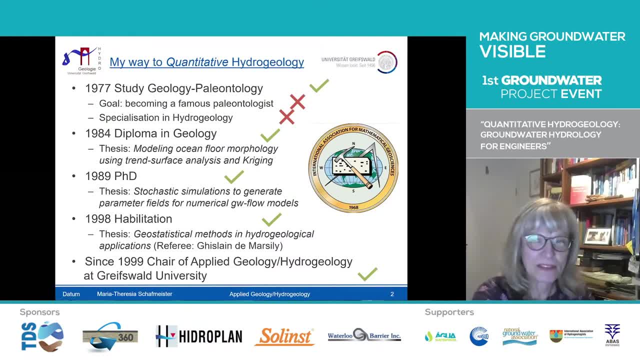 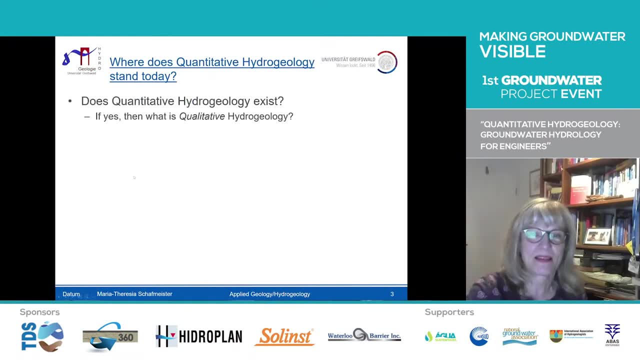 OK, This was a little bit my way to come to quantitative hydrogeology, But now I'd like to put a more provocative question. because does quantitative hydrogeology, Hydrogeology, exist? Because if it exists, this implies that we also have qualitative hydrogeology. 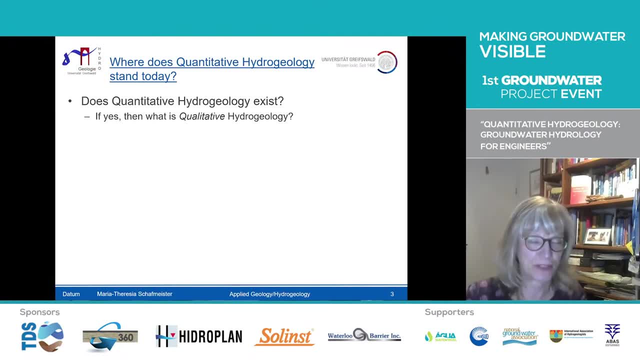 And actually I don't know what that should be: qualitative hydrogeology. We all know that it was those French engineers, Darcy and Dupuis, who first founded quantitative hydrogeology, before they even know what hydrogeology was, because the first definition of hydrogeology as we use, 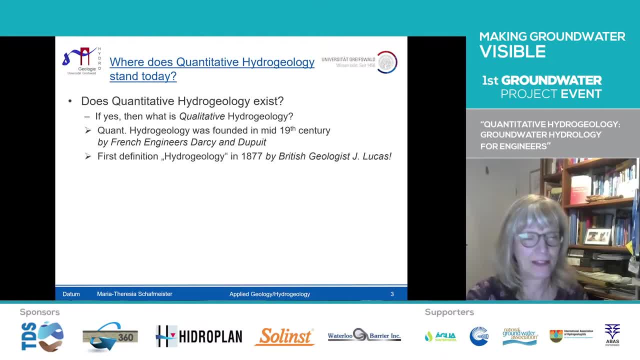 it today was done 20 years later. So my facet is: there is no hydrogeology without quantification. So hydrogeology is quantitative hydrogeology And I think this is something that Ghislain has recognized and has written this wonderful book about it. 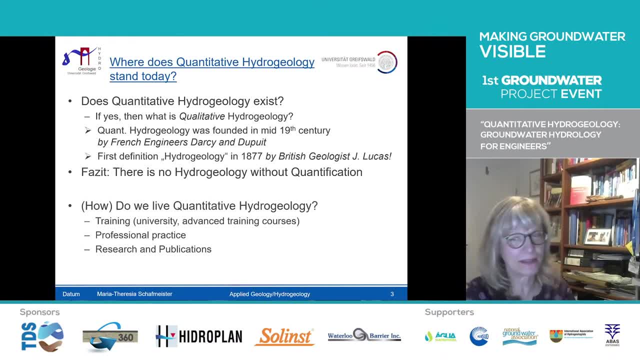 The question is, how do we honor and how do we live quantitative hydrogeology today? And being a professor- Professor at university, of course- I think of train. How do we train quantitative hydrogeology in university courses, or do we do this for advanced training courses? 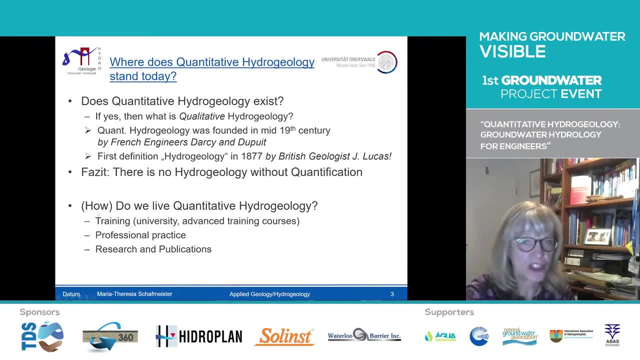 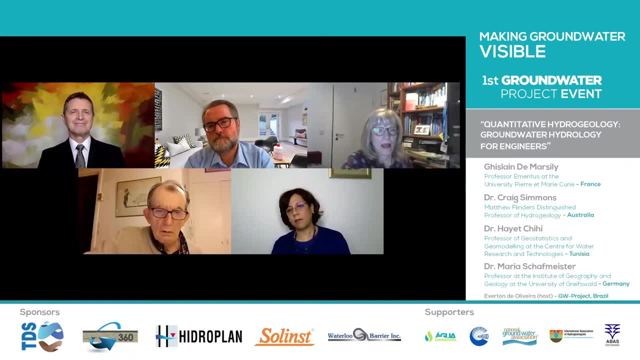 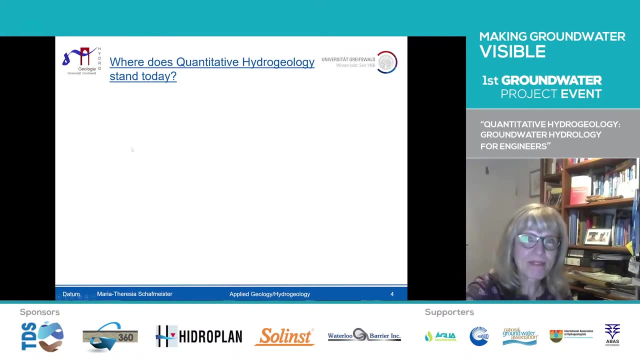 for professionals. Is there quantitative hydrogeology in professional practice? And, of course, what about research and publication? So what I could do within those very few days that I knew that I could participate- tonight or today, as you like. I did a brief review and I looked at German university courses. 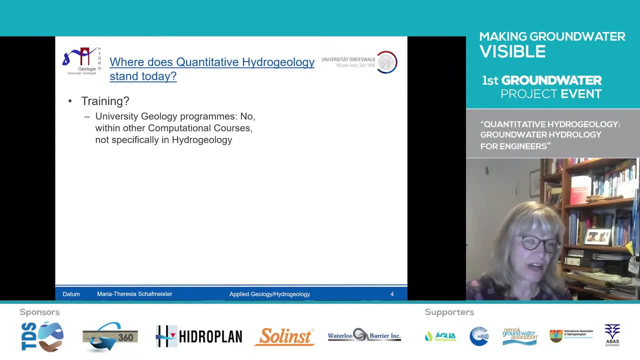 and there are no courses on quantitative hydrogeology, not at least in Germany, except one university offers quantitative hydrogeology And I was excited to learn what is the curriculum And to tell you what it was. the curriculum of quantitative hydrogeology is geochemistry. 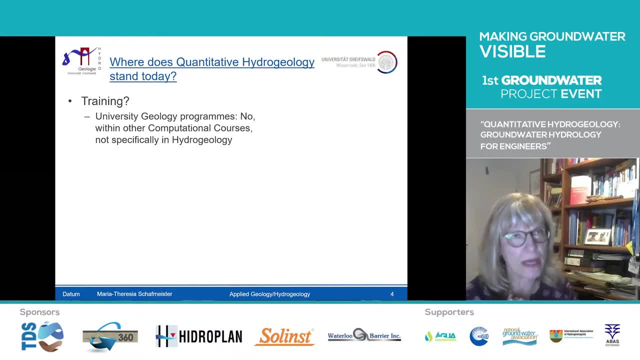 And Tracer hydrology and illegal aspects of groundwater. That is a curriculum of quantitative hydrogeology, And I don't think that this has too much overlapping with what Gillette wrote in his book. So so there is no real courses on hydrogeology. 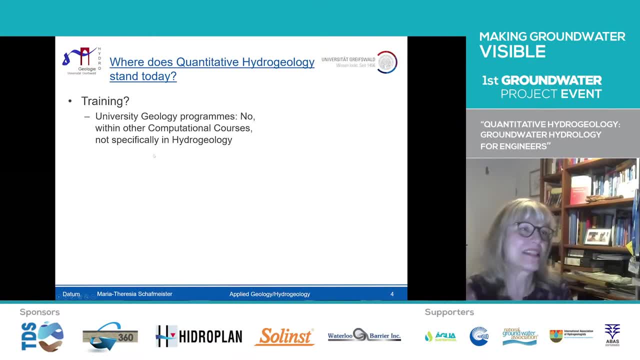 on quantitative hydrogeology, because it is always incorporated in hydrogeology And also we now have courses, other computational courses, where we do learn about mathematical methods in geology and hydrogeology. However, I think still in Germany there are many professionals, hydrogeological professionals. 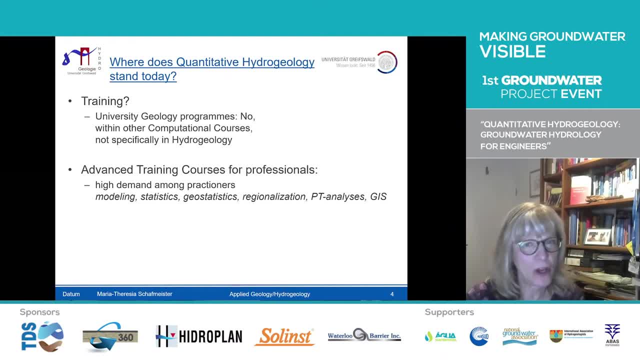 who feel a big gap between what they learned during their geology study and what they need now, And So there is a high demand to learn more about quantitative methods in hydrogeology, And I can give a number for this. The German Hydrogeological Society offers advanced training courses. 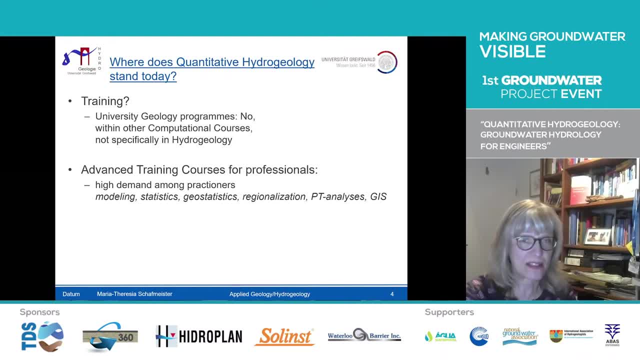 and about 80% of those courses deal with Quantitative hydrogeological methods in the broader sense, so modeling, statistics, geostatistics, GIS, pump test analysis and so on, And so there is a high demand to learn more about quantitative methods. 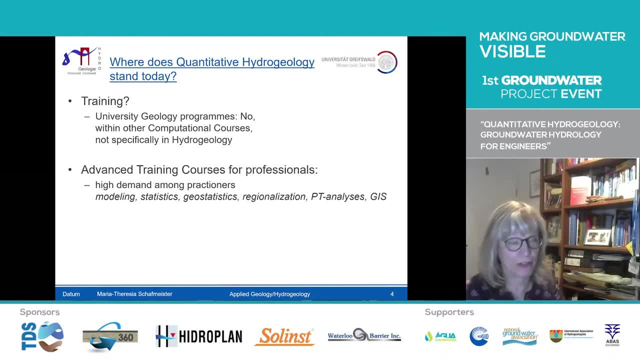 in hydrogeology. And also we now have a number of professors, another group of professors, who are working on collaborative and research at the University of Germany, And I can give a number for this- And of course we have standard city level research. 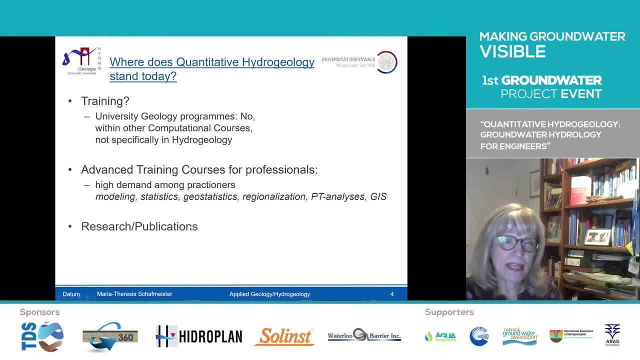 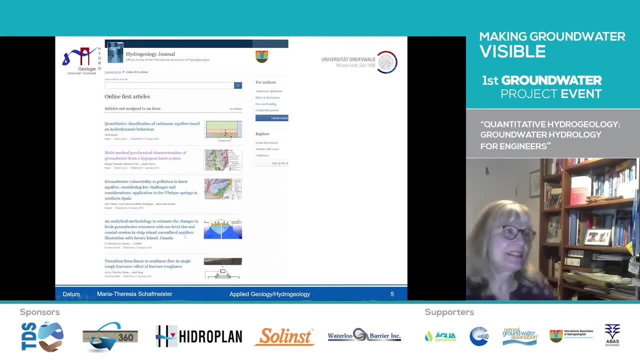 courses and research messages. And, lastly, we have, at a level of high demand to learn that there is much more research and public technical analysis, research analysis, digital analysis and some of the data, specific research and analysis that can be used in hydrogeology. 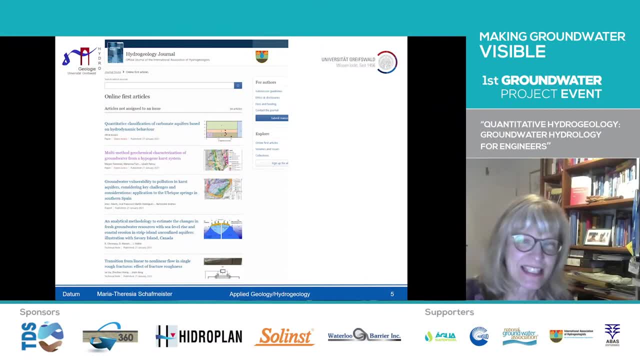 and that can be used to learn more about the status of hydrogeology and the environmental impact of the in-house study and the changes that can take place in hydrogeology. online publications of Hydrogeology Journal. So, since the beginning of the year, there were 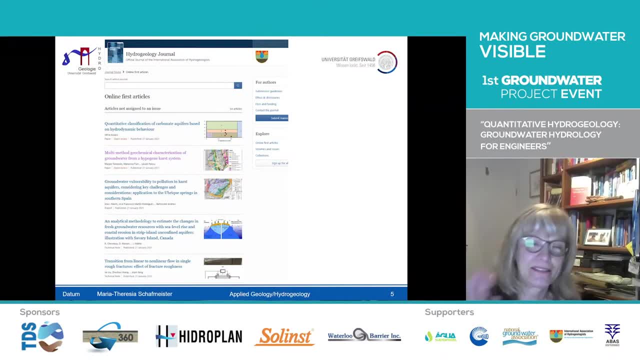 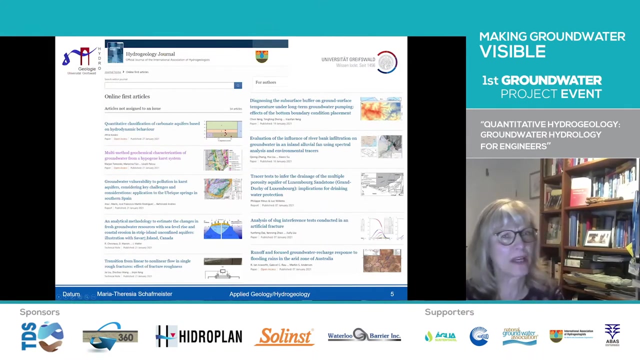 18 papers published and I did a brief glance at those publications and out of those 18 publications, 12 publications were really dealing with quantitative methods or even doing research on quantitative methods. You don't need to read this right now, but it's just to illustrate 12. 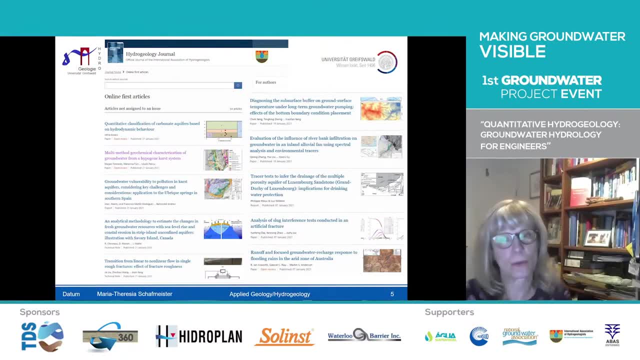 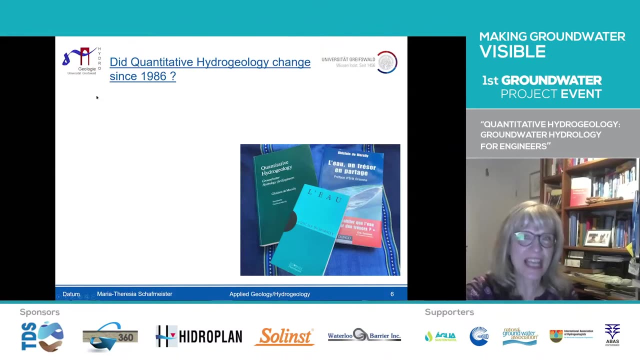 out of 18. that makes two-thirds. So I think this is again a proof that quantitative hydrogeology still lives Well. and then the question is: did it change since 1986, when quantitative hydrogeology was published in English? Here I have a very balanced answer. My answer is yes, and 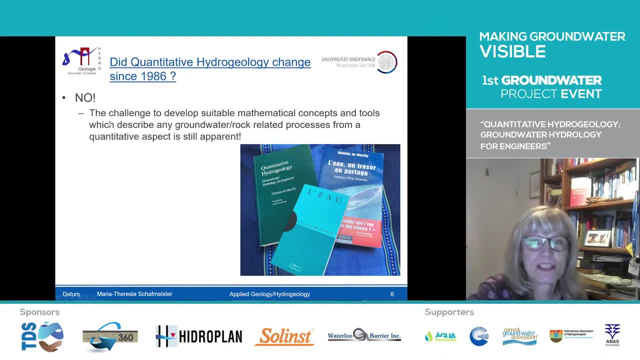 no, Because no, quantitative hydrogeology did not change, because the challenge to develop suitable mathematical concepts and tools which describe any groundwater rock related processes from a quantitative aspect, this challenge is still apparent. So nothing new about this, but yes, since 1986, the 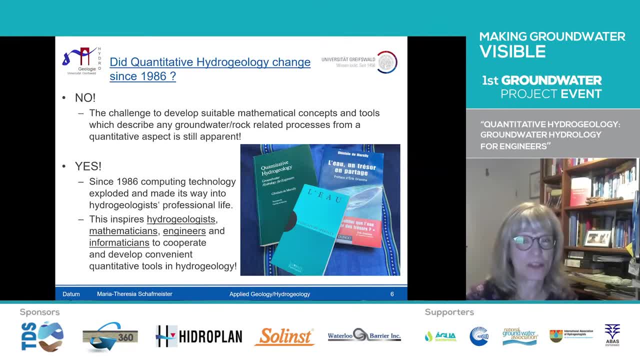 computing technology has exploded and it has made its way to hydrogeologists' professional life, And so this inspires hydrogeologists and mathematicians, engineers, informaticians to cooperate and to further develop convenient quantitative tools in hydrogeology. And we all have to thank Guylain for this, that he did some sort of ignition of this. 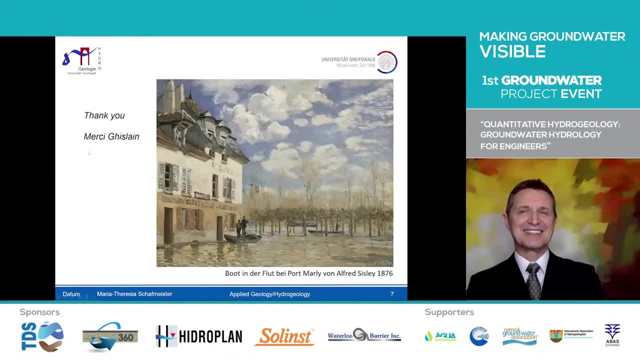 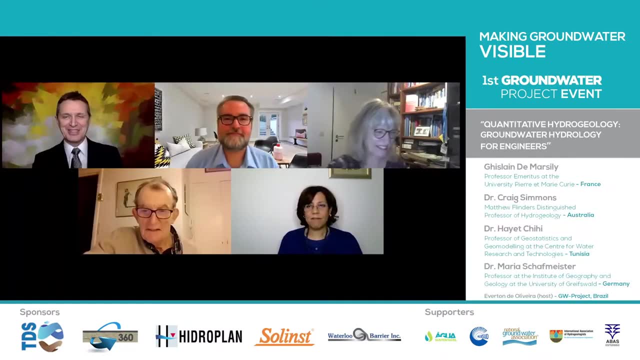 process. So thank you everybody, and merci Guylain, and I think you know this picture. Thank you very much. Thank you very much. Very nice presentation. Thank you for your effort and for your time. Please, Craig, your turn now. 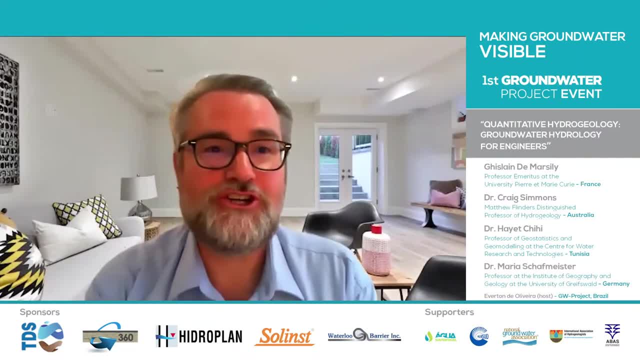 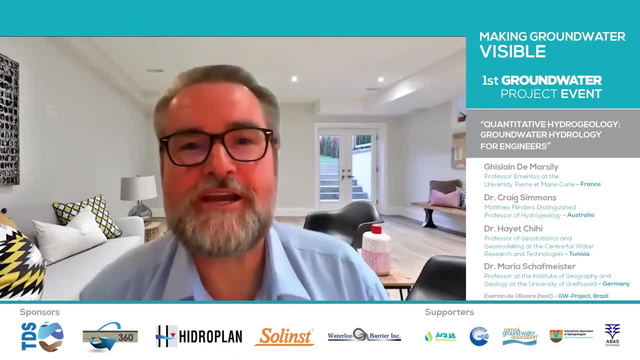 Thank you everyone, and I'm delighted to speak about quantitative hydrogeology and a tiny bit about my own contribution to this field. So, as I said earlier, I'm an engineer and physicist by training And I can't wait to talk to you about the future of hydrogeology. 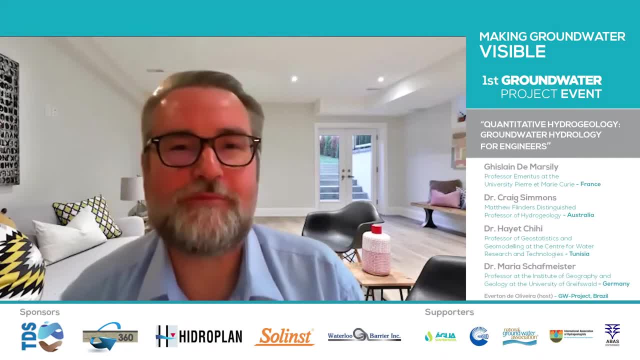 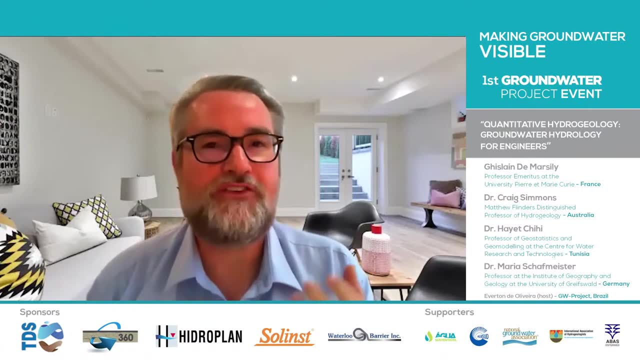 I grew up at CSIRO in Australia in the 1990s doing a PhD in hydrogeology and I was studying groundwater dynamics, variable density flow processes beneath saline disposal basins and salt lakes, running computer models of laboratory experiments that were made using helishore. 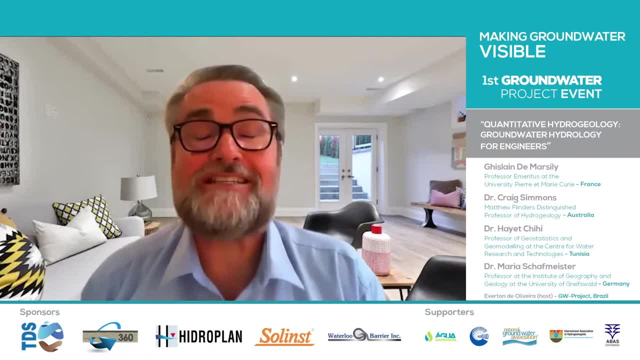 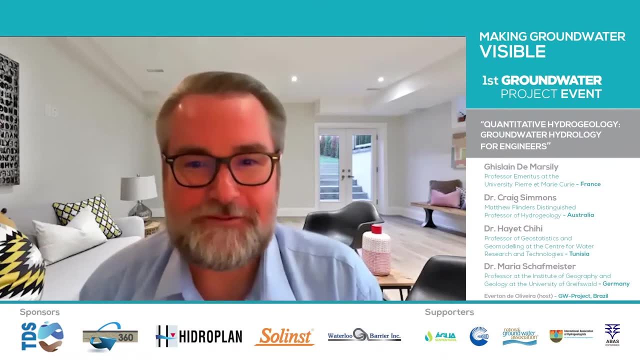 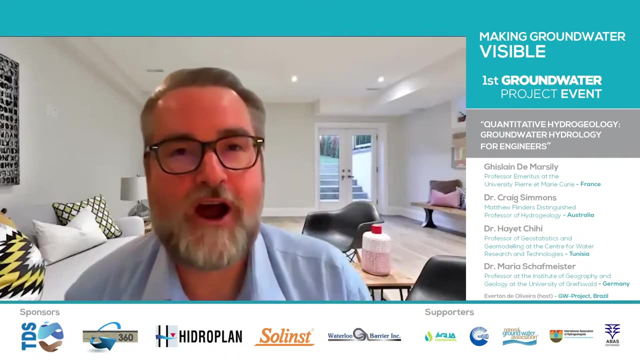 cells. Now. at that time the computer models would take days to run on the very fastest computers and the laboratory experiments took just six hours. And I went on to work in groundwater hydrology and groundwater modelling and I had the good fortune of building and running the National Centre for Groundwater Research and training. 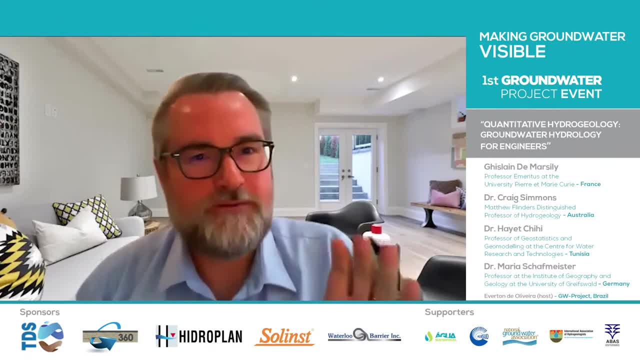 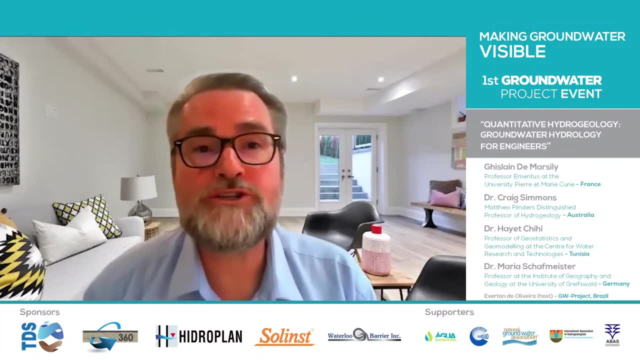 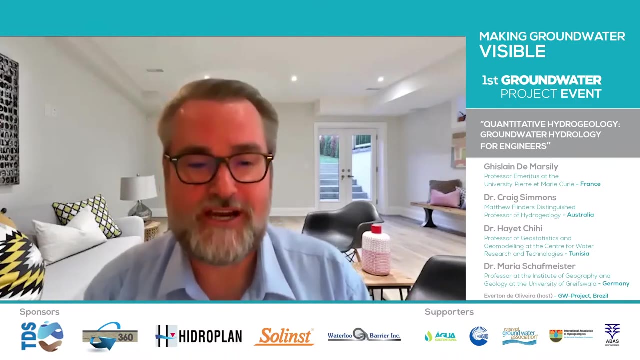 NCGRT in Australia. I thought I'd start with some very basic points about groundwater. just to set the scene. We know that groundwater supplies half of the world's drinking water and about 43% of the water used to grow food. Groundwater depletion and pollution are huge international issues. 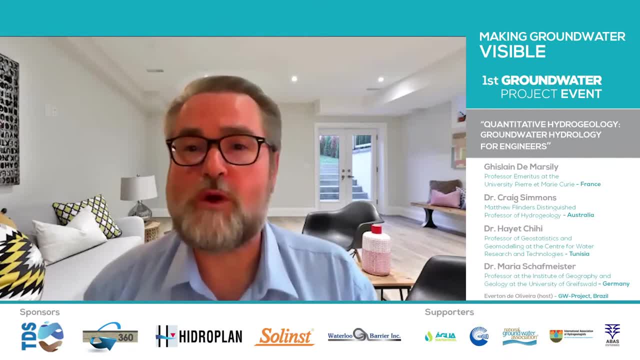 Water is front in major contemporary, pressing issues, whether we're dealing with water security, scarcity and supply, coal, seam gas, shale gas and fracking, food production, mining and energy, nuclear and radioactive waste disposal, groundwater contamination, to name just a few. 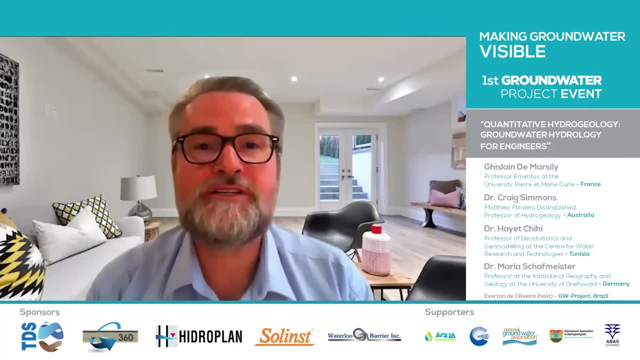 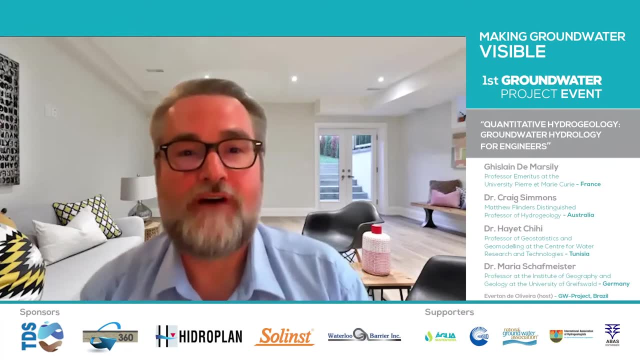 Now, as groundwater hydrologists, we study the occurrence, distribution, movement and quality of groundwater. Quantitative hydrogeology is a key part of understanding, considering and understanding of groundwater. It's a key part of conceptualising and predicting groundwater behaviour. 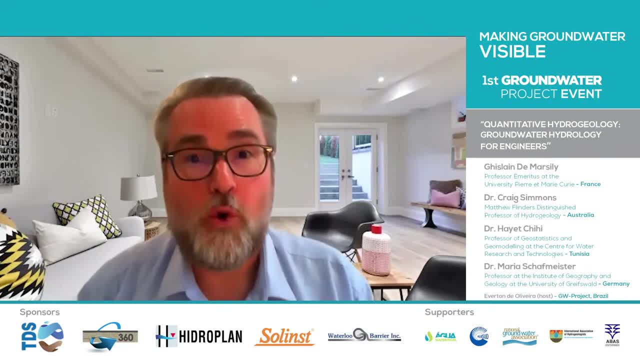 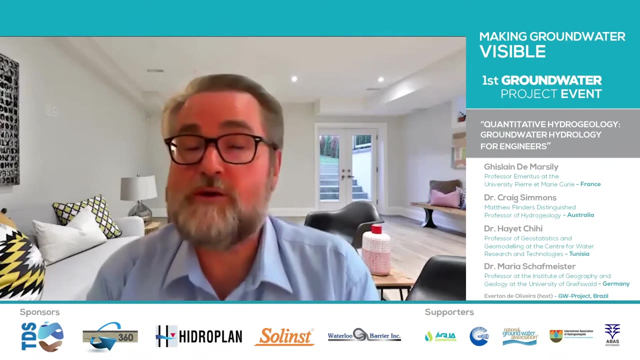 We ask quantitative questions that demand quantitative answers. How much water can we sustainably extract from an aquifer? How fast and in what direction is a contaminant plume moving through the underground geologic maze? Will contamination get into our drinking water supply? 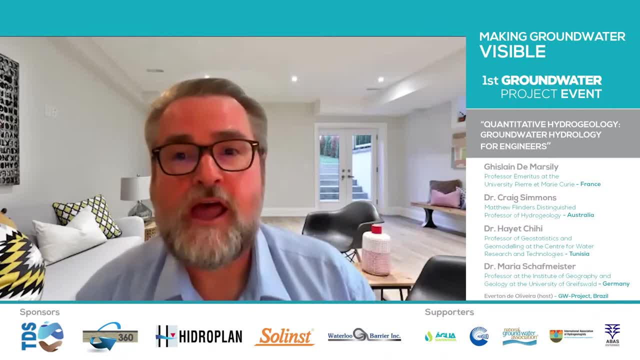 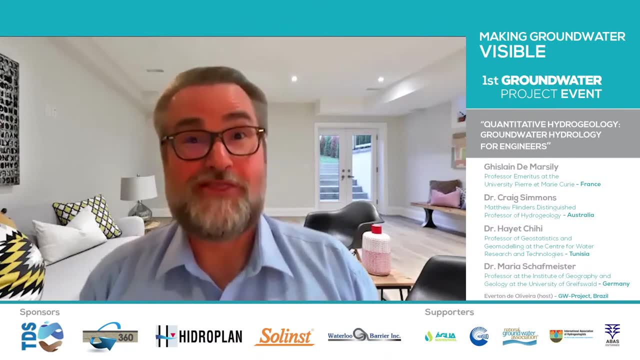 How quickly, By when, At what concentration And how much groundwater is discharging to the rivers, And how fast and in what direction is a contaminant plume moving through the underground geologic maze? Our first digital groundwater models were developed in the 1950s. 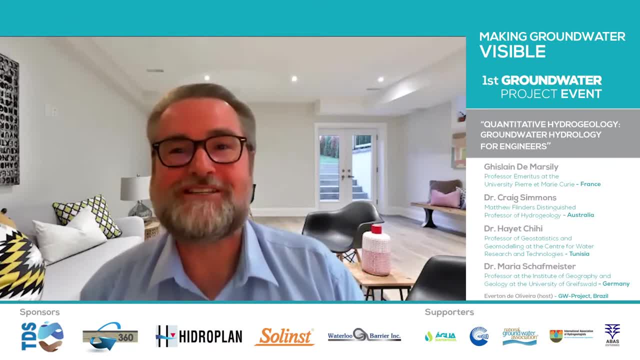 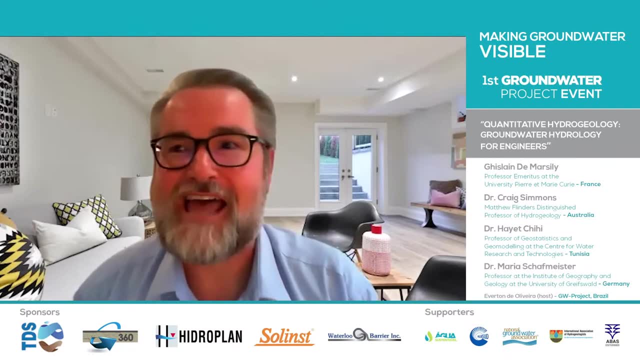 Room-sized electrical analogues for groundwater flow modelling were still in vogue, And I thought it was very interesting that in 1969, one of our pioneering groundwater giants, Alan Fries, author of the groundwater bible Fries and Cherry, had a dream. 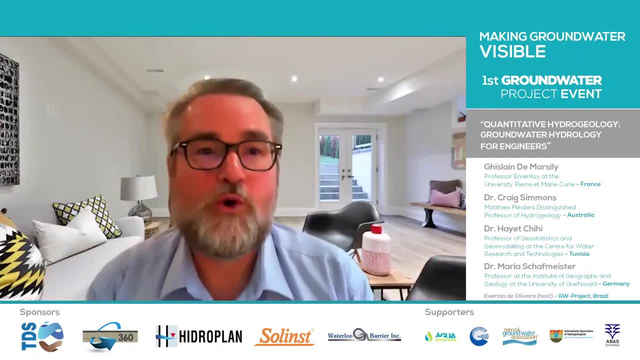 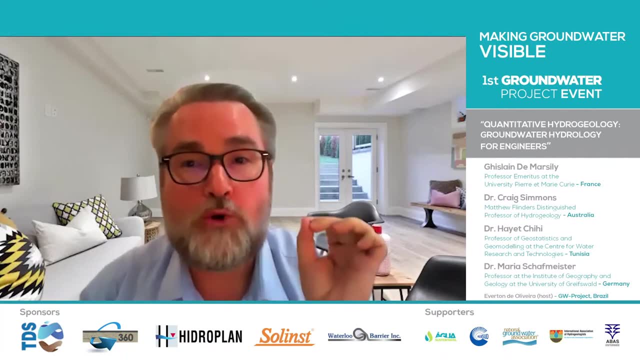 Fries imagined a virtual hydrologic laboratory where all hydrologic processes- rainfall, evaporation, runoff, re-inflation and re-exportation- were all possible. It was a dream, So the idea of water re-inflation could be modeled at large scales. 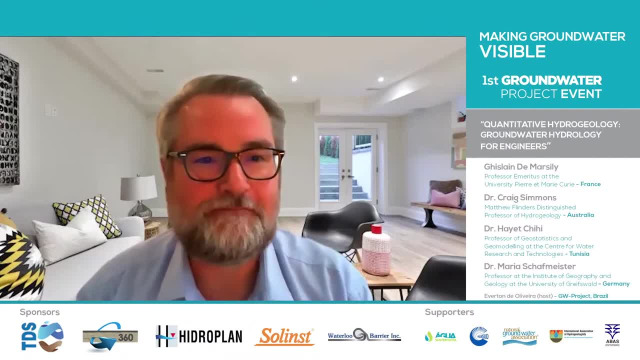 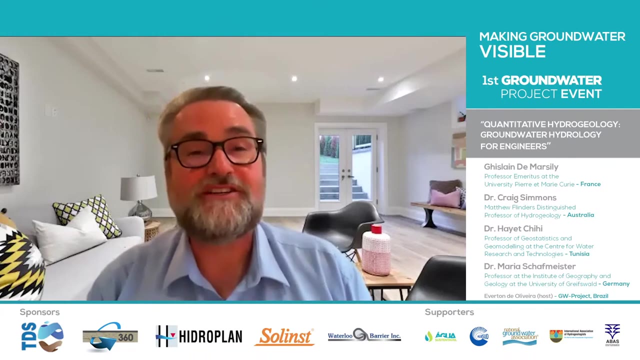 The problem could not be run on the computers of the day. In just a couple of decades, groundwater scientists began to make Fries' dream a reality. The development of integrated surface subsurface hydrological models took off in the 1990s. 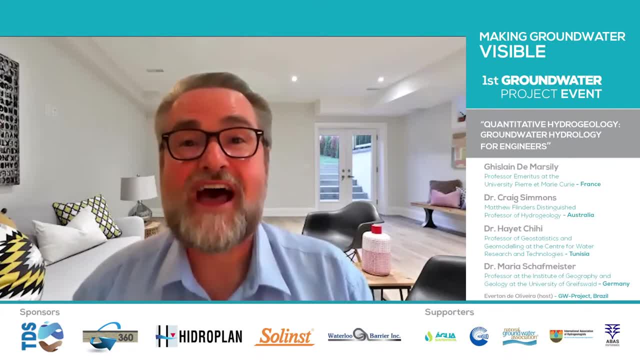 In 2010,, Kollett and co-authors used 16,384 processes to make a Green Earth model. The project responded with a worldwide apple of the eye. During the năm 1920s, Collett and co-authors used 16,384 processes to stretch the水. 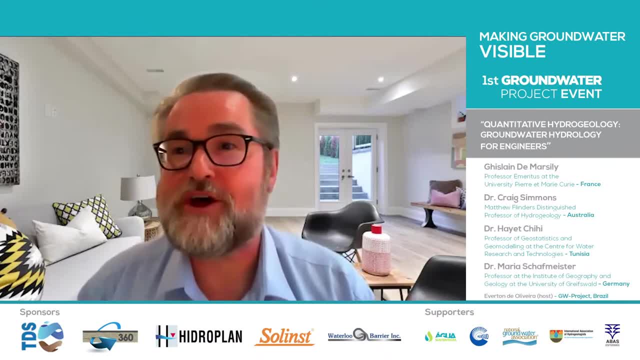 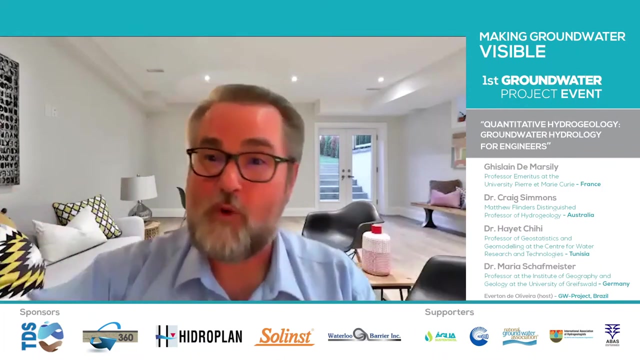 processes with nearly 10 billion grid cells to solve what was essentially the freeze problem. Quite amazing. Their extraordinary study demonstrated that regional scale hydrologic simulations on the order of a thousand square kilometers are feasible at fine hydrologic resolution- about one to ten meters laterally, sorry, and one centimeter to ten centimeters. 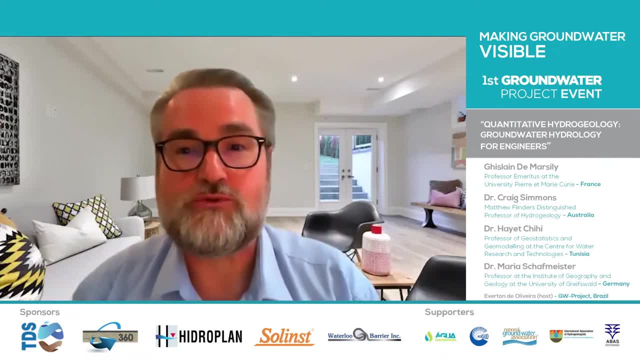 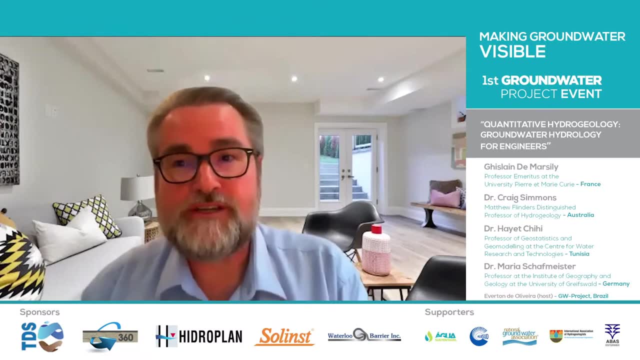 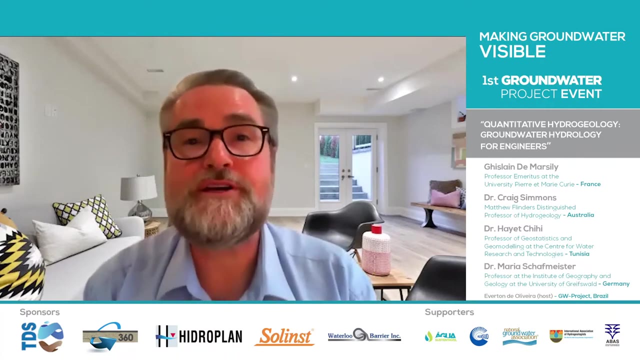 vertically within reasonable computational times. Now we don't stop at running one model. We run models thousands of times and we do this to quantify and inevitably reduce uncertainty in our conceptual models, in model parameters and in model predictions. And we do this to 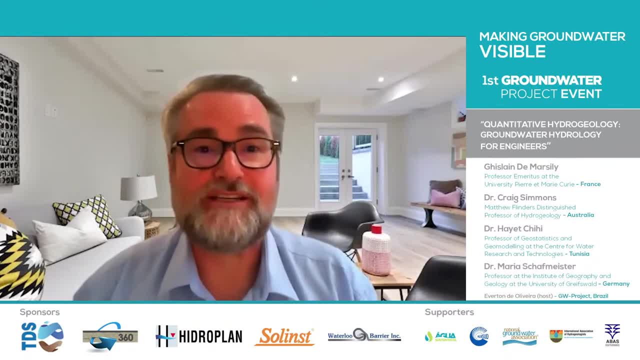 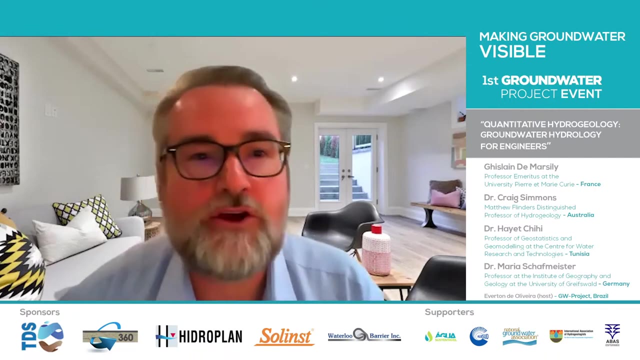 understand data work, what type of data to collect in the field and at what spatial and temporal resolution to best inform our model. So how do we get the best bang for buck? These ideas are inspired by Italian economist Vilfredo Perito's pioneering work: Parameter estimation, uncertainty analysis and data. 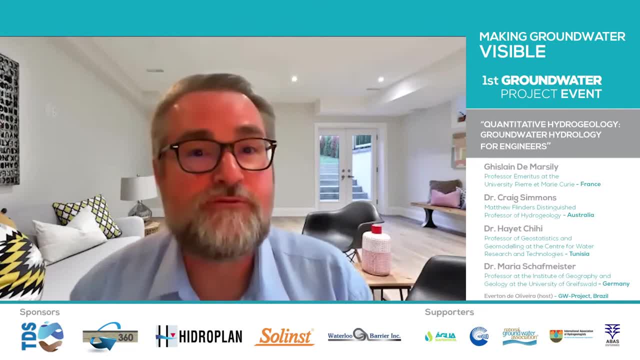 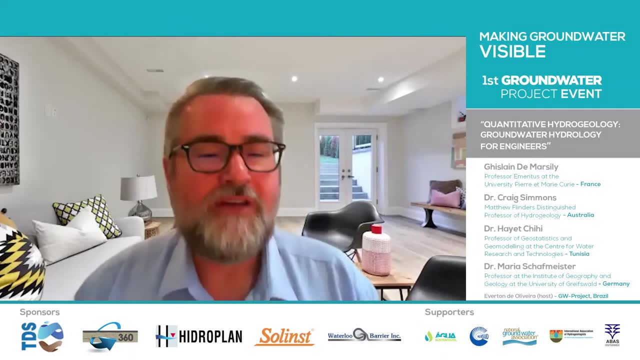 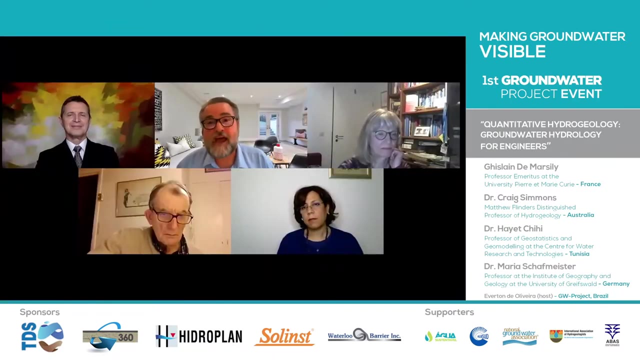 worth studies underpin smart, efficient and effective data collection strategies And they underpin risk-based environmental decision-making. They involve massive amounts of model-generated data. Now in days past, and is often the case today, we're lucky if we have one or two boreholes in a 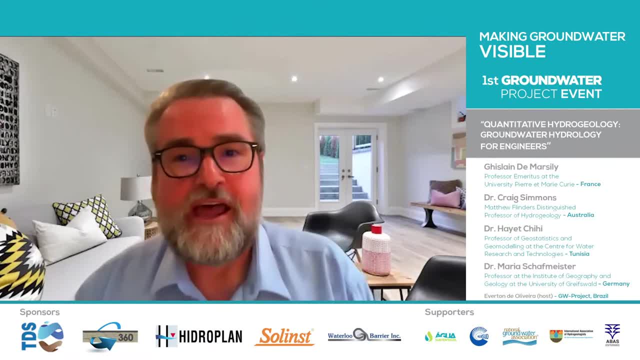 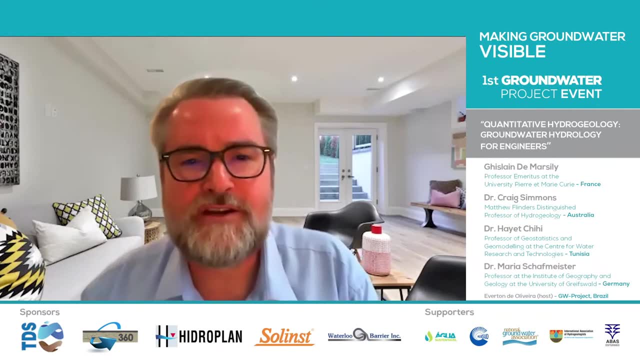 watershed Filled data is expensive: Each bore is roughly $100,000.. Acquiring urgently needed and grossly lacking fundamental data at appropriate spatial and temporal scales to support analyses that are relevant to the critical questions that we are asking in hydrogeology is a challenge, and 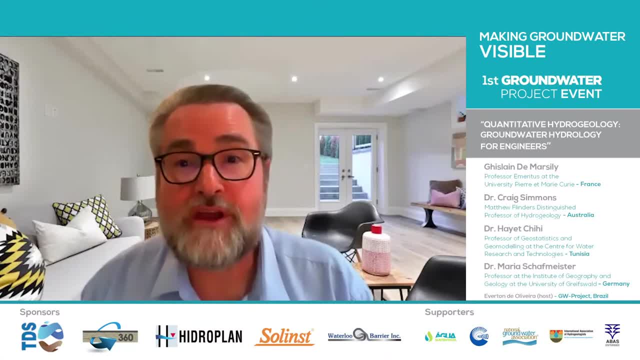 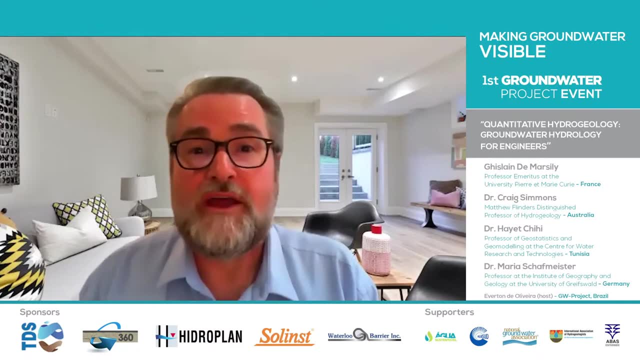 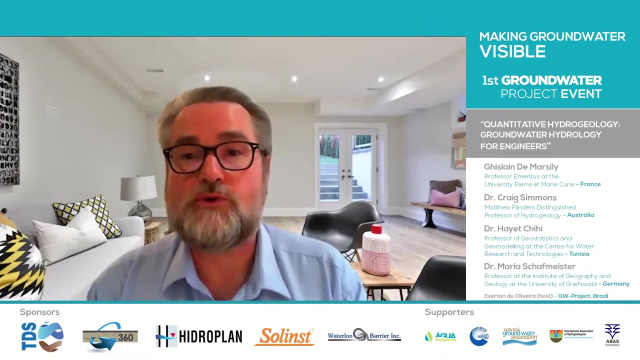 an opportunity, But more and more data are becoming available for use in groundwater modeling. New and extraordinary data sets have been collected. Satellites now exist, For example the gravity recovery and climate experiment, tracking, underground water storage and rich GIS data sets for vegetation and soil types. 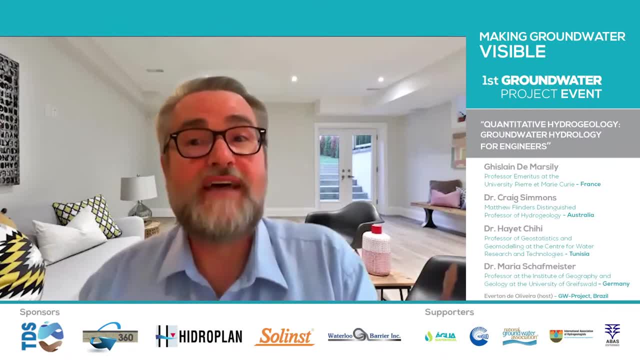 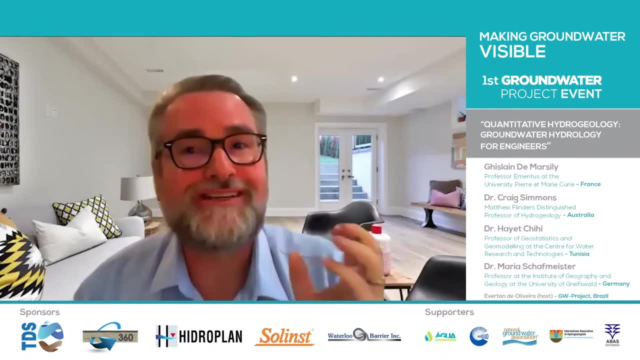 that have millions of data points in a layer. Big data is increasingly publicly available and provides exciting opportunities, So if you're interested in learning more about this, please go to our설vesorg. solutions and ideas that are simply waiting to be found. 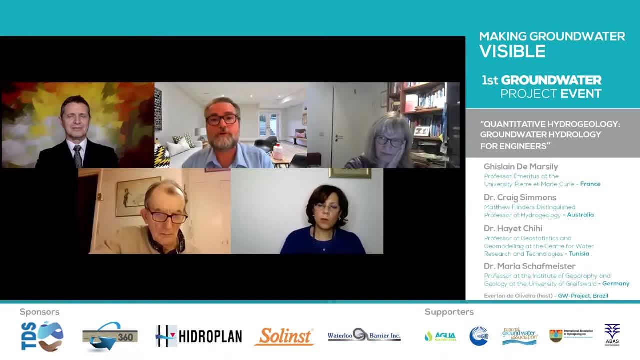 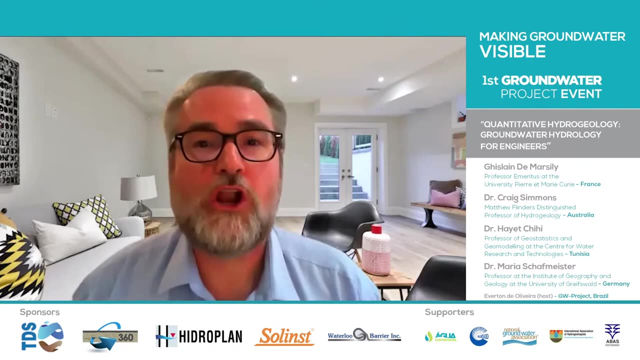 Addressing the continuing and pressing need to develop mature and robust groundwater models to predict groundwater processes that are underpinned by strong geologic and hydrogeologic conceptual models and comprehensive data remains a challenge Now. quantitative hydrogeology is not just about data or just about modeling. It is necessarily 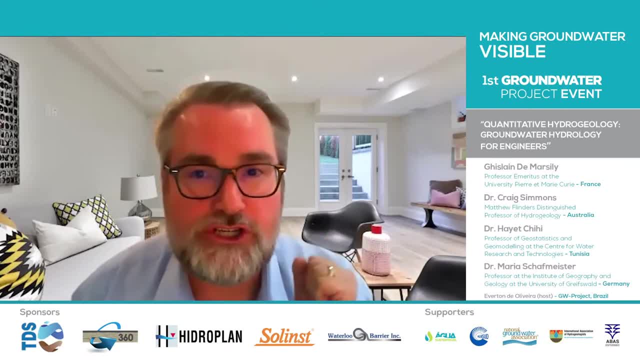 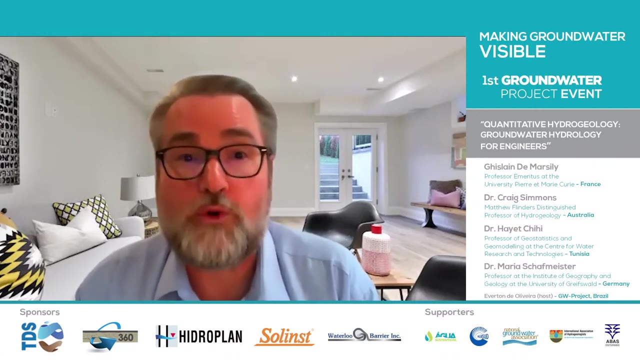 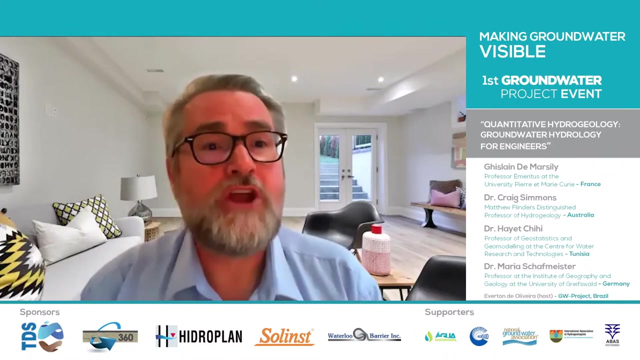 about both The nature. spatial and temporal resolution of the data we require will depend on the specific questions that we are asking, their representative spatial and temporal scale and the intrinsic physics. Data assimilation is a growing challenge and opportunity for groundwater science. Different data types, for example environmental traces that Maria mentioned just a moment ago, can help reduce model non-uniqueness. 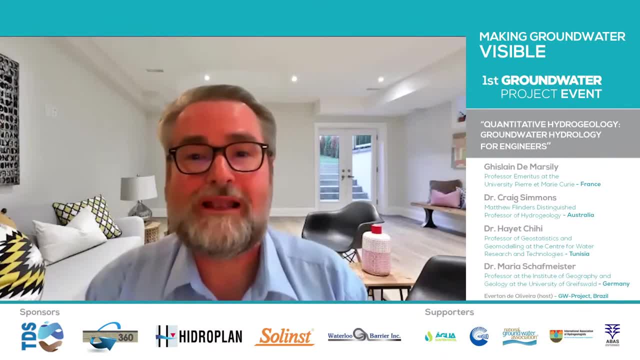 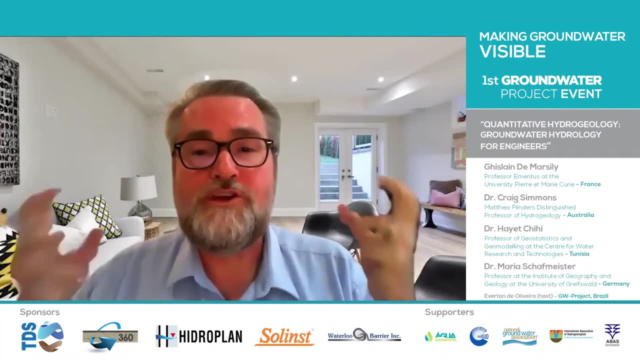 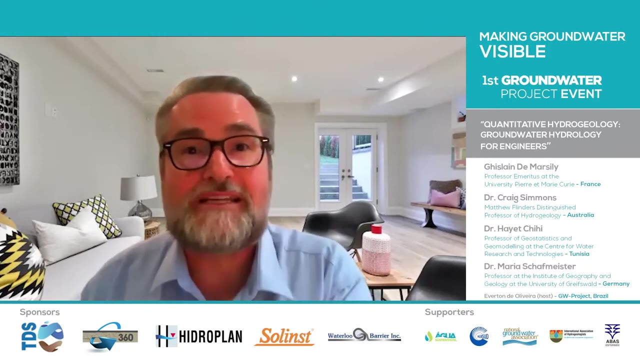 Now, quantitative hydrogeology will clearly need more than an abacus and it will need to pay attention to the often problematic what I call theory to measurement ratio in groundwater analyses. finding the sweet spot, the appropriate level of simplicity, complexity for modeling and requisite data to answer a specific question at appropriate scales- remains a challenge. 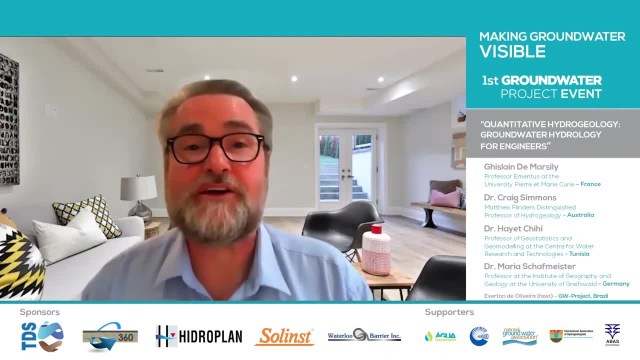 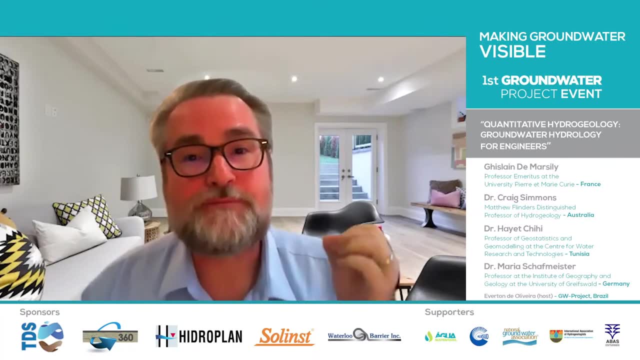 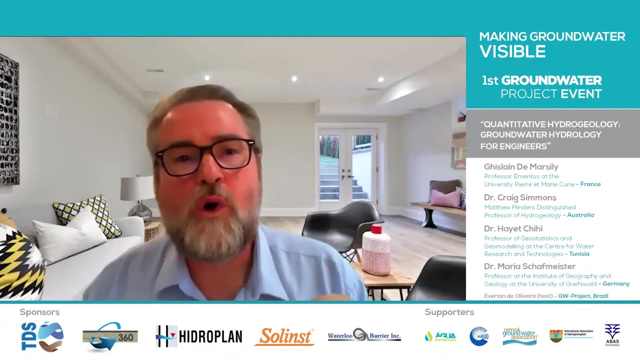 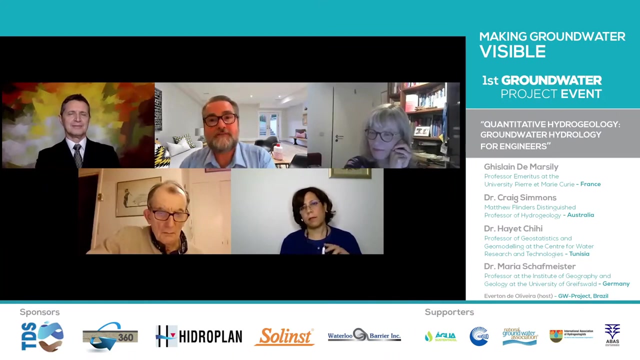 Occam's razor and Einstein's advice that everything should be made as simple as possible, but never simpler, are guiding philosophies. They must be implemented, quantified and assessed mathematically. And, crucially, there are always unknown complicating factors which cause the actual behavior of a groundwater system to deviate from prediction or expectation. 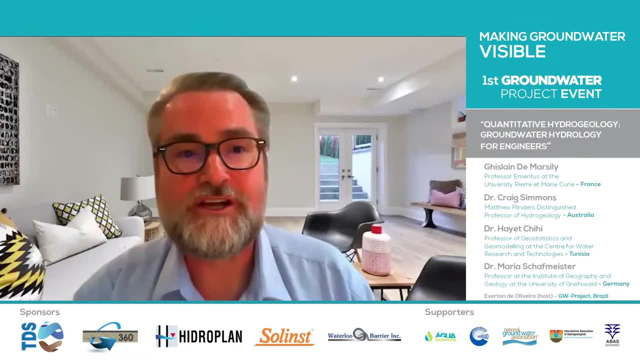 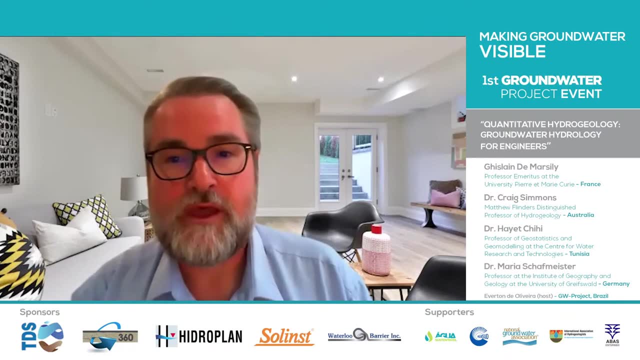 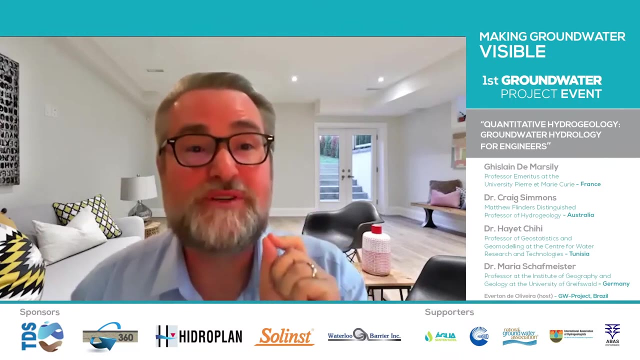 And this includes conceptual model surprise, as John Bredehoft puts it, surprise being, I quote, the data that renders the prevailing conceptual model invalid And based on empirical data. Bredehoft, 2005, estimated that surprise occurs in some 20 to 30% of model analyses. 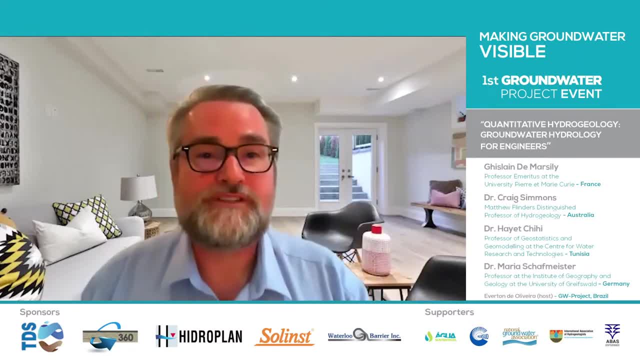 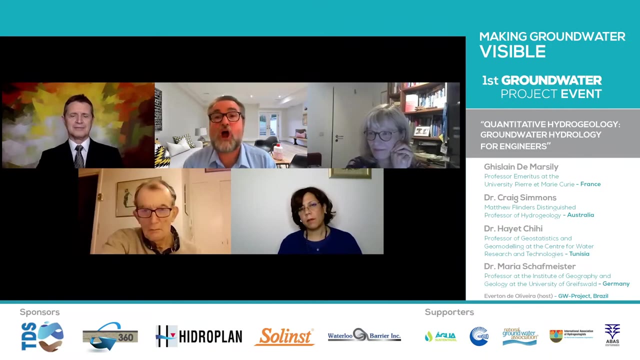 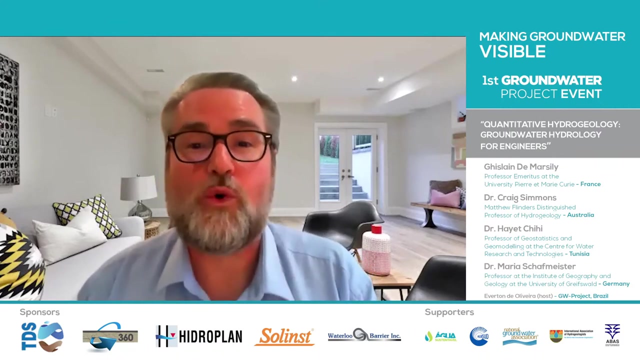 Geologic heterogeneity may be one root cause for surprise. Dealing with geologic heterogeneity continues to pose a major challenge in understanding how groundwater systems behave. The Earth's maize has properties that vary by over 12 orders of magnitude. Now the difference between walking and the speed of light is eight orders of magnitude. 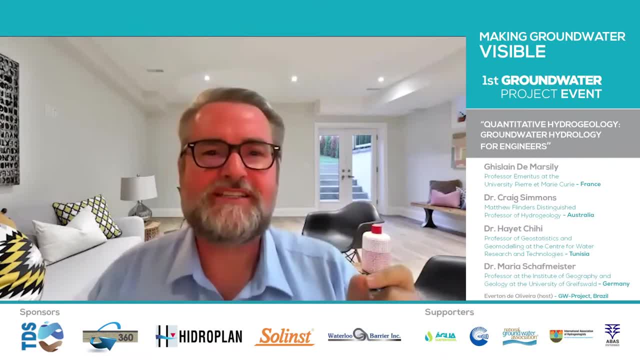 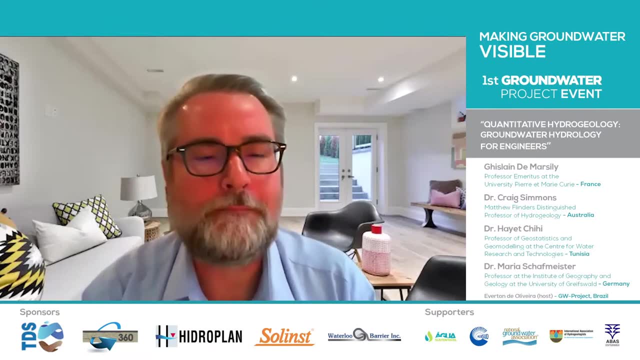 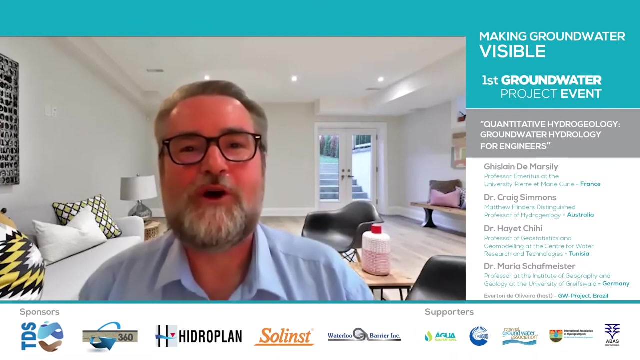 And someone once said to me: we put man on the moon in 1969, and hydrogeologists are still saying that they cannot predict the fate of a contaminant plume. Now, after scratching my head for a little while, I responded that if the pathway between the Earth and the moon was anywhere near as complex and as heterogeneous as that which we encounter in aquifers, that we would not have got to the moon either. 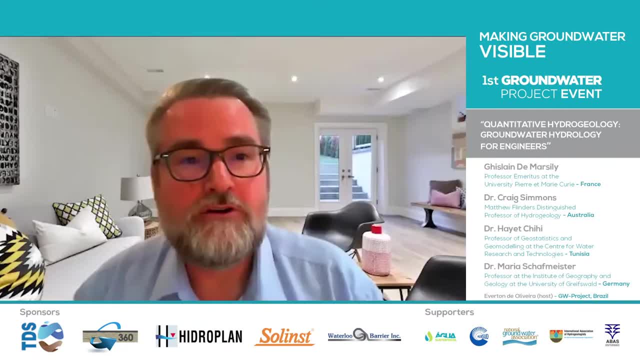 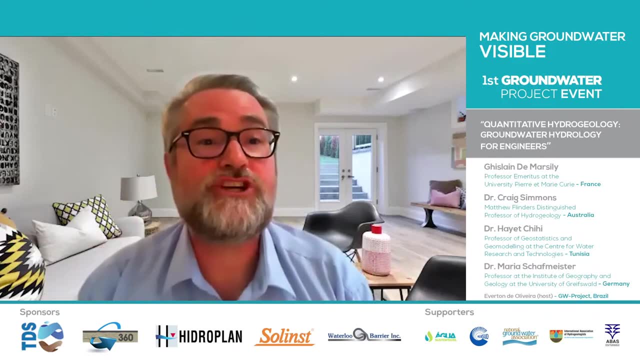 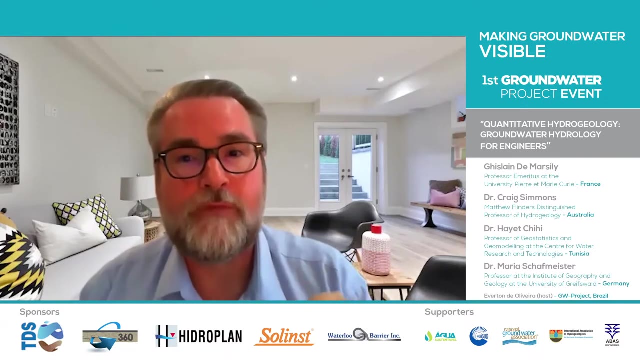 Putting geology back into hydrogeology remains a challenge, but we will never know where every fracture or every fault is, nor every detail of heterogeneity at every scale. Understanding the crucial features of our conceptual model is key. What is material and when does it matter? 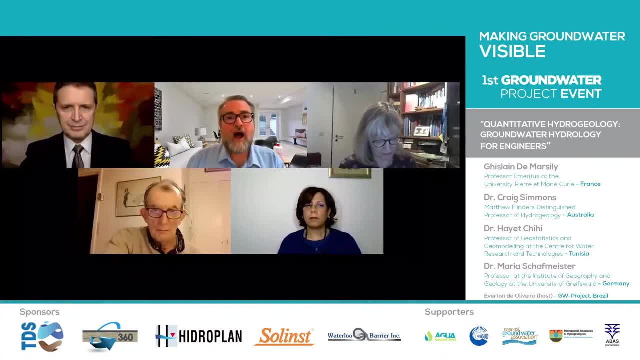 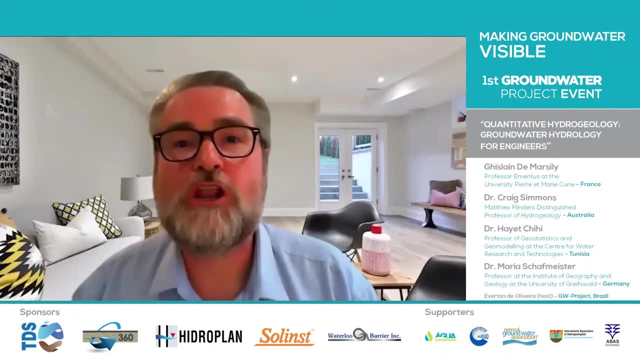 Is our analysis fit for purpose? In their article Dealing with Spatial Heterogeneity in Hydrogeology's Special Theme Issue, The Future of Hydrogeology, Demarceli et al, 2005, make the point, and I quote: 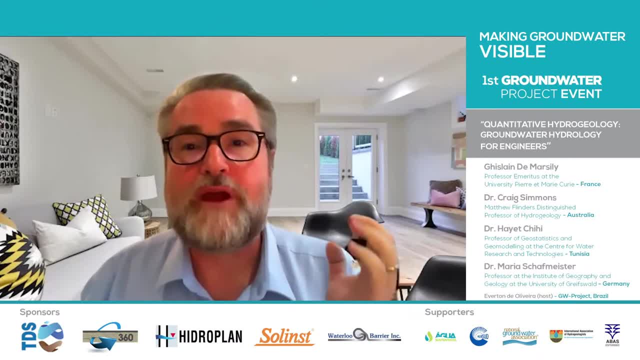 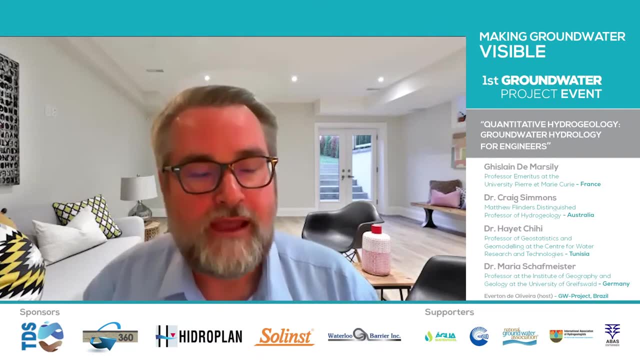 Until the large-scale permeability of an aquifer can be reconstructed from small-scale methods, there will be a credibility problem for our discipline. Ilan Demarceli, following George Matheron's seminal contribution, made some fundamental developments in geostatistics. 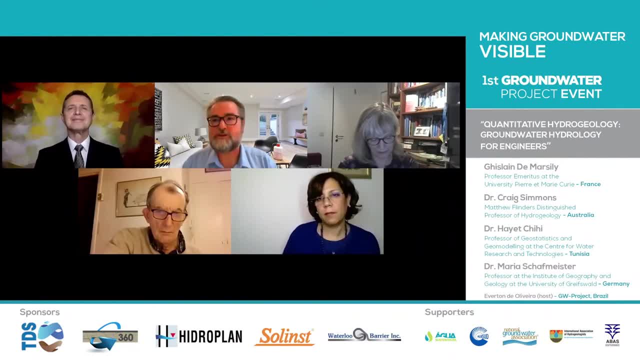 Both with Jean-Pierre Delhomme, were highly influential in bringing geostatistics to the groundwater world, exemplified in Demarceli's seminal textbook book Quantitative Hydrogeology, itself an important tool in the study of heterogeneity. 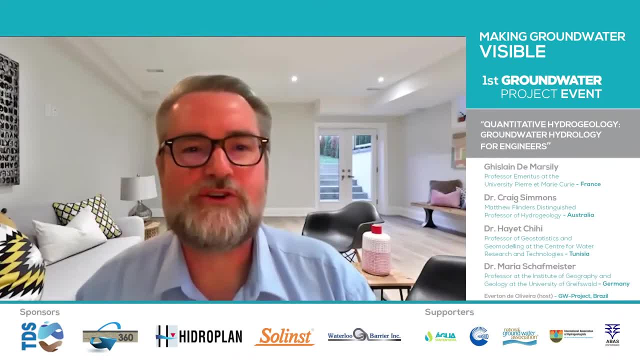 So we must use every tool in our hydrogeologist's toolbox. As American psychologist Abraham Maslow said, and I quote, If you only have a hammer, you tend to see every problem as a nail. And there are many examples of new advances in parameter estimation methods, uncertainty analysis, geostatistics optimization, environmental traces for characterizing groundwater. 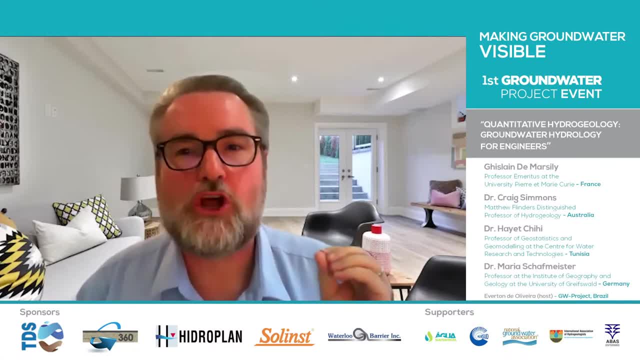 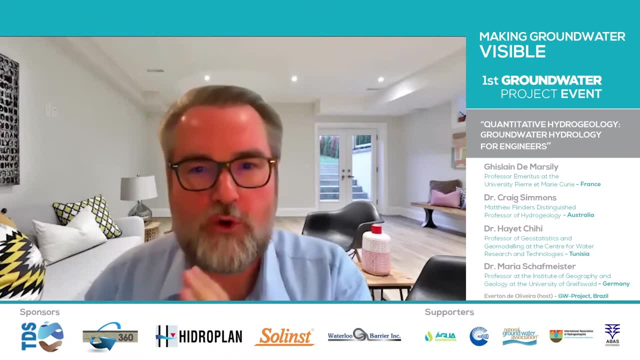 and linking geologic information with hydrogeologic models that have not found their way into everyday practice, And this builds on and touches on a point that Maria made a little while ago. So, as we look to the future, linking and integrating groundwater with soils, surface water, ecosystems and climate science are exciting challenges. 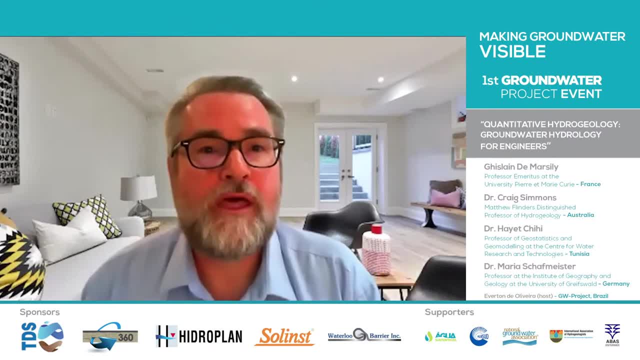 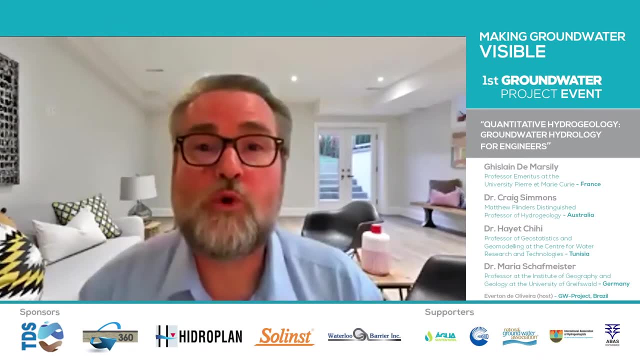 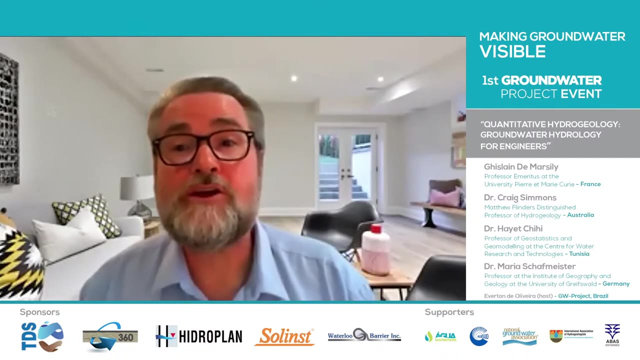 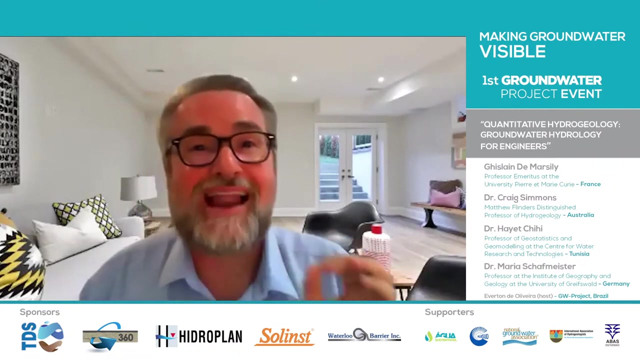 And there will be others that are currently unknown. Contemporary groundwater problems have moved well beyond classical hydrogeology, concerned as it was with how much water was stored in or could be extracted from an aquifer. Quantitative hydrogeology, including 21st century groundwater modeling, uncertainty analyses and the manipulation, processing, analysis and storage of gargantuan amounts of field-based and model data, will be necessary to advance and solve many of these problems. 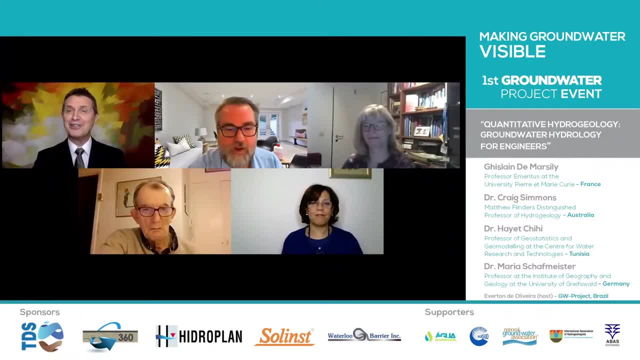 Thank you. Thank you very much, Craig. Thank you all for a nice presentation. I would like to start our session here asking one personal question to Guylain. You mentioned quite impressively for me that a professor turned you out from his geology course because you know an amazing reason, right? 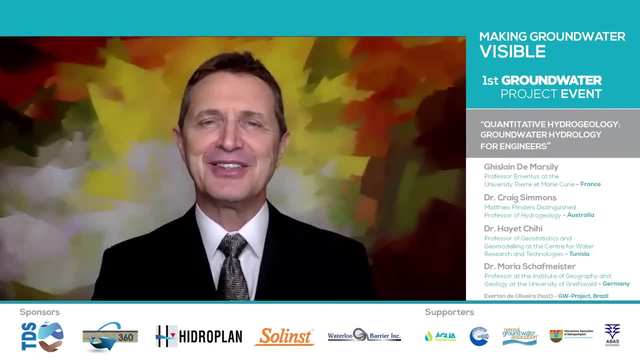 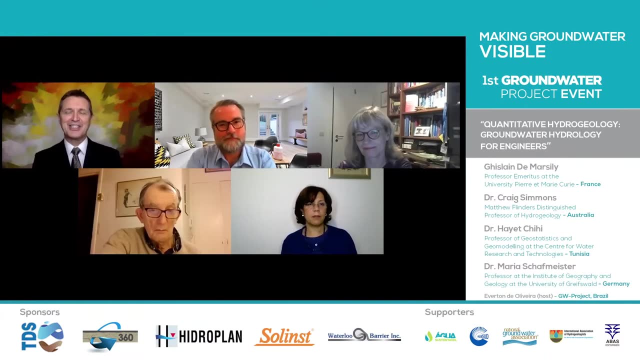 And even though you You became a very good hydrogeologist regardless of that, you know, silly decision, I would say: Well, that for me strikes in a position, because you wrote your book, You were not that old. 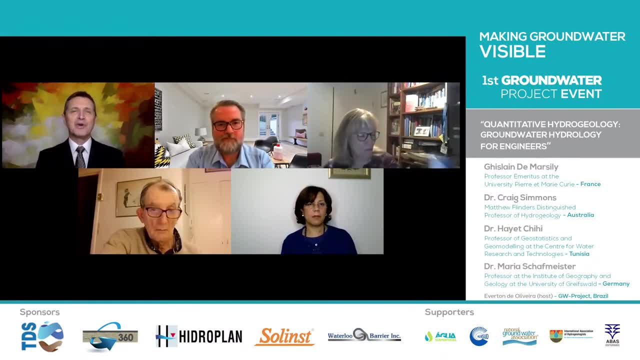 You were young when you wrote Quantitative Hydrogeology. What makes someone become so confident to write a book when you're young and put it to people? And did you have any idea about what the book would become? Because you wrote other books in other subjects. 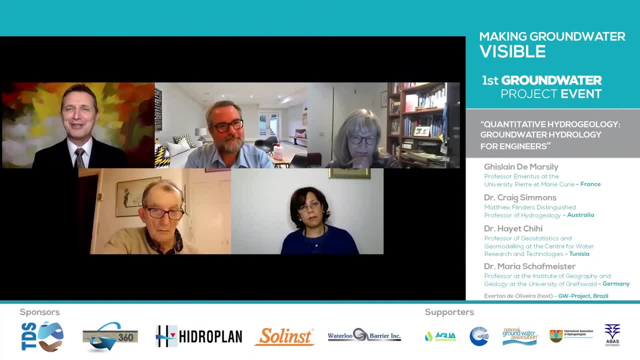 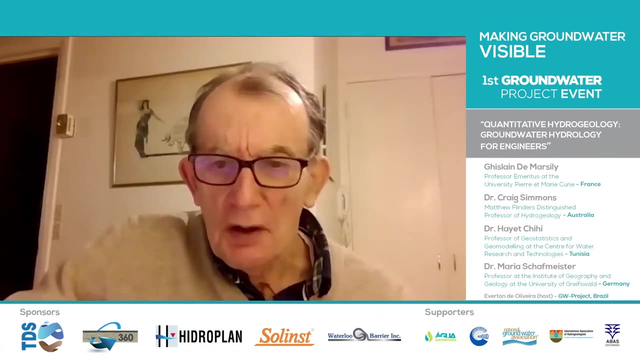 Where does the confidence come from, Please? It's a tough question. I was about 40 when I published the first version of the book in French And, as I said, my motivation was to give something to the students I was going to teach. 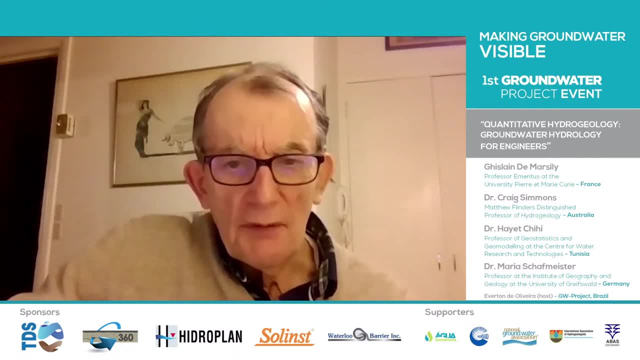 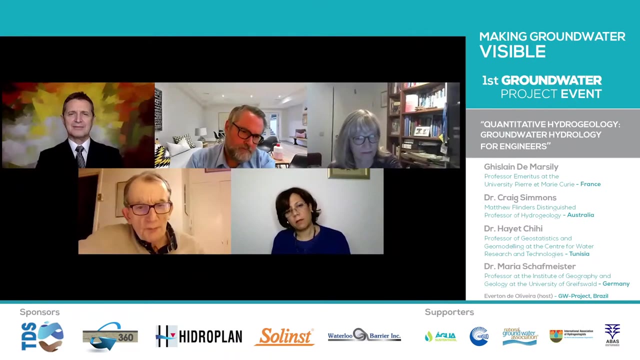 So I wanted them to have written material that they could look at if they didn't understand what I said orally in class. So my real motivation is to help students understand and learn and integrate what the course was. First of all, when I wrote this book, many colleagues came to me and said: 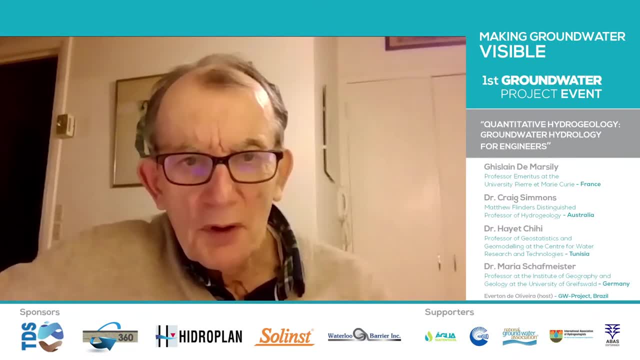 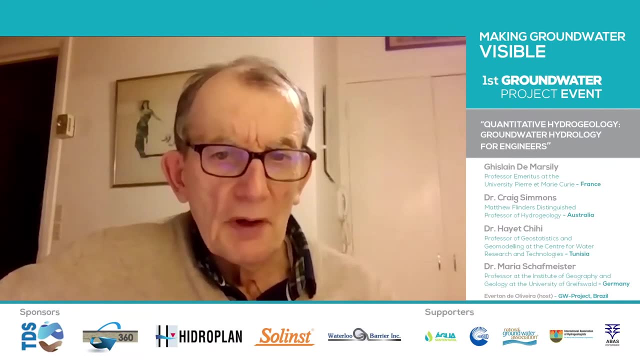 You're stupid. Why would you waste your time writing a book? You should write articles. Articles are much more important for your career than books. And forget about the book and go on and write good articles in good journals, And that was not my philosophy. 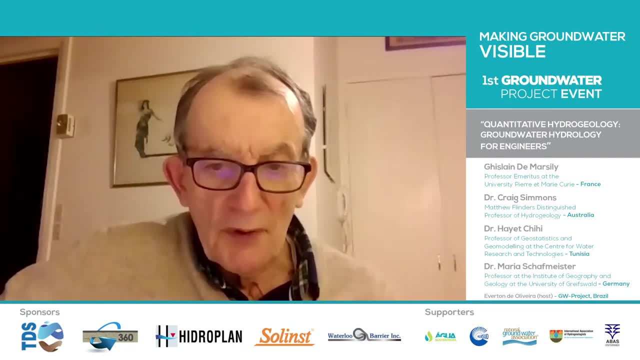 I didn't want to work. I did publish papers, of course, as everybody does, But my main motivation was to teach and help students. So this is why I wrote that book, And I think that if this book has some success, it's due to that. 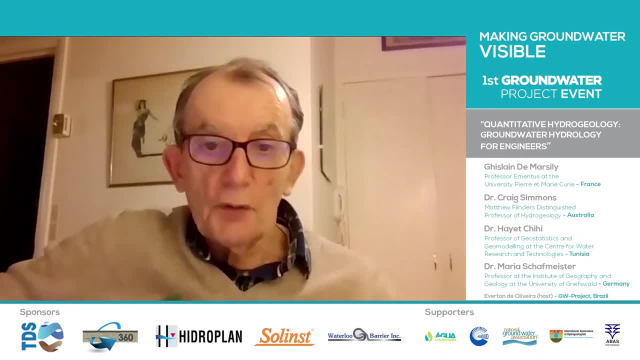 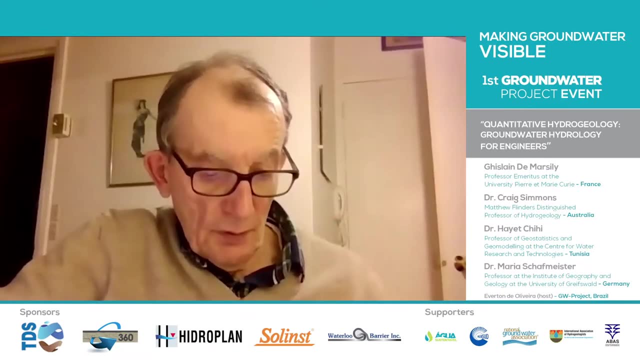 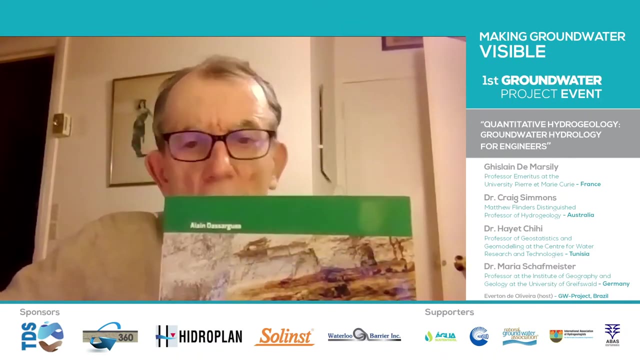 I'd just like to show you this new book, which has been written by a Belgian colleague whose name is Alain Dassarg. Alain Dassarg has written this book Applied Hydrogeology, which was just published this year and the year before, both in French and English. 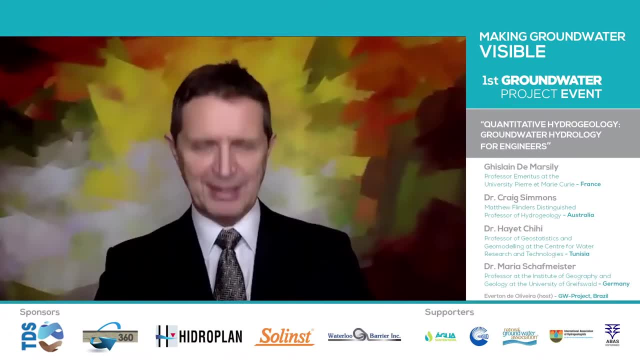 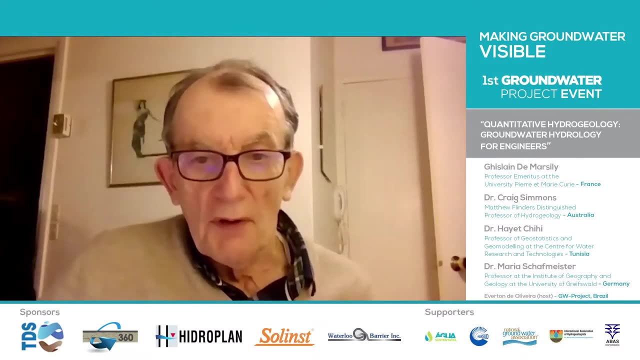 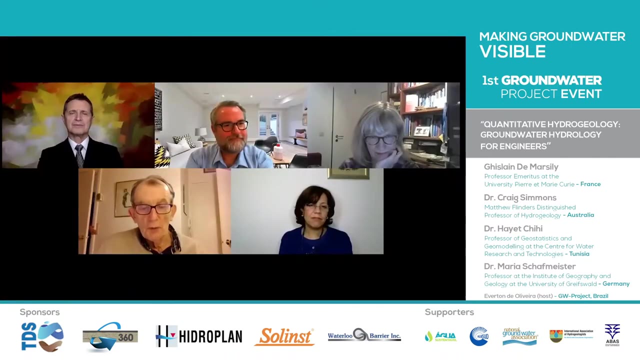 I think it's. many of the chapters of that book are based on my old Quantitative Hydrogeology, But I'm very proud that you know, a new book written by somebody else and improved and with new topics and new so on, was published recently. 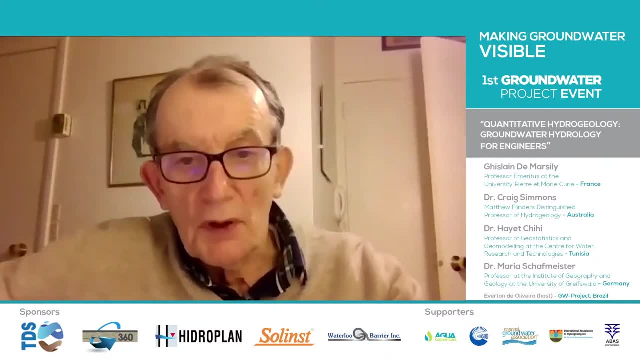 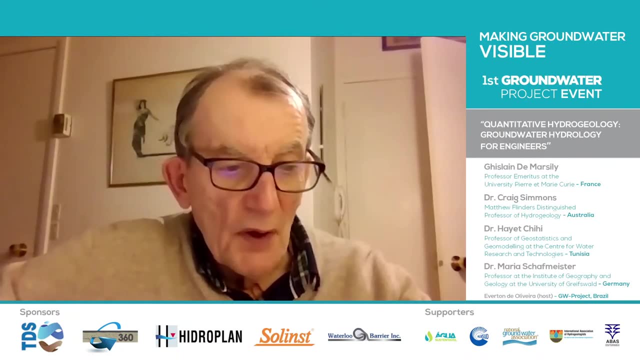 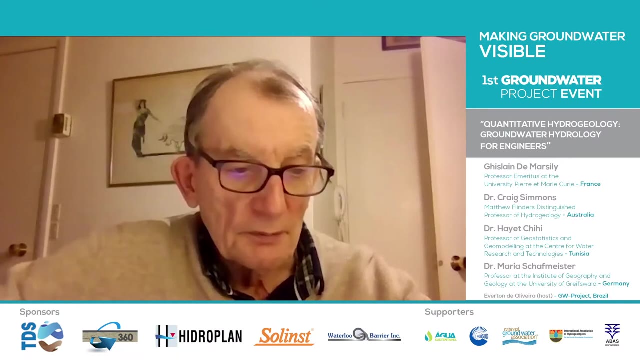 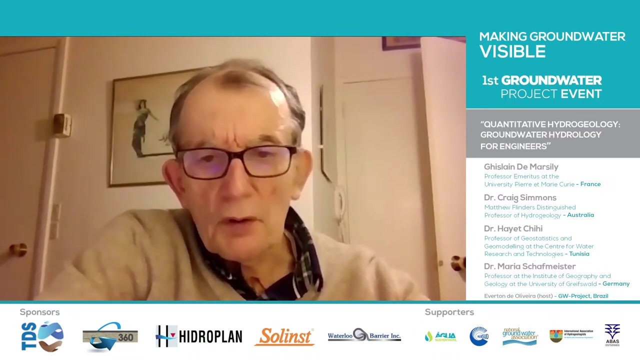 Continuing the work I started with writing books. If I may, I'd like to add one idea which may be crazy but which came to my mind when listening to the other speakers. You're all familiar that in other disciplines like, for instance, meteorology, atmosphere, climate and so on, 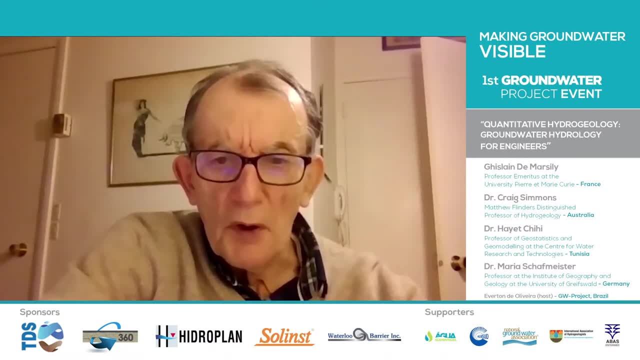 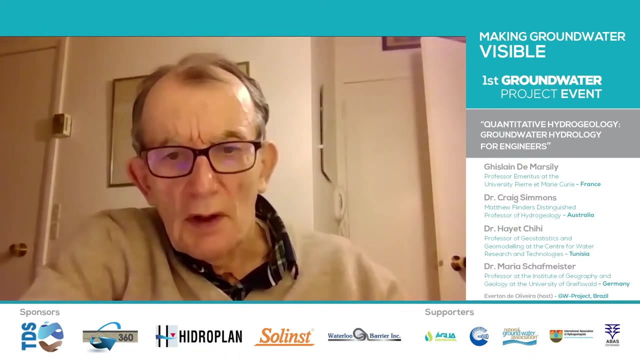 They are slowly turning away from modeling in the usual sense of solving flow equations And using what's called artificial intelligence. In other words, they collect data because it's easier to collect data on weather and clouds and sun and temperatures and wind velocity. You can have huge databases. 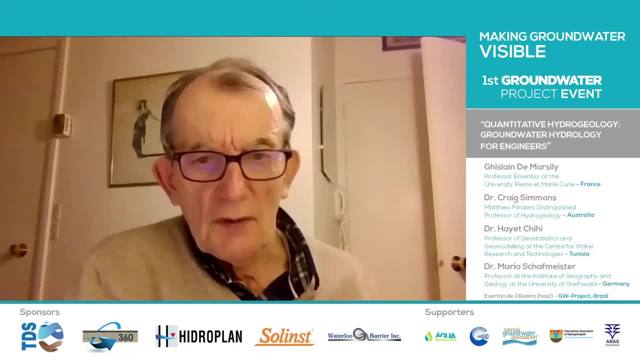 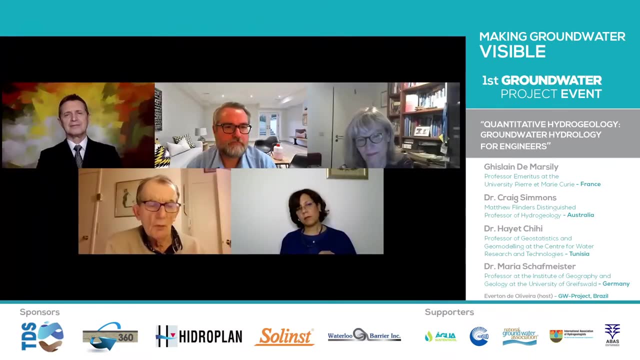 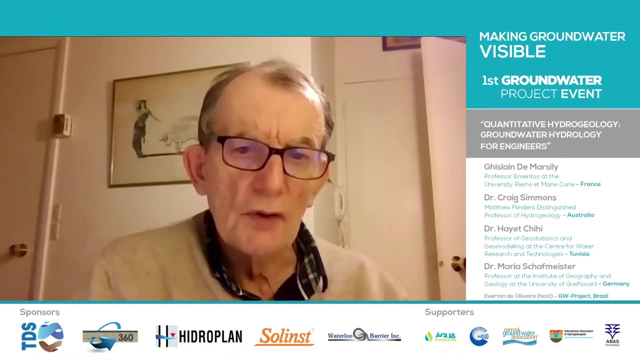 And what they say is that if you have these huge databases and you have a situation here today, If you look at what happened maybe a hundred or no tens of years before, If you find the same situation, then you can predict what's going to happen here today based on what happened 10, 20 years ago for a similar situation. 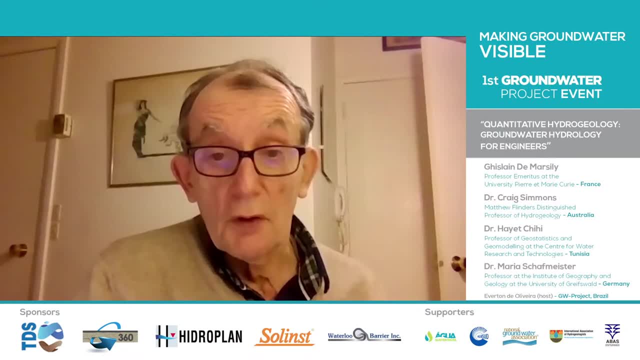 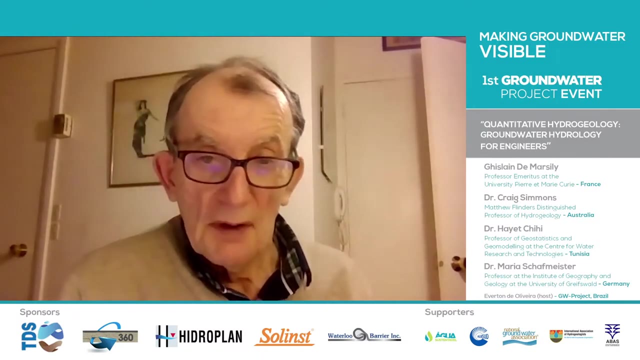 This is called artificial intelligence. It's to accumulate many data on the past and then use that very rapidly to extrapolate to the future. Now, there's no clear evidence that this can be used for groundwater, But still you have so many differences and similarities between various aquifers in different places. 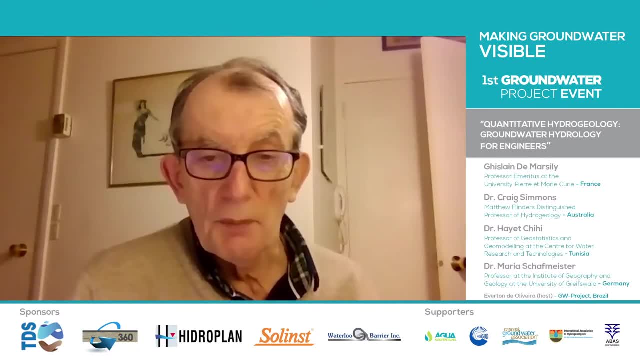 So then one should look at: is it possible to extrapolate, you know, the behavior of an aquifer based on another aquifer somewhere else? I'm thinking about South America. You have on the east, on the west coast of South America, you have a long, long, long, long line. 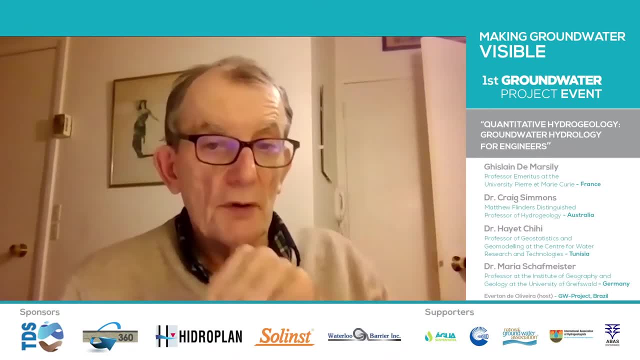 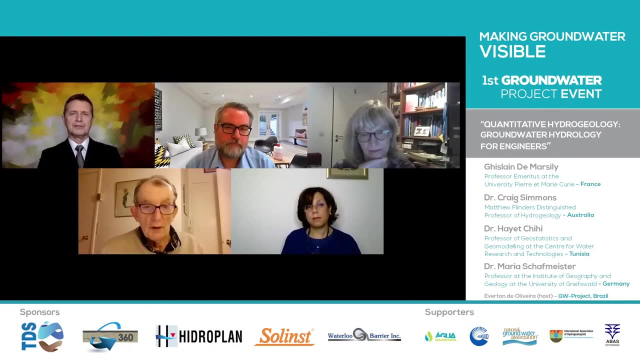 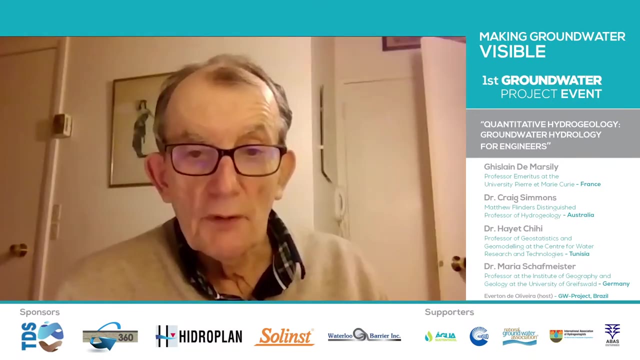 And you have the high mountains and you have rivers transporting sediments towards the sea. Each of these little rivers create a small aquifer, an alluvial aquifer, And these aquifers- I mean we have hundreds of small aquifers generated by the same phenomenon: mountain erosion, sedimentation. 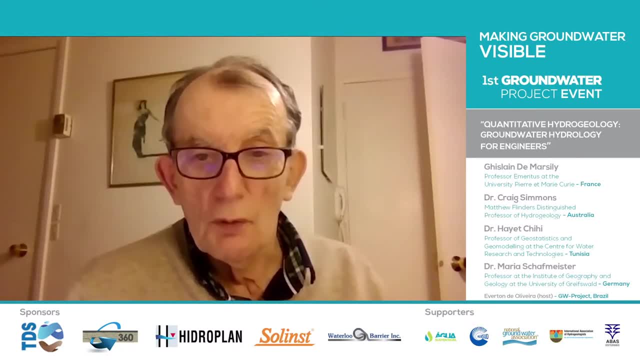 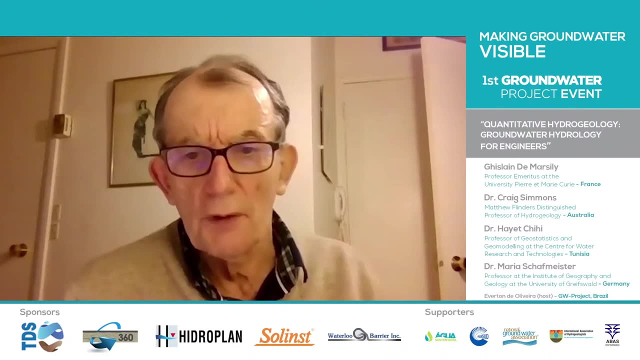 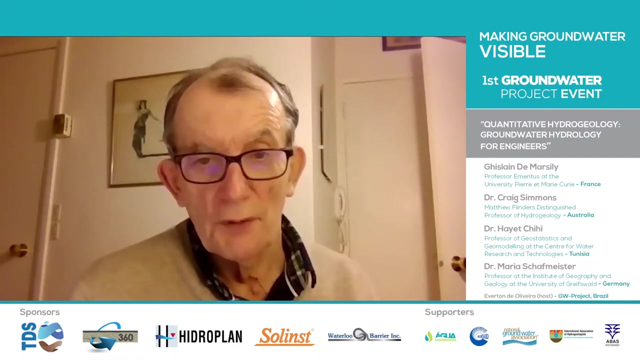 And there's certainly some possibility to use artificial intelligence to correlate what we see in one aquifer with what happens in others. So this is not modeling, but I think there is some benefit to make as trying to see if one can use artificial intelligence to improve our understanding of what happens today with hydrogeology. 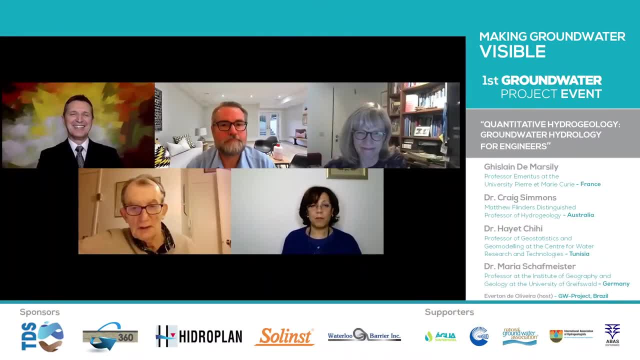 It's just an idea. It needs to be worked out. Are you cooking another book on that or not? No, no, no, I'm too old to write anything. You're good at that. No, no, no, no, no. 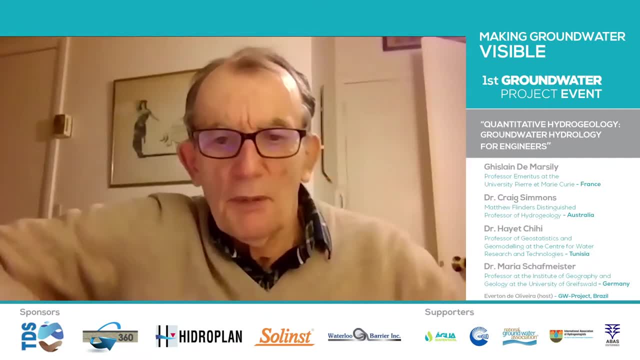 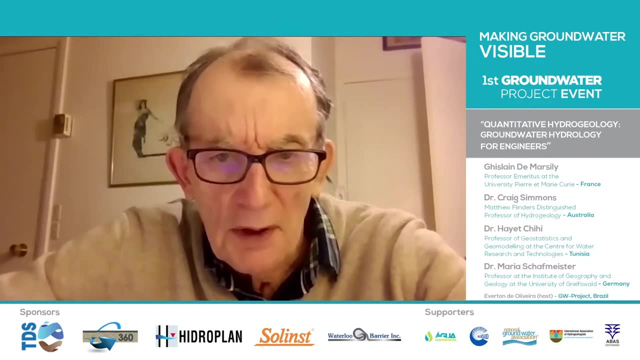 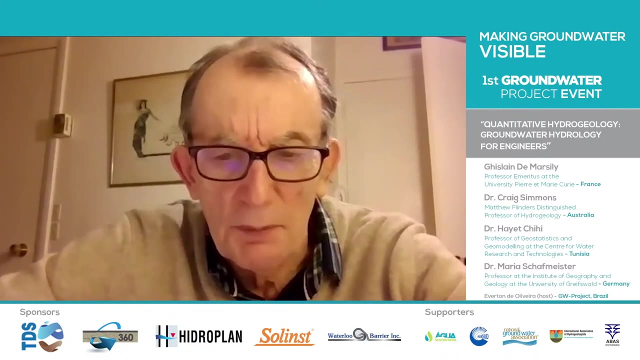 What I like to do is perhaps help others, help students, help younger faculty to develop and write what they want, But I'm no longer going to write a book. I was asked by the publisher of quantitative hydrogeology, Academic Press, To revise the book, make a new version. 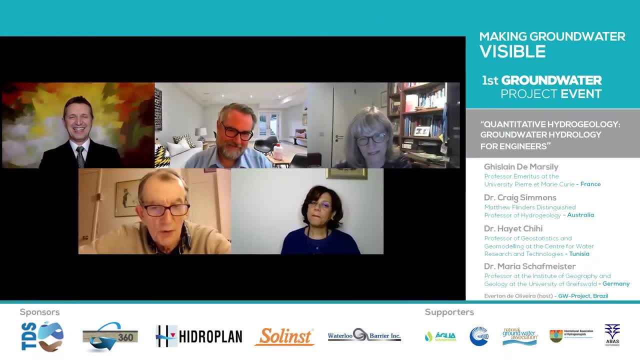 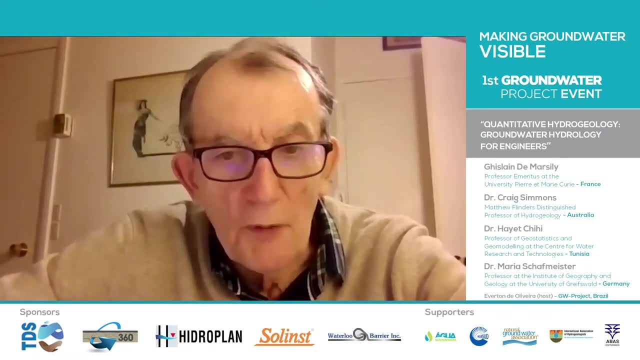 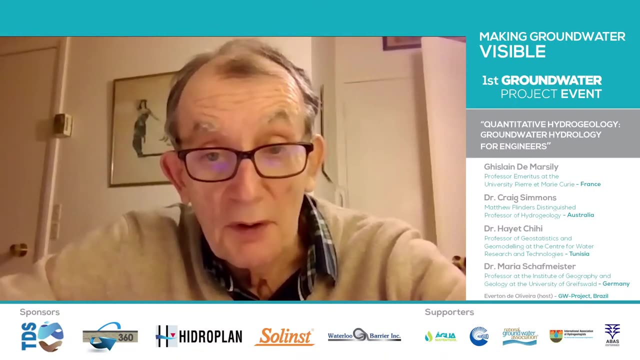 I realized that I couldn't do it on my own. I mean, it's too much. new things happened since the last 40 years, So I needed to have help from former students. So I approached quite a number of them and said: hey, would you be interested in revising my book and adding some new chapters and correcting the errors in the first version, and so on. 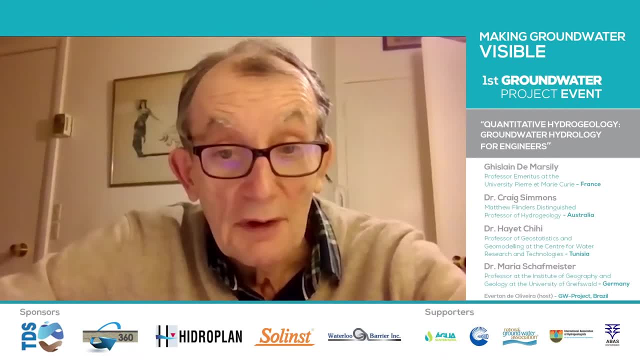 And all said yes, yes, yes, But in fact they do nothing Because you know you have better things to do than rewriting old books. So you should start new things fresh and go on with new ideas and new concepts and new authors. 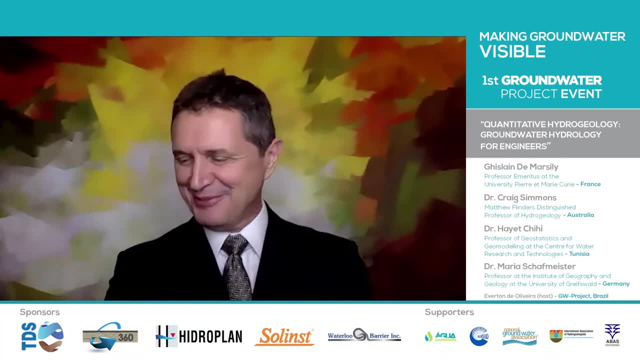 Well, you are. that's basically the idea on how the groundwater project arrived, Because it was a revision. The idea was to review the Freezing Cherry book. But then John says, well, what's the point? We need to rewrite new chapters. and things grew so fast. 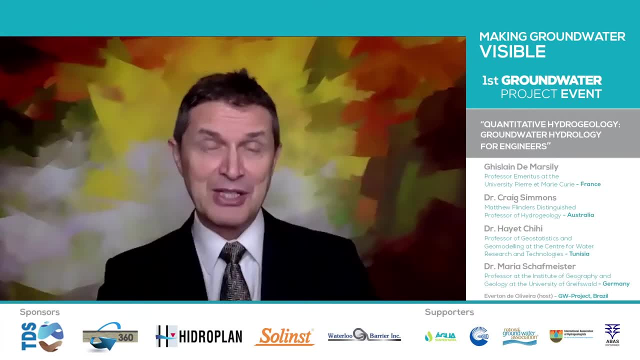 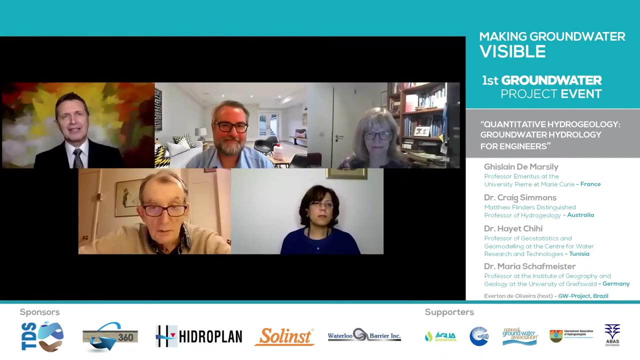 But I have one question for everybody, Because you have three colleagues that are here, of course because of you And of course because of Hayek, she invited Maria and Craig. The question is for the four of you. First is Ghislaine. what's the feeling? 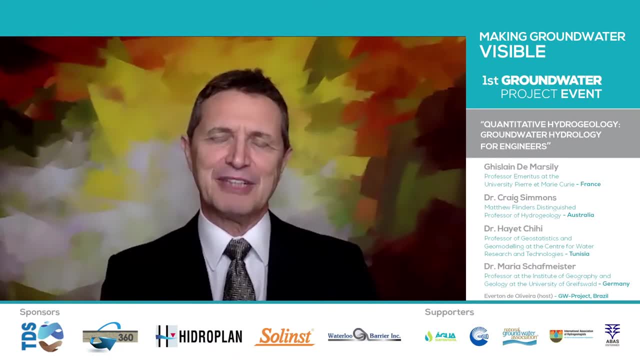 Because you know you're one of the finest and well-known hydrogeologists on Earth. basically, right, Yes, yes, Well, what can you say? Don't be modest. That's true And it's easy to see, because you have influenced people in Brazil. 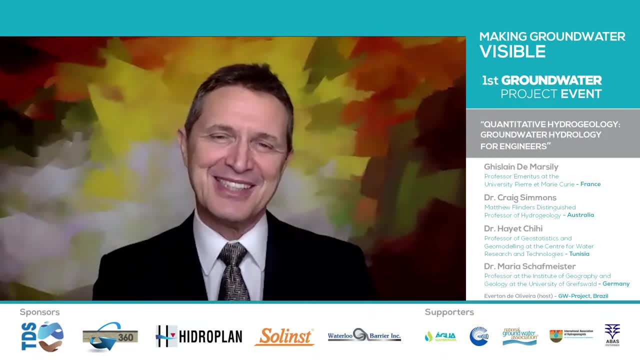 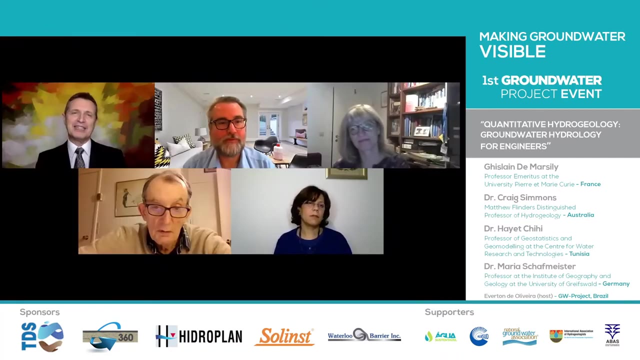 I studied it with your book. You have Hayek from Tunisia, You have Maria from Germany And you have Craig in Australia. So it is true, Okay. So for me the question is: what is the feeling of that? And for you guys, how did you get to know him? 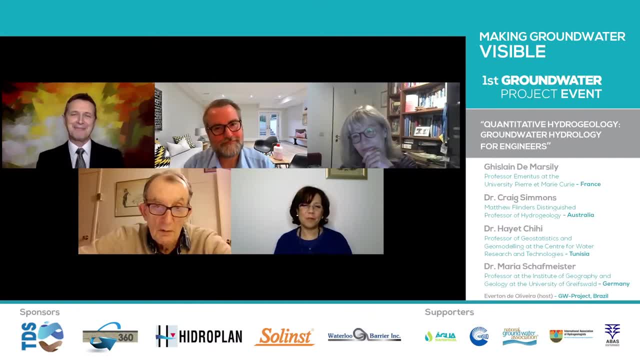 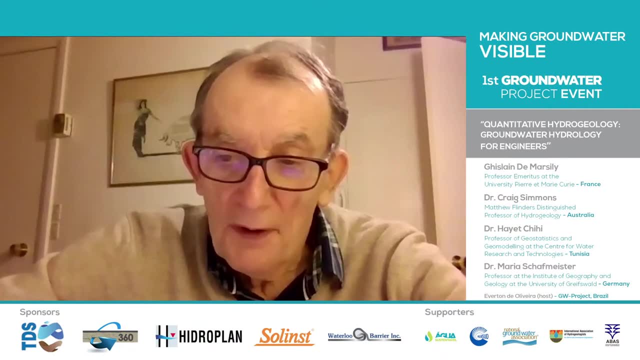 And what's the impression of working with Ghislaine? You can go first Ghislaine. Oh You know, If I think of going back to writing a book, I think it's really a personal work. I wouldn't very much like to share the writing of a book with even the best friend I have. 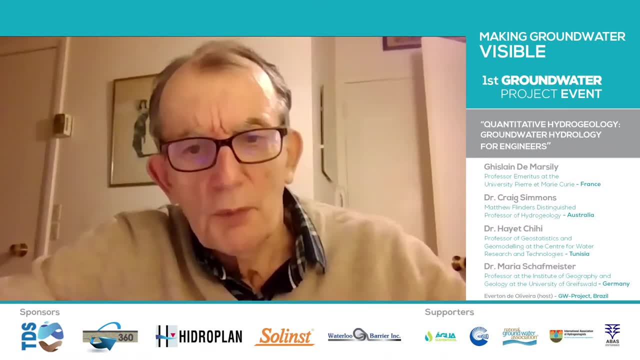 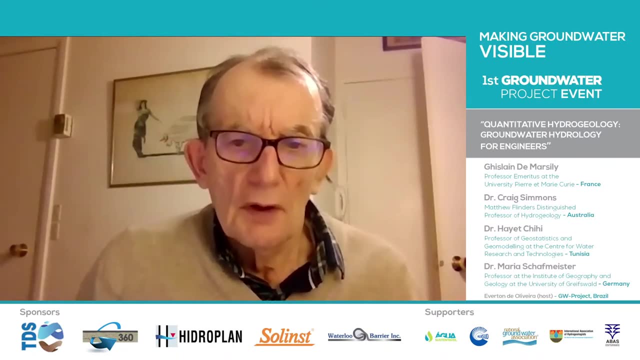 I wouldn't like that because you know it's something personal. You put your own spirit on writing a book. So what Frise and Cherry did was very good, because Cherry was bringing the chemistry And Frise was bringing the physics and the geology. 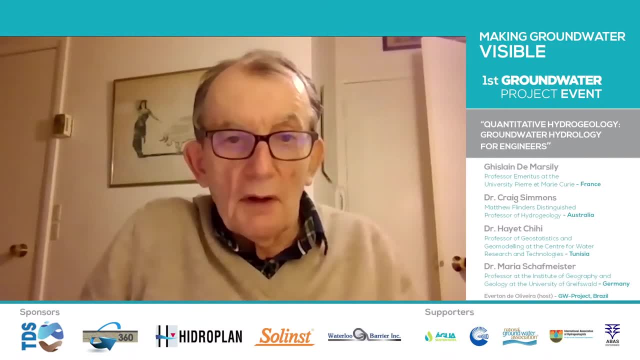 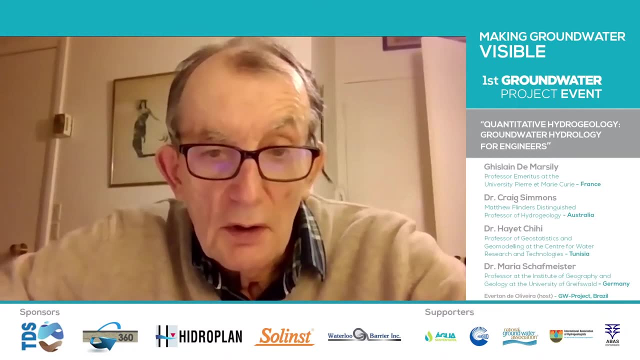 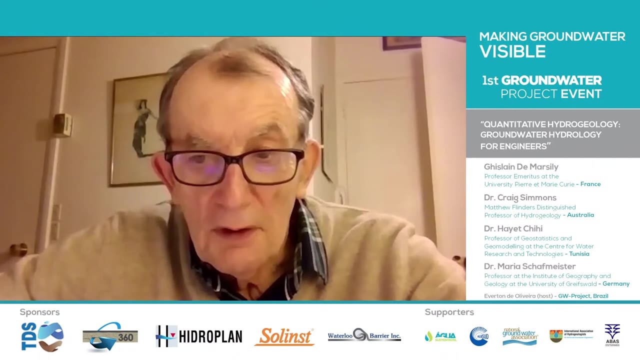 So this is a good way of coupling things, But when you talk about one topic like quantitative hydrogeology, you can perhaps divide that into a few chapters with different authors. But in fact, I think writing a book is something which is very personal and you have to have motivation to do that. 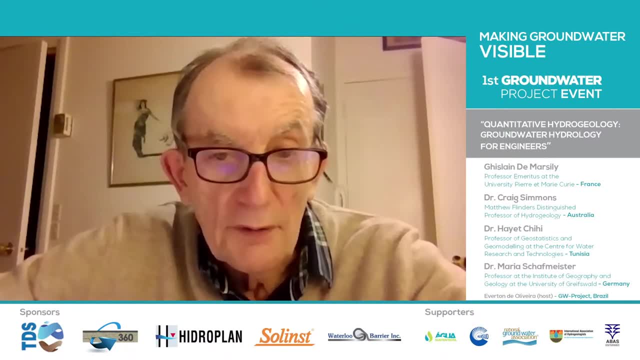 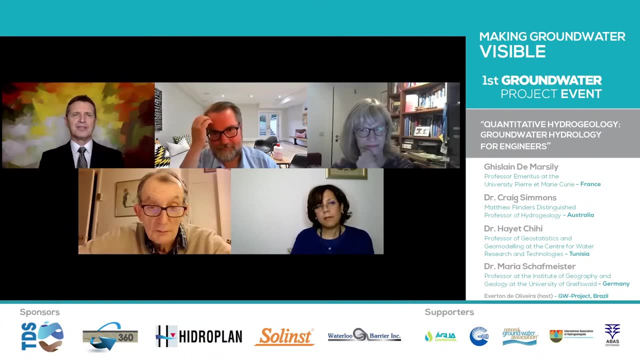 And it's difficult to do that As a large group. I think so, Yes, it is, It is, I agree, I agree. But the people, as you mentioned, they're producing books independently, They're producing independently. So that's how it goes. 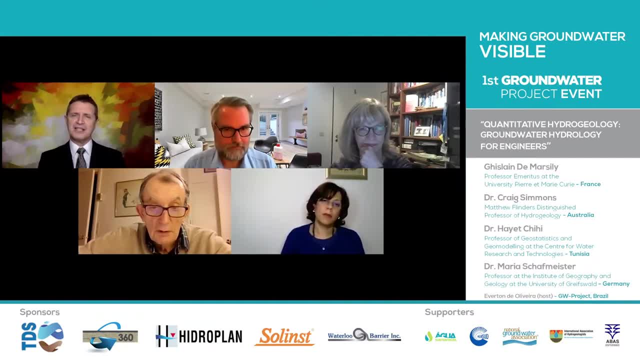 Yes, No, No, It wouldn't be easy. I agree with you. You guys, how did Ghislaine influence your lives And how did you get to know him and work with him, And how is it working with Ghislaine? 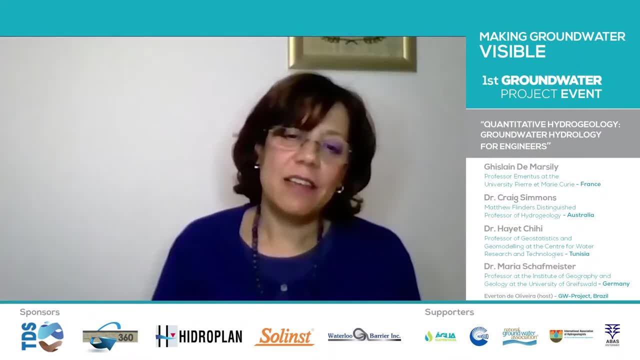 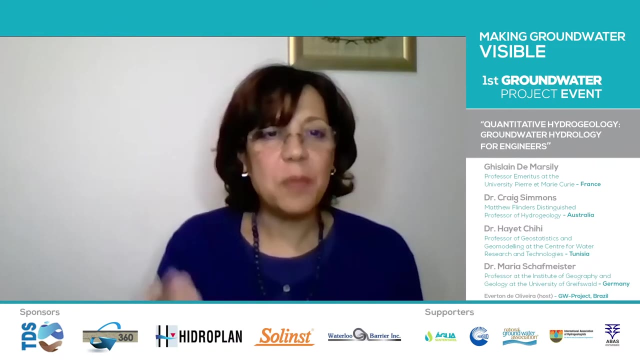 Haye, you go first. I think that Ghislaine de Marseille is a very humble, generous man. When he's speaking with you, he speaks with you as a very competent person in that discipline or in that science. So He started knowing you, how you are working, your personality. 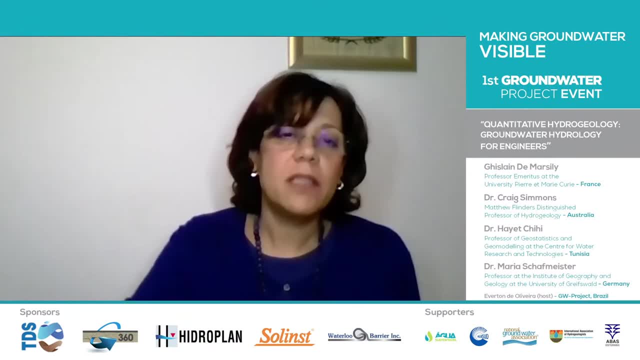 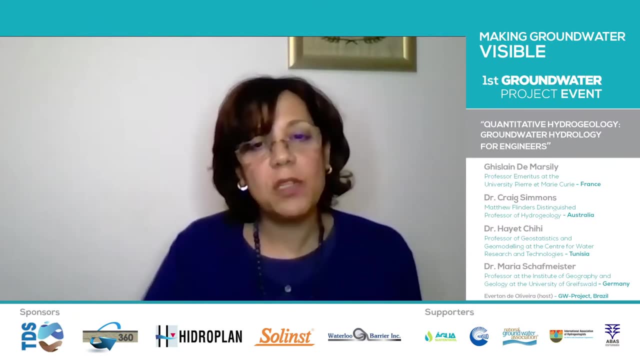 And then he invites you to study at your mana. I remember when I was a PhD student of Ghislaine de Marseille, the first question was: have you a home? Yes, Yes, So that's the first answer. You started doing your thesis. 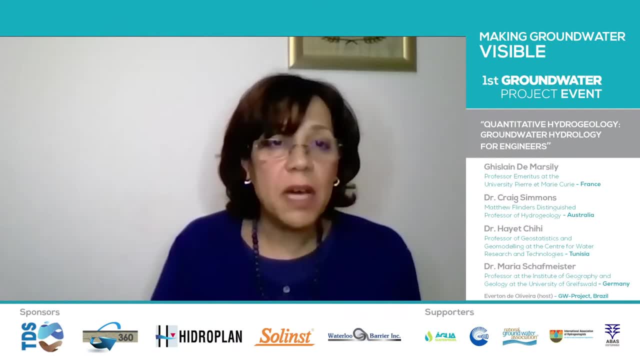 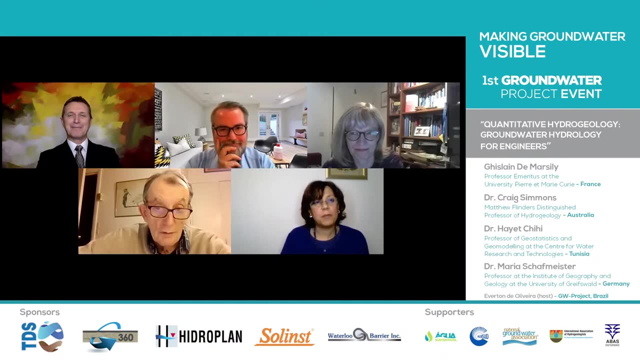 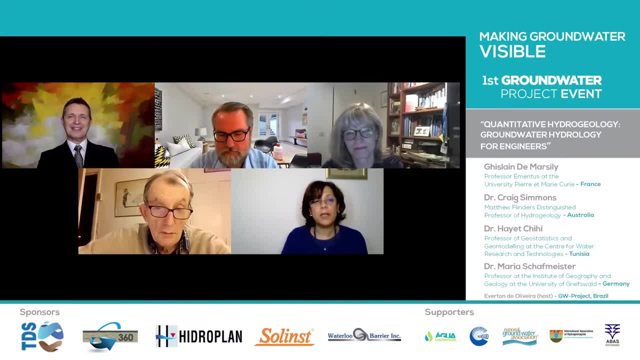 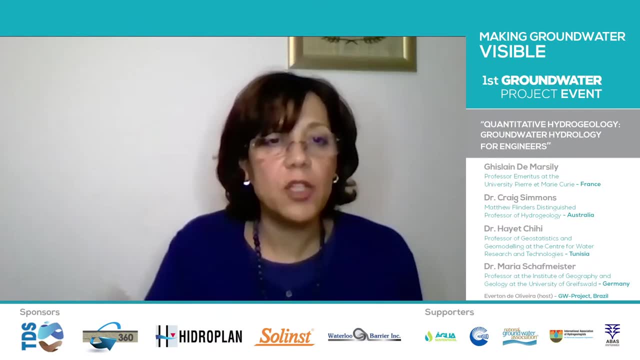 Yes, Yes, Yes, Yes, Yes. Michel Tesson to help me in sequential stratigraphy. He invited Alain Galli to help me in non-stationary geostatistics And he's continuously helping me to, for example, 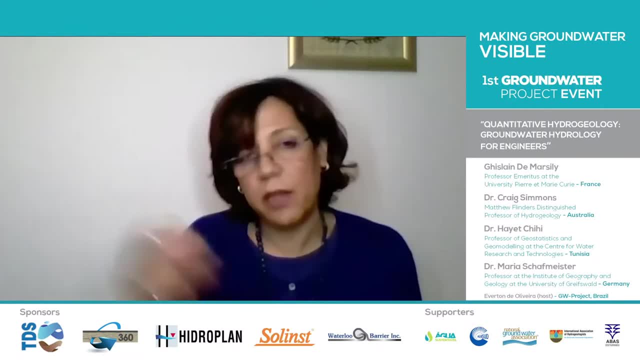 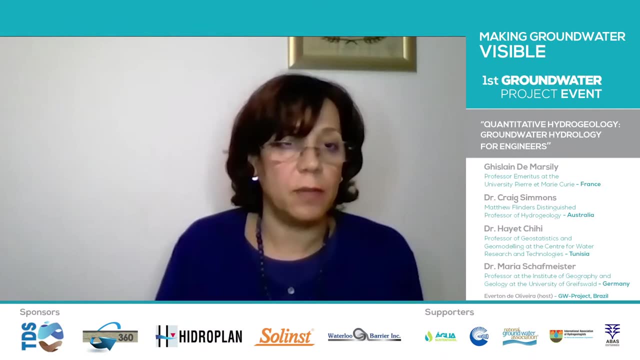 the major difficulty in Tunisia and everywhere for modeling aquifers is the data scarcity And how to do this By cooperating with other international institutions or who are working on software like GeoVariance, for example, And this is very important, And he's one of working a lot. 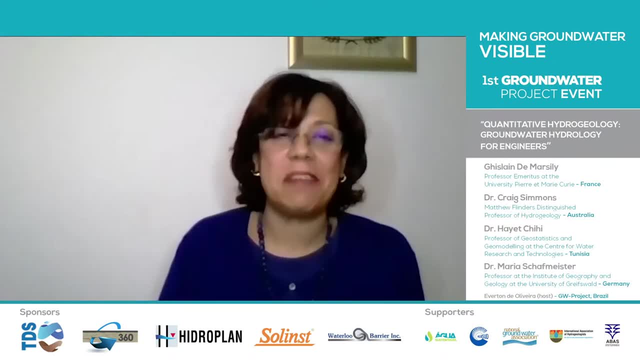 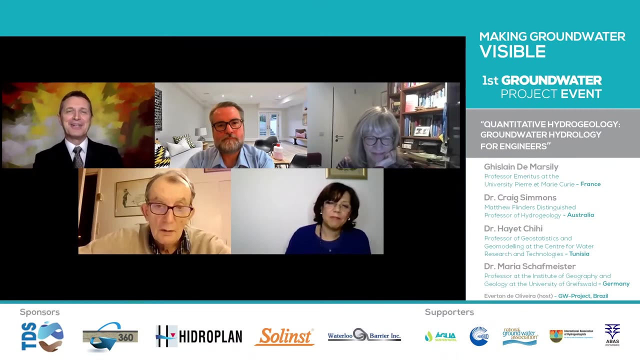 Even with my students, I'm doing exactly the same thing. They are my sons and my brothers. They are my family and not a stranger person. That's very good. This is very nice, Very sweet. Thank you And, Maria, please your experience. 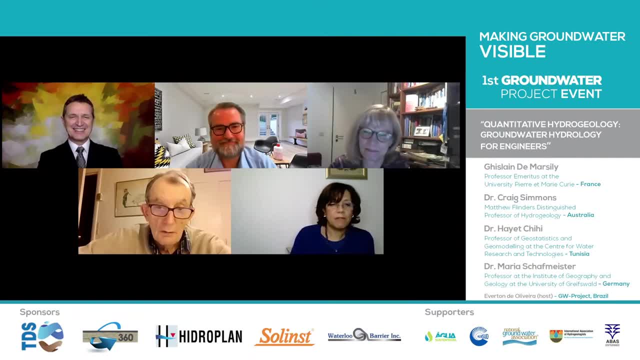 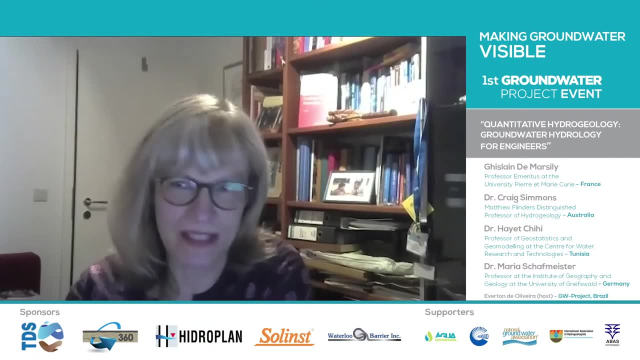 I can completely confirm what Hayat says, But maybe I can also add something. Gila was always very inspiring, So when you discuss with him, you soon get new ideas you never thought of. So, as we just had an example a few moments ago, 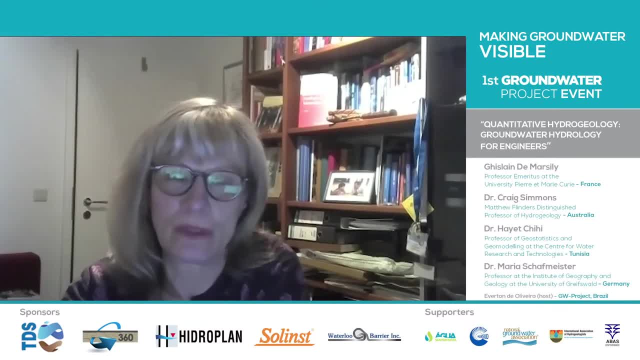 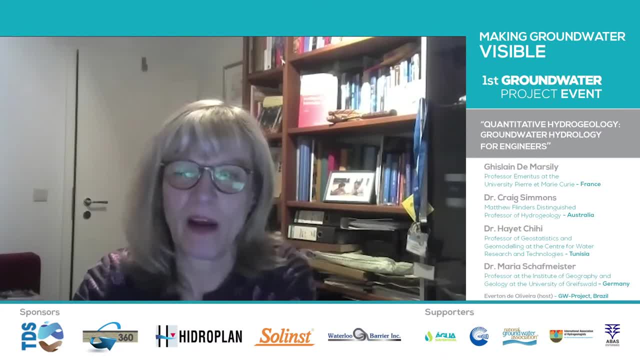 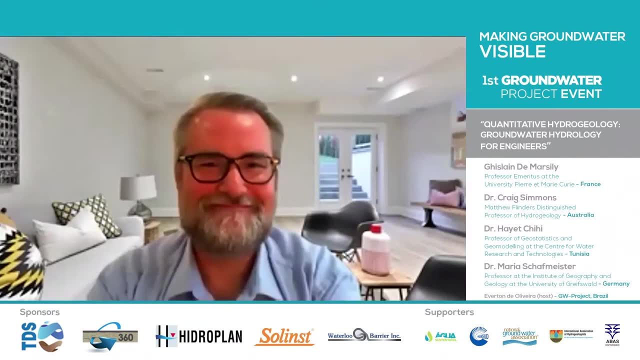 I found a new course with you, Gila, on geostatistics in hydrogeology, And at that point I already thought that I had understood the principles of geostatistics. But that wasn't true. But then you gave some examples. 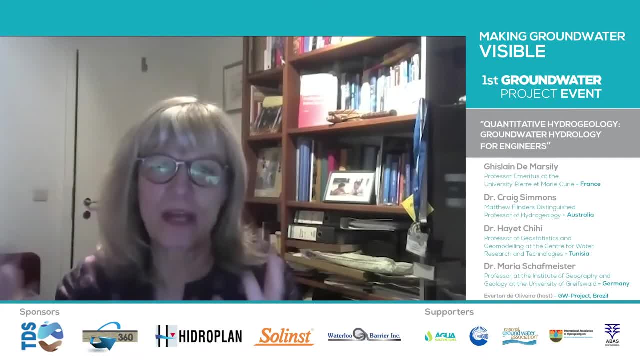 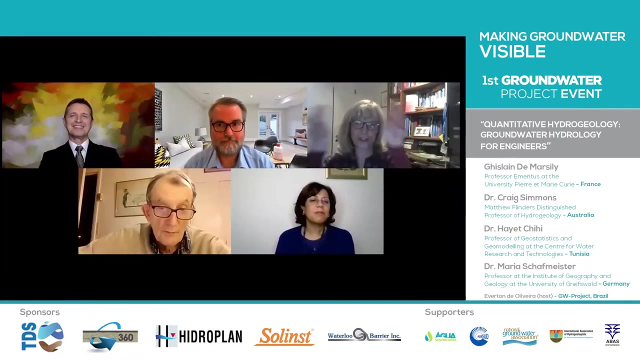 And as a geologist not too familiar with equations, so you always put some illustrations- I remember how you tried to explain to us the geostatistic pairing this with those dunes in Tunisia- you remember this. So which all have the same shape. 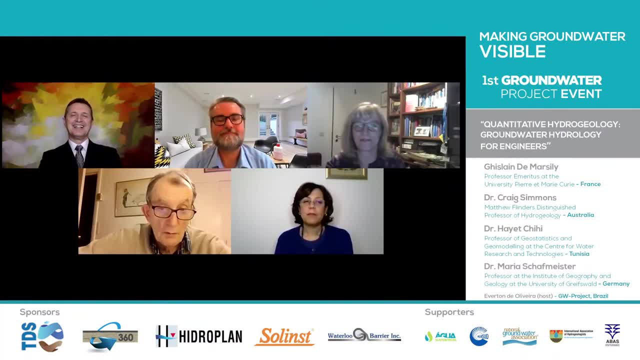 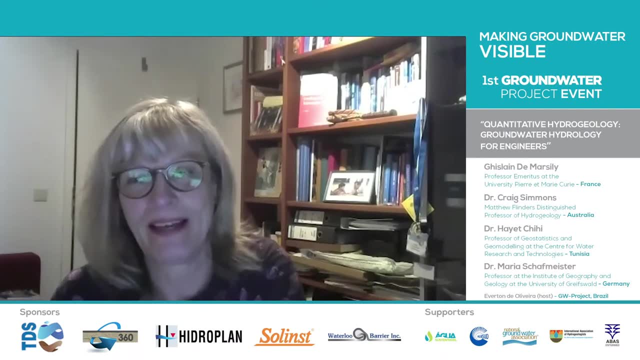 and so they are all analogs of one variable. So this I liked very much and well, this was extremely inspiring. And one thing maybe I'd like to say: I have learned something from you, and this is- it fits into these times today. 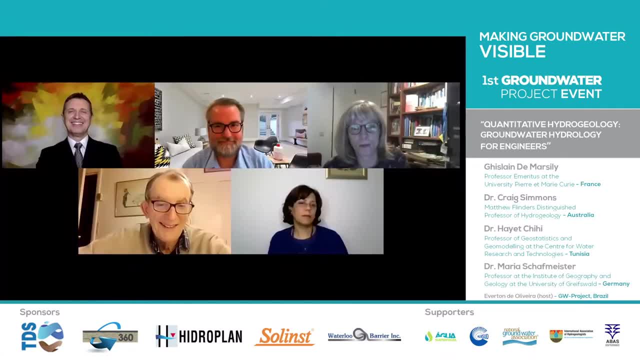 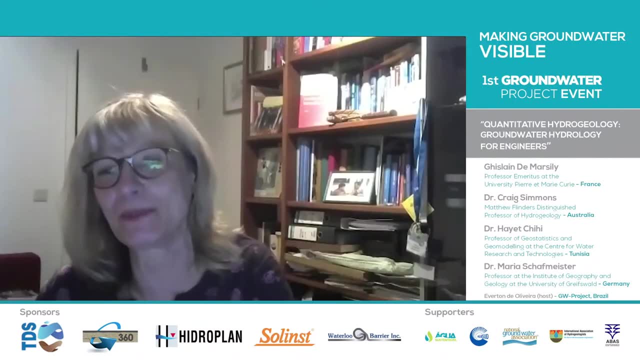 Since I know you, I drink Corona beer. You might remember that we once traveled together and we had some beer and this Corona beer doesn't make this foam which we Germans like, and I was complaining about this. but since then I only drink Corona beer. 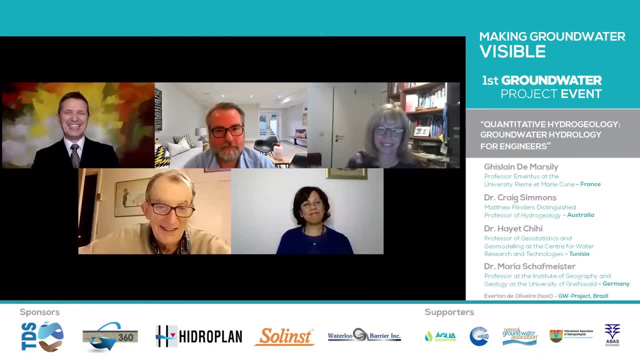 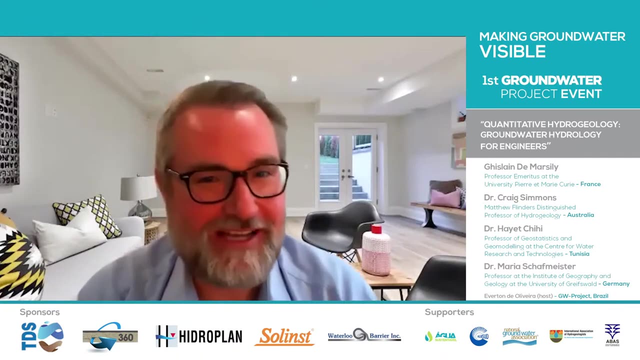 no German beer. So this is something I have from you, Not the only thing. Thank you, Maria. Thank you, that's very nice, Craig, please. Thanks, Everton. I first met Ghirlane it was in 2006. 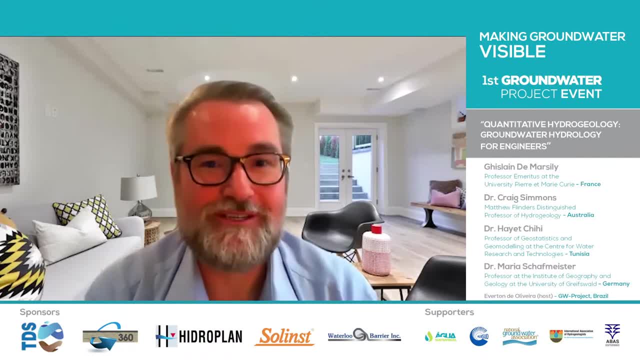 and it was at the Groundwater IAH Conference in Dijon in France. It was the 150th anniversary conference of Darcy's Law And I think that the way in which this came about speaks a lot about Ghirlane and the way he thinks. 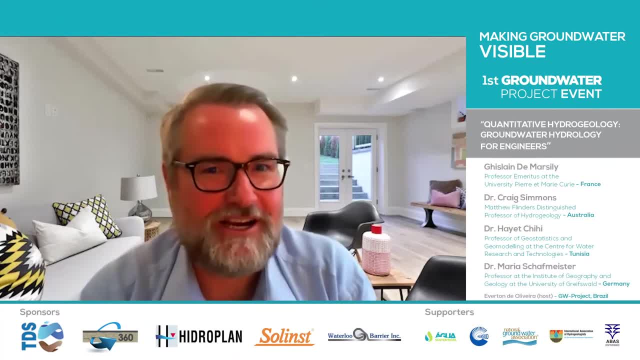 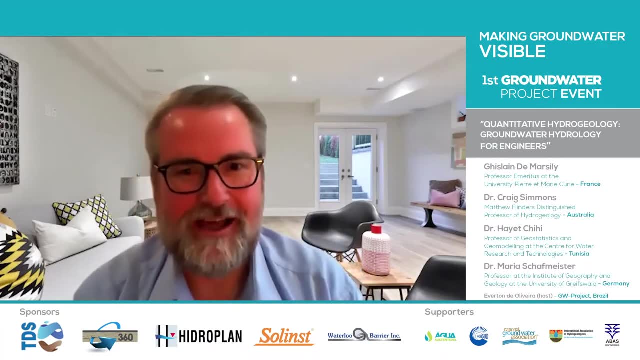 And I was in my early thirties at the time and had an interest in Darcy and had written a little editorial for Hydrogeology about Darcy and so forth, And Ghirlane had invited me to give the opening plenary address for this conference. 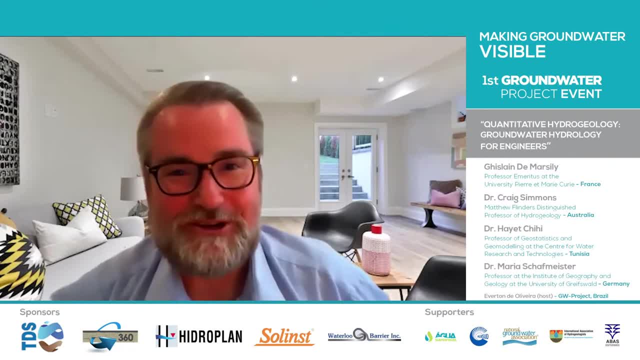 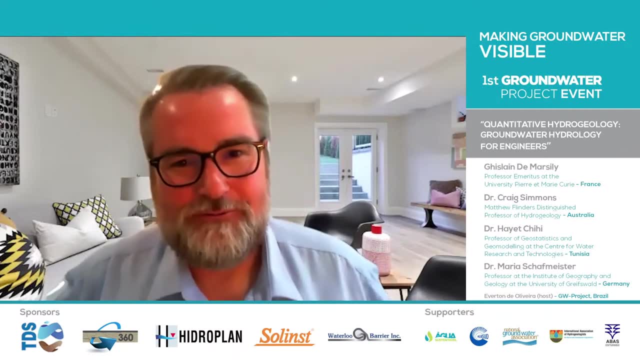 So taking a chance on an Australian kid to do this, I think was a little bit about how Ghirlane thinks, but thank you, Ghirlane. And so So we've worked together. Ghirlane was involved in chairing our international board. 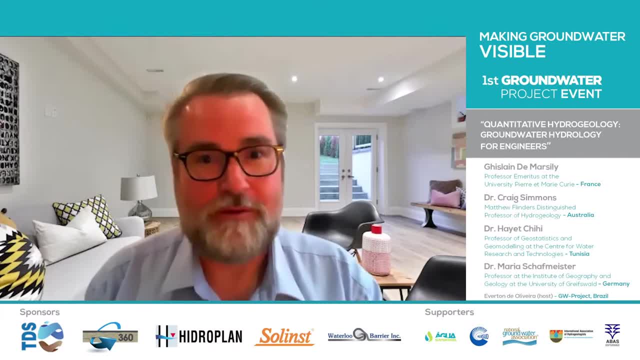 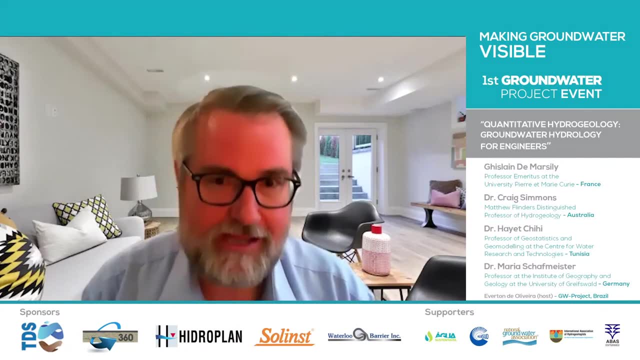 for my center and really inspiring me but many other students both in our center but also around the world, And I know personally that Ghirlane has been a mentor and an advisor and a friend and really a philosopher guide that has really helped and shaped so many aspects. 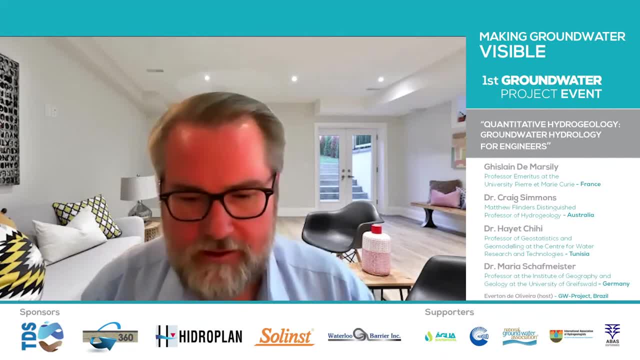 of my career, And so I agree with everything That's been said. I find Ghirlane to be extremely generous and selfless and highly dedicated to the people that he works with and to his students, And I know that all of the students that I've spoken to- 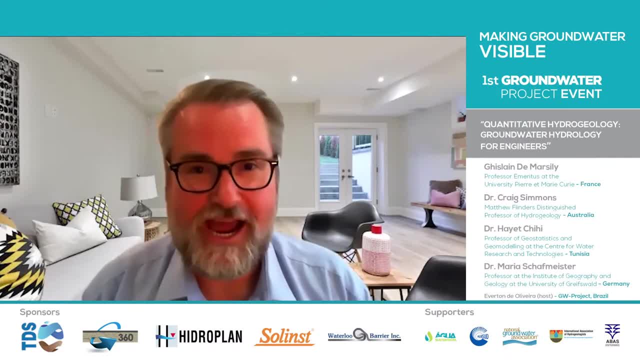 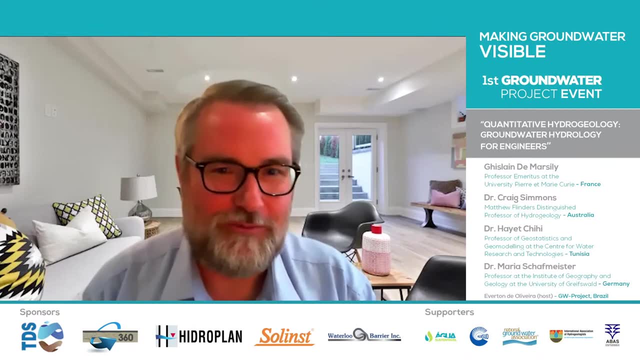 that have worked with Ghirlane and his colleagues feel the same, And I heard them recount- I don't know if this is true, Ghirlane- of late nights in the laboratory where they would be working and you would be coming into the lab nearly at midnight. 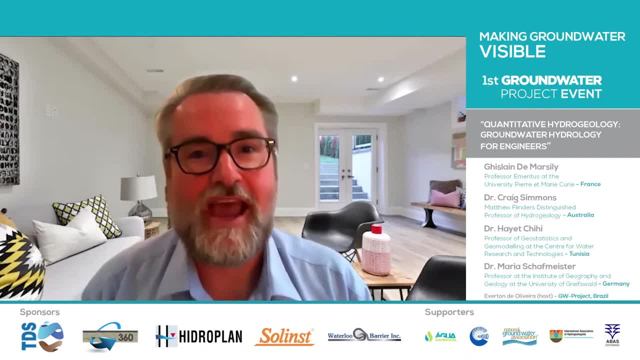 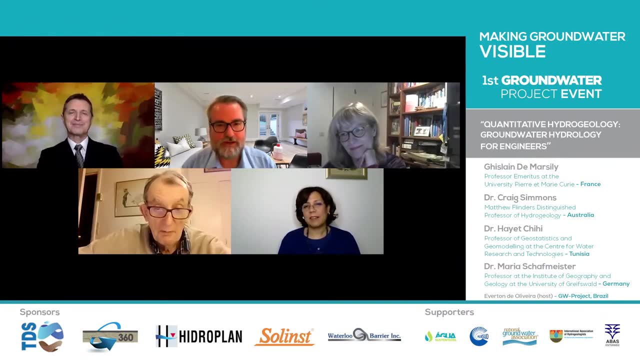 and so forth, And so you clearly had the passion and the energy and the commitment throughout your career, for which we're all very thankful really. So it's been a true honor to work with and know you. Thank you, Craig, Thank you. 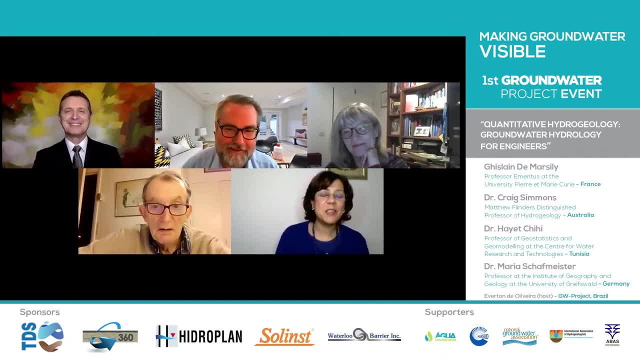 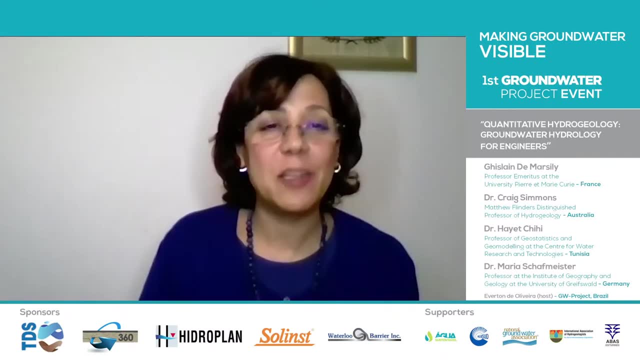 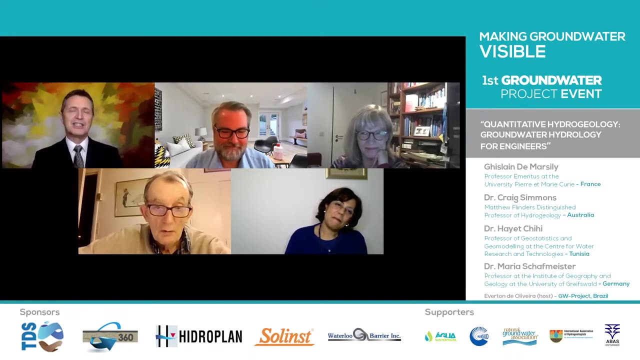 Yeah, He is spreading science, peace and fashion. The Mercedes is spreading science, peace and fashion. That's very true. That's very true, Ghirlane. one question: You just mentioned that your friends at the time mentioned that you're crazy about writing a book. 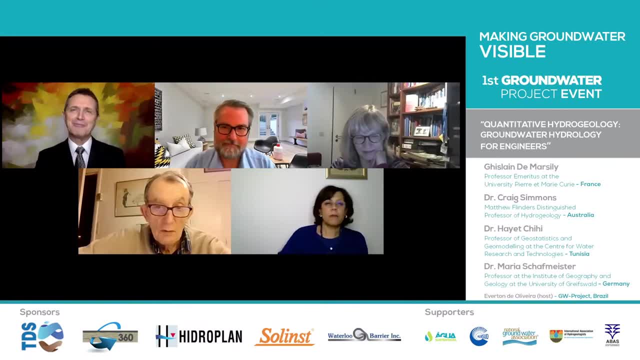 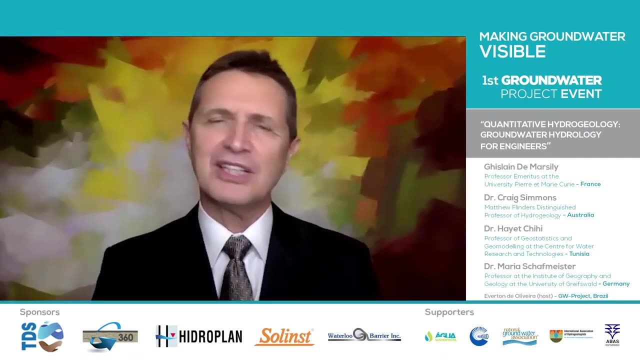 because you do better publishing papers. Papers matter as more. This is a very, very important point today, because today books, printed books, are very expensive and professors are not interested in publishing books. They're not interested in publishing books. They're not interested in publishing books. 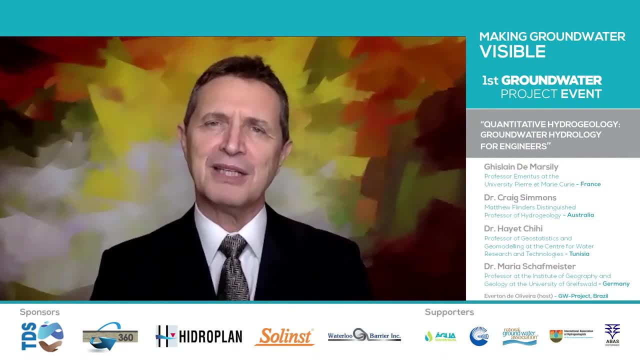 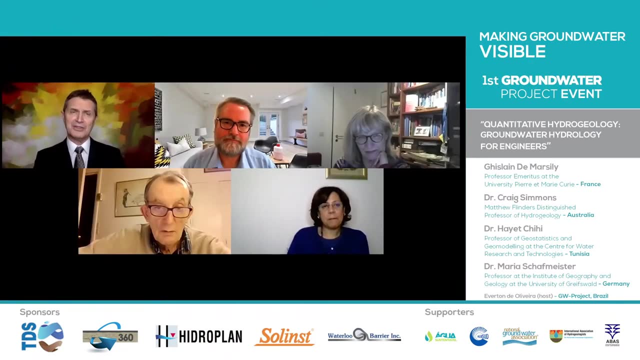 You don't see many textbooks being produced. You showed one, but we don't have as many. We have some older books And now our idea with the Groundwater Project is to spread knowledge. One question is if people say don't write it. 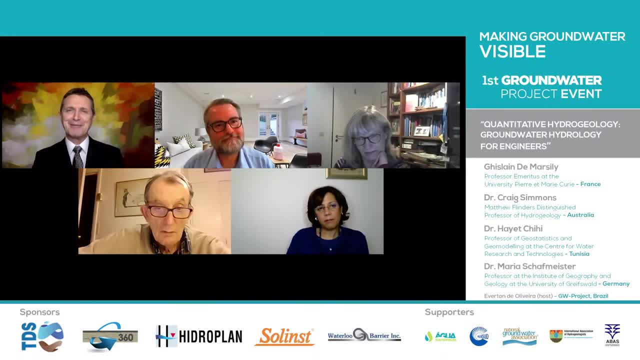 because it's not good for you. You could write a paper. it's more important. And another thing is that we know that books don't make you rich, right? So if it's not good for a scientific career and you don't make money, right. 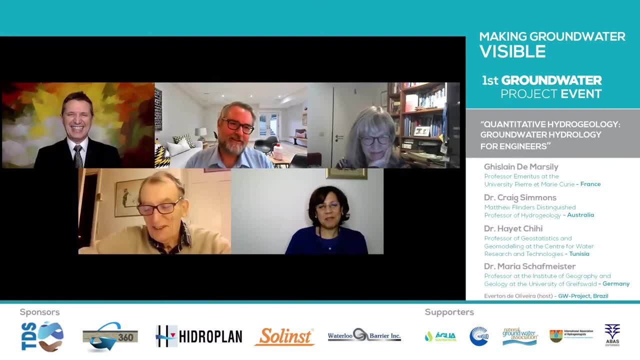 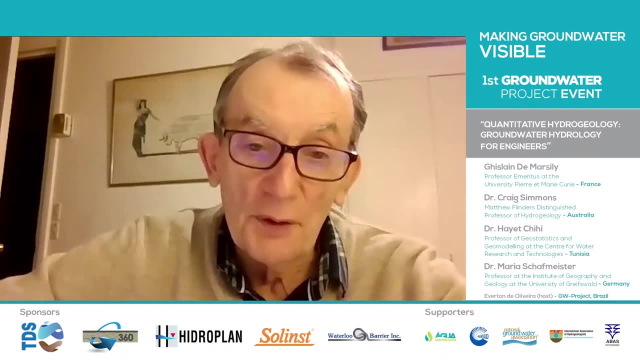 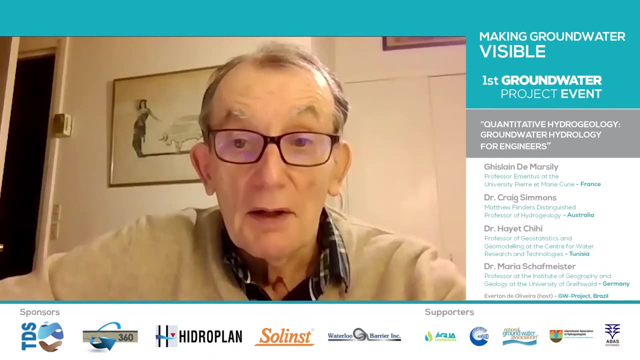 Why write a book? Yes, it's a good question, But my goal in life was not to make money. That was not my point. And my goal in life was perhaps has been said by Maria, by Hayat and by Craig- is to try to help. 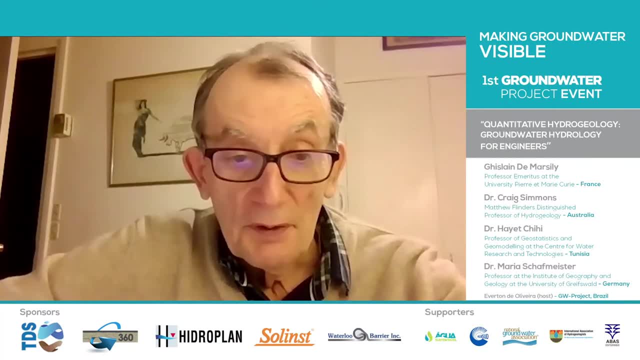 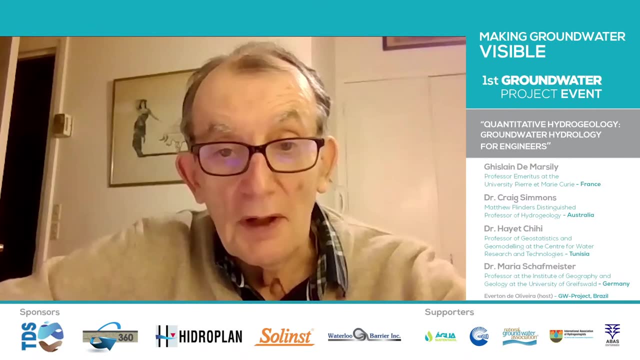 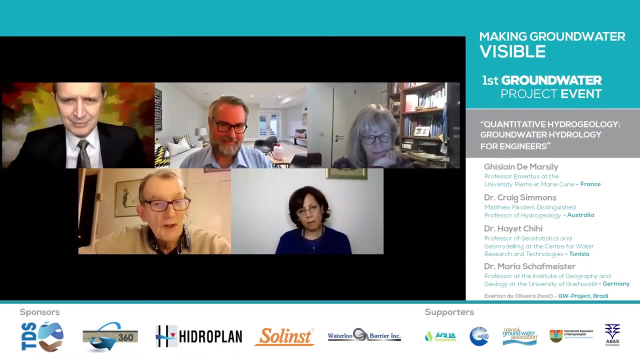 students and to help colleagues. And to give you an example: today, unfortunately, in my view, most professors in class use PowerPoints and they have projectors and they show graphs and so on. I would never do that. I mean, I've been trained to teach. 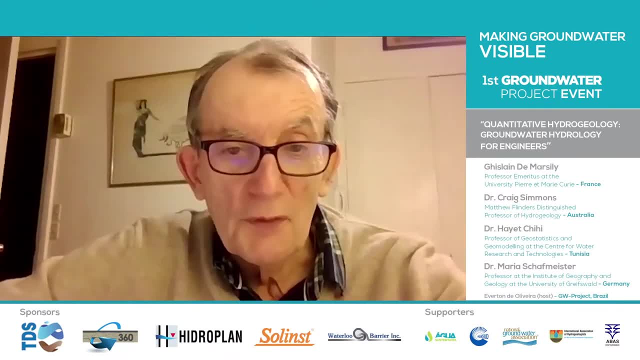 with a piece of chalk and a blackboard, and I think you transmit much more information to your students by writing on the blackboard, showing them a beautiful, well-arranged with nice colors PowerPoint image. So it's probably more time-consuming to write by hand on the blackboard. 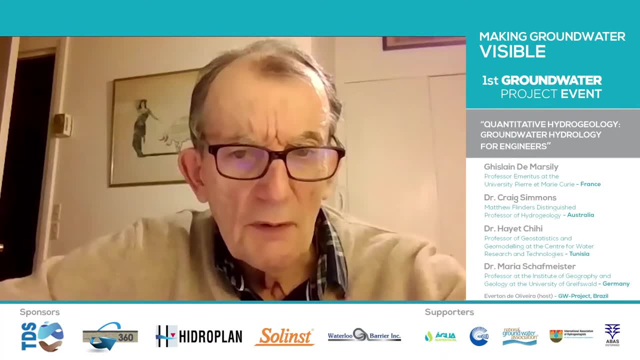 But it's more efficient And what I like is to have efficient methods to teach, And I don't think that a PowerPoint which is nice to do and can be reused in the next course next year, I don't think that's a good idea. 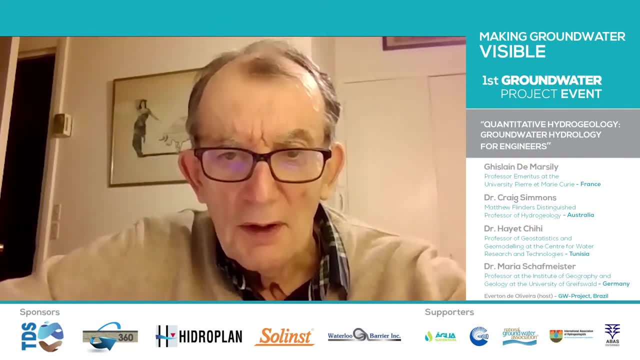 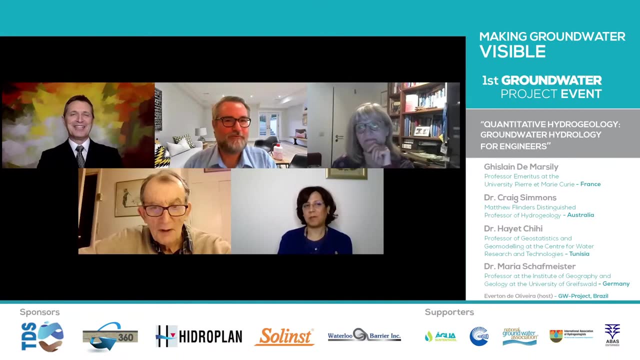 And maybe economically it would make sense. But you know to teach. I don't think it's a good idea. We've heard from students. I've heard from students Everton that the students absolutely love Guylain's lectures on the blackboard. 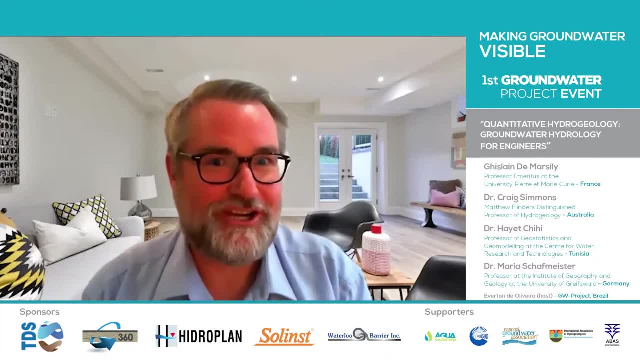 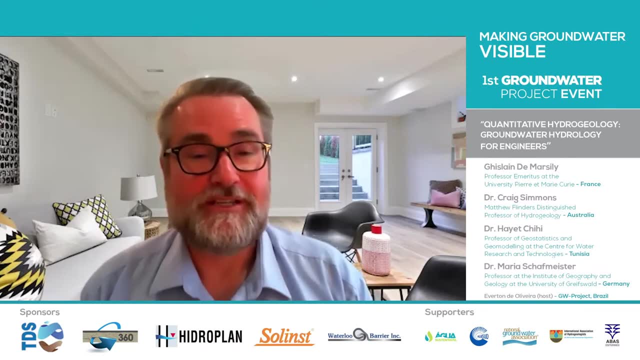 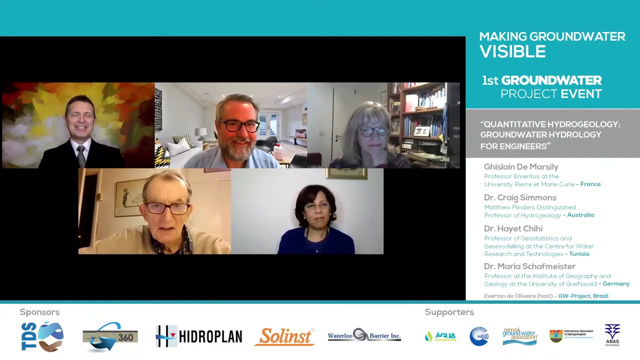 And when you were in Adelaide a few years ago, Guylain, you gave a lecture, It was on a whiteboard because the blackboards had gone And the students were just Just loved it. Yeah, Thank you, Craig. Well, but it's a, you know, I agree with you. 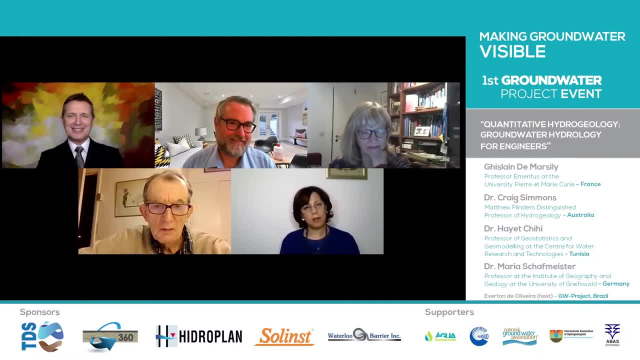 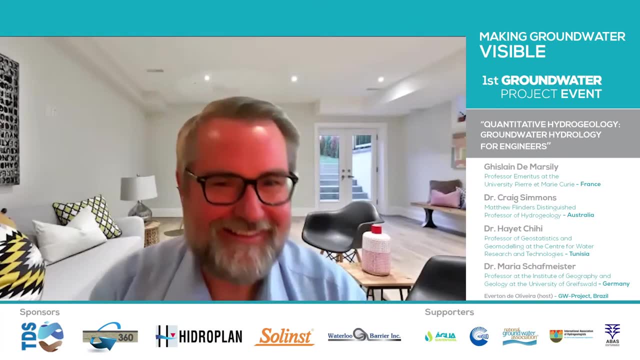 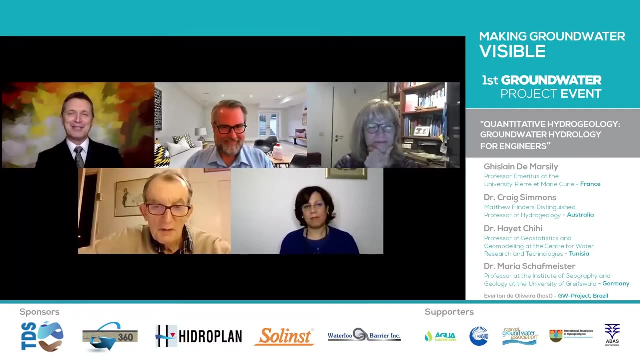 But using a blackboard, well, it's a talent. Not everyone can do it. You do it naturally, But you don't think that that comes naturally to anyone. That doesn't happen that easily. No, that's why, people, It's much easier using PowerPoint, because you can play around. 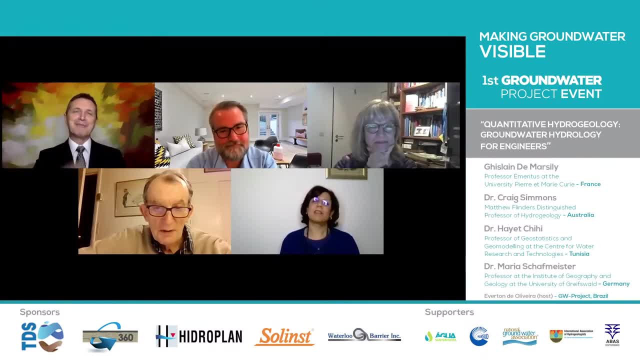 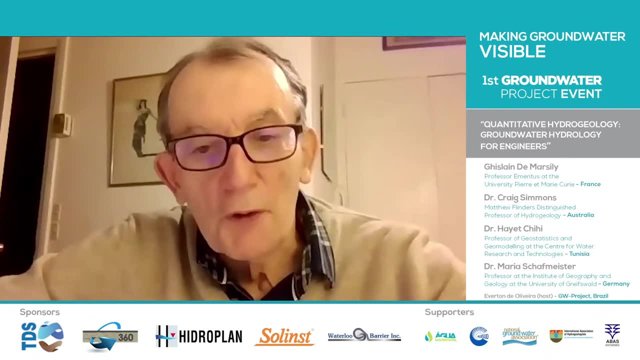 You can bring in, You can do nice stuff. but preparing a nice blackboard it's not easy, You know. it reminds me of my first experience. The first year I started teaching that course. I was writing on the blackboard. 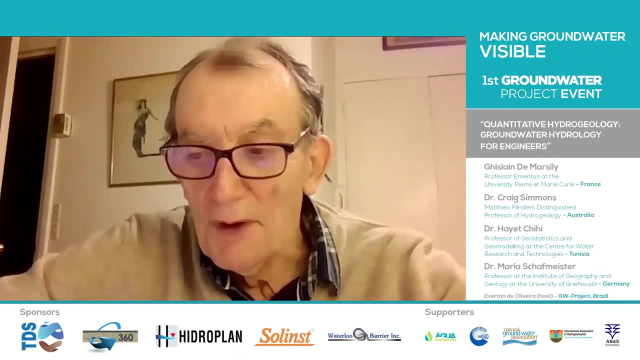 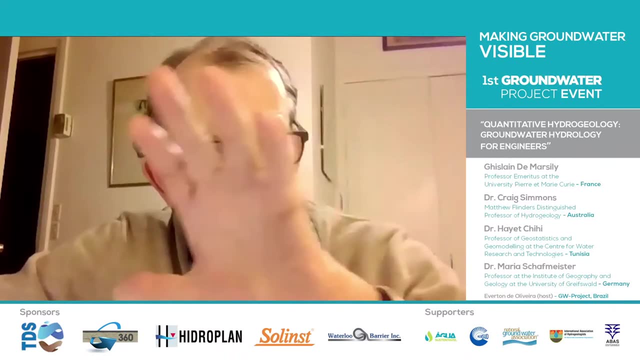 And at the end of the class a student of the class came to me and said: Sir, writing on the blackboard is fine, but you have to have a well-organized blackboard with things that follow each other and so on, And it's neat. 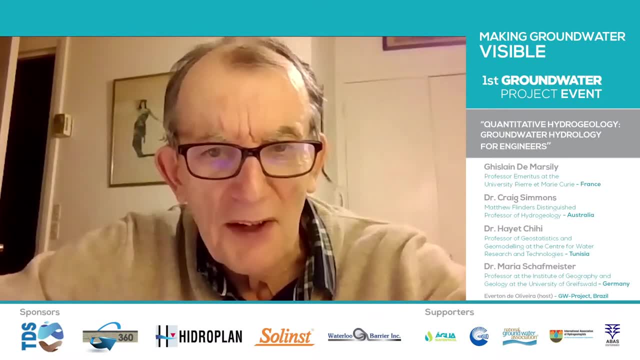 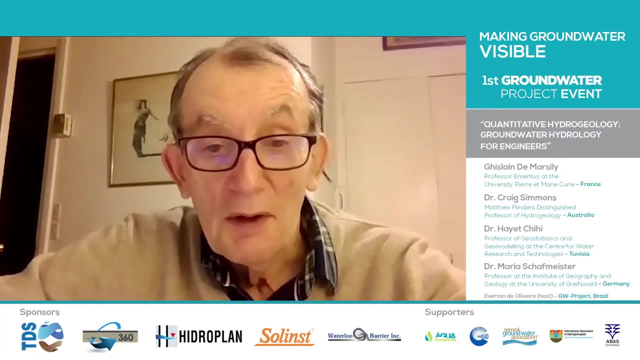 And you? You are messy. What you're writing on the blackboard is completely messy and I don't follow you. So you have to teach and learn how to do proper work, proper job with teaching on the blackboard. But I'm afraid that any class today doesn't have a blackboard anymore. 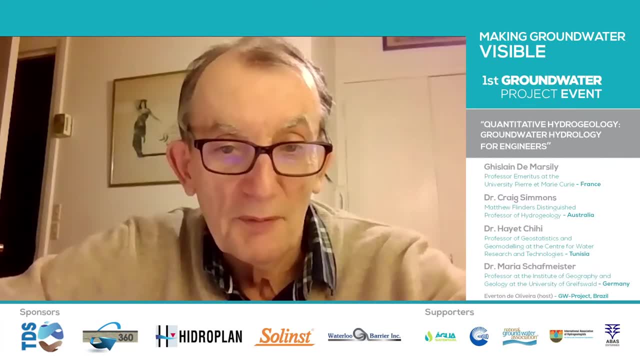 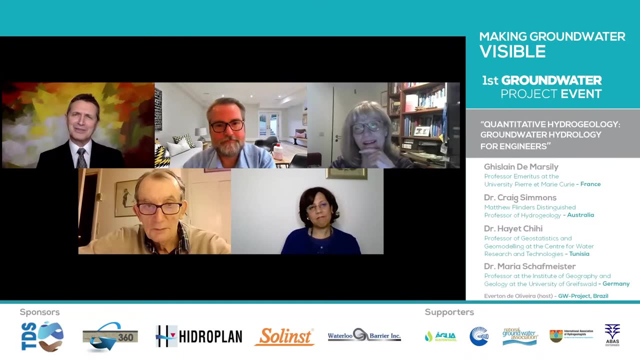 Even a whiteboard. they don't have anything, just have PowerPoints, which I'm not happy with. Well, I think there are black or whiteboards. I'm there. What do you think, guys? I may say something. Actually, the blackboards are going away. 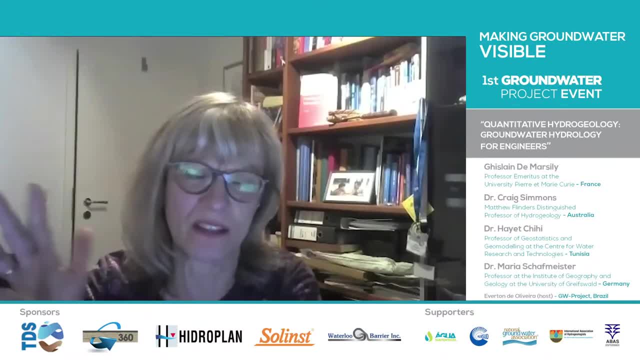 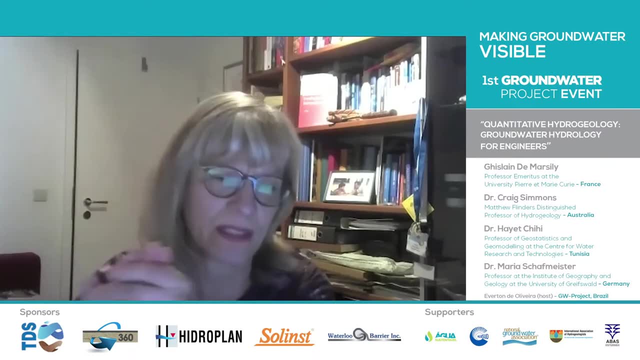 The whiteboards are again. Now you have some mixed technique between presentation PowerPoint and presenting it to the wall and something like this. However, we must say I mean since last year, March, I do all my lectures on this same place here- 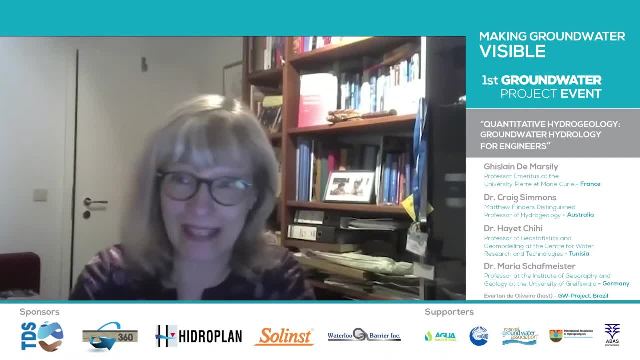 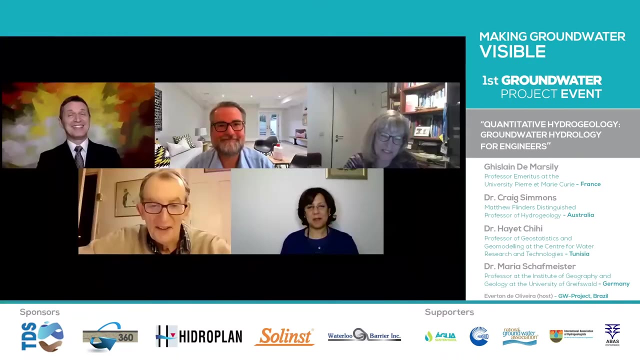 looking into a blackboard. So I have a black screen due to Corona, and well, I would love to do my paintings again, but in Corona times we are happy that PowerPoint exists. Sorry, Yeah, It's a good point, It's a good PowerPoint. 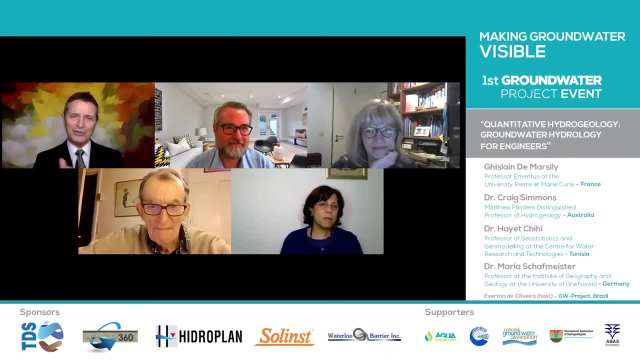 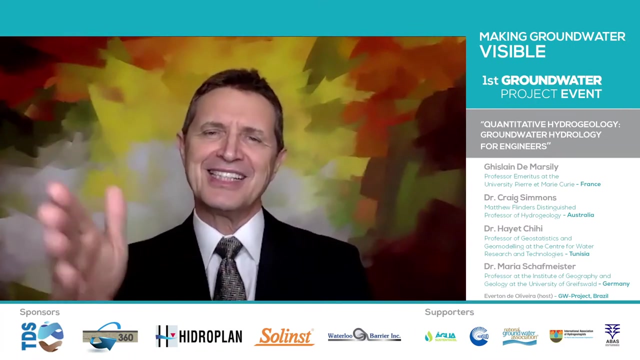 Well, you mentioned one thing. Uh, you, you want to say something, Craig, please go ahead. No, no, no, all good Everson. So the one point, Guillaume, you, when you write a book, and I, I, I study on your books. you and Hayad mentioned, and Craig mentioned that the you know your thinking is properly organized for, for, for a reader. 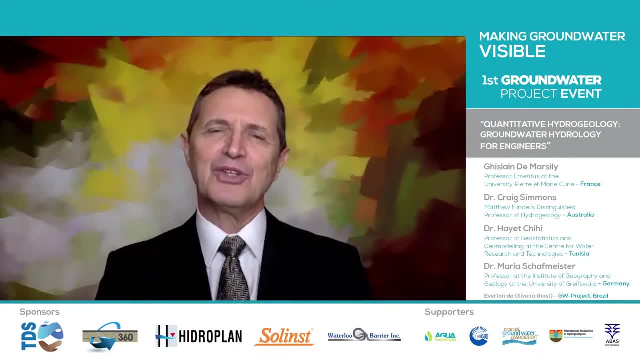 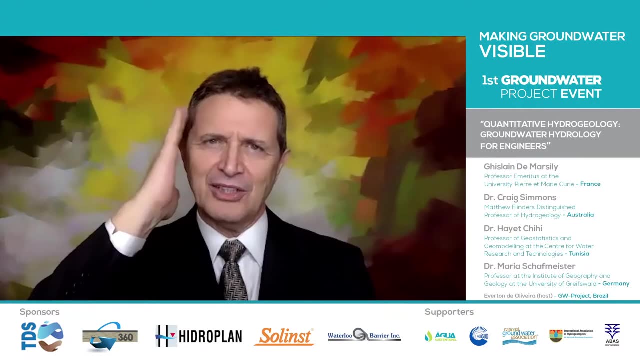 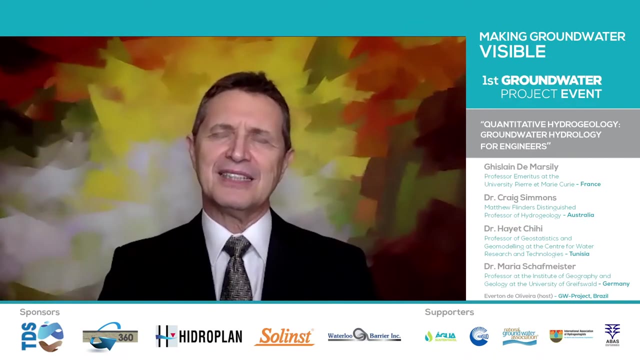 It's good to learn because it's organized And when you go and prepare a presentation, you're not going to make any mistakes. presentation yourself that is not organized, you have to have an all organized in your head and and as you go on the blackboard, uh, if you have it for you, like i mentioned, it's a talent. 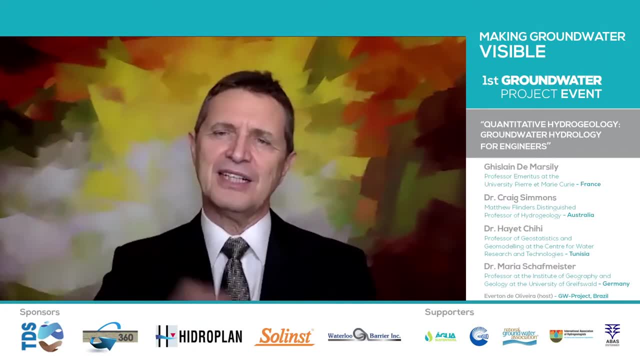 it's easy, but it's not for anyone. and you go there, i remember i, i just like you, i go to to to my students and say: well, you have to learn how to use the, the blackboard or the board, because sometimes you go to a meeting doesn't have to be a a classroom, you're going to present something. 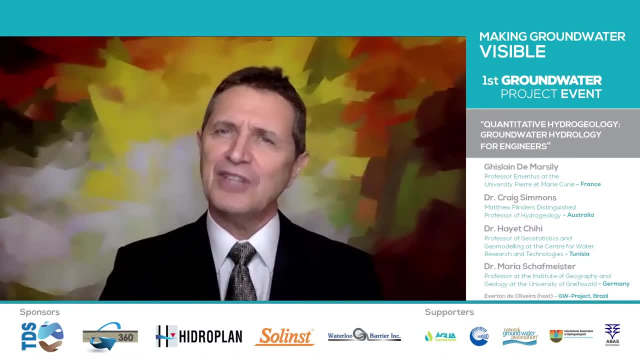 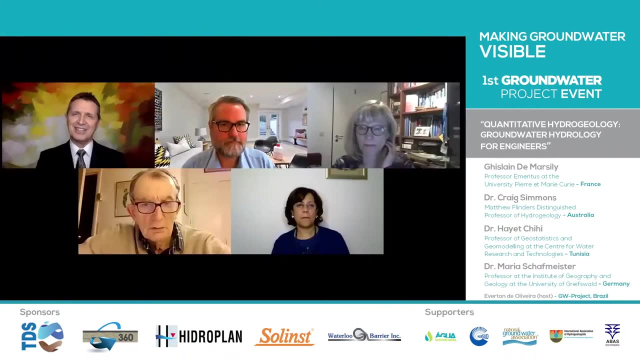 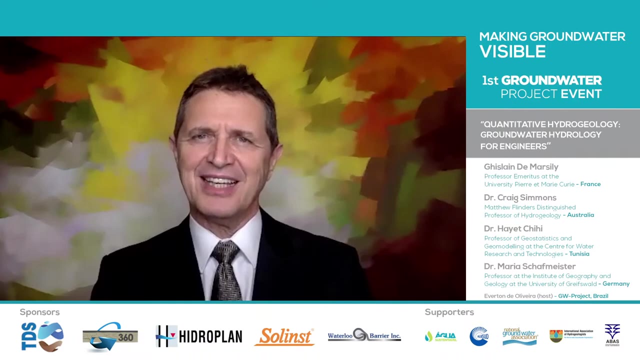 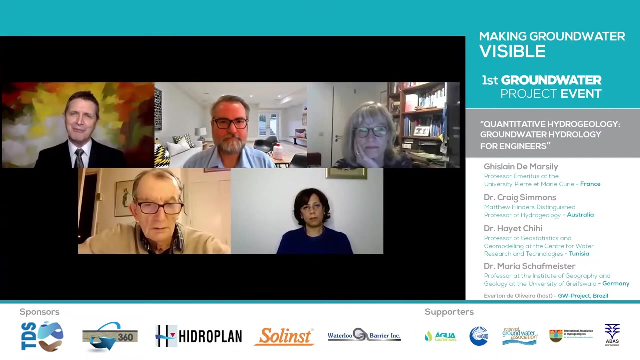 and you will have to write something there and you have to organize your, your, your thought before you talk, right? so what? what is your experience? because after today is easy saying that because you, you, you, you went through these classes so many times. it's all well organized, but i know you. you published a book on food production. 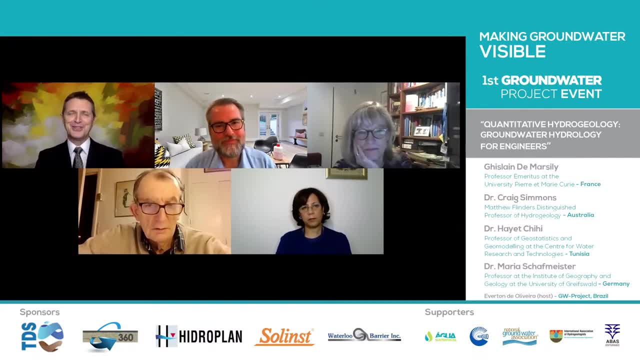 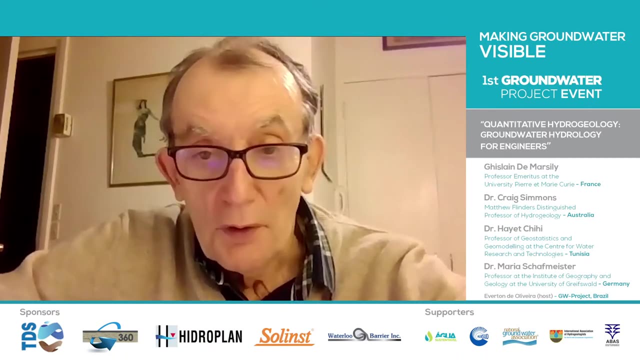 how would you teach something new using the blackboard? that's the point. i don't know if i can answer that question. it's a good question. i think, in fact, that you you had the right word. you need to have something organized in your mind, because before you can, 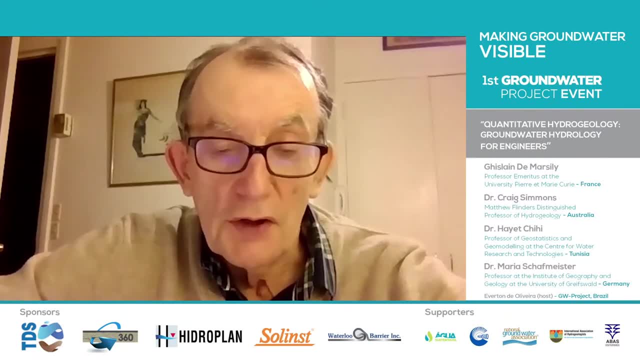 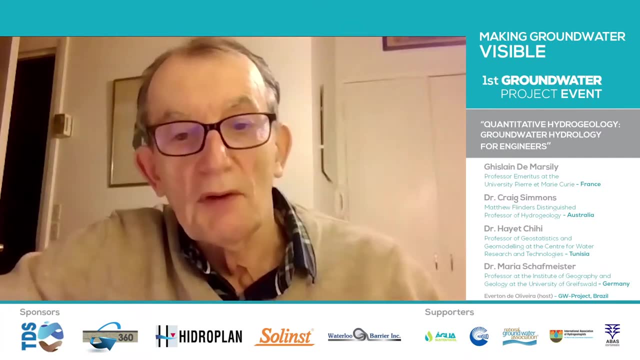 teach something, you have to tell the teacher what you want to teach, that you want to teach, and so, uh, if you're just teaching and putting words on a blackboard, on a white sheet, it doesn't matter. so you have to get organized on your, the order in which you want to present your stuff, and 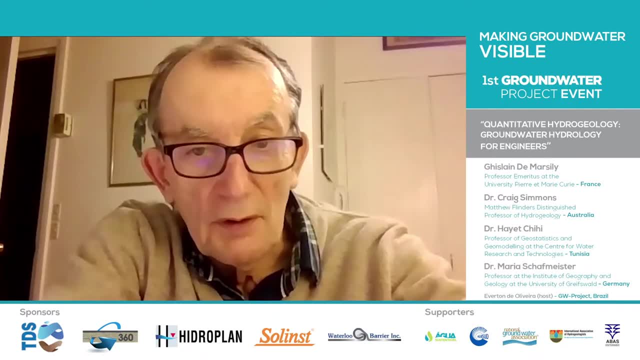 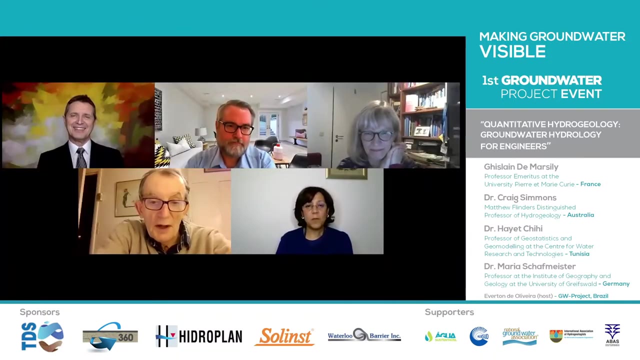 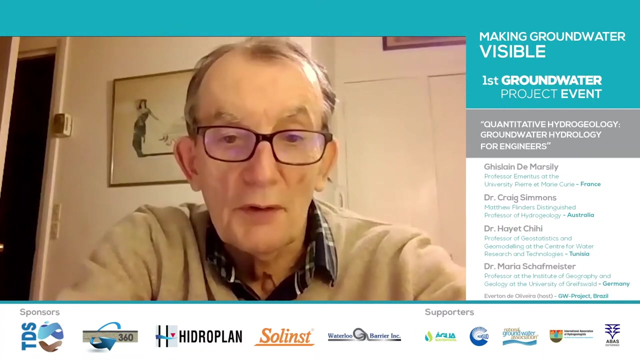 the links between the various stages and if this is significantly coherent and, uh, easy to understand. and i think you've done at least half of the work of preparing the course. organizing is the important matter, yes, And then you have also the help of the students who interrupt you or they ask you questions at the end of the course and they say: 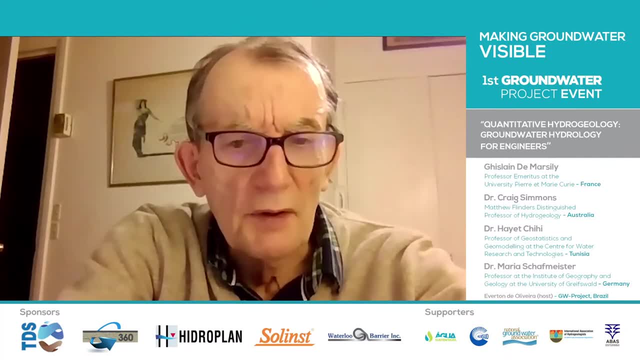 I didn't understand that. Can you explain again? Why did you say that This is wrong and so on and so forth? And it reminds me of a lovely Russian student which came to me from Vladivostok to learn hydrogeology in Paris. 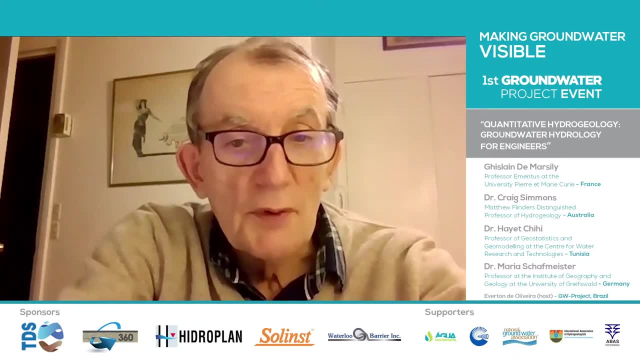 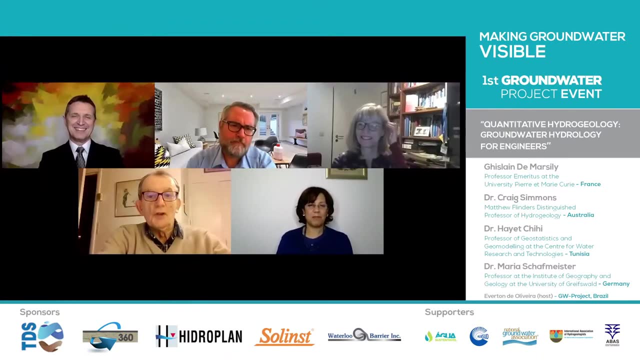 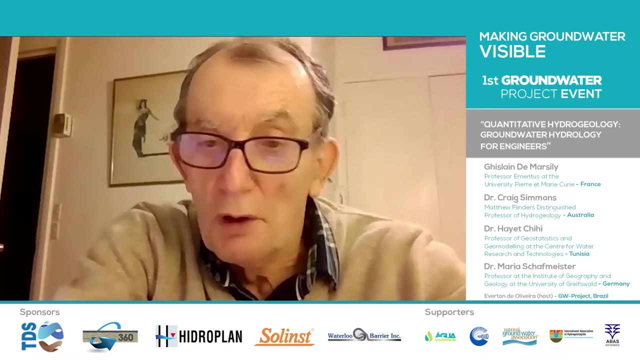 And she came to the class And she was absolutely shocked by the fact that the students were interrupting me during the class And she said: you should not never interrupt a professor when he lectures, And this is something that for the Russian culture. 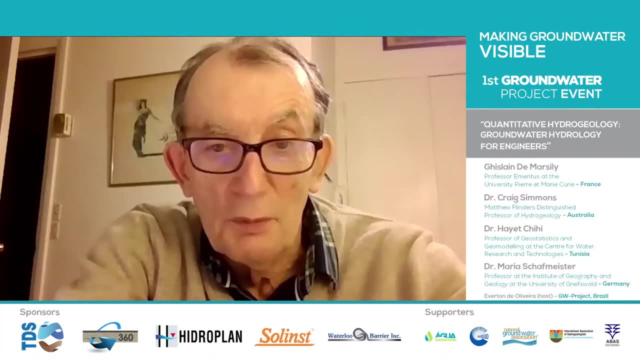 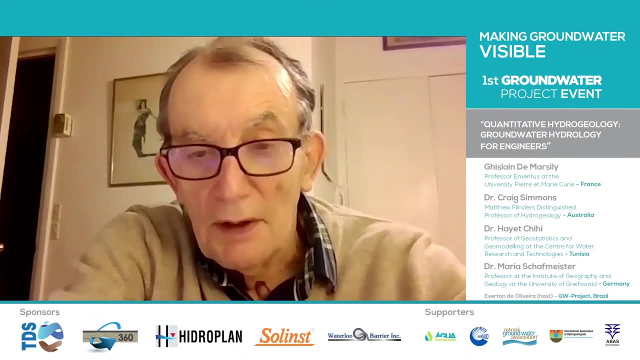 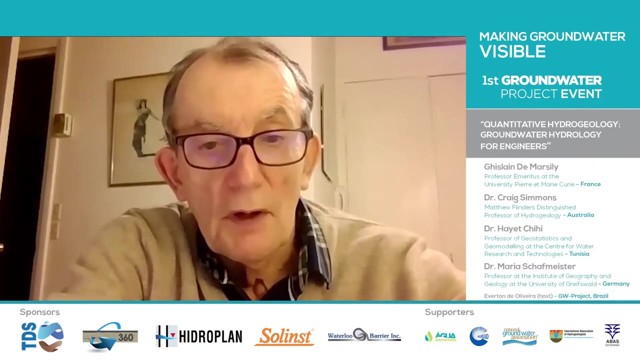 it was unacceptable And, on the contrary, I like that. I like to be interrupted and to have the students comment and ask questions, Not that they prevent you to speak, but at least to clarify questions and so on. And I think you have a lot of improvement of your teaching if you have good students or poor students. 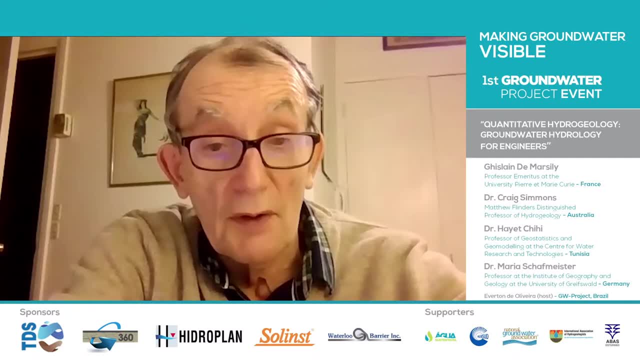 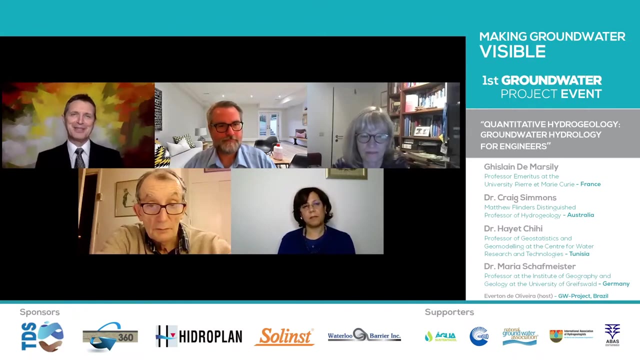 It doesn't need to be good students. Even poor students can ask very nice questions and very important questions. So I think the interaction with the students is something important In the class. I totally agree with you Totally, Which is not happening today, with the pandemic working on computers. 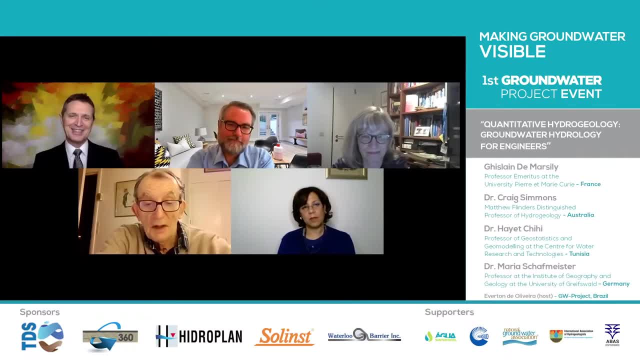 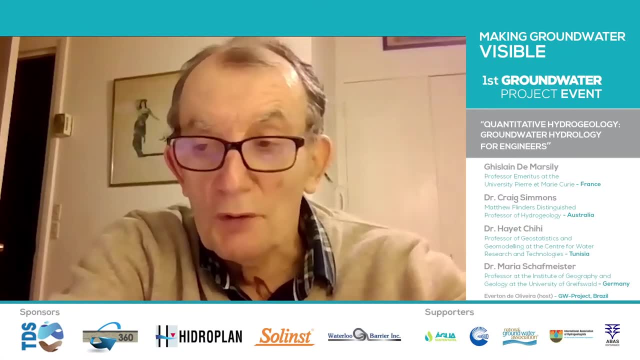 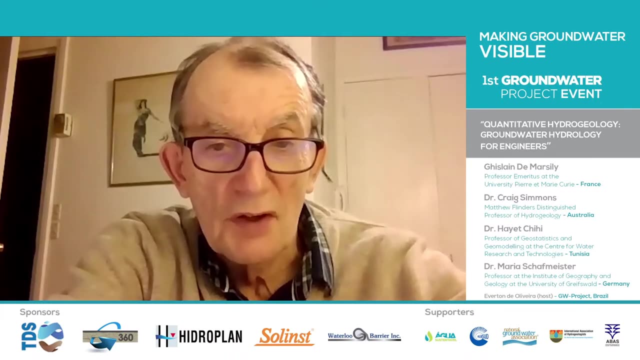 You don't see the students right, And then they rarely ask questions Yes and no, because we interact. We are miles and thousands of miles away from each other, Not just for the coronavirus but partly for that, And we managed to interact and we managed to have an exchange and so on. 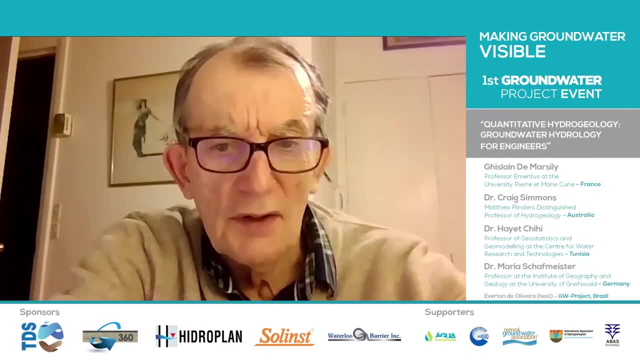 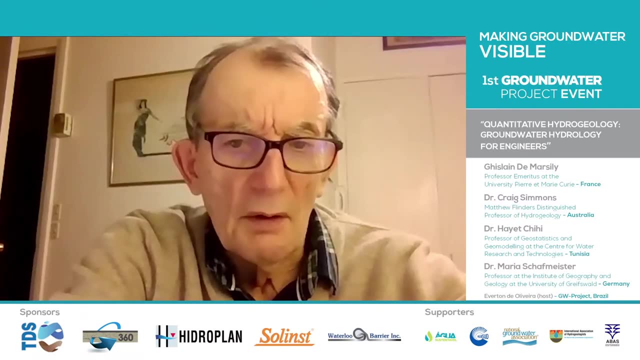 So I think we have to learn how to exchange, How to exchange ideas and to communicate with these new tools like Zoom and any of those softwares which help propagate ideas. I think it's something we have to develop and learn how to use. Yes, that's true, That's true. 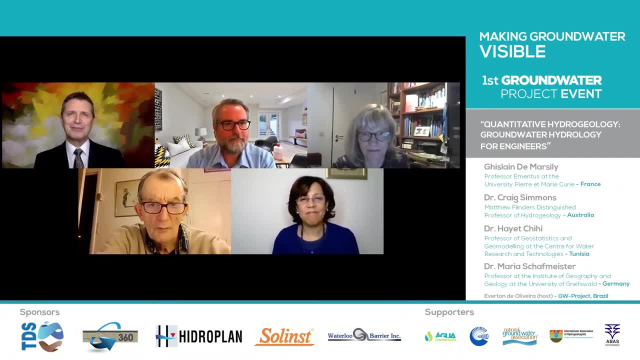 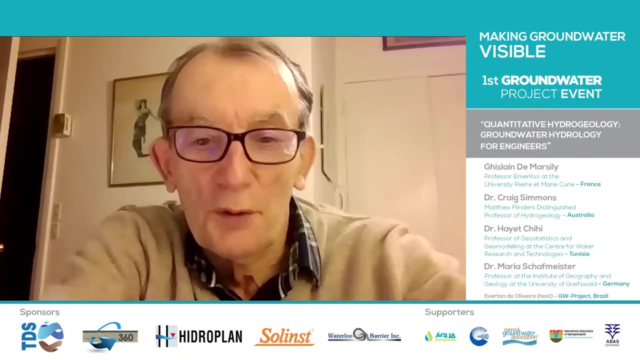 Well, guys, the conversation is so good, But we have a limited time to talk. To talk here, I'd like to. Yes, You're the boss here. You can say that. No, If you're going to conclude, I'd like first to thank all the participants, Hayet, Maria and Craig. 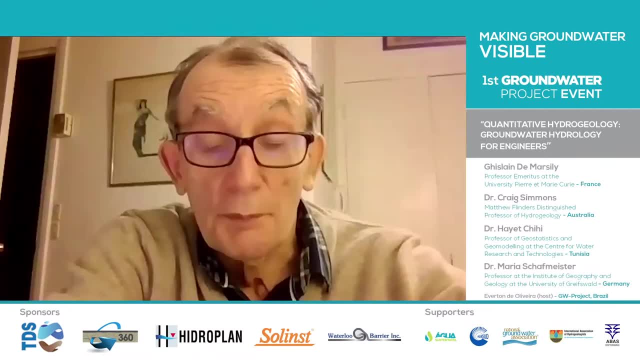 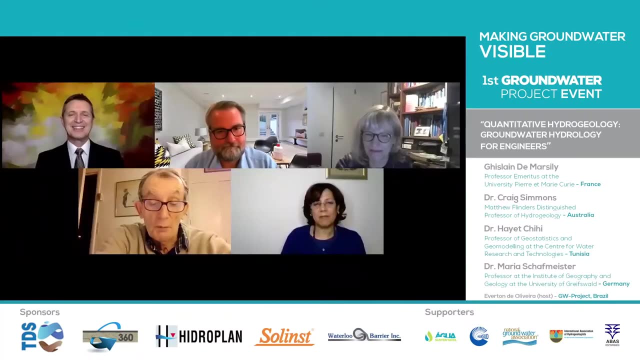 And the staff from the groundwater project who helped organize this meeting, And thank you for all what you've prepared, all what you've said, all the examples you gave, And I'm afraid we talked too much about me, But I think those colleagues and friends did a very good job. 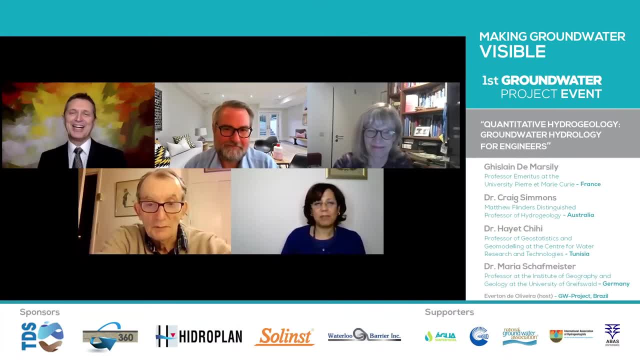 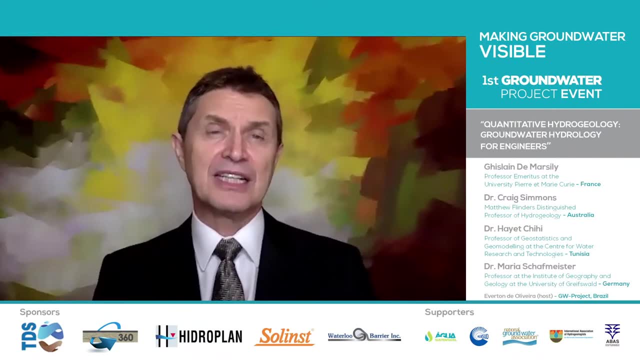 And I thank them very much. No, that's okay. That's okay. I'll give some time for your final statement. Just a moment, I'd like to ask you guys and ask you one final question. We're working on the groundwater project. 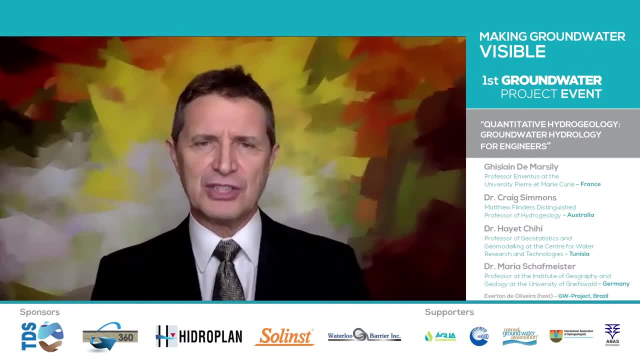 And our idea, as I mentioned at the very beginning, is to spread knowledge. One of the things is that we are now speaking in English And language. it's a tough barrier for students. We want to do the books that we are preparing. 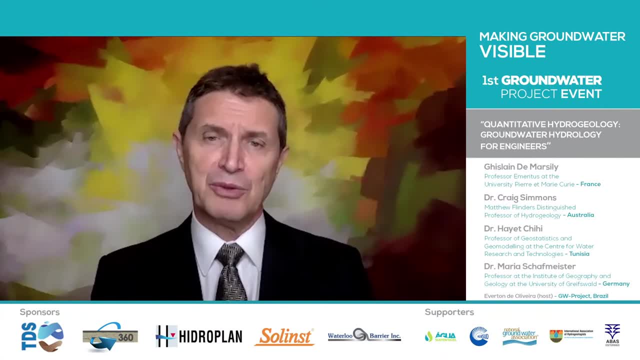 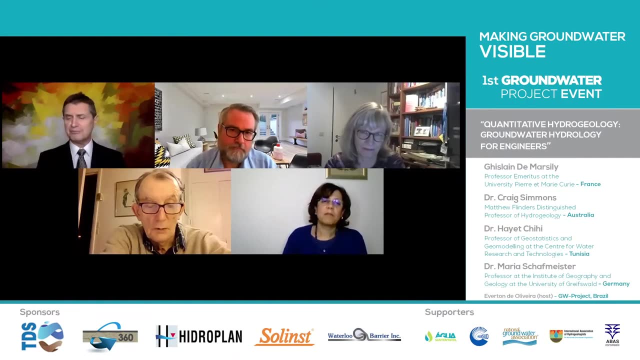 First, we are preparing books in English, But we want them to be translated. Translated into French as well, Not only into you know Portuguese, Any language People say that you know. all people that speak French can read English. 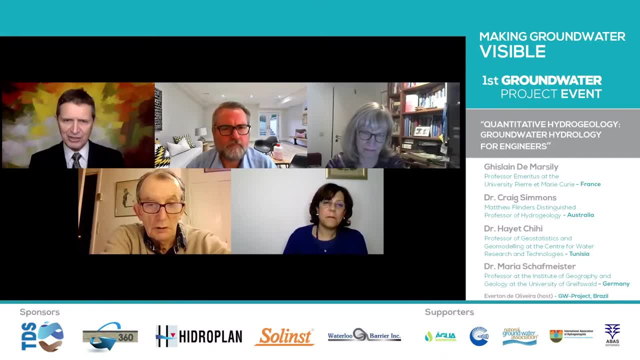 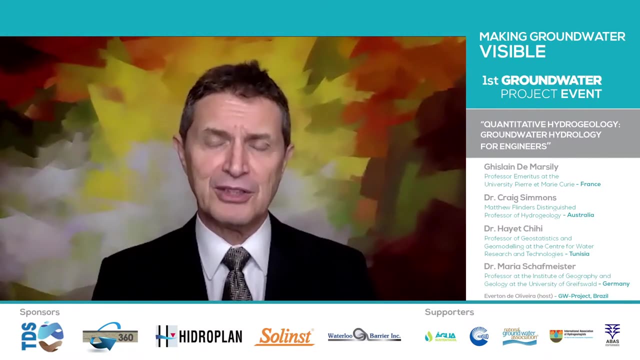 And we know that this is not true. This is not true for any language, Not for you, Not for French, For any language, Right? So we would like to have people helping translating books. So I would like you to say something for us about the importance of distributing knowledge for free. 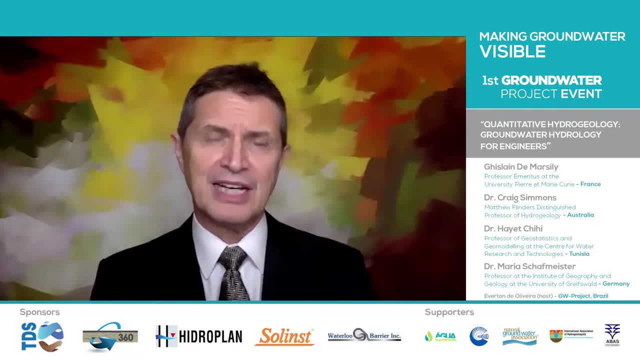 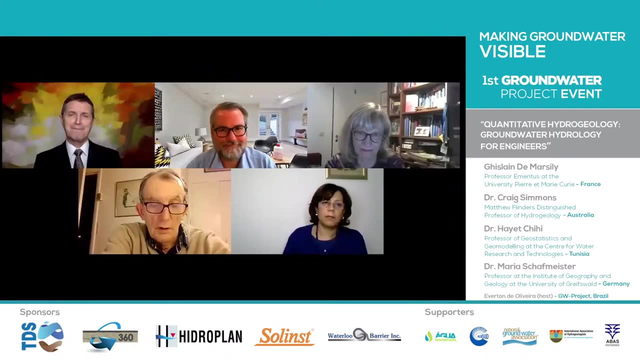 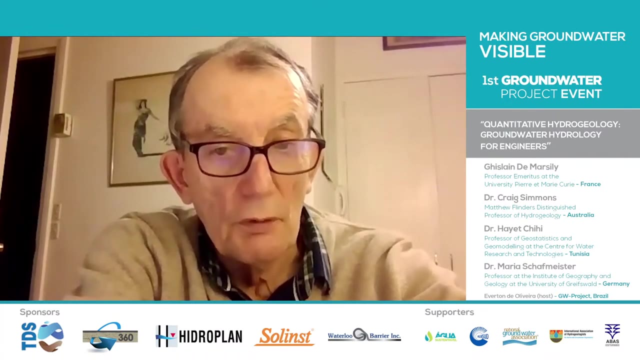 And the importance of distributing knowledge in your life, as an example for other people who are producing books to the groundwater project, Please- No, that's a good point. I think you need written material. You need written material to really learn, Because you can follow a lecture. 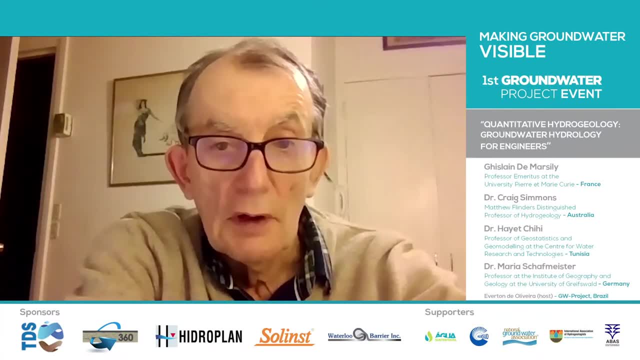 But then you have to go back and read something and confirm what you have heard And put that into words. Now the problem of the difference in languages- French, English or Portuguese or whatever Spanish I think- is going in a few years to fade away. 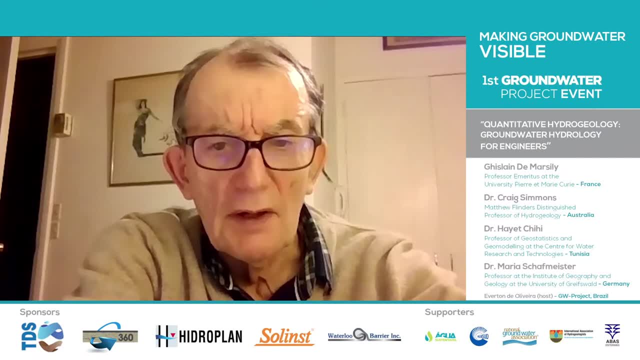 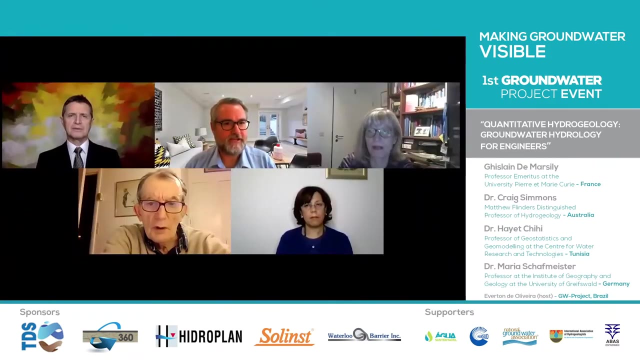 Because automatic translation is becoming increasingly correct, It's becoming increasingly good, And I have used a software- It's not the Google- to translate, which is not very good, But I forgot the name of the software: DeepL. I think you learned. 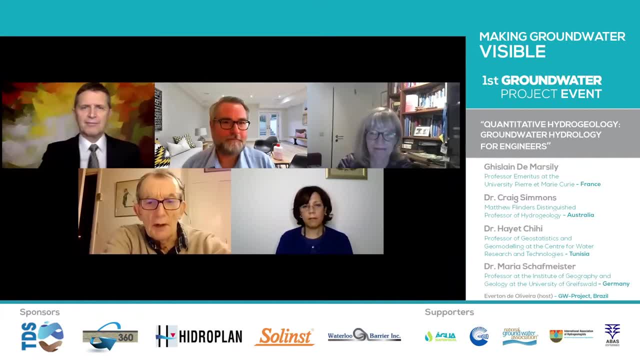 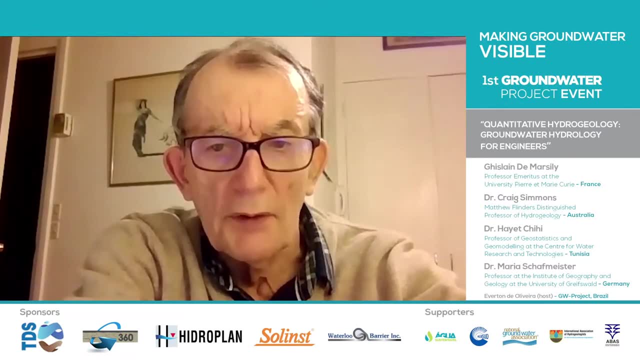 DeepL, DeepL, DeepL, yes, DeepL. There may be others, But DeepL is really very good And of course, you cannot always rely on it. You have to read and check that every page doesn't contain a mistake. 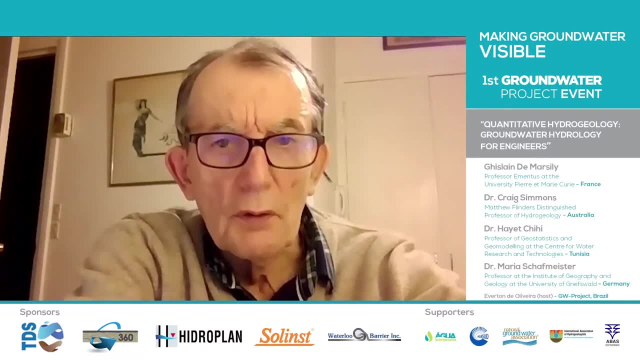 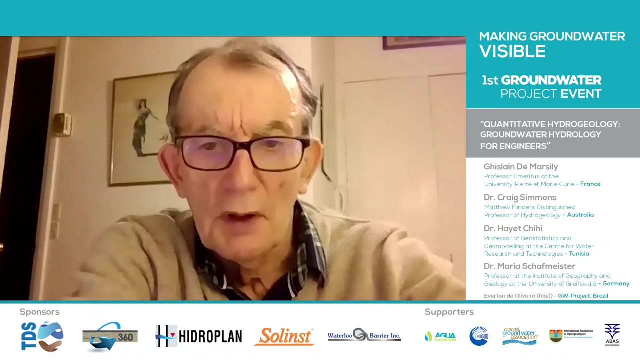 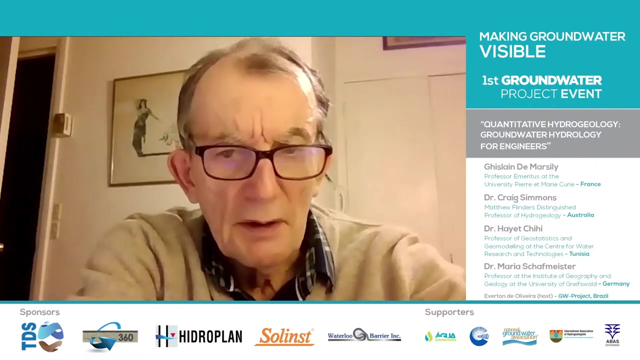 It's so good and so true to the meaning that really it's impressed me And I think in maybe 10, 20 years, speaking in French and being automatically translated into English, as you talk, is going to be possible And books will be translated at no cost and very little cost and very high speed. 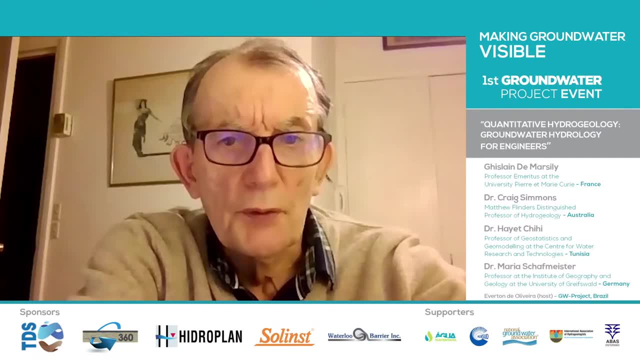 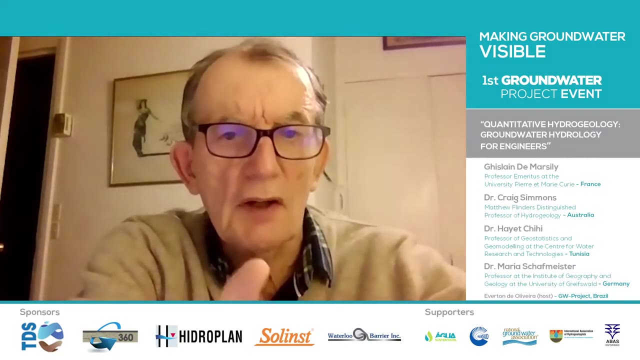 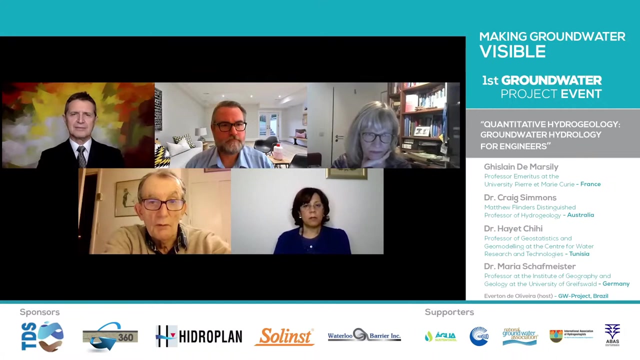 So I think you're absolutely right. It should be put this written material in common, But I think it's better to translate than to hope that students or colleagues will learn French, English, German, Portuguese, Spanish and whatnot, and Chinese and any of these Asian languages that we need to be aware of. 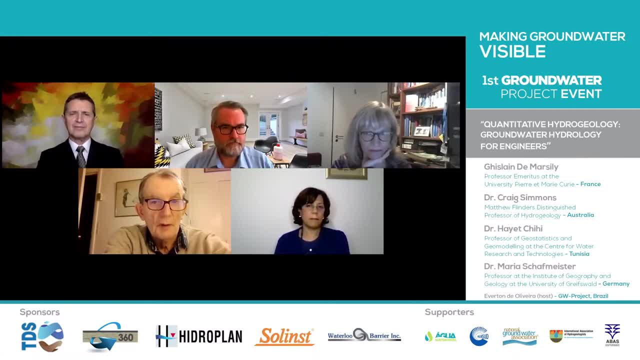 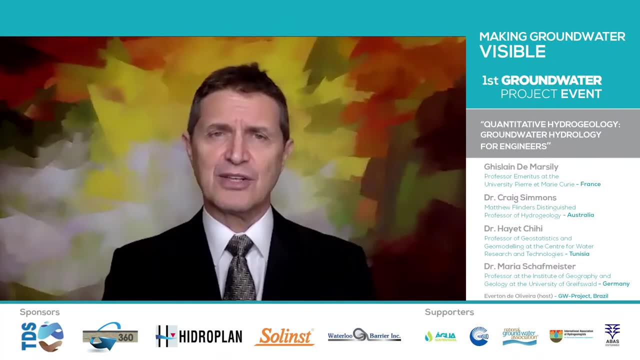 But I think that's a problem that will be solved Well, I agree. So just let me add something. It's my understanding, just like you, that the software will improve fast. But translating science it's a bit harder because of the jargon. 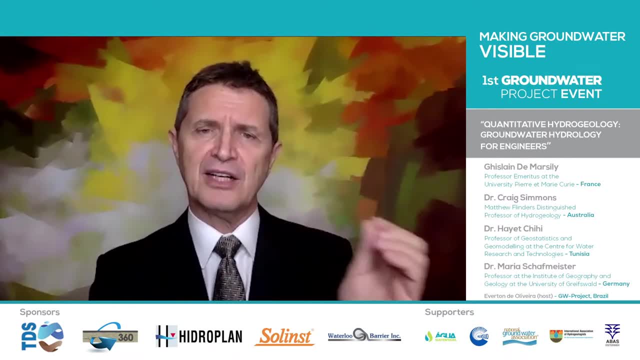 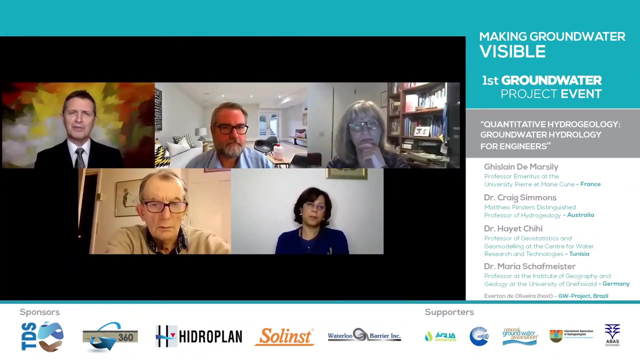 So if we have more people translating our books, that could be used for artificial intelligence later to help improving the translations to our field of knowledge. That's an improvement that we could add by using the groundwater project Translations into different languages. That's our aim. 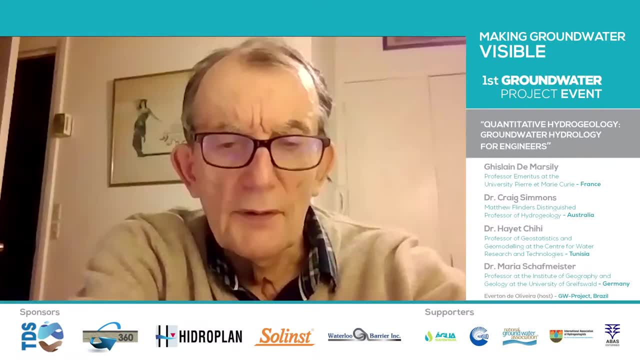 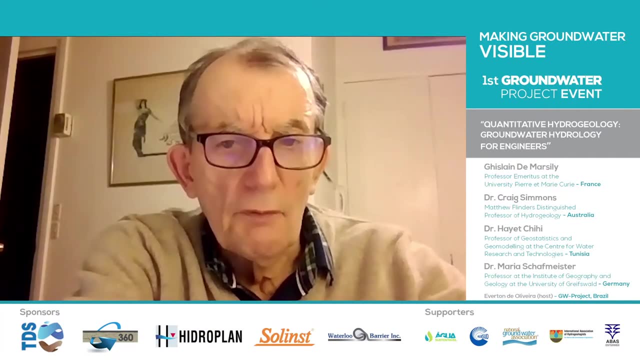 Yeah, I agree. I mean these new softwares that translate so well. they are based in studying text in English and in French and text in other languages And to compare them and to determine how do you translate this expression and not words by words, the expression and the meaning. 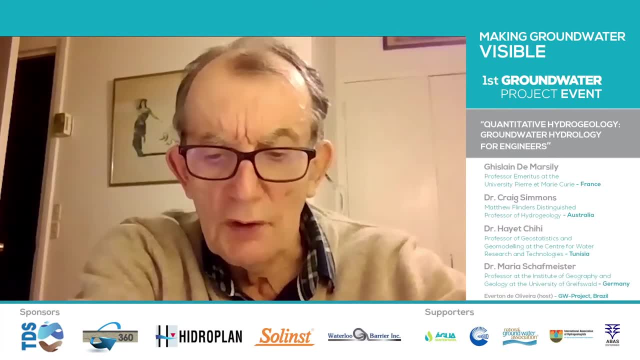 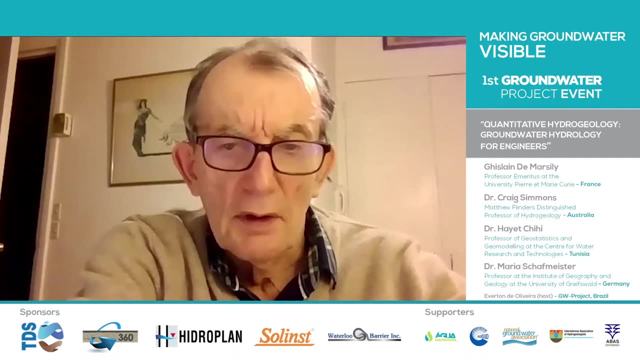 So I think artificial intelligence is really beautiful, a beautiful tool to help translate, including all the details and the theory behind it. So I have good hopes that this will be easily available in a few years. Well, I hope so, I hope so. 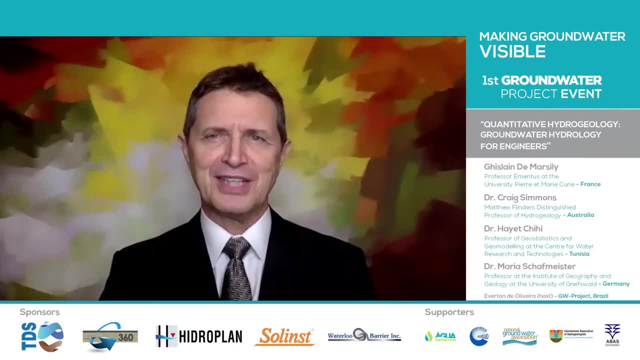 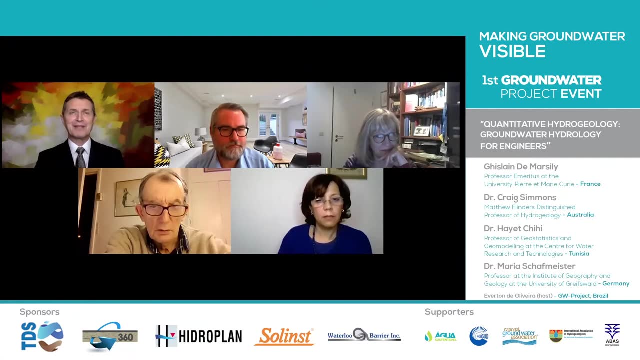 I'm pretty sure it's going to help, but I'm not sure how long it's going to take, but it's going fast. So, guys, could you please add something about that? And before I think our time is up, now could you please make your final statement and we leave Guylaine for the last word, please? 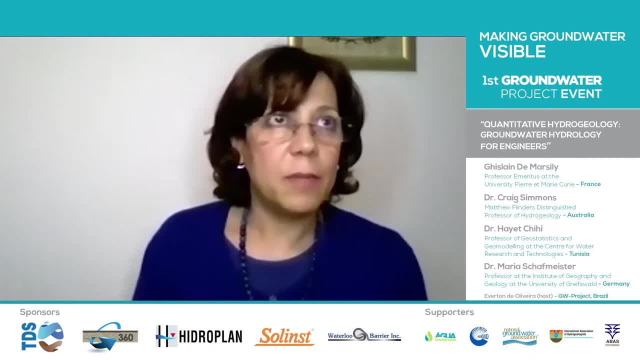 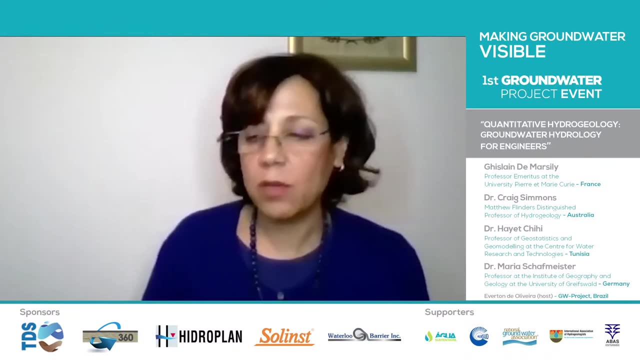 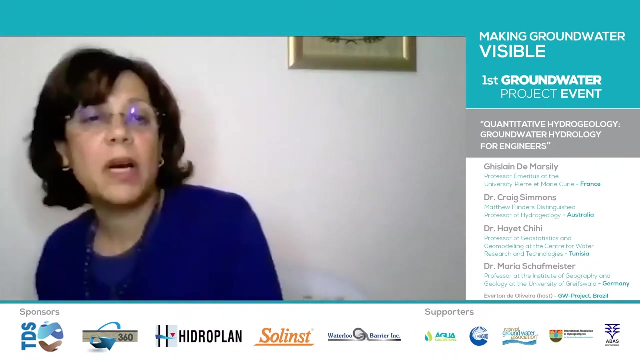 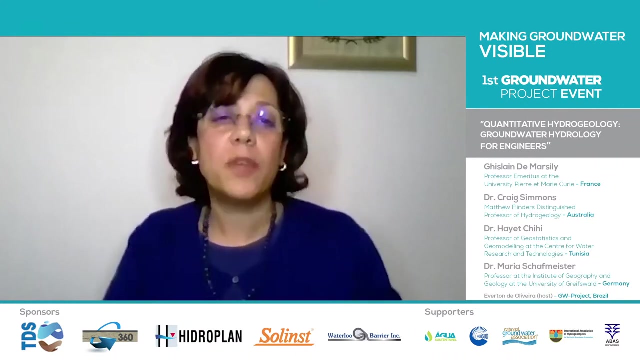 I think about writing books introducing geological properties, physical properties, Heterogeneity in general was nicely represented in journals, in books, in petroleum models, But in hydrogeological and aquifer modeling it's not. there's not too much text writing adapting or transforming geological properties in mathematical equations. 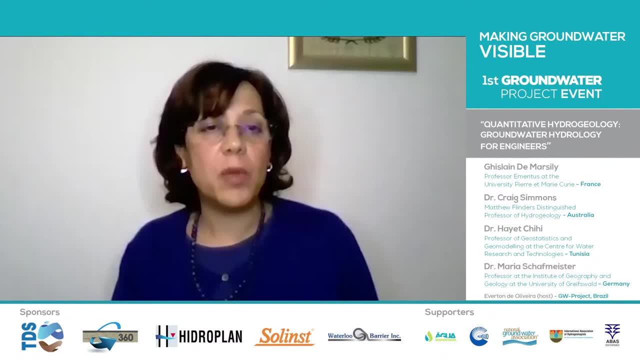 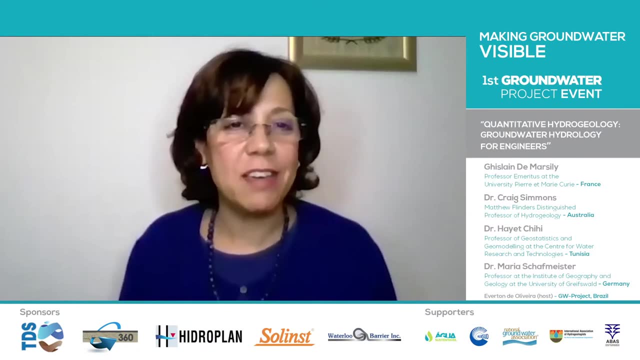 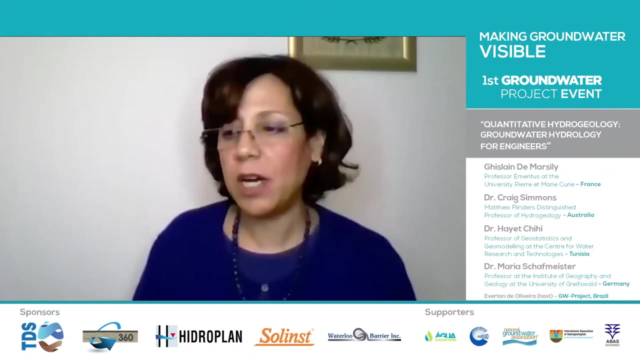 I think that we have to write papers and books on that, Concerning how to teach using blackboard. Blackboard or PowerPoint or paper for illustrations. I think that we have to use all of them. For example, PowerPoint was an aid for us to continue studying and teaching, et cetera. 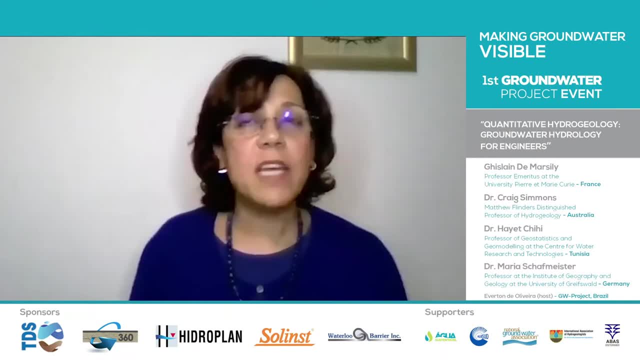 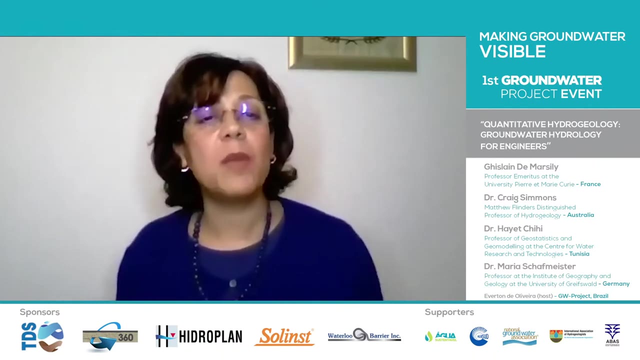 But it's not the same happiness when you are transmitting the message. It is like playing football with the PlayStation or on grass Right. I think it's not the same thing. Concerning the blackboard, I think that we have to subdivide it into parts. 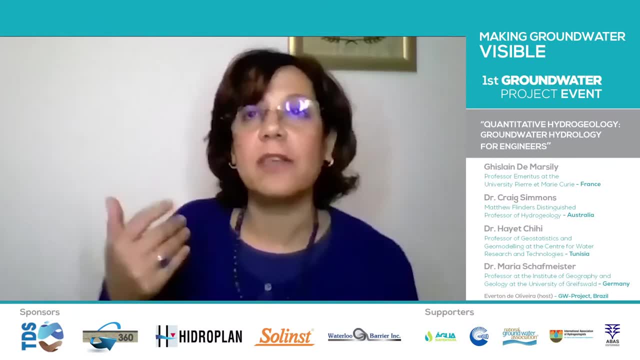 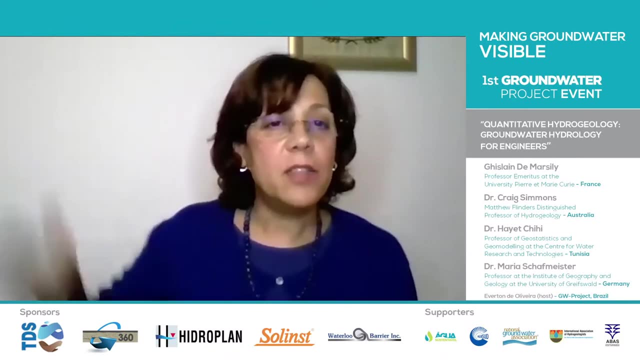 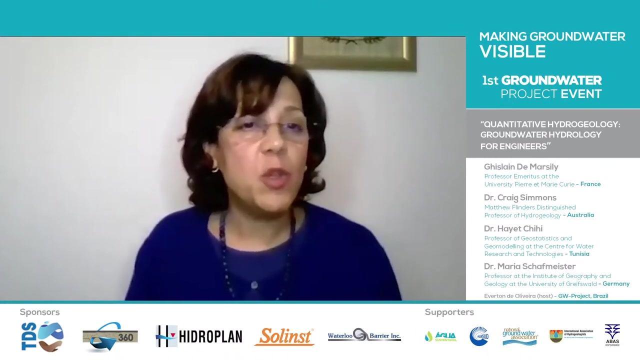 One part to present the lesson as we have organized it in our mind, in logical thinking, And a part for the question coming from students and to think together on the question that comes from them, To encourage them discussing, Because if you will reorganize your, it helps us to reorganize our lesson for the next time. 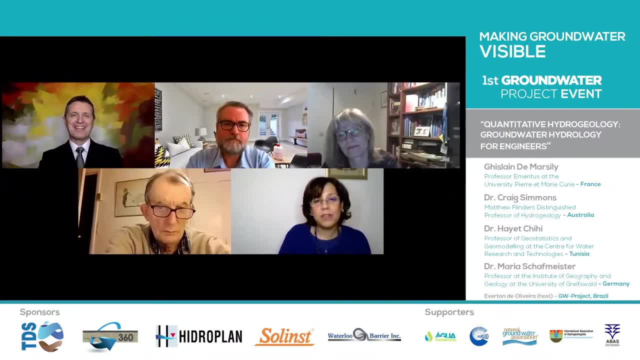 I would like to thank Professor Domarsili Craig and Maria for this nice discussion, And I would like also to thank you, Everson, And all of the Groundwater Project team for organizing this international event. Thank you for inviting us. 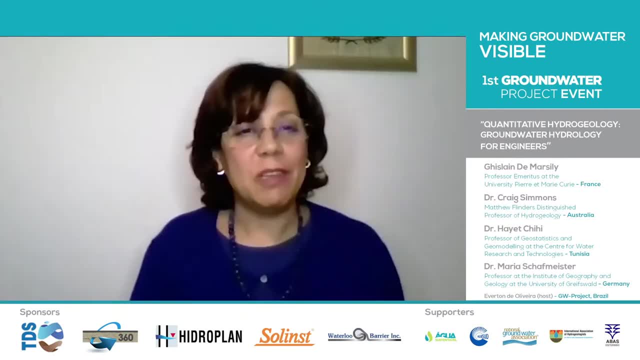 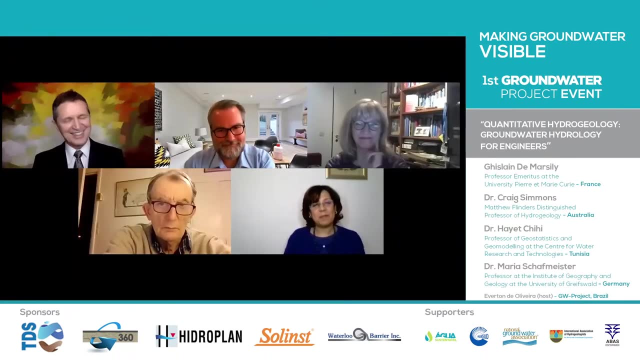 And let's continue doing conversations and writing books and papers. Thank you, Thank you very much. You won't get rid of me that easily. I'll be after you soon, Don't worry. Thank you very much. Thank you for your help. 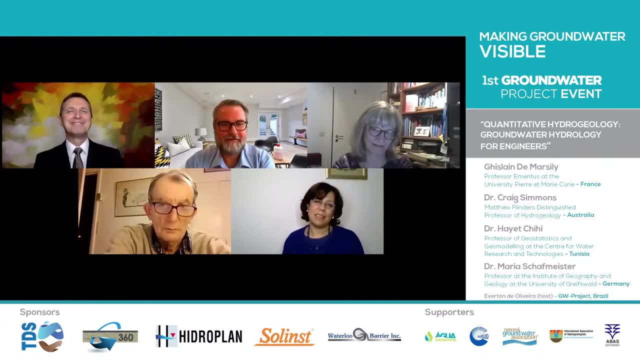 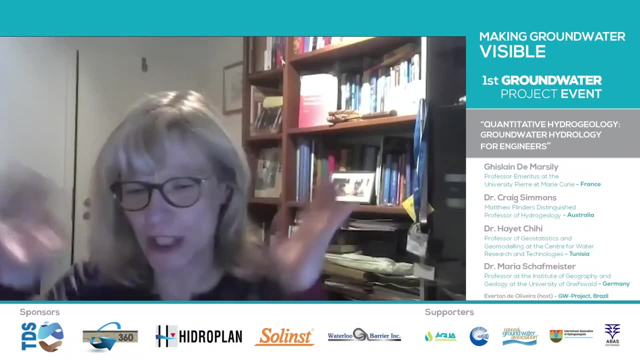 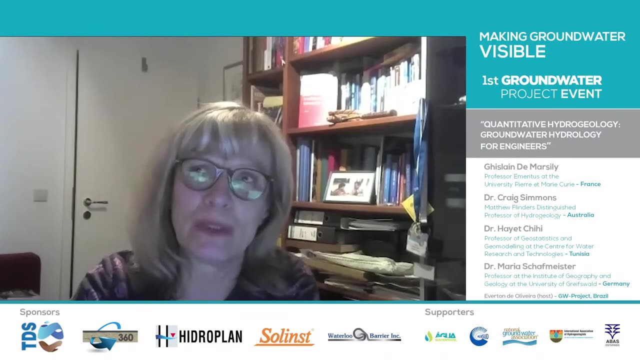 You helped us very much, Please, Maria. I think I make it short What we need, whether in quantitative hydrogeology, geology, engineering or philosophy, we always need teachers who are inspiring and who are able to explain complicated things easily. 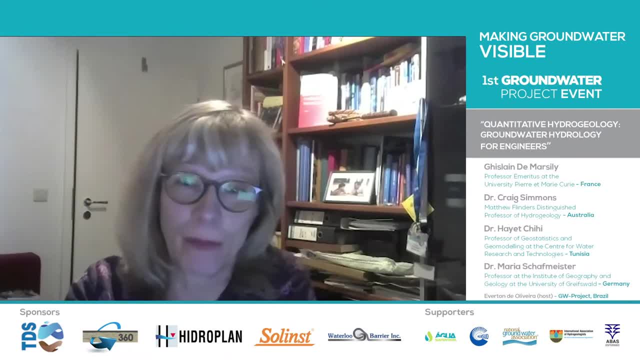 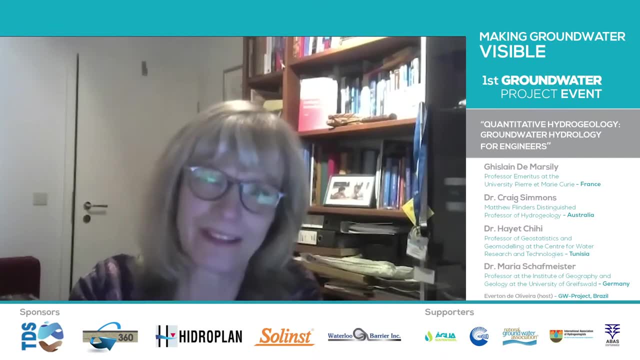 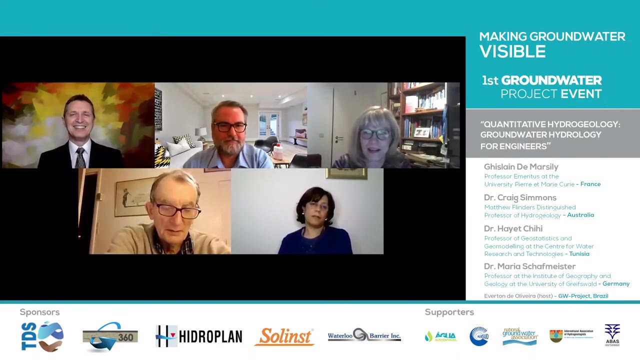 And in this Guylaine, you are for me really the master And I always try to do it like you. Of course I don't, But I try And I really thank you for being as you are and that I was able to learn from you and with you. 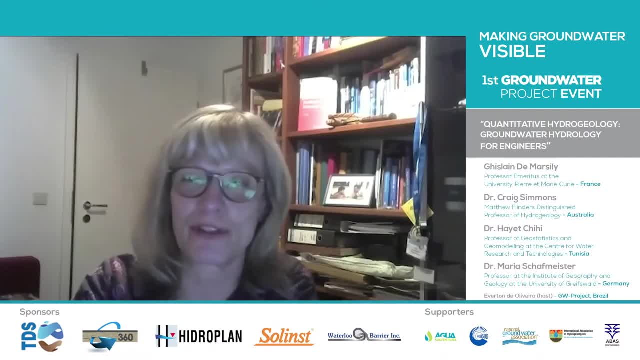 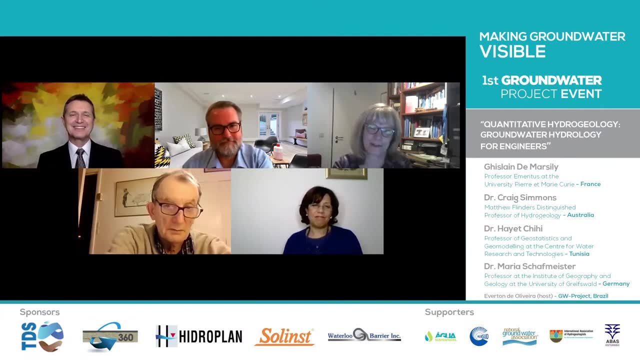 Yeah, that's my famous last words here And of course I want to thank everybody And Hayat and Craig- So good to meet you again And, of course, to see you again in good shape. Guylaine is also a pleasure for me. 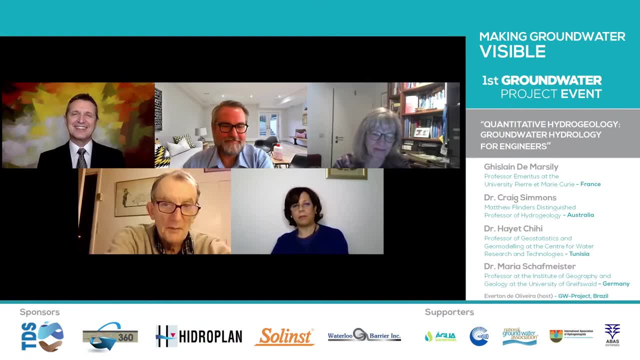 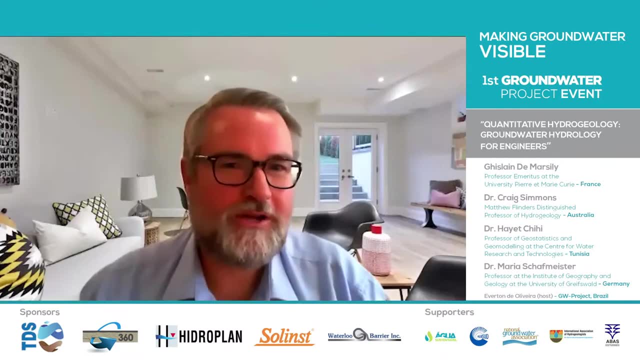 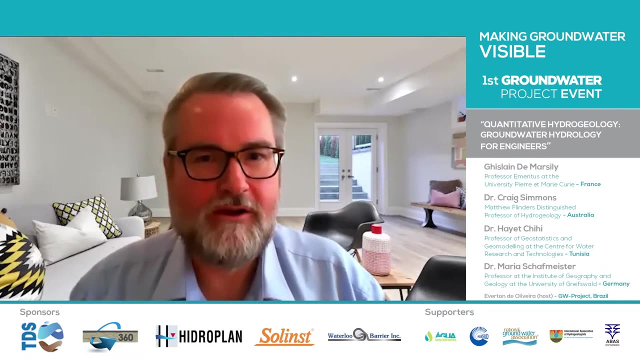 Thank you everybody, Thank you to the team, Thank you very much, Very kind, Very kind. Craig, Craig, you please Look. I think it's impossible to predict the future with any great level of precision, But I think we know one thing for sure about groundwater: 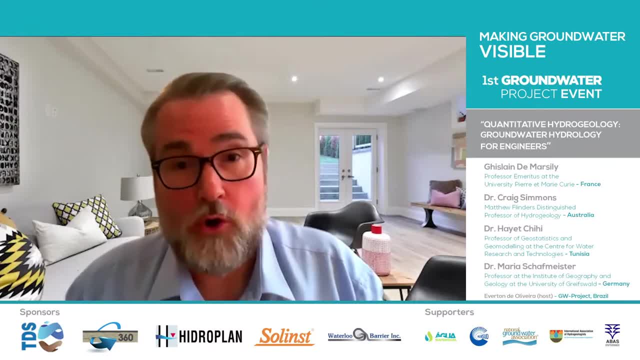 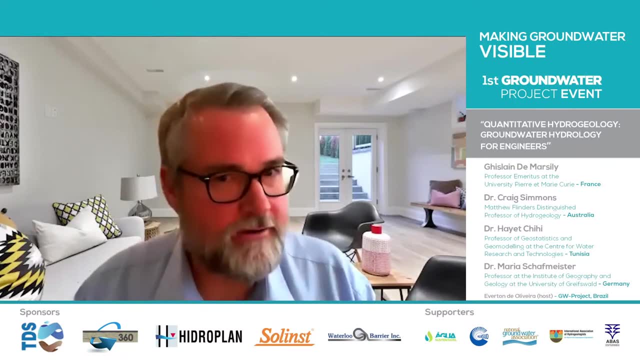 And that is that the number of problems that we're grappling with now already significant, as I mentioned, from water supply and security, scarcity, coal, seam gas, fracking, food production, energy. There's a huge number of those issues, But climate change, population growth will only exacerbate pressure on all of our natural resources, including water resources and groundwater resources. 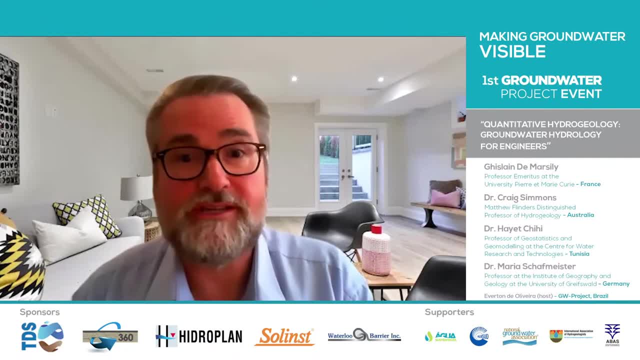 So groundwater is here to stay, if not to grow, and its significance and its importance, And I think science and research is one part of that, But I think management and policy and governance is also crucial And getting all of these interacting, you know well, is crucial. 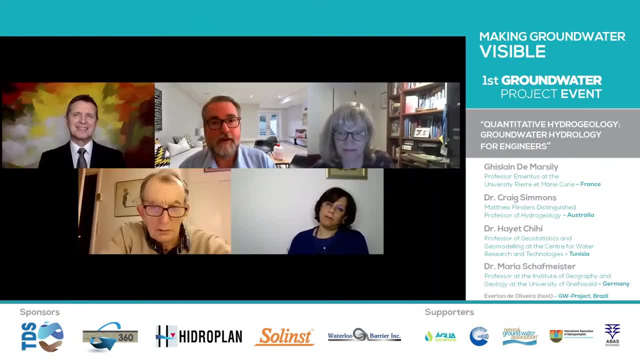 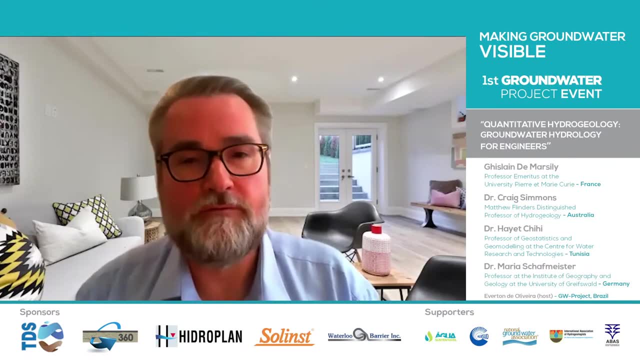 And education and capacity building And all of those things. So training, teaching and textbooks are a huge part of the issue there. Getting research out into the public domain And so People use it needs education and training. So textbooks, books, the groundwater project are playing a crucial role. 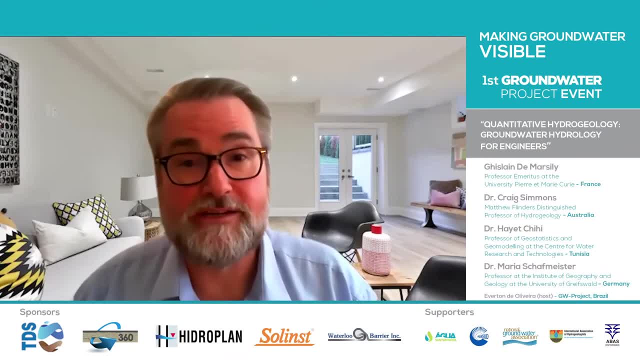 And, clearly, translation and accessibility are a huge part of that. So I think all of these initiatives are important And, again, as everyone here today has said, it's been a great discussion, An honor to be involved in today. Thank you for the invitation. 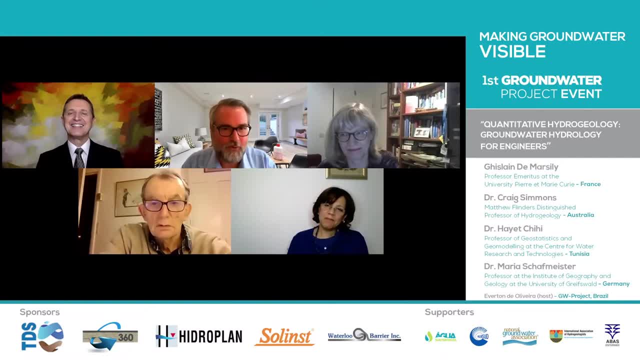 And I look forward to working with you. no one work with you, Gilan, So look forward to many more years. Thank you very much, Gilan. your final statement, please. I know you, It's your second final statement, please. 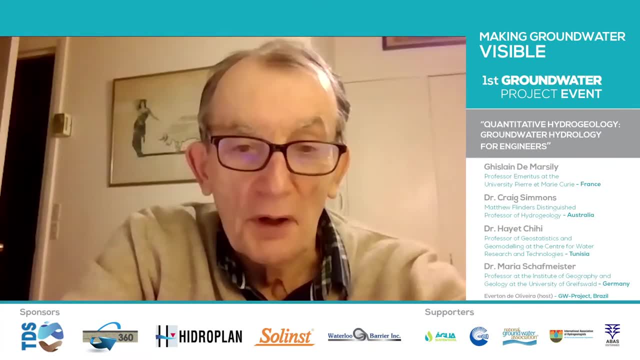 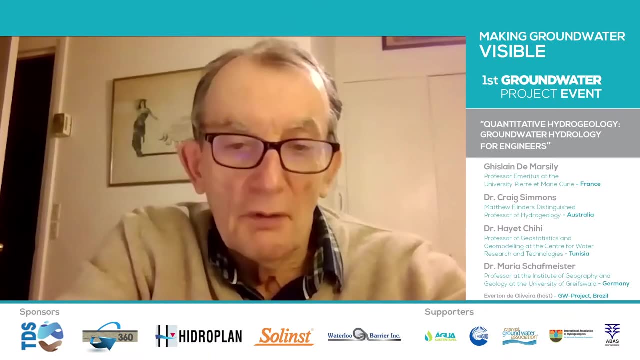 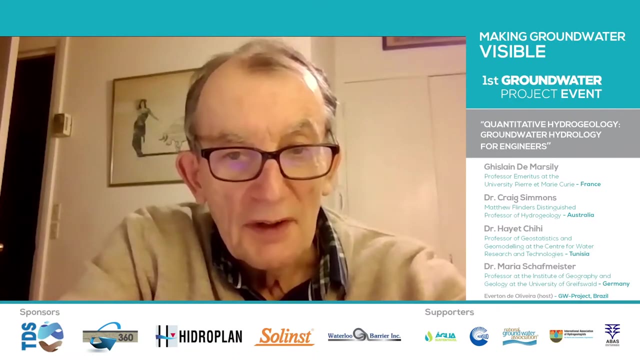 What I'd like to say is that I didn't know anything about groundwater hydrology when I started learning at school, And slowly I developed the understanding of hydrology in the underground, And I think the reward I had to study this topic is at least two times. 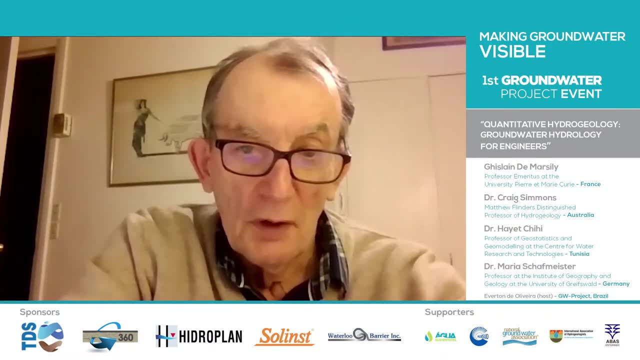 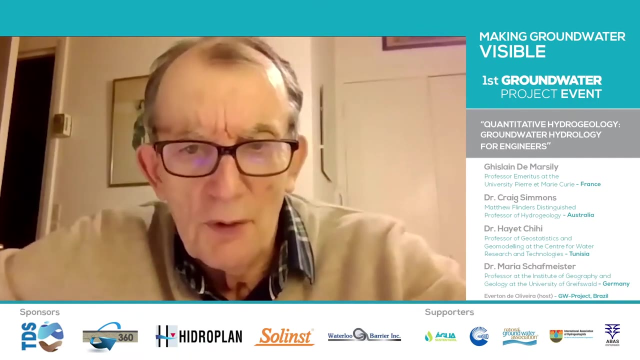 First, I met a large number of good colleagues, of people who were interested in the same topic, and we became friends. So it's an area where people work together, exchange ideas and they don't hide what they found in the cupboard. So it's an area where there's a lot of exchange. 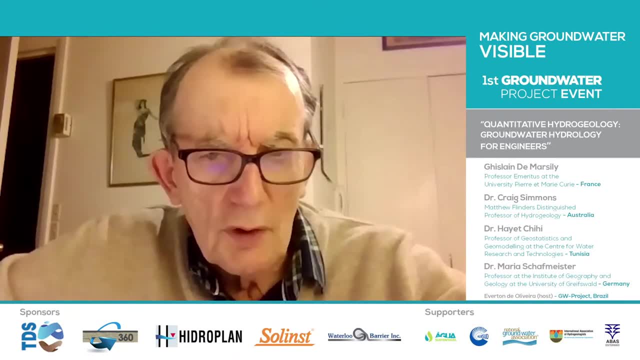 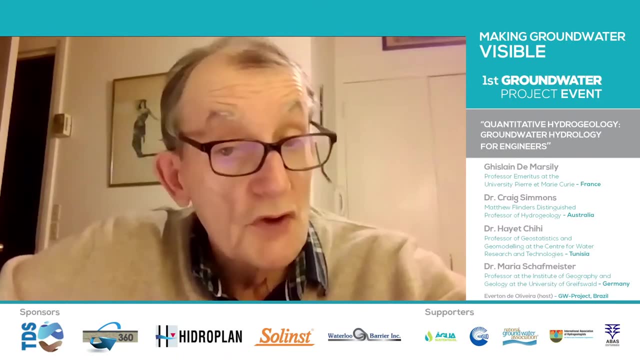 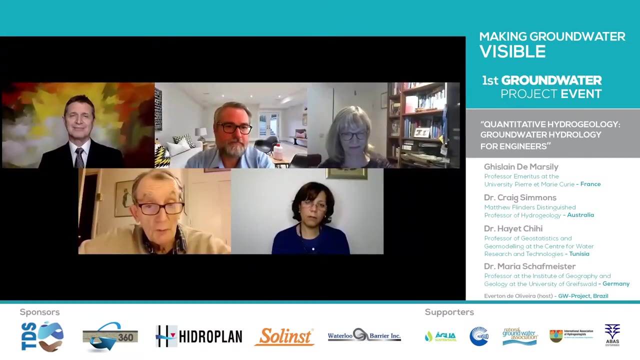 There's a lot of exchange between the researchers and the professors and the students, So it's a very lively atmosphere to study a topic which is difficult Because groundwater hydrology and quantitative hydrogeology is not easy. It has a lot of peculiarities and uncertainties and equations and whatnot. 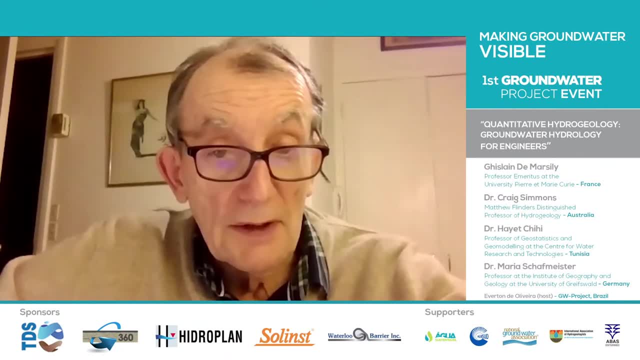 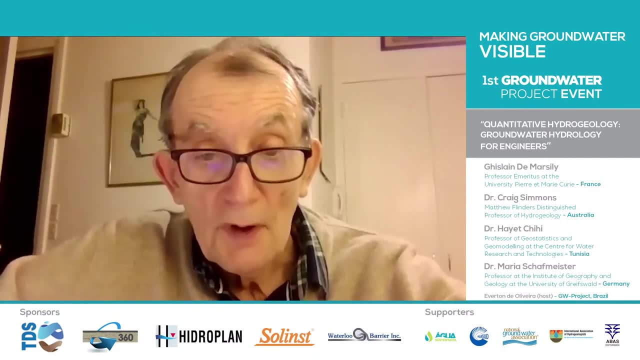 So it's a very- at least scientifically- deep problem to work on, And the last point I want to make is that it's also an area where there are very significant human problems, or society's problem: Water resources, water pollution, energy storage, whatnot? 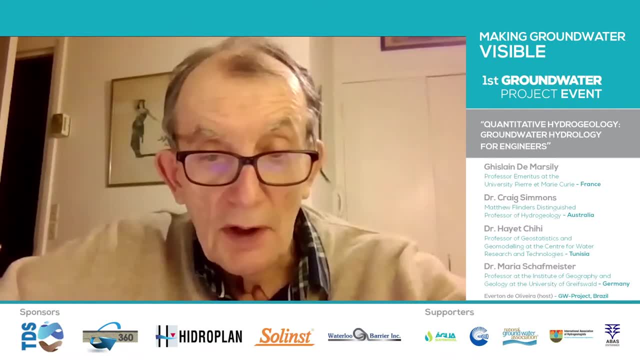 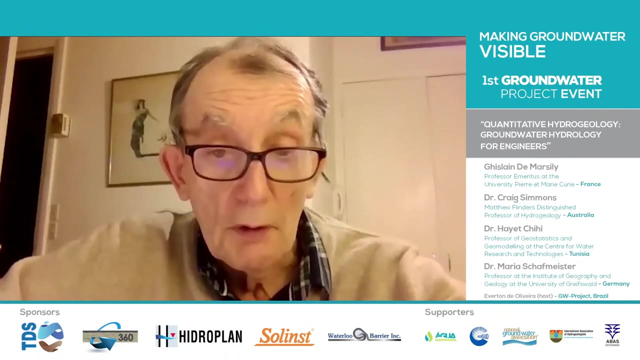 So there are many instances where hydrogeologists trained in quantitative hydrogeology are needed to help society. So it's an area where you can think, Think, Think that you can help solving problems, applied problems, real problems from the world in different countries, and help here from what you've learned there. 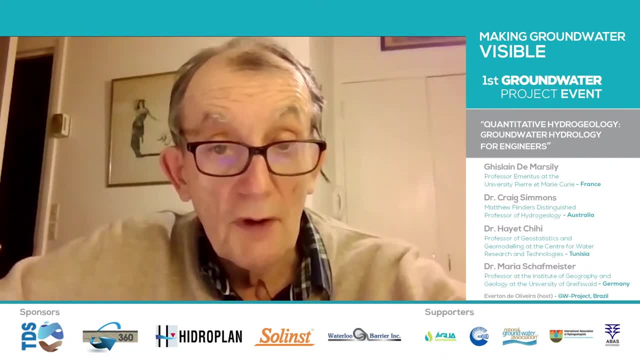 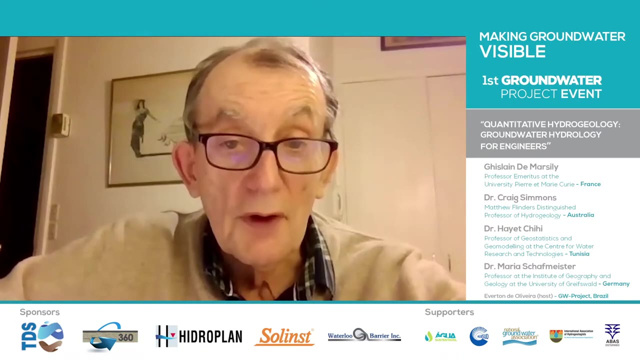 It's something where you exchange, So it's a very fascinating job, And I recommend students who have not yet selected what side or area of geology they want to learn To learn or to work on To consider hydrogeology as one of the most fascinating facets of geology. 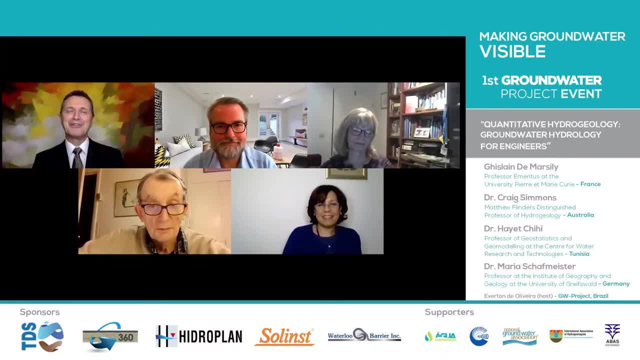 Thank you very much. Very good words. Thank you everyone. That was a very, very entertaining and very instructive session for me And, I hope, for all the audience here. It was a pleasure and an honor having you with us, Guylain. 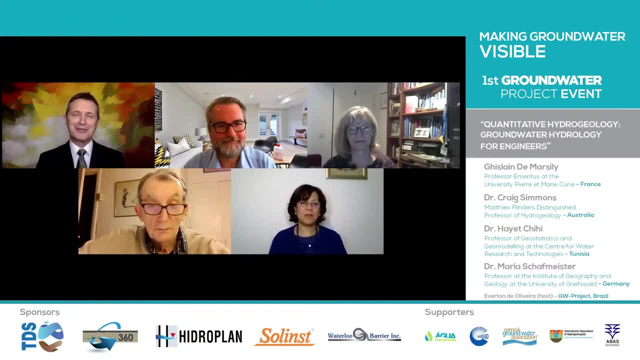 And I hope to see you soon, Thank you. Thank you for your participation in the groundwater project And we'll get together and we hope we can help us spread the knowledge of groundwater better than you do, which is hard because you're doing quite well. 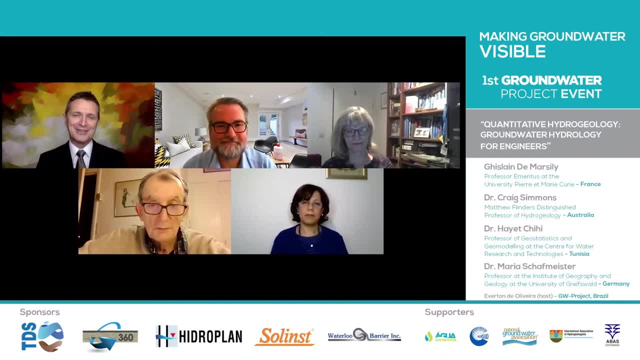 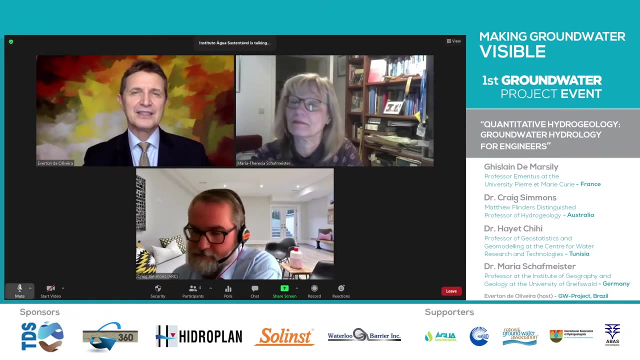 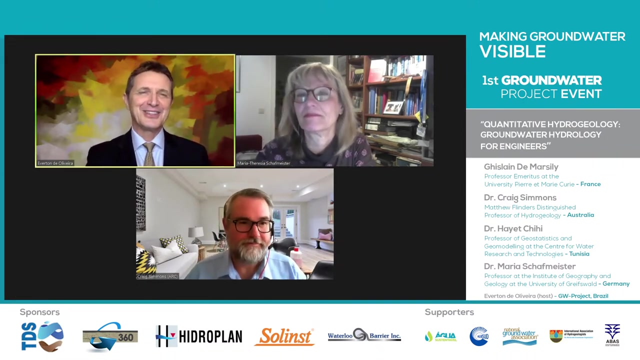 Right, So we're looking forward to have your help for us. Okay, Thank you guys. Thank you very much. It was very nice having you together with us. Bye, Goodbye, Okay, Thank you. Thank you for our talk with Guylain de Marseille. 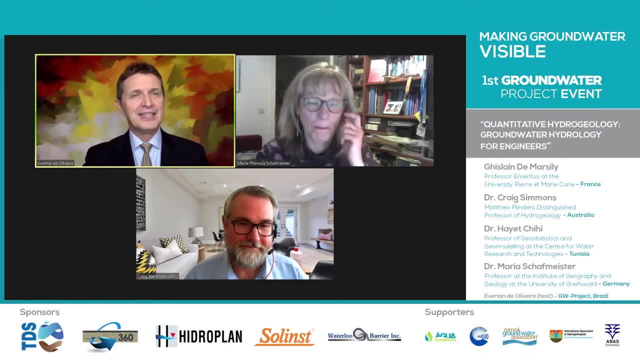 We have to excuse all of you because Guylain cannot make it for the question and answer session, But we have the kind participation of Maria and Craig. They are here to help us and to offer us, offer us a little bit of our knowledge. 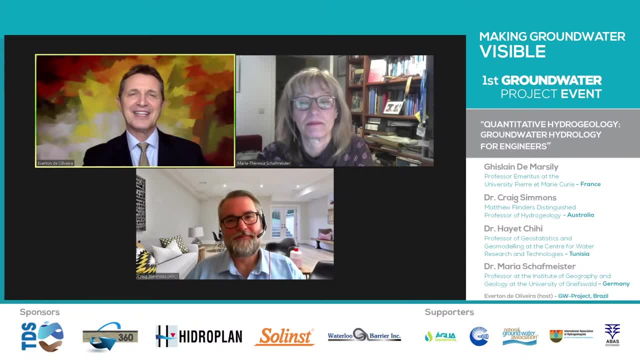 and understanding of Guillaume's work. Thank you, Maria, Thank you Craig And everyone. thank you. So, from there, I'll have a few questions here. Let me do this. There's a question here to all of you. 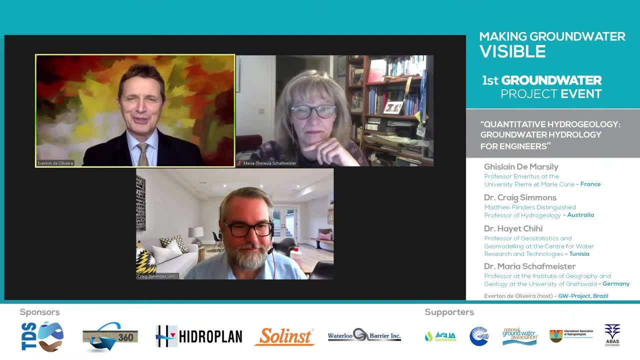 And since you know his book, it's better asking for it. The books bring the fingerprint of their authors on them. What do you believe are Guillaume's fingerprints on his book? Was it his style, his thinking? What was it? Maria, do you want to have a first crack at that? 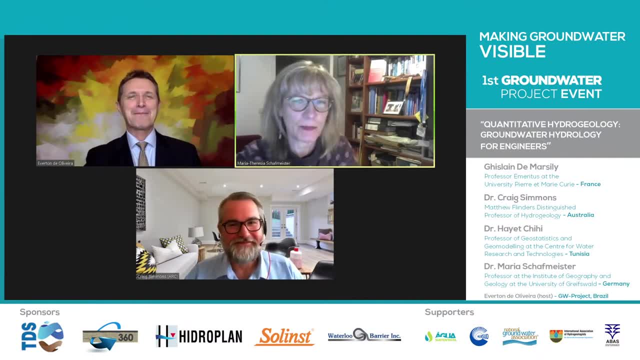 I'm not sure whether I understood the question correctly, but the fingerprints of Guillaume. I think it was really to put geostatistics. I think he put geostatistics into the context of hydrogeology. Guillaume de Marsilly was already a brave geostatistician. 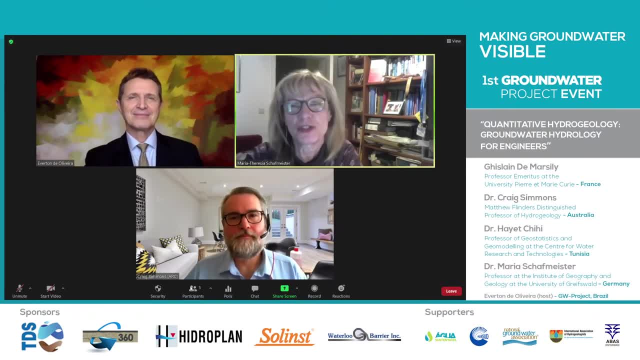 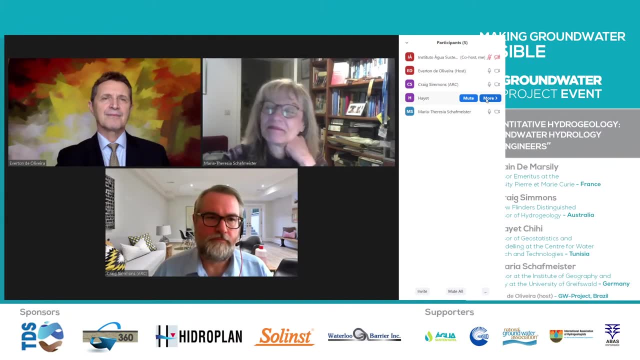 but then he put this knowledge into hydrogeology and this is something which still holds. I'm not sure whether I understood the question correctly, but the fingerprints of Guillaume, I think I can rephrase the question. The question is: 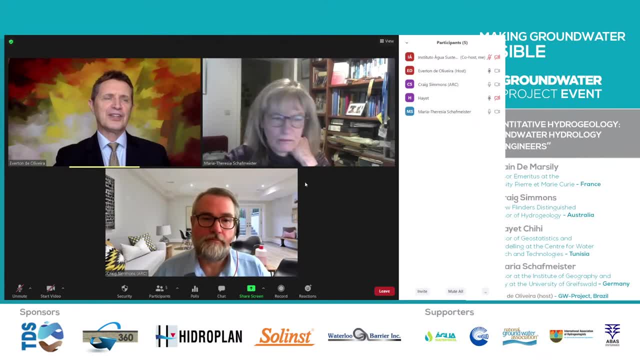 The context of hydrogeology. When you see, When you see the. Could you please turn off your presentation, because you're listening to it there from there. I can't hear you. Okay, I muted her. Okay, now, it's sorry for being impolite. 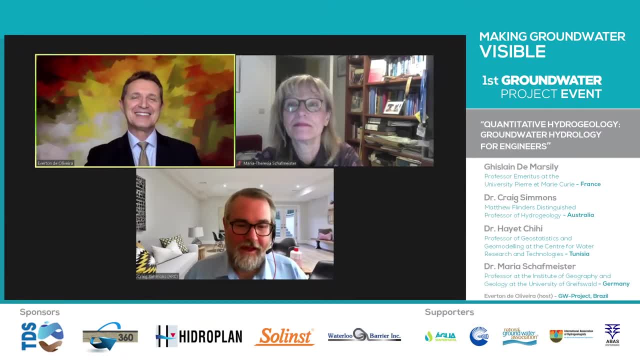 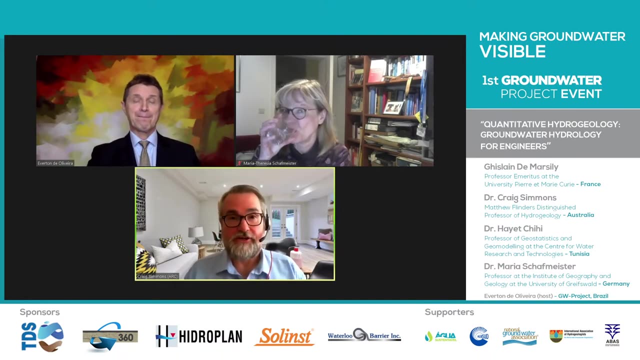 Can you answer that, Craig, please? Yeah, look, I think that obviously Ghislain's background was in geologic engineering and he always had a big interest in the geology but also the engineering and the mathematics. So he's always had an interest in the field side of things, but especially 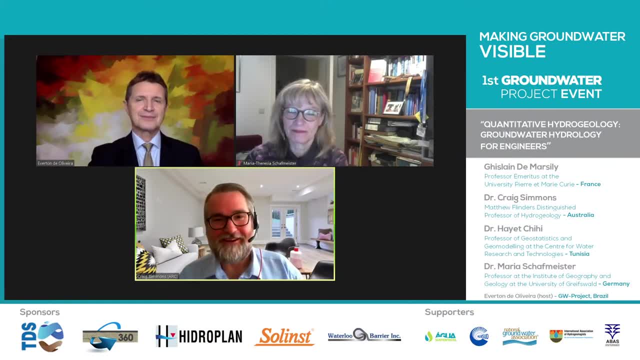 and he said it in his talk about, you know, his professor not thinking he'd get into hydrogeology because of not going into the field and so forth, but he loved it And so he always had an interest in the mathematical and quantitative and the modelling and so forth. 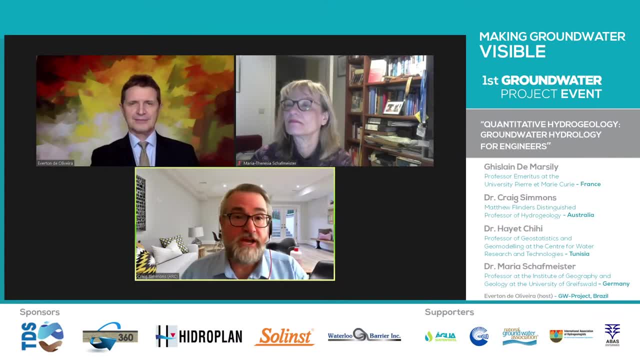 but not exclusively, And so the genesis of the book was out of teaching For the most part, because I know that he was putting lectures together, you know, often at the very last night before giving the lectures, and then he had a whole course. 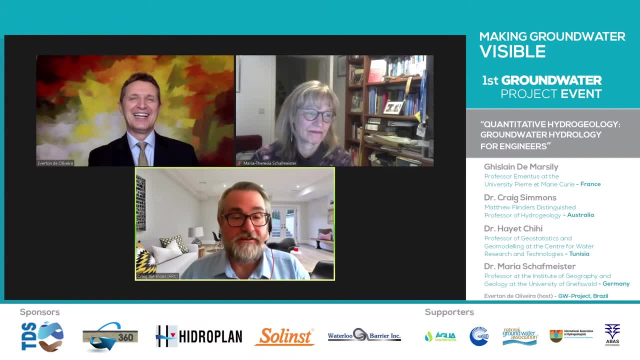 and thought, gee, this could be an interesting thing to put together as a book. So I think in a way this also reflects Ghislain's passion and interest and dedication to teaching, And the teaching in a sense was the motivation and the genesis of the book. 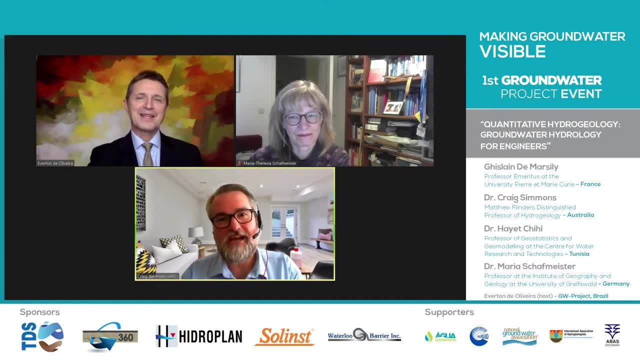 And now all of that was in the future And the French edition and then translated by Ghislain's wife, Gunilla, into English and so forth. But I think it's that quantitative interest but also a desire to teach. Ghislain loves teaching and getting information out there and working with people. 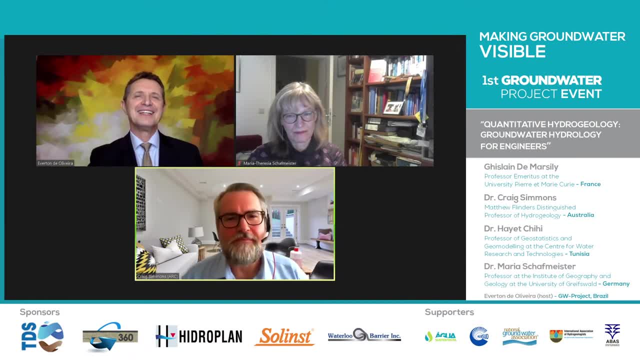 And I think his book's been a terrific mechanism and medium for achieving many of his own personal goals and motivations. But I think that The point of the question- I think that was missing there in the answer- is: like you, Craig, you're writing a book right now for the Groundwater Project, right? 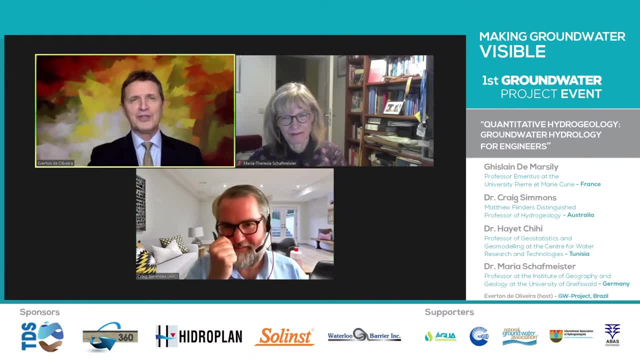 Yeah, You're writing a book. And I mean, when you write a book, your writing style shows something about yourself, right? Or usually we try to hide when we write technical stuff, But authors always leave a fingerprint on that. You can't. 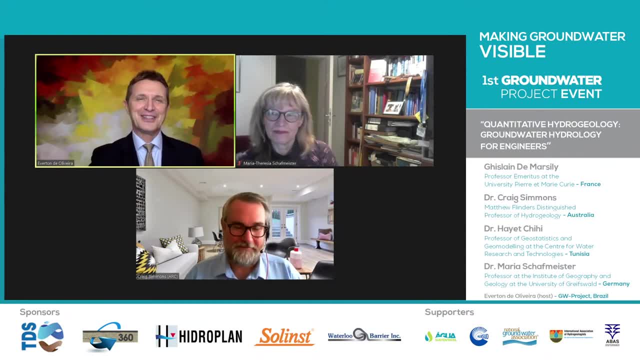 You can tell a little bit about the author when you're reading something, And so that was the point. When you're writing science, when you're writing an article, it's very simple, because it's too dry, You know. you just go for the very specific of the science and no space for explanation and discussion. 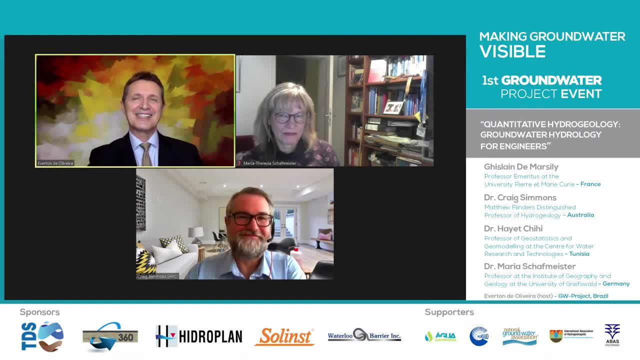 So what would you think is his fingerprints on his book? Because you've read it, I think Attention to detail and also being a perfectionist as well. So no stones are left unturned, but also a happiness with equations, And not all textbooks are quantitative. 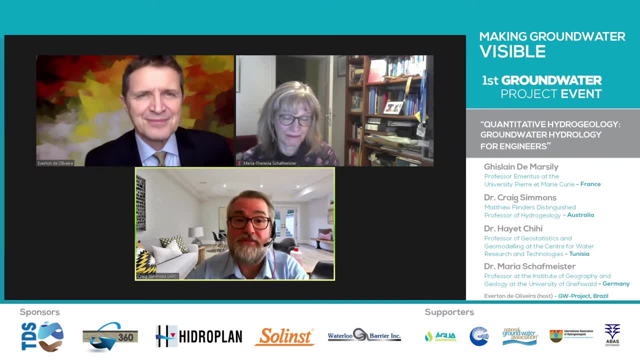 And in hydrogeology. not all textbooks are quantitative And I think this was a very deliberate part of Gilan's way of thinking, et cetera as well. So there are very There are various fingerprints that come through for me. the attention to detail, the perfectionism, the comprehensiveness, the happiness level with mathematics and the emphatic desire to have quantitative dimensions in that book was hugely driven by Gilan's own personal inspiration and drive. 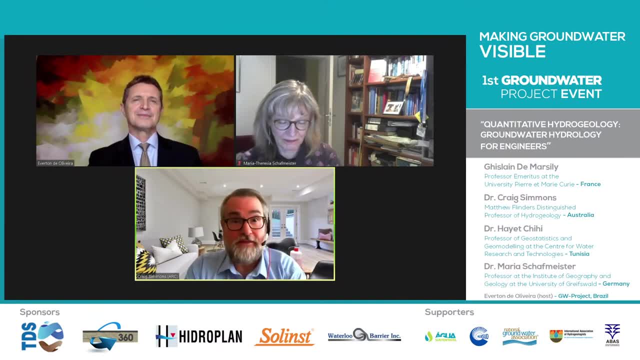 And. But also there's an entire chapter in the book on geostatistics which I think was It was pretty novel for the early 1980s in a textbook And that came out of Gilan's interest working with Georges Matheron and Jean-Pierre Delon and others on that. 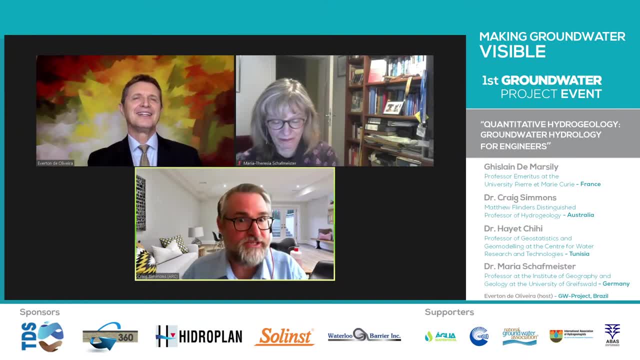 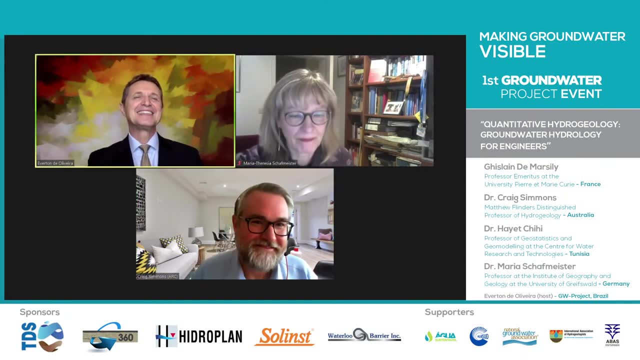 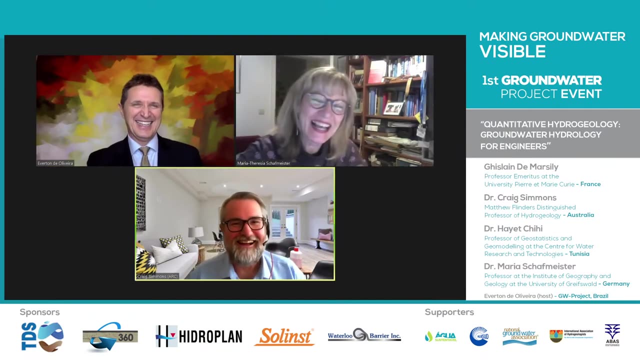 And that's a huge fingerprint of Gilan's own personal interest and work. You want to say something, Maria? When we were talking, I was just looking into the book again And there's one thing I think which is really characteristic for him. 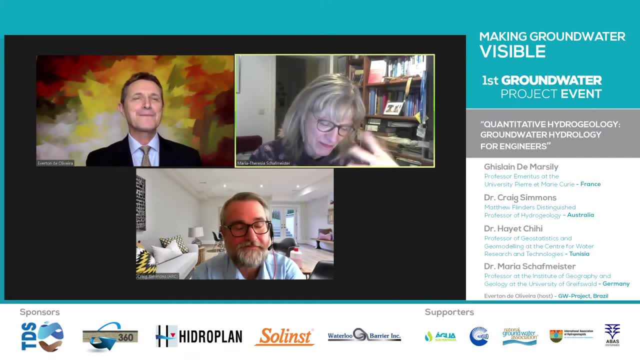 The very simple black and white sketches. Nowadays we are familiar with colored and even animated pictures, And he has very distinct, very simple black and white pictures which make things extremely clear. There is nothing around it. No, No decoration, It's just the fact he's trying to show and to illustrate. 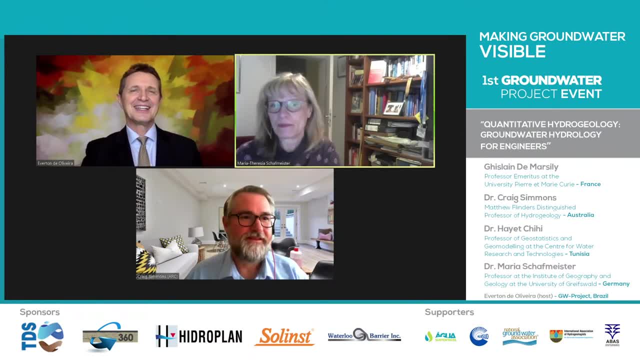 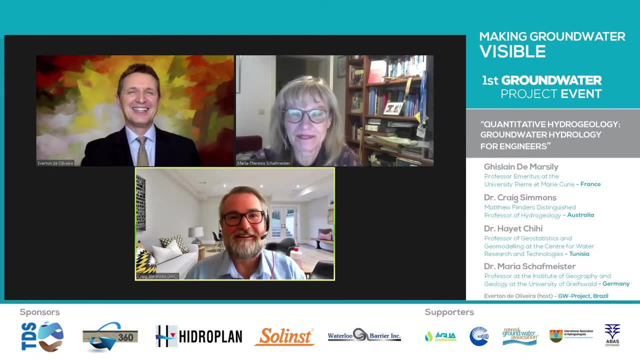 And this is something we can still use today in black and white, And it's a great point, Maria, And if you've ever seen Gilan give a lecture- and a number of us have seen Gilan teaching and giving lectures and they're amazing- 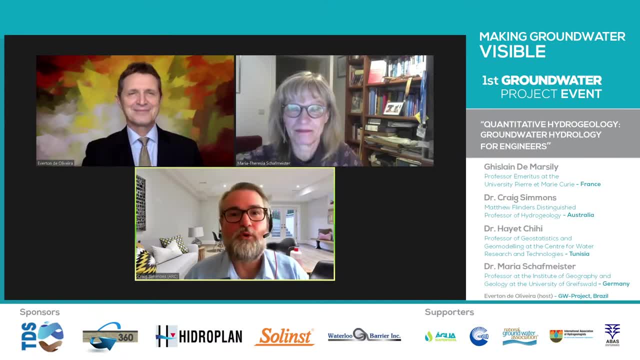 Because he has this remarkable ability to get on a blackboard with a piece of chalk or a whiteboard now with a text, And draw a picture that boils it down to the most salient fundamental features And it reflects just the incredible intellect of the man really. 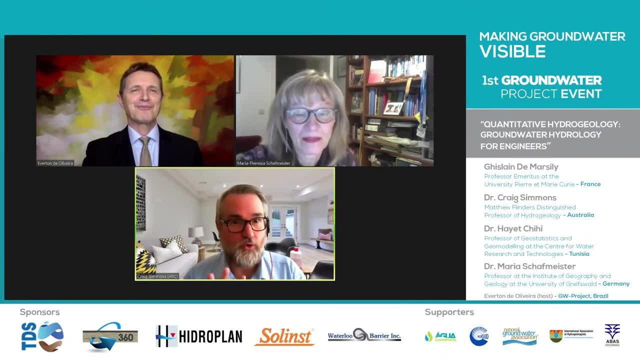 He can see right through to the most crucial parts of what needs to be explained, And I think that's why he's an outstanding teacher, And I know that his students- all of those that I've spoken to- have said that as well. 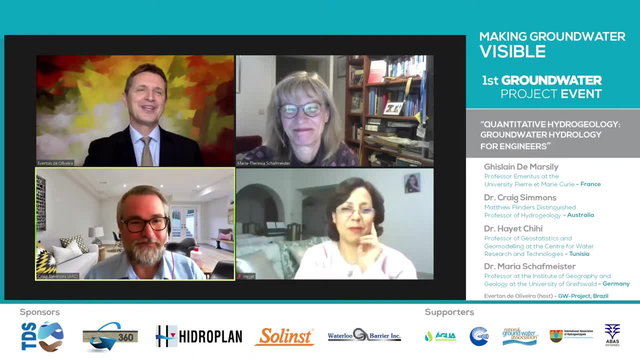 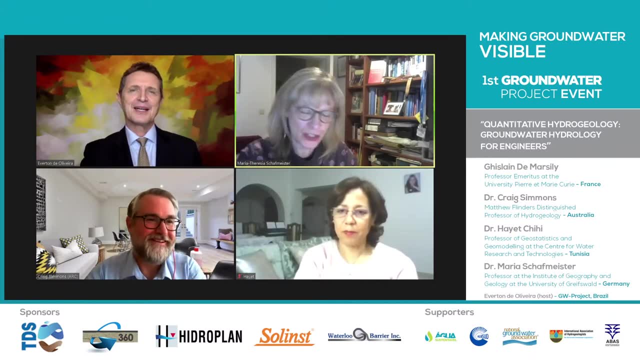 And it reflects Maria says in the textbook. If I may add something, there's just one picture in the book which is not a black and white sketch, but it's a photograph which he take in North Africa. He did not take this photograph, but it's about a well digger. 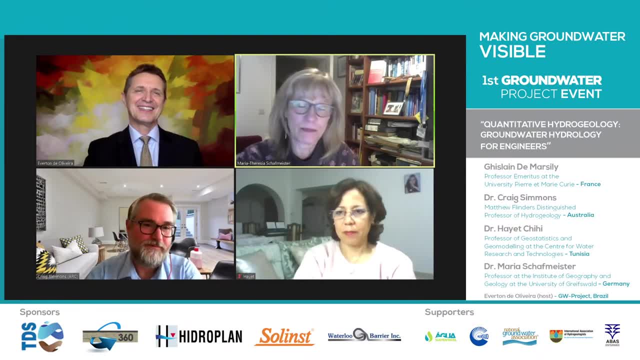 And I always show this picture in my lectures, in my very first lectures on hydrogeology. I show this picture because it also shows his big respect for our subject, for groundwater, for water. So it illustrates what human beings do to get water. 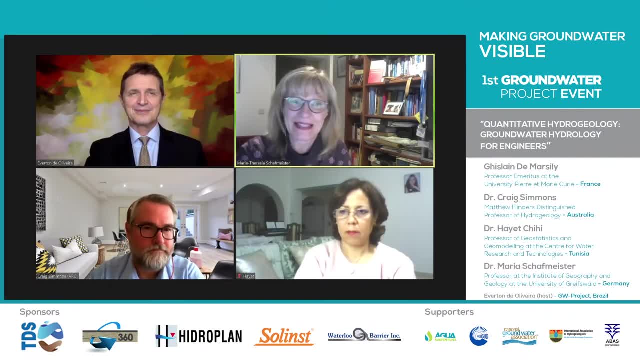 digging 80 meters deep wells by hand and not being sure whether they survive this digging. So this picture I love and it's the first picture I show to my students from this book. So sorry, I had to add this. I have an idea. 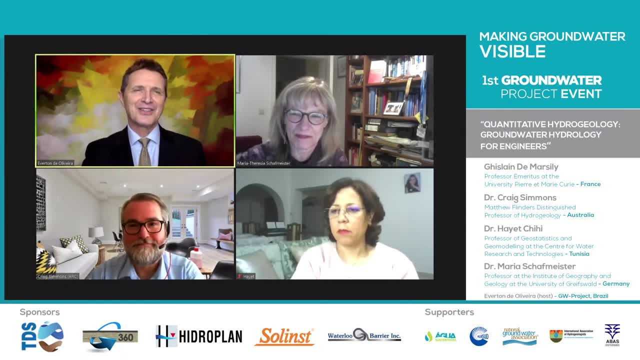 When we talk to Guilan, he has this: you know he's such a kind person, you know that's himself, And the way he- you know he tackles the subject reflects that kindness, because even you know the tough subject. 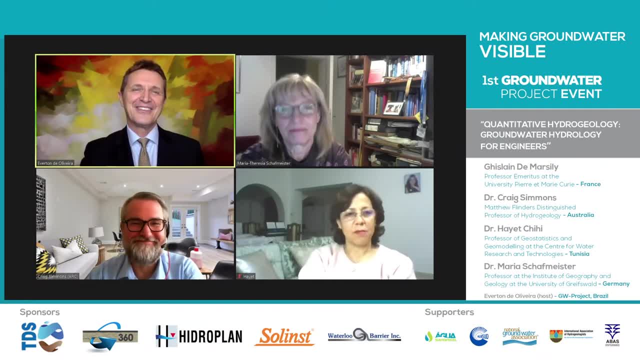 you know you go there and it looks smooth, right, when you're reading the book, And I think this is that relates to the author quite clearly. Because, when you, because for me, I first studied and then I met Guilan, right, probably same with you guys. 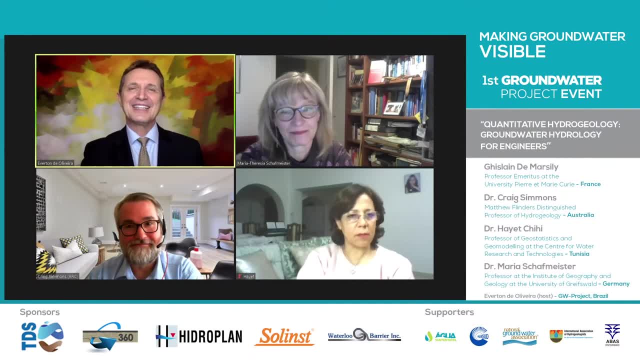 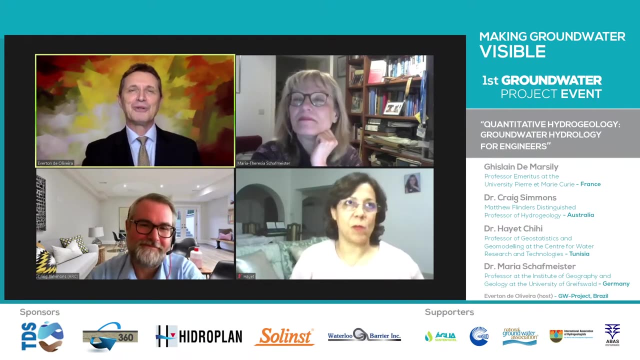 And that is exactly what we see. Hi, you were Guilan's student, right PhD student. What do you think about the relationship between his writing and his personality? That's what we're talking about. You have to unmute yourself, please. 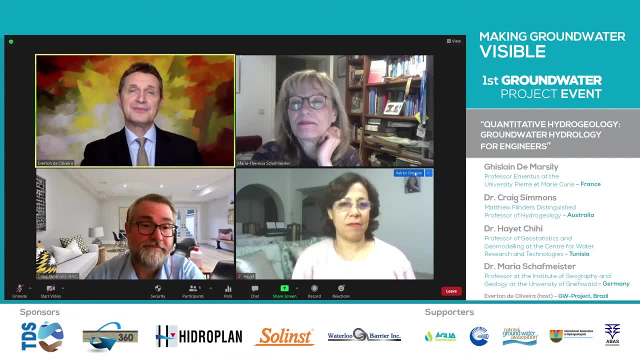 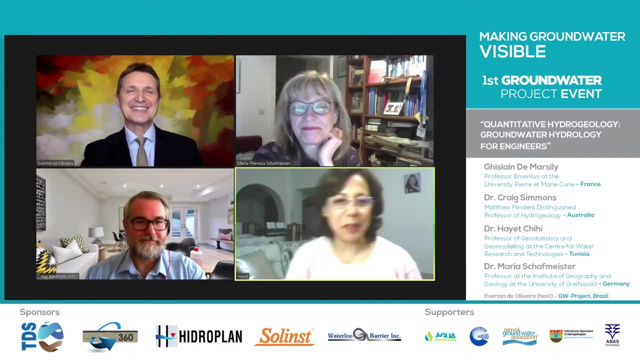 You have to unmute yourself. Your phone is muted, Please, Okay, Hi everybody, I think there is a link between his personality, his way of teaching and his way of writing. He writes in a simple way and he's treating people. you know, as if they were his friends. you know, and he's treating people as if they were his friends. you know, and he's treating people as if they were his friends. you know, and he's treating people as if they were his friends. you know. 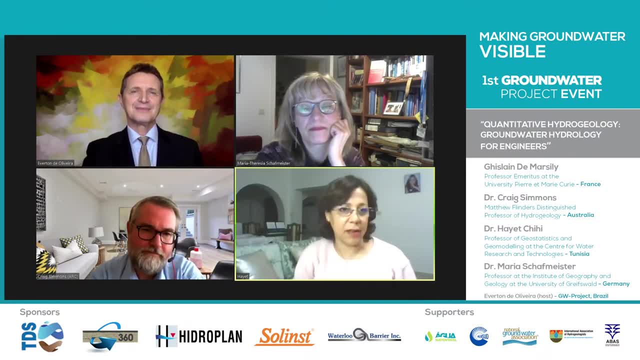 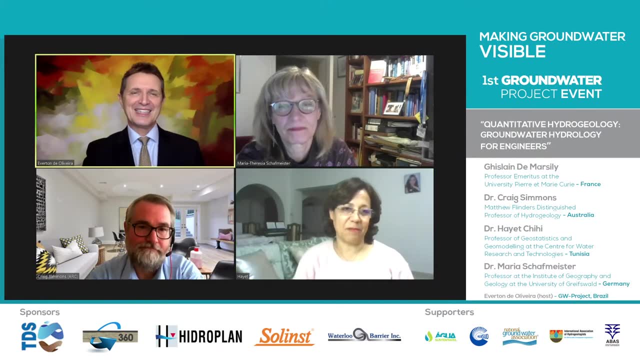 and students in a simple way, innocent way, generous way. That's it, That's true, That's true. Well, there's a question here from, let me see, Luis Hernandez. I think that goes to Maria, I think. 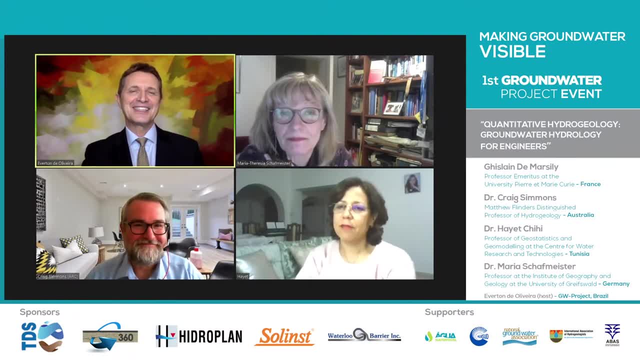 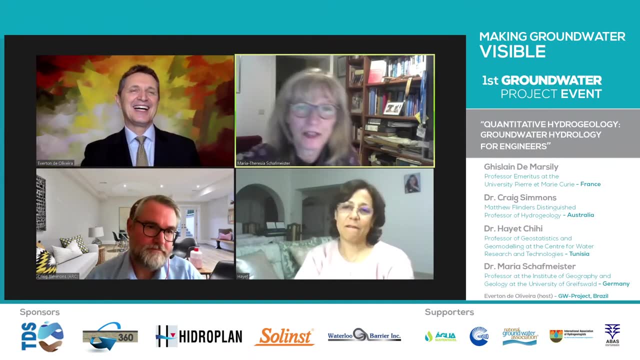 Doesn't geostatistic limit our understanding about how groundwater is seen? Does geostatistic limit our understanding about how groundwater is seen? Does geostatistic limit our understanding about how the geosystem works? I don't think that geostatistics limits it. 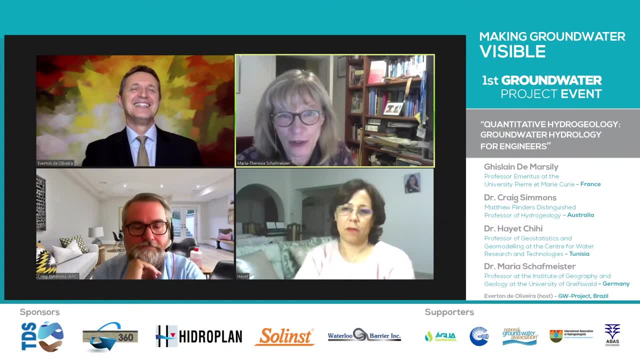 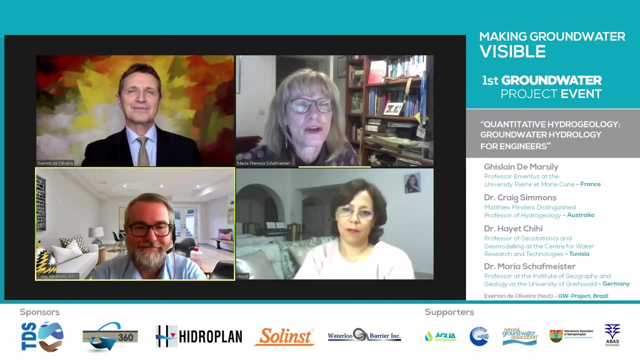 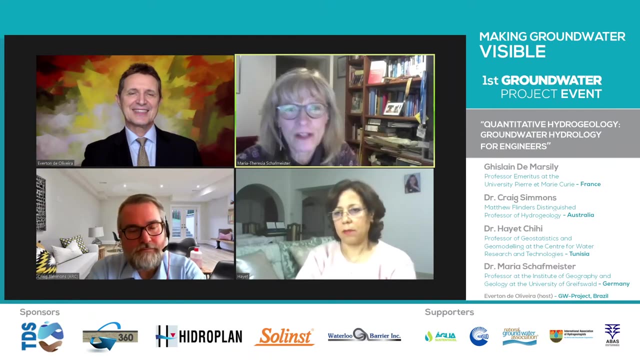 I think geostatistics enhanced our knowledge. As I told you earlier, I was sitting in a conference this day, which is on nuclear waste disposal sites, And every minute I was listening to all those talks, I found out that, you know, there's a lot of information. 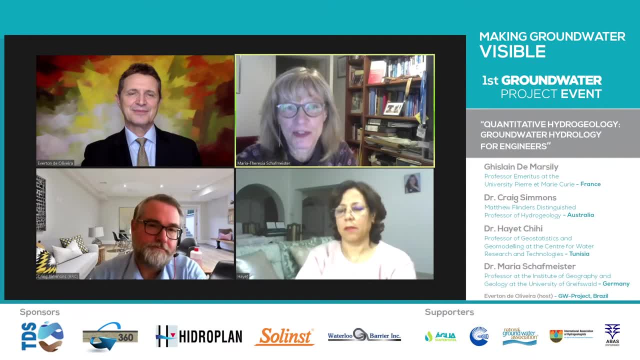 There's a lot of information. You know there's a lot of information. There's a lot of information. There's a lot of information, I think you know, describing heterogeneity of the subsurface. that is exactly the question. 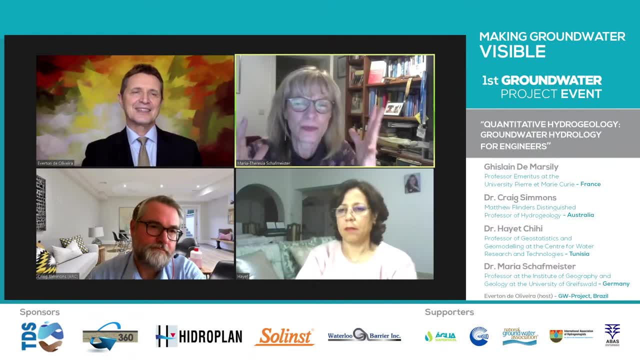 We can calculate so many things, we can build models, we can have ideas, but we never will be able really to describe the heterogeneity. And the first step to do this was geostatistics. And so no, geostatistics does not limit. 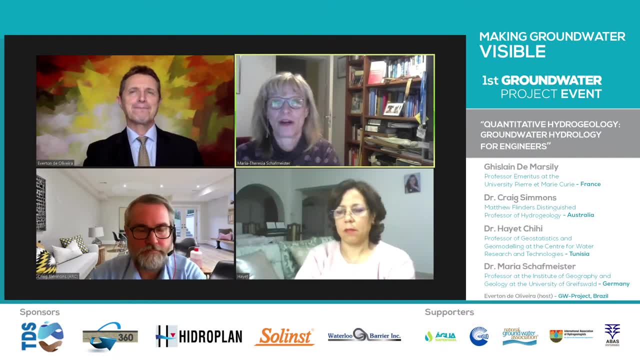 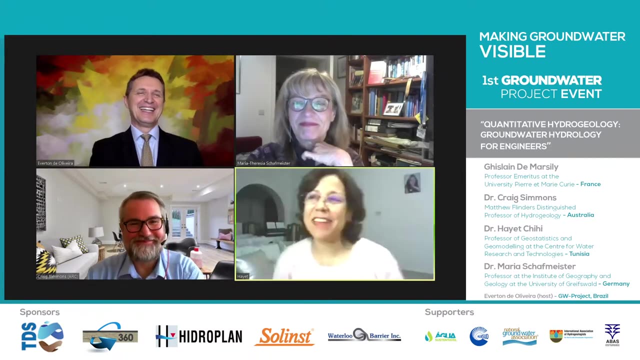 but it's one step. but enhance, as i understand, our understanding of fluid flow in the subsurface. totally agree, hi, i have a question for you, hyatt. i think that, uh, you're afraid of my my questions, but i'm going, i'm gonna do it anyway. 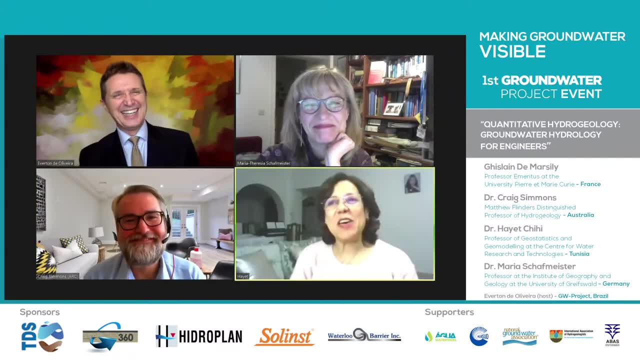 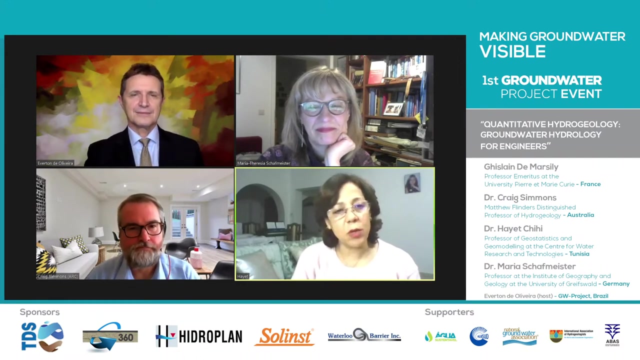 no, i don't think that. i don't think that the geostat sticks limit our knowledge about or our calculation when treating with geological modeling. in my experience, for example, the the, the only way to integrate multi-source data is by using geostatics in aquifer modeling we have. we don't have much data, so we have to expand data. how to extend? 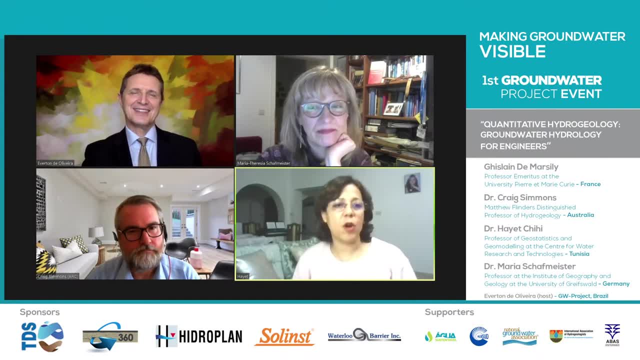 data from outcrops, from end of burr holes, from geological knowledge, and how to transform that into digital data is by geostatics, i think, and as i i says, maria, the ambiguity when to to understand, uh, the process controlling the, the dynamics of water and the pathway of. 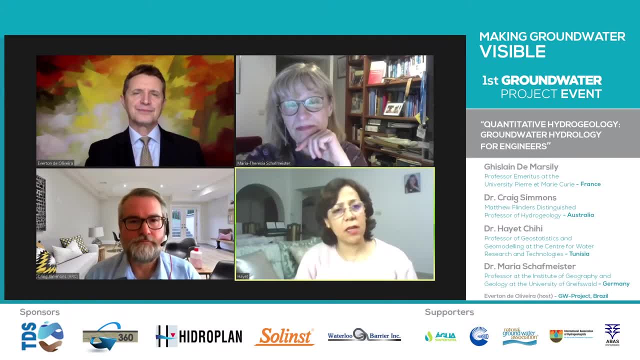 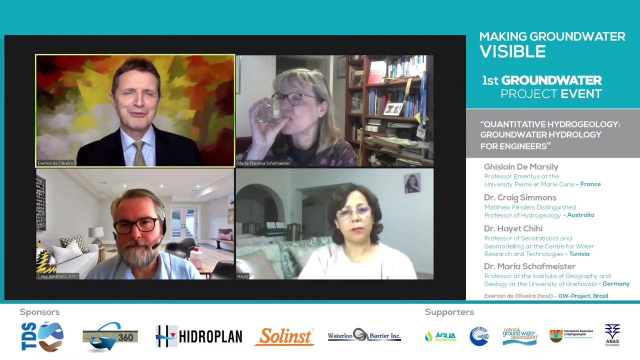 water is to understand the heterogeneity and the lateral facies variation. so we have to use the stochastic modeling and the stochastic simulation of facies to to understand the conceptual model of, of the the aquifers. yes, true, i'd like to thank some people here from the community today. uh, alfonso, there's a lot of good questions from um, from, from, from. 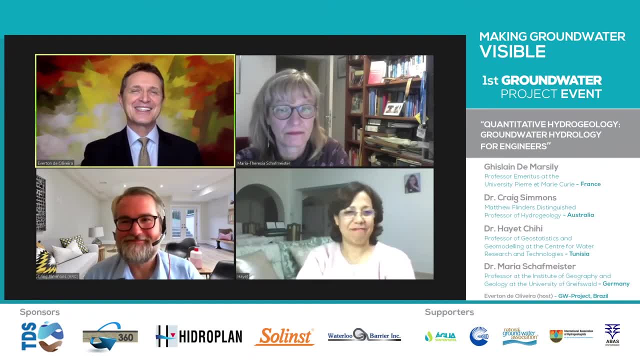 the? uh from the west. those are, um, some very interesting questions. to know is one question from an al-hamdi al-risa. i'm talking about vanuỳi from venezuela, uh from virginia, the al-samurai from libya, uh obun from uganda for being such frequent flyers with us. thank you very. 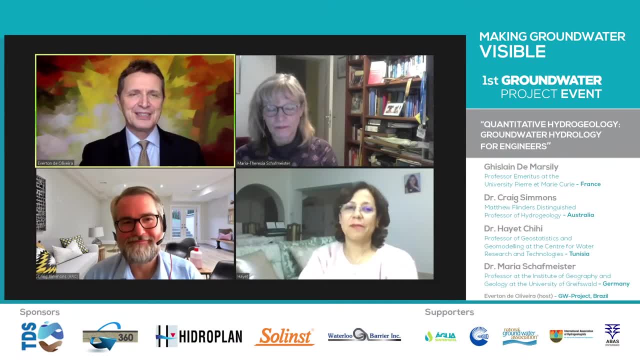 entered by Professor Demarcy. Yee, I have here Dick Jackins. Dick Jackins, ah Jesus, When you speak French, then it changes the. you know the way we speak, it gets better, Dick Jackins. Jackson says: 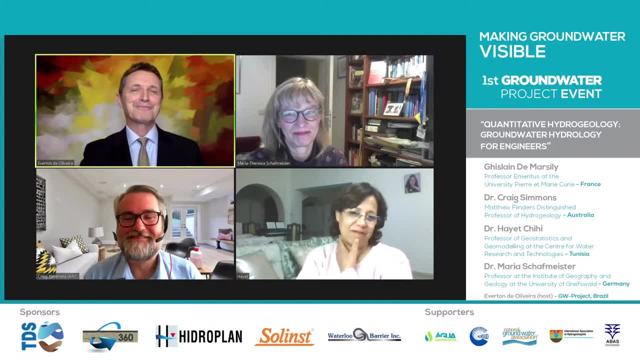 that's for Bern directly. Alessandro Cesarino from Brazil. Yes, Is there a an an intention to translate the quantitative hydrogen hydrology as ground water was like free to all? Um, I might try that. I don't think so. not for now, because 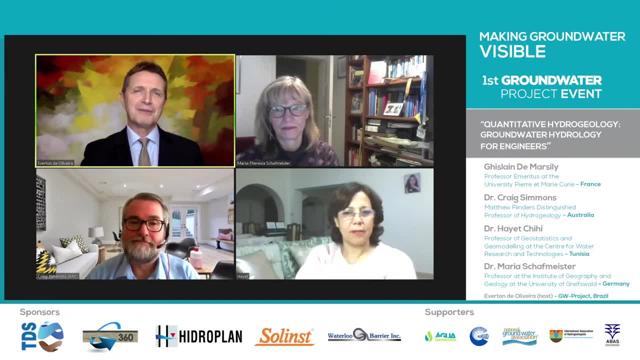 the rights I think are still with the publisher right. So the groundwater from Fries and Cherry, that was a long way to get the rights back to the authors so they would allow to translate and to distribute that for free. We have the same. I'm answering that based on the answer that we've got from Emilio Custodio and Llamas. 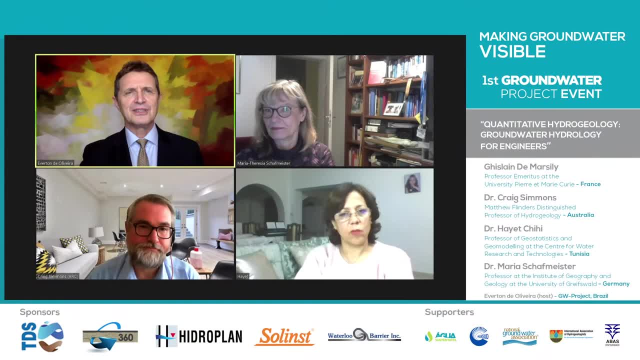 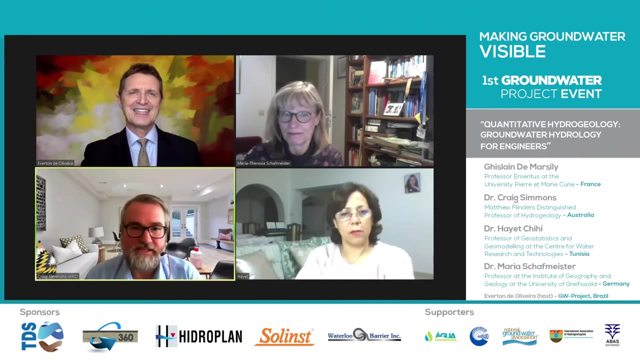 Their book also belongs. the rights belong to the publishers and they don't have the rights to distribute, so translations are still not free to anyone. Could you add something to that? What do you think, guys? Am I right? That's consistent. 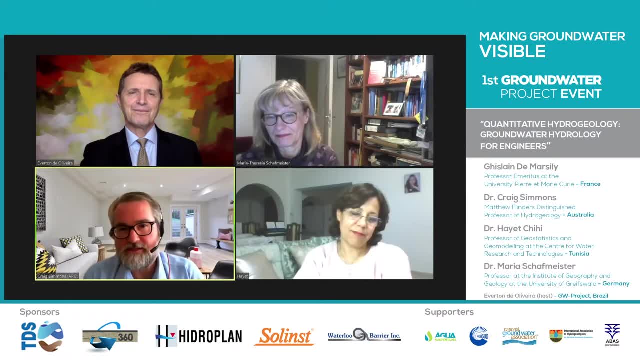 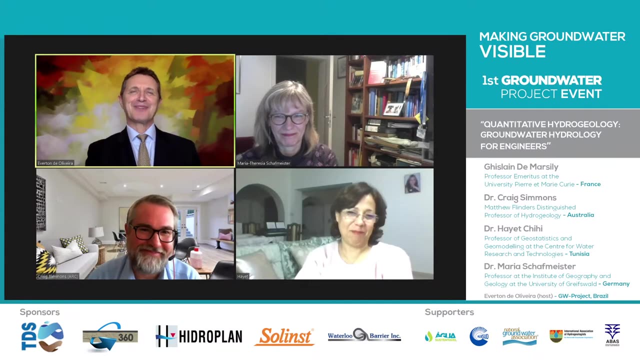 Fully consistent with my understanding, Everton, that the rights are still with the publisher, as with many other books, And so your answer is spot on. Very good. I have a question for you, Hayat. How was being his student when you were there? 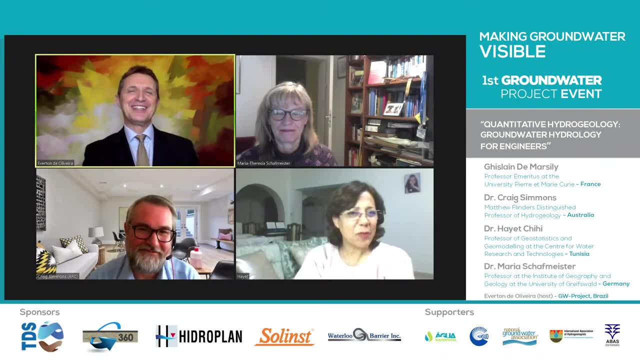 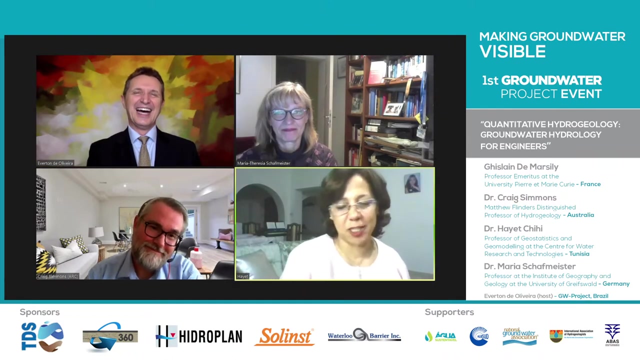 You know you told me a nice story because you were. you know you were pregnant when you were doing your PhD. That's hard work, Jesus Christ. I could hardly finish my PhD. This is a personal history. I think I don't know how to tell it in English because maybe you will translate for me. 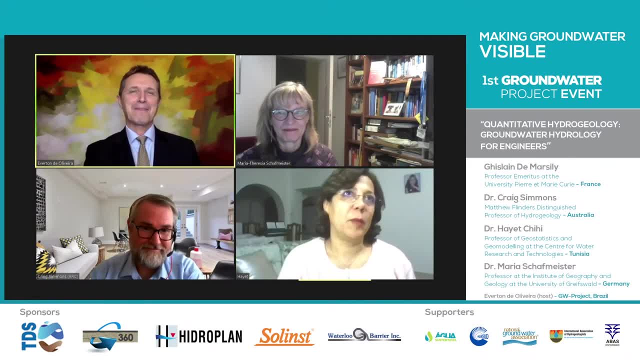 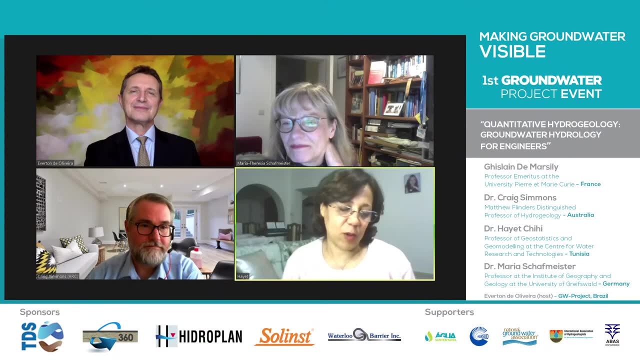 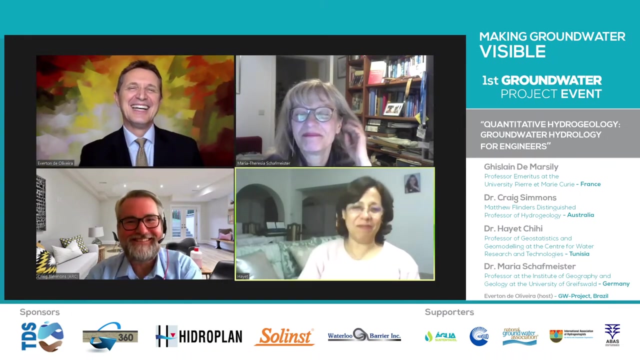 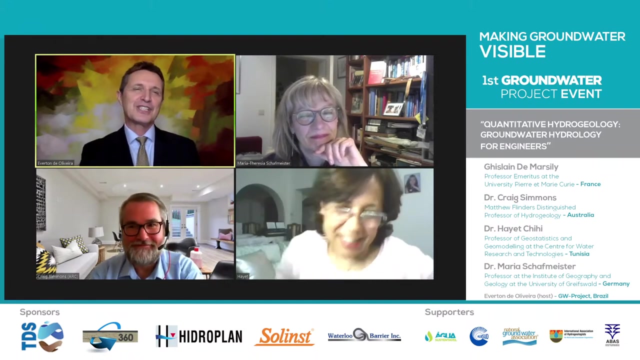 I can try. I can try. Last year I was writing my thesis. I'm not a good translator, Don't go too fast please. So you're saying that the Last year on her PhD she was working in the lab with Marseille and she was pregnant. 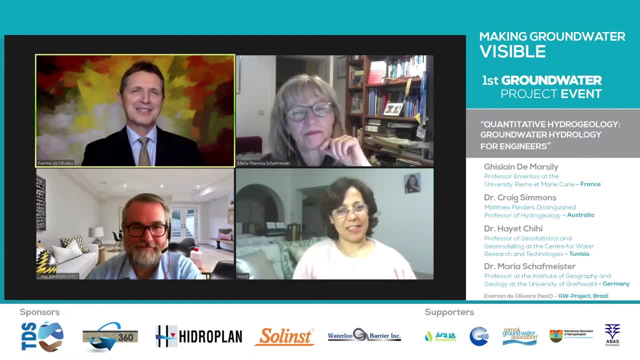 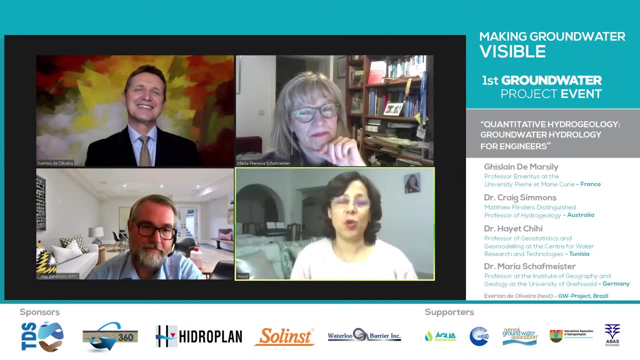 It was five months pregnant, something like that. Is that correct? Yeah, So I. So I tried at all costs not to meet Marseille because I don't know, For me it's the father. So I was wearing shirts that are a bit. 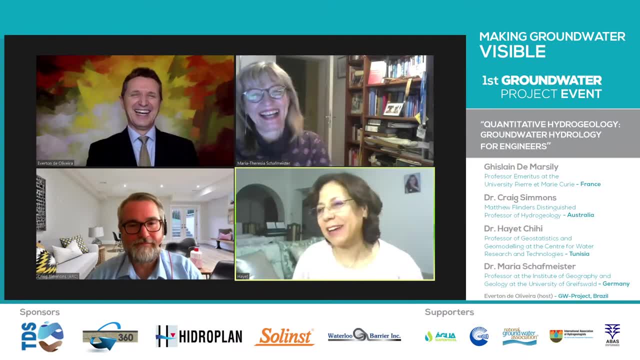 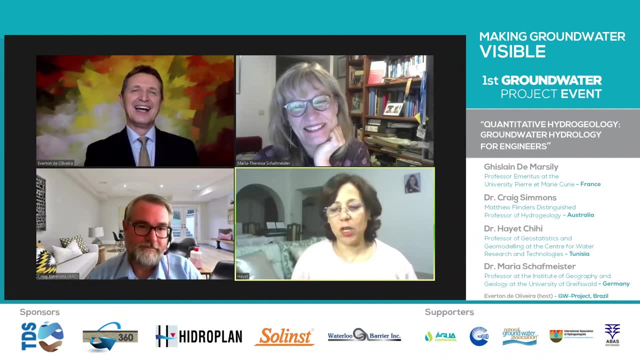 Vast to not, Vast to not. Vast to not. So I said that I wanted to continue to write my thesis and to do my thesis without people realizing I was pregnant, And to not cause them. you know, some pity. 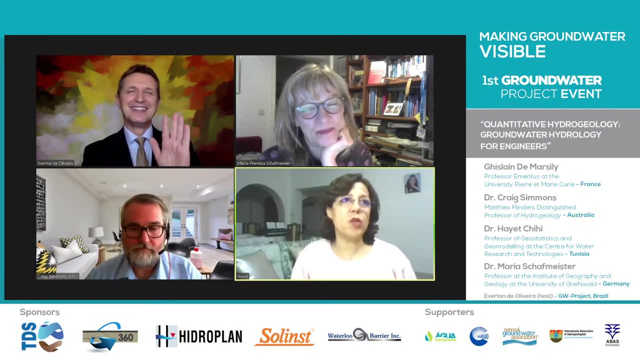 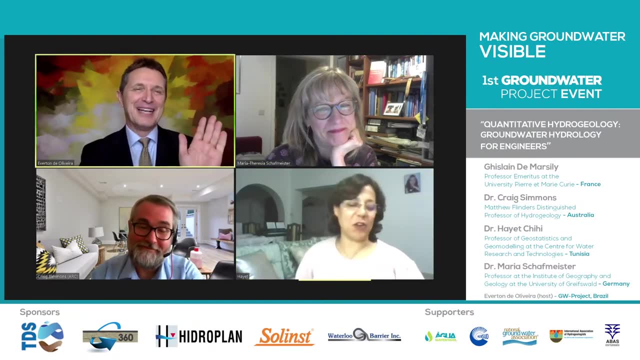 I didn't like that And I wanted to submit my thesis and then tell them: So, No, no, no, no, Okay, Okay. So she said she was a bit shy about that. She was concern about what would be Ghislaine's reaction knowing that she was, you know, pregnant at the 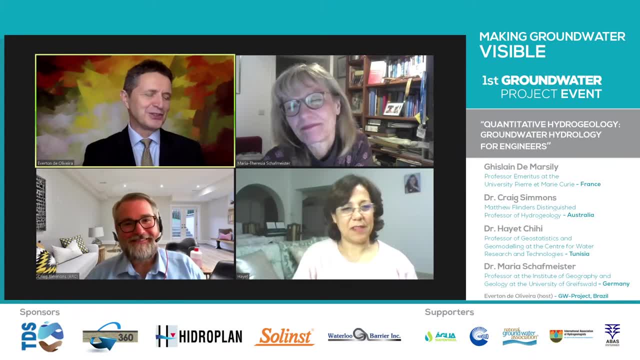 end of her PhD. She wanted to hand her, you know- her thesis before people know. in that situation she was using, you know, a bit loose clothes, not to you know- to try to disguise the situation. Please go ahead. So I will be finishing in two seconds. 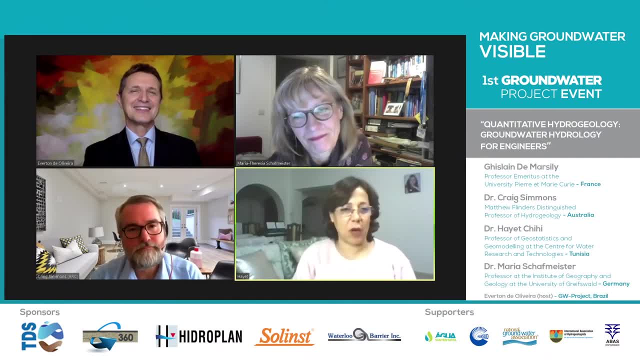 I went to the CNRS and they doubled my scholarship, that's it. And I realized that by going to the bank and I saw that I had a lot, a lot of money. I was happy, of course, but where does this money come from? 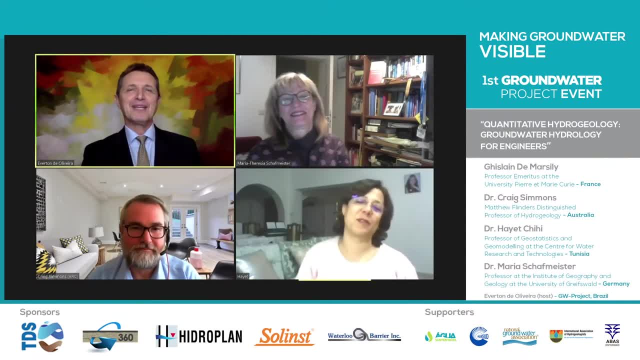 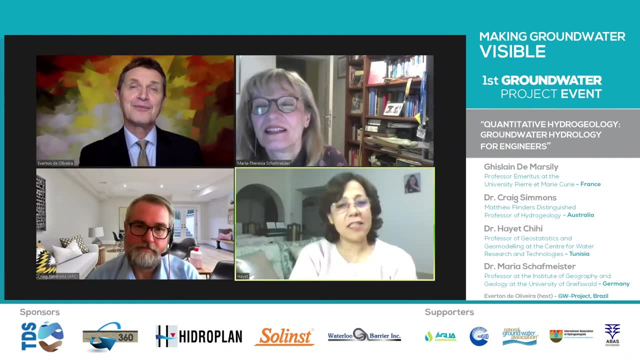 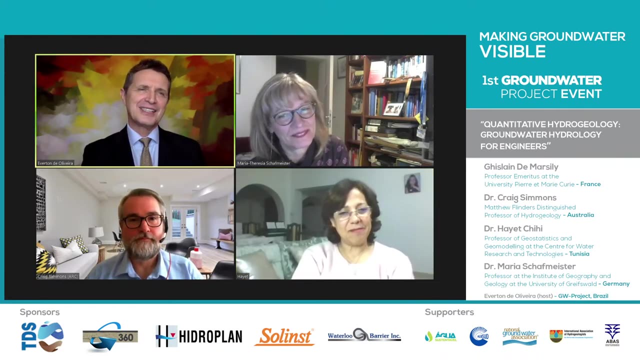 And then I realized that it was Marcini who doubled my scholarship. How is the number of professors of other professors? Christian Ravel, Christian Ravel. So she says that, although she hasn't told him the other professor, she had another, a co-supervisor. he mentioned to Ghislaine that she was a bit, you know, a bit tired because she was pregnant already. 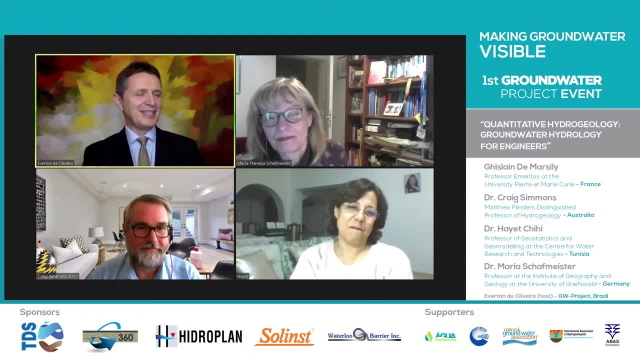 And without telling her she he just doubled her scholarship. And she just knew that at the moment when she went to you know the CNRS. And she just knew that at the moment when she went to you know the CNRS. 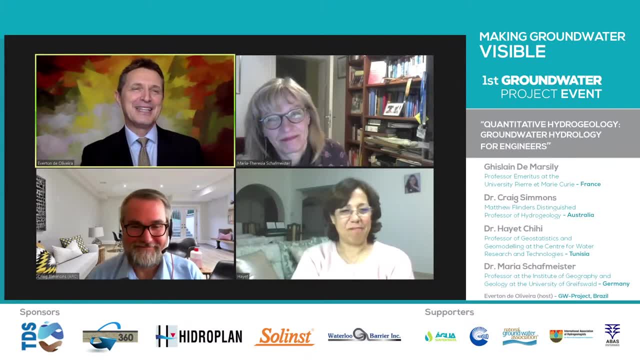 And she knew that at the moment when she went to, you know the CNRS, And she saw that there was way more money that she was expecting, And that was kindness from him, Thank you, Thank you, Brian, That's really a nice story. 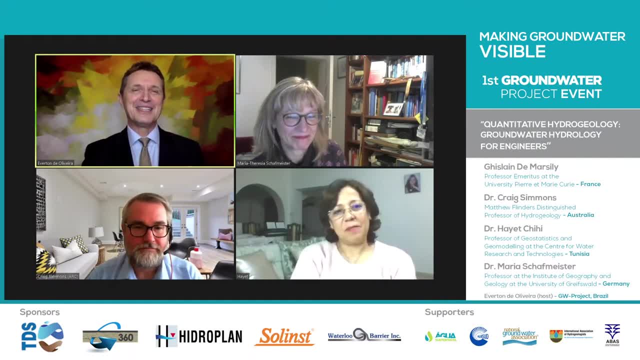 Yeah, Yeah, that tells a lot about about Guian. It's very nice And that was. you know, she was high at once at the same time, taking PhD at the same time. Yeah, Yeah, Yeah, yeah. 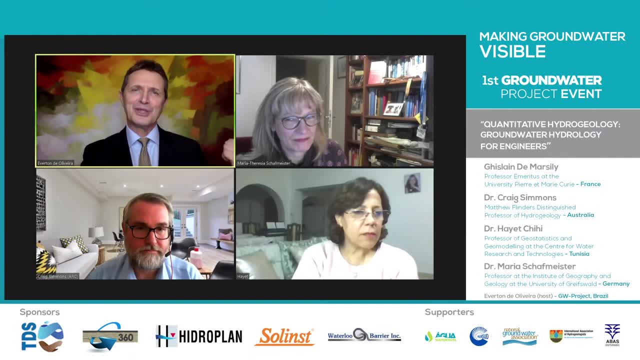 Yeah, phd, at the same time when i was in waterloo. you're in paris, right? good guys, i know we're talking and, uh, we're having fun here, but our time is short and we have to finish. i'd like you to put a good word. 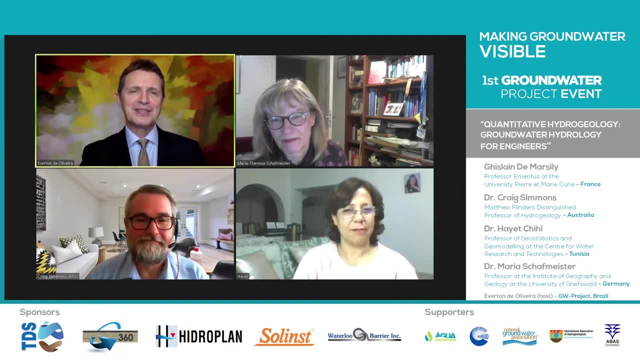 to about the the marci, and to people that are watching us here so we can wrap up our presentation today. i'd like to thank you for participating. please, who's first? okay, maria you. what can we say? i know because, because you said it, because it's late in germany. 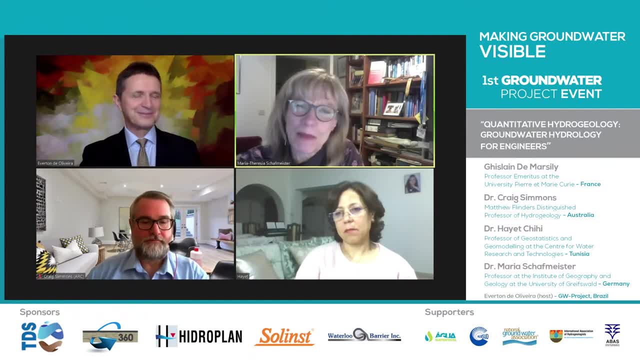 what i want to say about guillermo. i think he's one of the best friends and colleagues and teacher, of course, but first place friends i ever had- and i still have, hopefully, and he's so generous and we had so good time together and uh, well, i'm really glad that i. 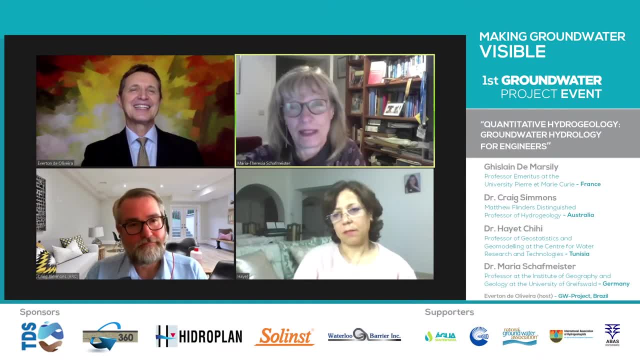 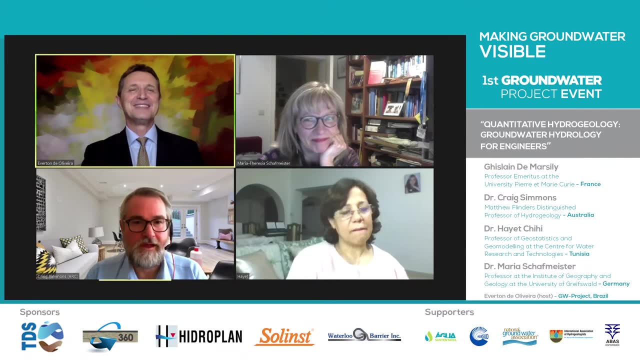 once met him and that i have the honor to be one of his friends. thank you very much. very kind, you're great. um, yeah, look, i fully agree with maria. uh, as a scientist and an engineer, ghilan has made so many pioneering contributions, uh and seminal. 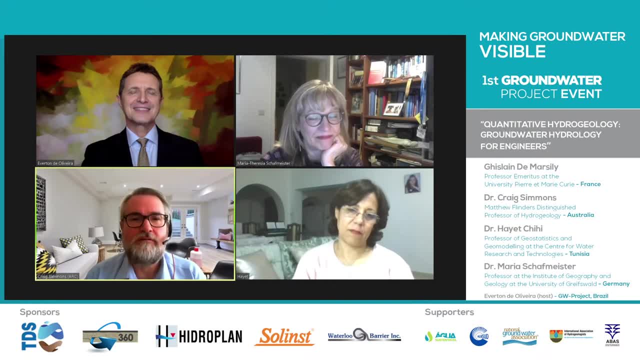 contributions to hydrogeology, and- and there are so many of them- from fundamental research, contributions in things like geostatistics and and many other areas, but also in really understanding applied issues as well, whether it's food and water and energy, working with african colleagues and really coming back to the issue of the textbook, ghilan's passionate about. 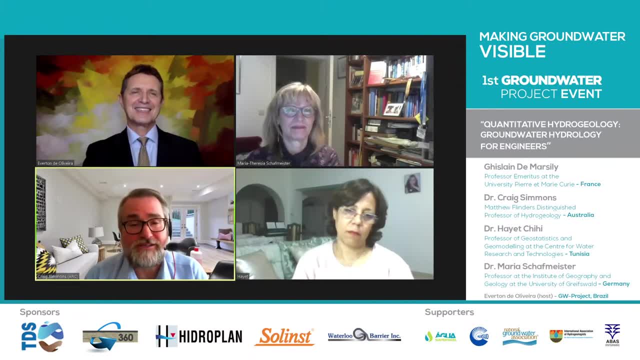 people in other countries, africa and elsewhere. it just speaks so much to him and the way he thinks and how he feels about the world, um, and and teaching, um. there's just so many ways he's contributed and given so much to us in hydrogeology. at a personal level, um, like maria i, i feel. 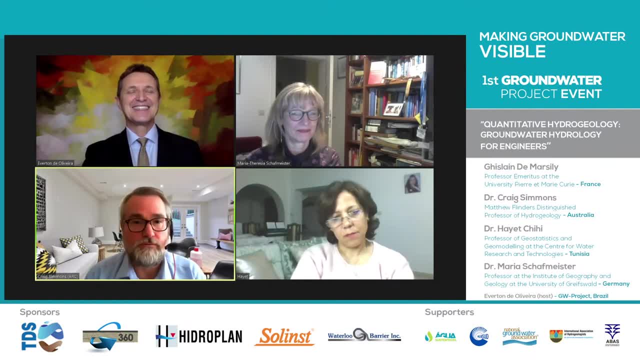 tremendously privileged to have had the opportunity and the good fortune of meeting ghilan and knowing him uh now for for a while and and it has been literally life-changing. he has been an advisor, a mentor, always happy to answer questions, to tell you if you're doing things that are good. 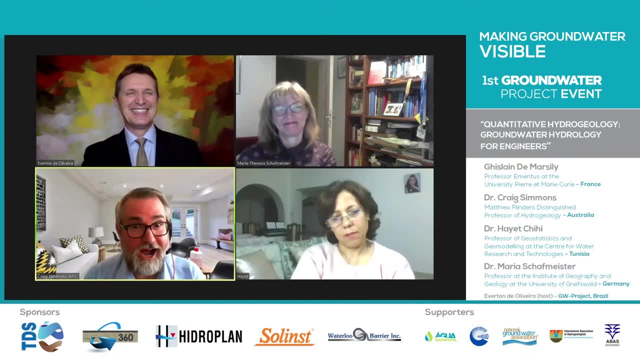 to tell you, when you're not doing, things that are that are right or how they might be done better, and the advice is always incredibly smart and incisive and caring. it comes from a really genuine place in ghilan's heart and he is a very 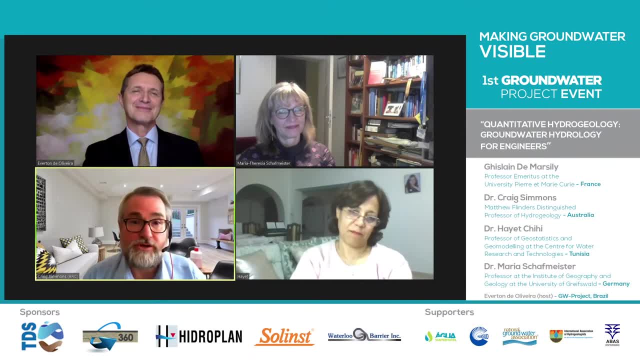 kind, generous and very selfless person who has given so much of his time and his life to hydrogeology, to research and and to students and so forth. um, and so i also like maria phil, but it's a real privilege to have ghilan as a friend. it's been amazing. thank you very much. great, nice work. 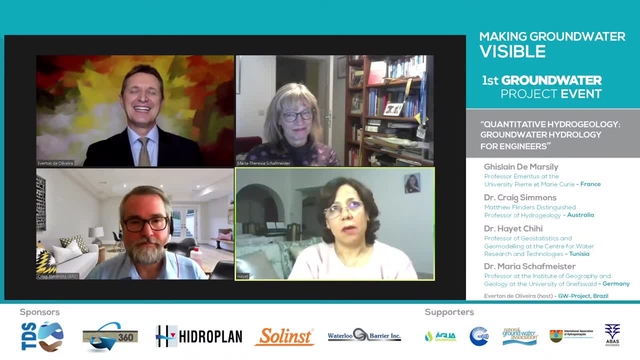 uh, what can i say? i'm still impressed by ghilan and marceline. uh, his way is to to work on uh too many subjects to with too many people, with everywhere in all over the world, and i'm impressed uh uh of his uh moving from hydraulics to geology, to hydrogeology, to geostatistics and to uh food security and to uh. 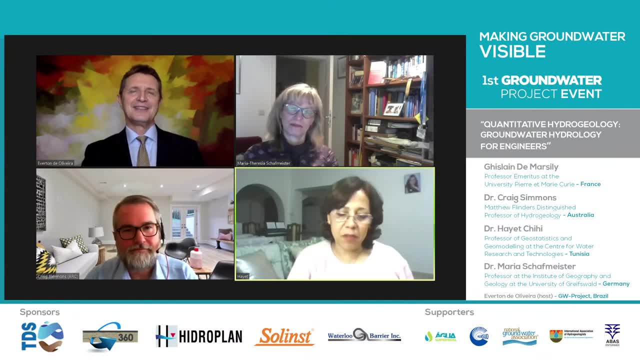 he's impressive also when, when, simplifying problems. and what can i say? simplifying the problems even when, when, when, giving lessons, when, when, resolving uh, pupil and pupil and students problems also, uh, the other thing which is impressing me, he is, he, he cont, he is continuing. 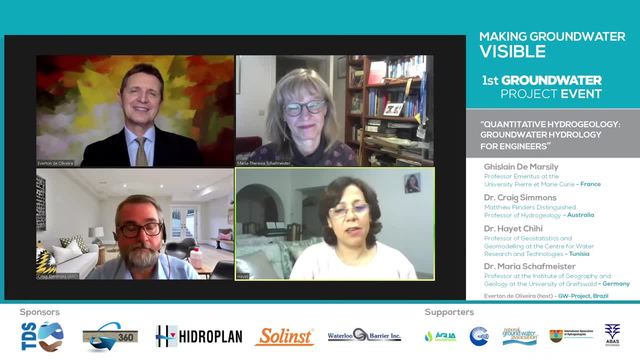 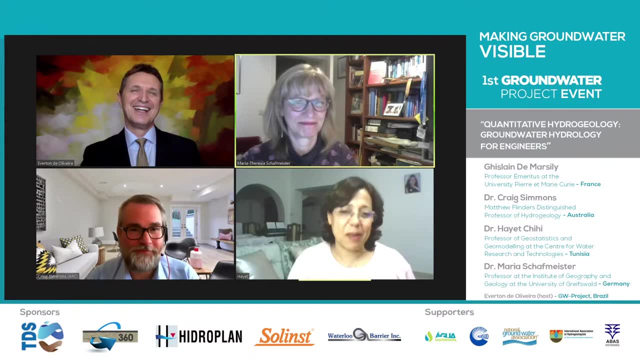 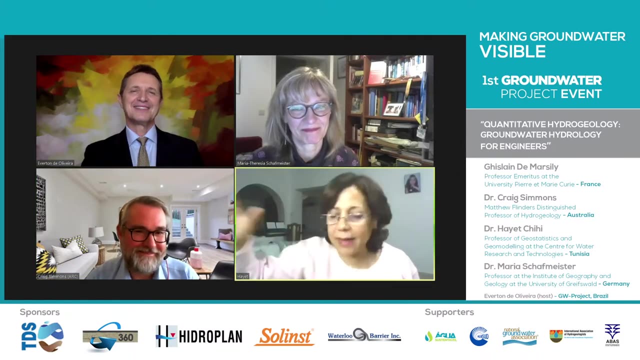 working until now at his age, and when i'm tired i say to myself: look at the mercy he's continuing combating. yeah, uh, one day i i i said i sent him the email, i am tired. And the next day I asked: what do you think to work together on that subject? 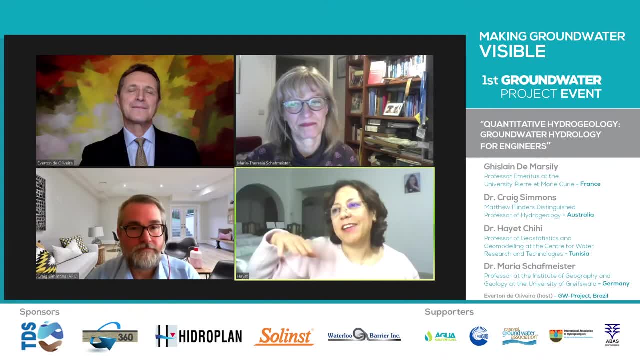 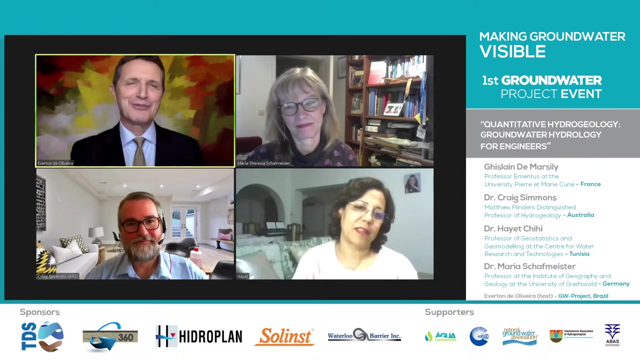 So this at his age now, I think that he's how to say in English: he's impressing, he's Very impressive. Yeah, Yeah, All right, Thank you guys. Thank you very much for your kind words and for helping us here, Actually, in our work. here we brought Guilherme de Marcelli. 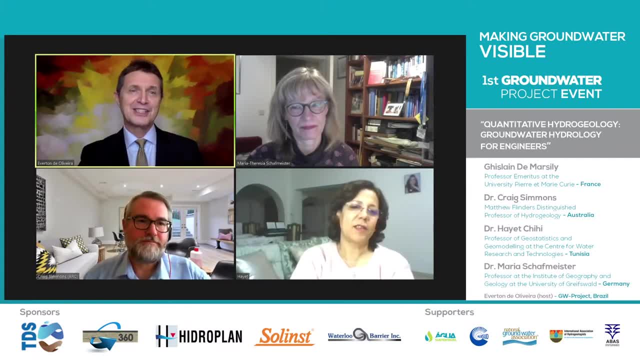 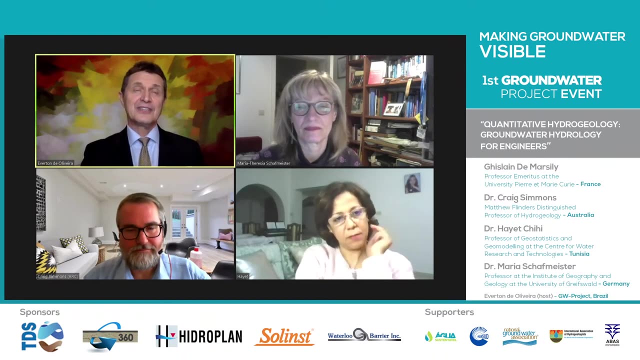 as we brought famous authors and we have not unfamous people like you guys. You're very, very famous as well in our field of expertise. in our field of expertise, To help us show our audience that doing hydrogeology- doing good for the world- is also fun. We have good people around, We have friends working, We're